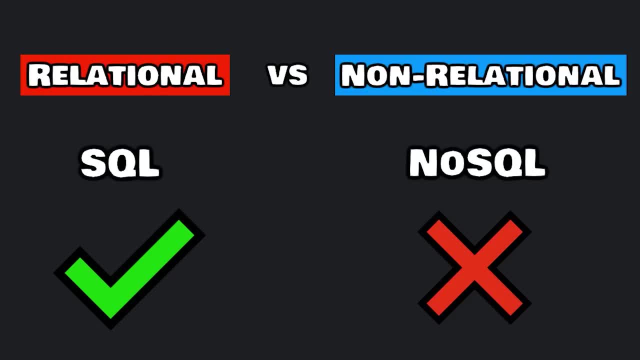 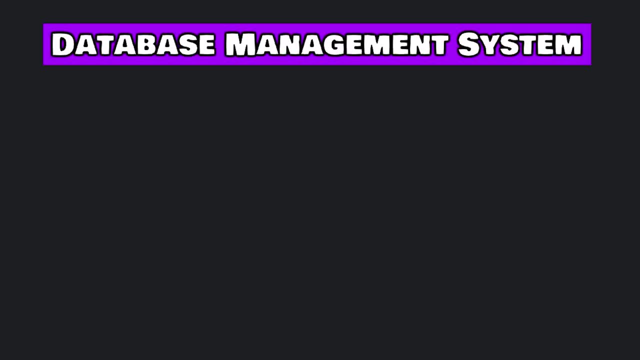 SQL series. we will be working with SQL and relational databases, So let's get started. Relational databases, not non-relational databases. To write SQL statements, we would need the help of a special piece of software known as a database management system. People. 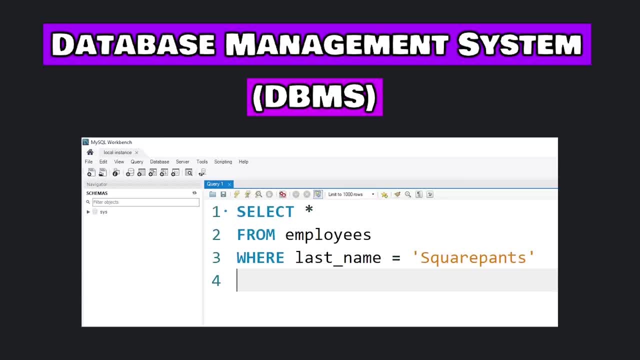 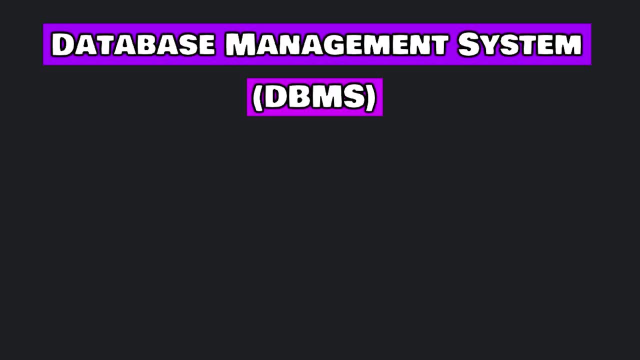 shorten this to simply DBMS. It's a workspace for us to write SQL statements and generally just work with our database. It'll make our lives easier. There are different DBMS systems you can use, one of which is MySQL, Microsoft SQL Server, Oracle and Postgres SQL. 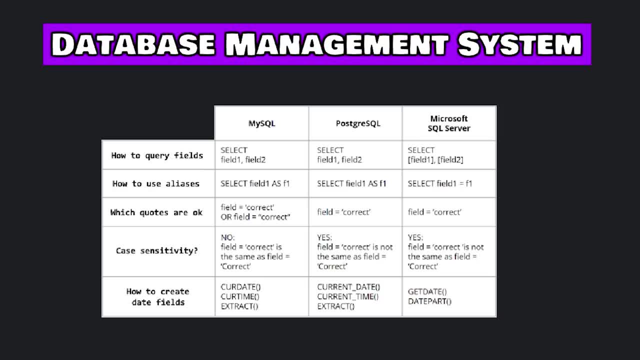 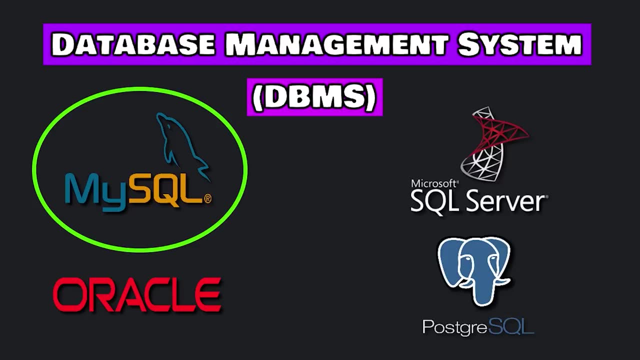 but there's still many more out there. Each of these database management systems all use SQL, but there's subtle nuances between the syntax of each database management system. If you're familiar with one database management system, transitioning to another will take little to no effort at all. In this series, we will be working with the MySQL database management system. 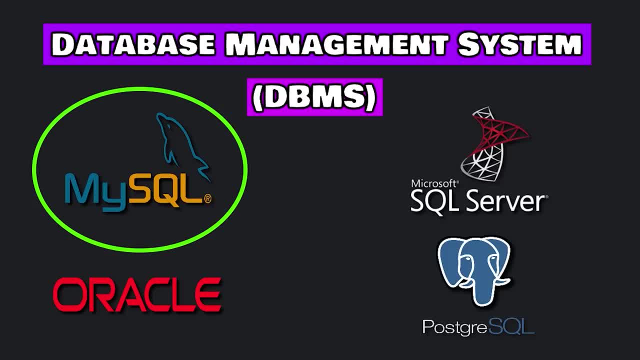 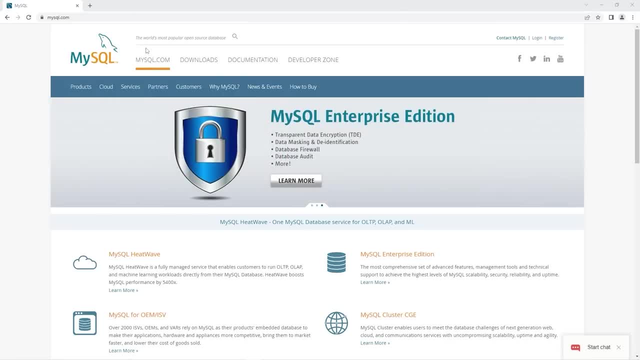 and I'll show you how to download that for both Windows and Mac OS. Hey everybody, in this topic I'm going to explain how we can download MySQL using the operating system. First of all, head to this website, mysqlcom, then go to the Downloads tab. 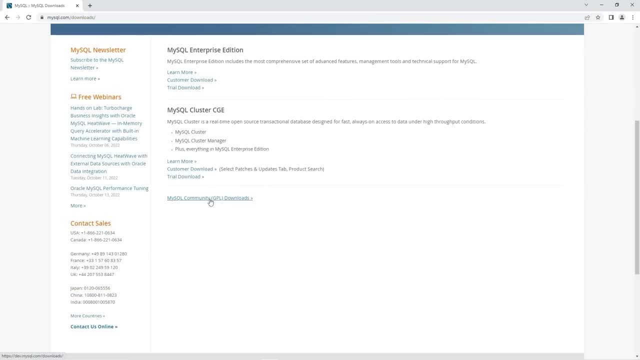 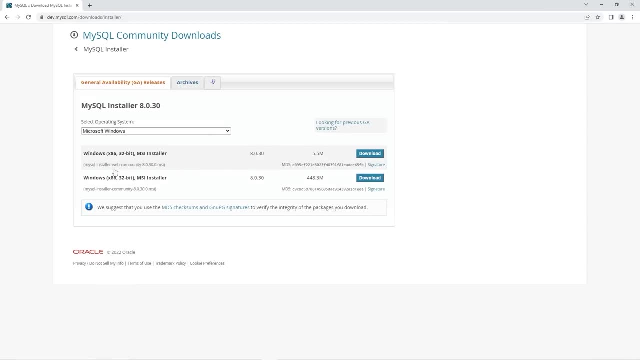 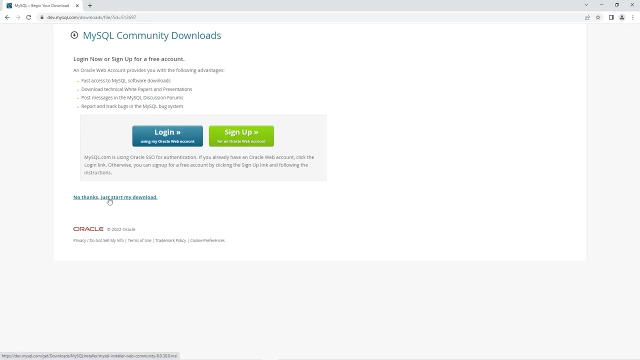 Scroll down, look for MySQL Community Downloads. We'll click on that. Click on MySQL Installer for Windows. Make sure that we have our Windows operating system selected. Then download the first installer. No thanks, just start my download. We will open this download once it's complete. 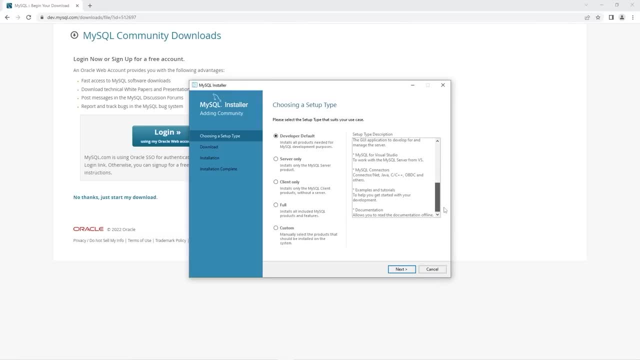 There are various setup types depending on what packages you need For this series. all we need is the server and the workbench. We'll select the Custom Radio button, Click Next. We will need the most recent MySQL server. Add that to Products to be Installed. 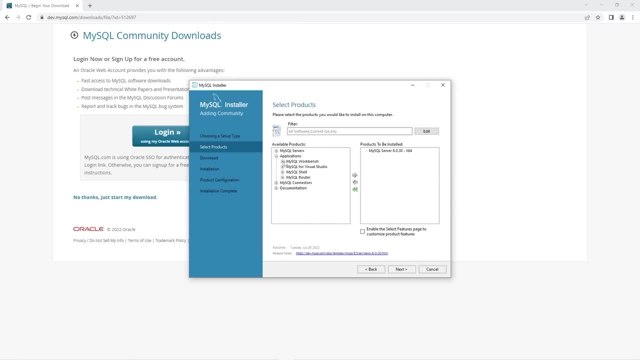 Open Applications. Go to MySQL Workbench. We will add the most recent workbench. We can close out of that. There is a shell if you're interested in using that, but I will be sticking with the workbench in this series. Once we have our server and our workbench, I will click Next, then Execute. 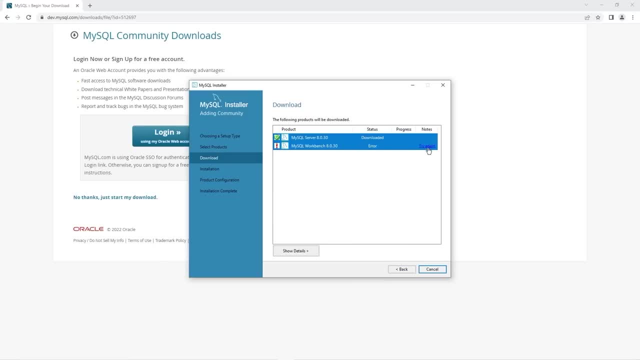 It looks like there is an error downloading the workbench. I'm going to try again And it worked this time for some reason. Let's click Next Execute. give it some time. Once the installation status for the server and the workbench is complete, we can click. 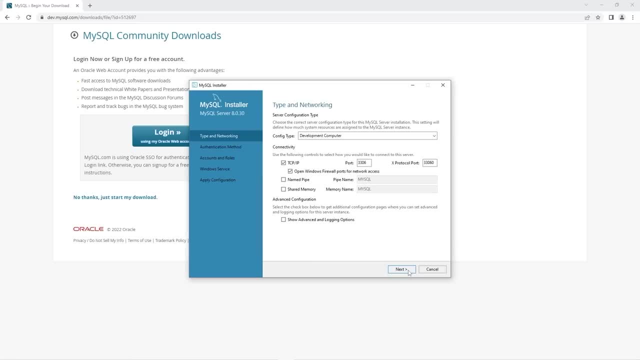 on Next. Next, I'll keep these default configurations. Next, Use strong password encryption for authentication. Let's click Next. Here we're going to set the root password to X. Let's click Next. Here we're going to set a password to access the server. 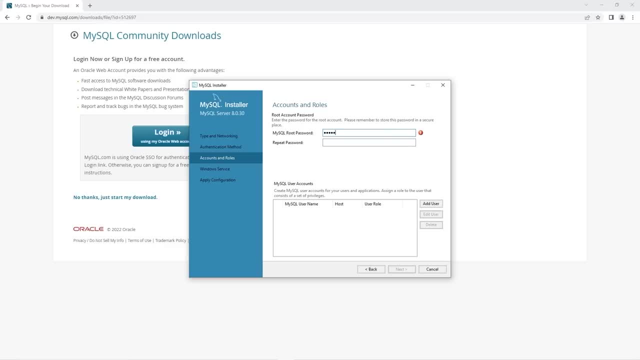 Think of some password you would like. I'm just going to set mine to be password. I'll keep it simple. Yeah, of course, the password strength is weak. You can add user accounts, but that will be outside the scope of this series. 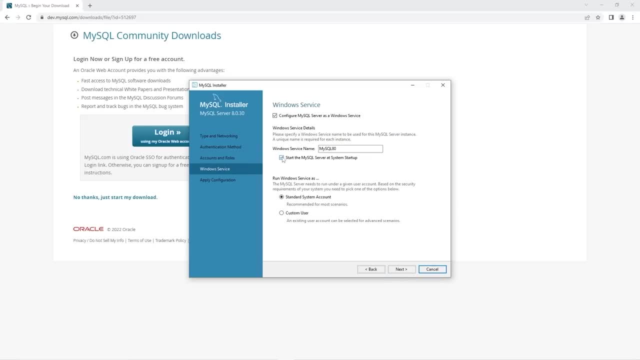 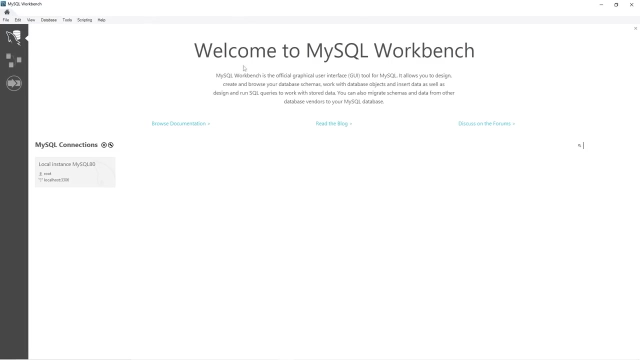 Click Next, You can start the MySQL server at System Startup. if you would like, I'll keep that on. Click Next, Then Execute, Then Finish, Then Next. Yeah, we might as well start the MySQL Workbench after setup. If this window doesn't pop up, you can easily just search for it. 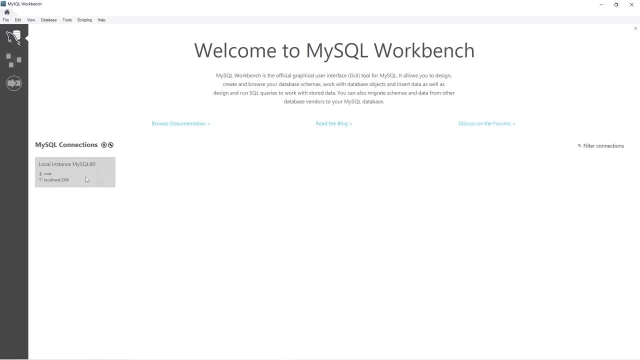 Just look for MySQL Workbench. Now we should have a local instance. We can click on this to access our server. Let's pretend that this wasn't here. I'm going to right click delete connection. If you need to set up a connection, hit this plus button. 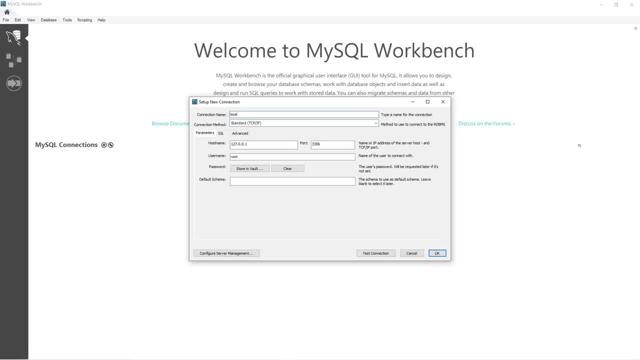 Click Next. We'll need a connection name. I'll name this local host. Connection method should be standard TCP IP. The host name is 127.0.0.1 at port 3306.. Then press OK. So now that we have our connection set up, we can click on it. 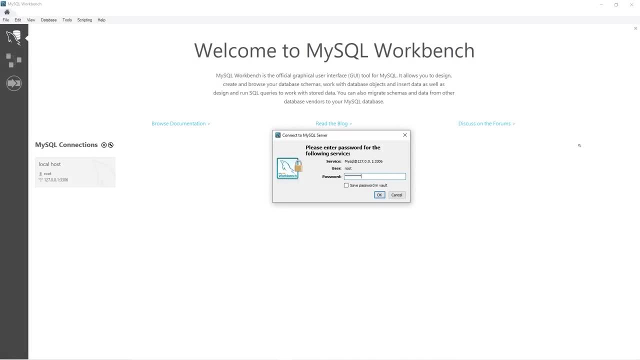 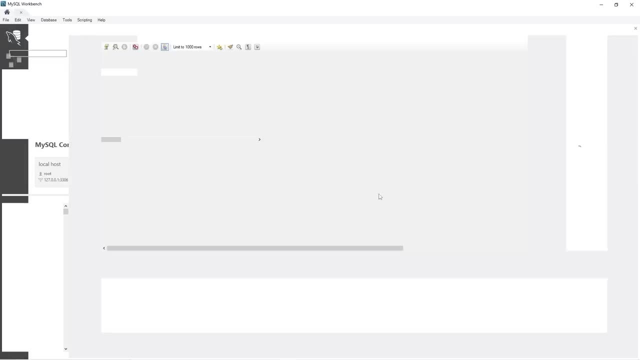 Type in the password you set for the server. Mine was simply password. You can save the password if you want. I'm going to save this one. I'm going to save this one. If you want, I might as well. Then OK. 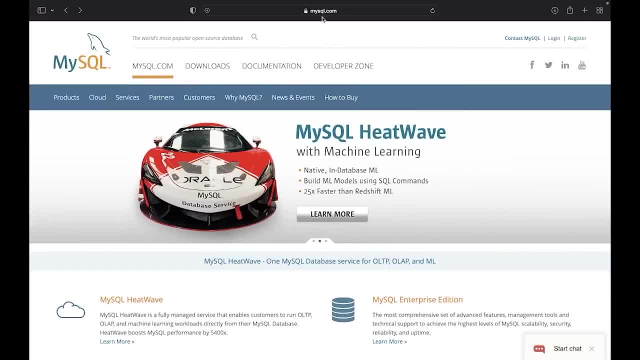 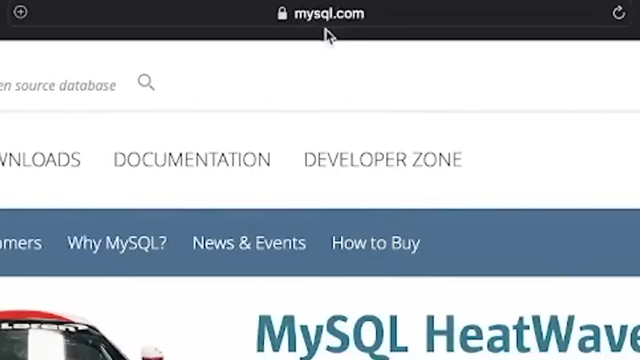 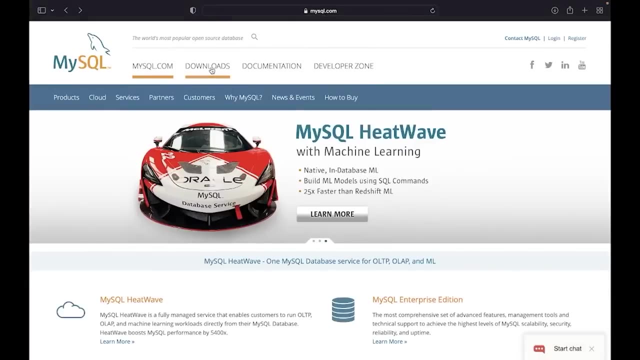 And here we are within the MySQL Workbench. All right, everybody. In this topic I'm going to explain how we can download MySQL using the Mac operating system. First, head to this URL: mysqlcom. We will go to the Downloads tab. 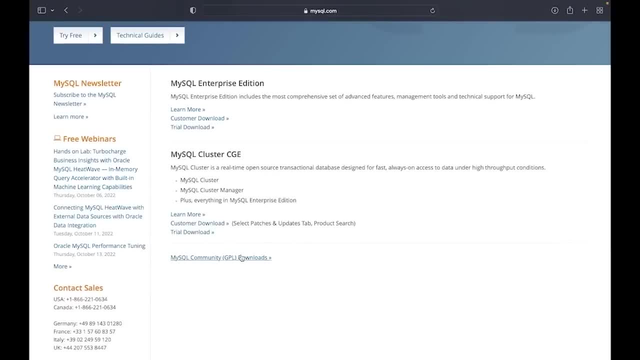 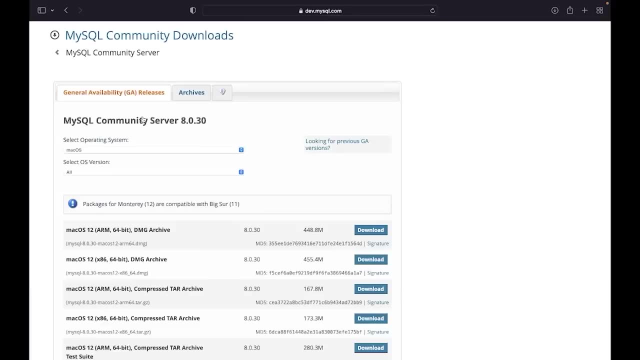 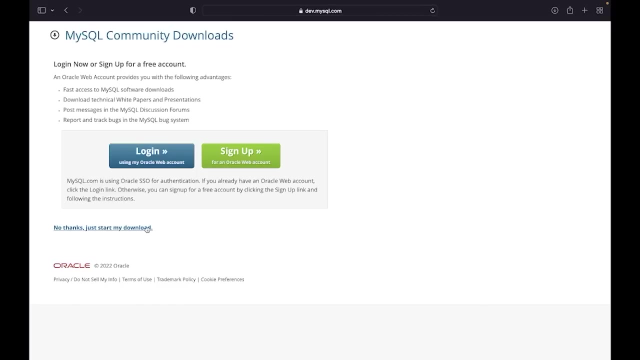 Scroll down. Look for MySQL Community Downloads. We'll need both the server and the workbench, but let's start with the server. Click on this file. Mac OS 12 DMG archive- Click the Download button. Click on this link. 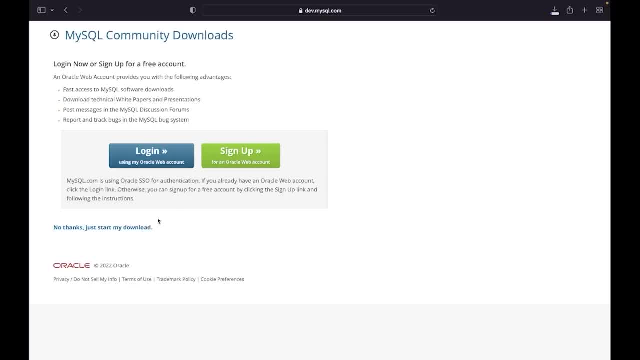 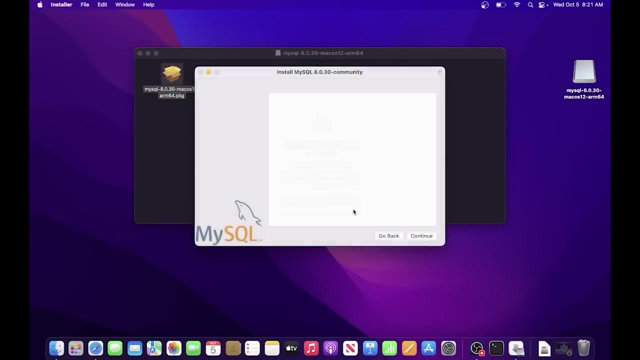 No thanks, Just start my download. When this DMG archive is finished downloading, we can double click on it. Just give it a second Double click on the DMG archive. Allow, Click Continue. You can read the license agreement. I'm going to pretend I did. 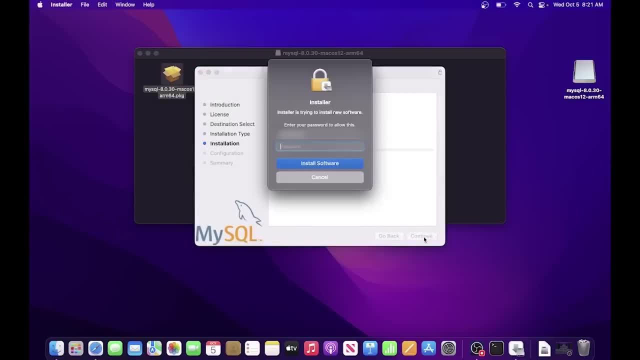 Hit Continue. Install Type in your computer's password. if this prompt comes up, Use strong password encryption. Hit Next. Then we'll need a password for our server. Type in whatever password you would like. To keep it simple for this lesson, I'm just going to set my password, to be well. password. 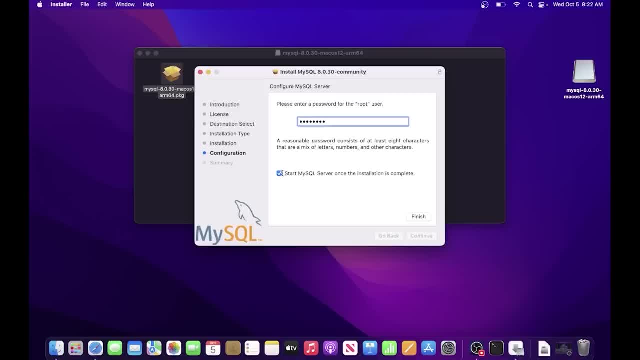 By checking this box, MySQL Server will start once the installation is complete. You might as well keep this checked, but for demonstration purposes, I'm going to show you how to start the server manually. Let's go, I'll go ahead and move the installer to the trash bin. 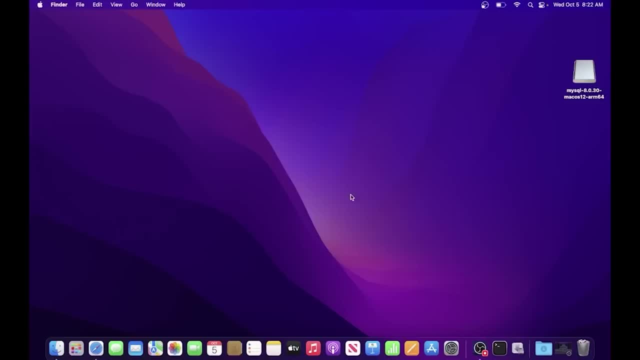 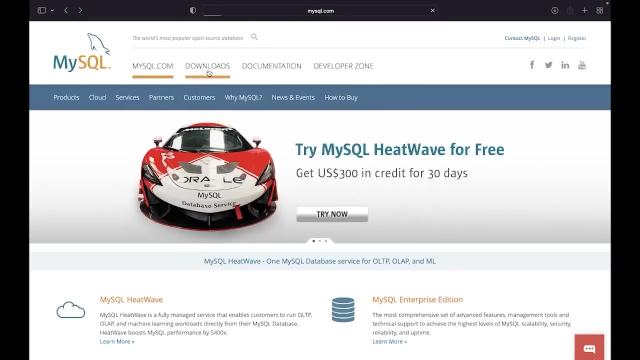 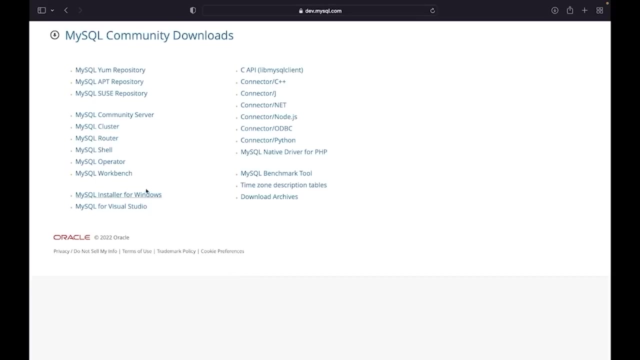 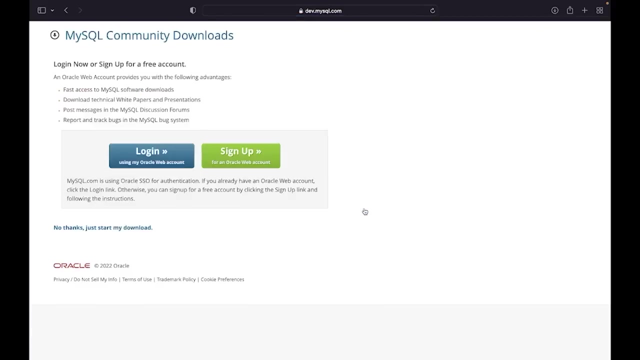 We have the server downloaded. Next we need to download the workbench Again. head to mysqlcom, Go to Downloads, Scroll down to MySQL Community Downloads, Click on MySQL Workbench, Then hit the blue download button. No thanks, just start my download. 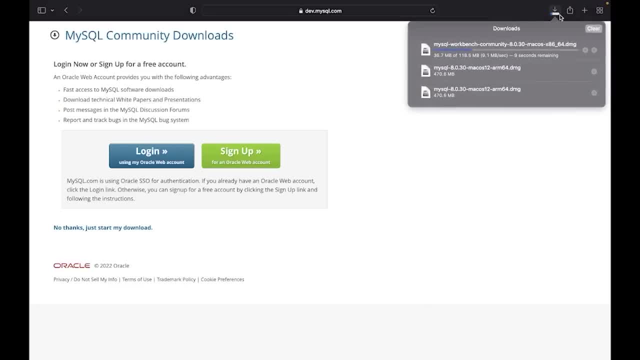 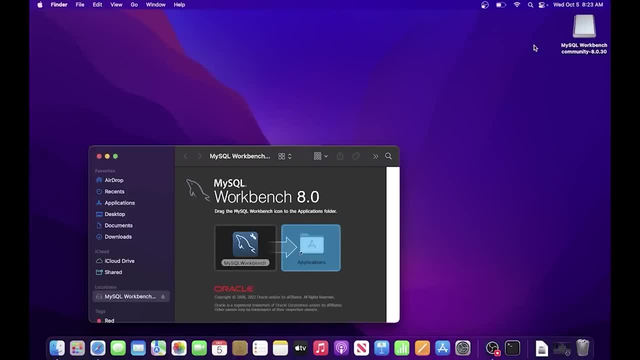 Then we can double-click on this DMG archive when it's finished downloading. Double-click, Drag and drop the workbench icon into your Applications folder. Updown to MySQL Multimedia. Scroll down to MySQL Workbench. Drag and drop the Workbench icon into your Applications folder. 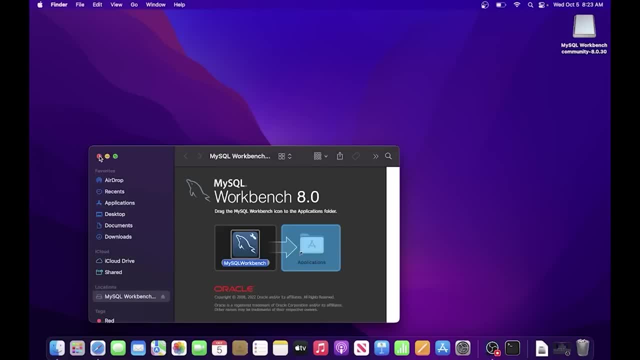 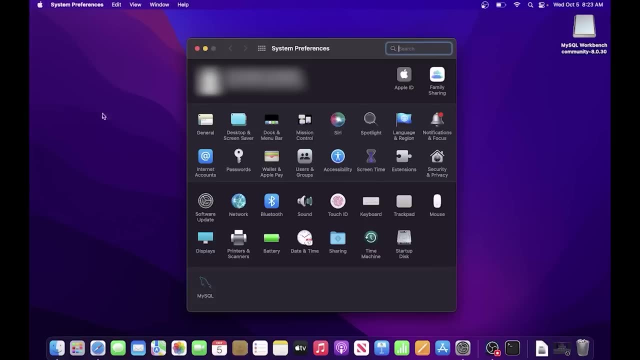 Before we access the SQL Board, we need to fill out the Unfolder, the workbench. let's be sure that the MySQL server is running. Click on the top left Apple logo. Go to System Preferences. At the bottom left corner, look for MySQL. 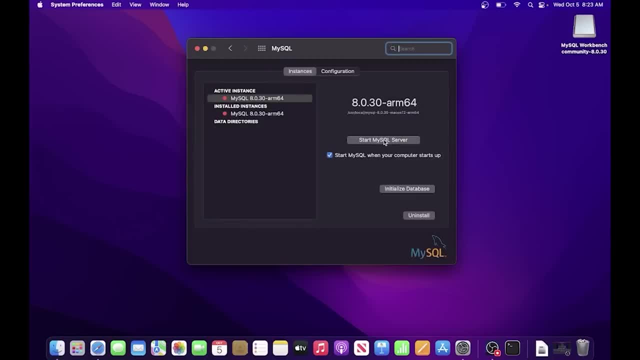 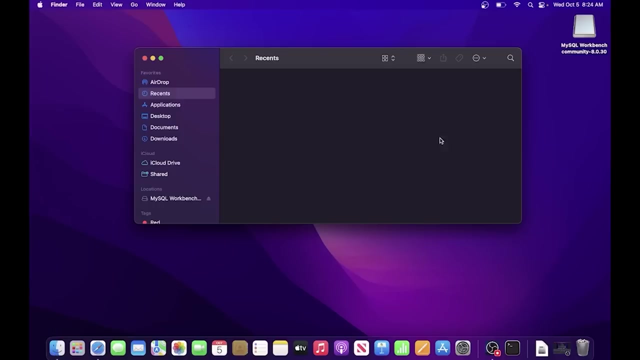 Click on it Then start MySQL server, if it's not started already And you can check this checkbox so that your computer starts up with it running. Alright, you may need to type in your password. The server is now running. To run the workbench, we can go to Finder, then Applications. Look for the MySQL. 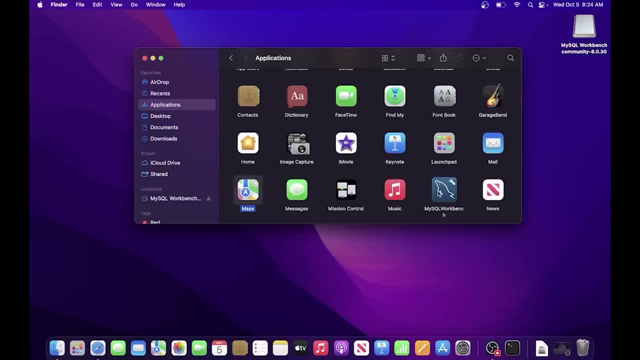 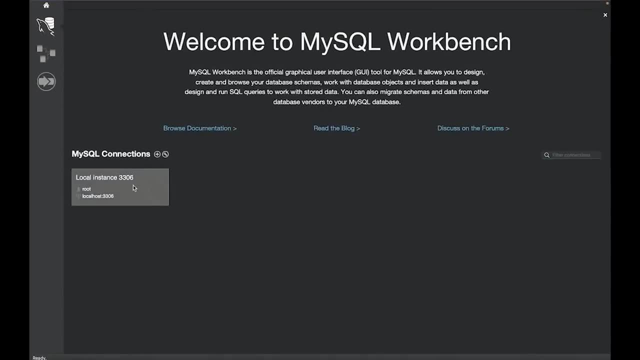 workbench icon, Double click on it And here we are within the MySQL workbench. To access the server, you can click on this local instance connection, Then type in the password that you originally set for the server. But if you're missing this connection, you can hit the plus button Then create. 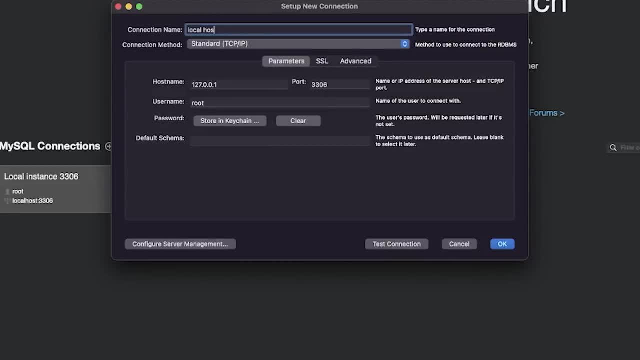 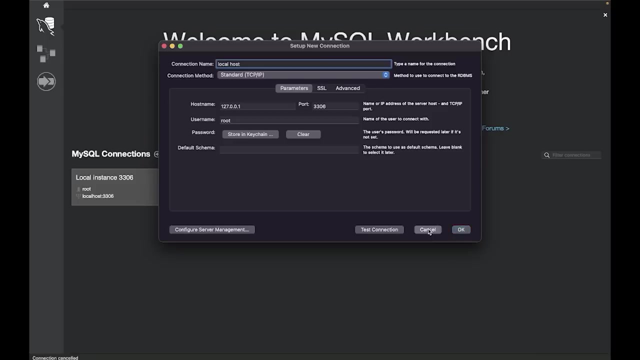 a new connection name. I'll name this localhost. Use standard TCP IP for the connection method. Host name should be 127.0.0.1 and port 3306.. Then press OK. But I already have my connection set up. Click on your connection Type in the. 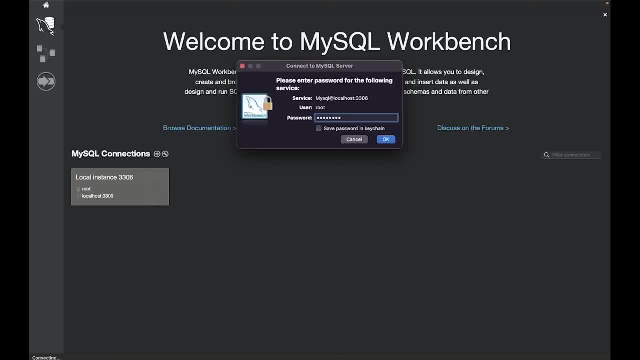 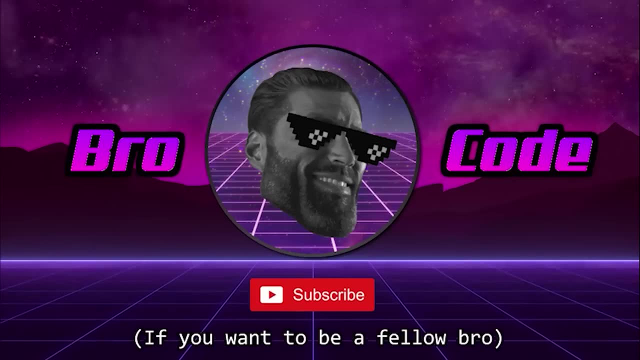 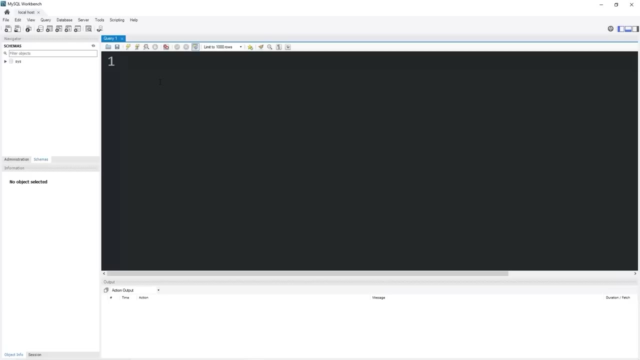 password you set for the server. Then press OK And here we are within MySQL workbench. Hey everybody, in this topic I'm going to show you how we can create, alter and drop a database. What is a database exactly? Think of it as a folder. It acts. 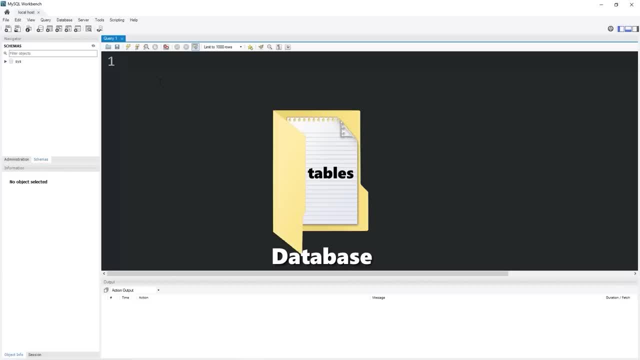 as a container. Tables, on the other hand, would be the files found within the folder. In this topic, I'm going to show you how we can create the database itself, but we won't be working with any tables until the next topic. We'll need 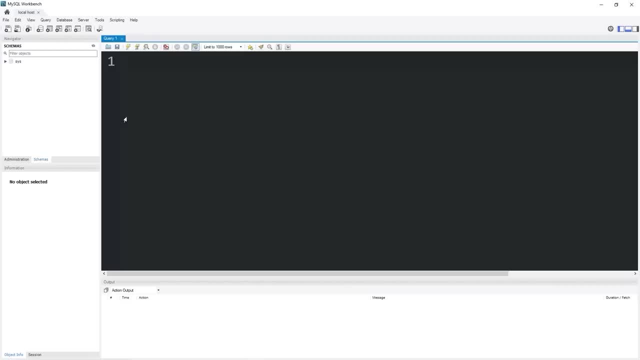 to begin by heading to our database. In our query window, which is this large window right here, we're going to write a statement To create a database. we will type create. There is no case sensitivity in MySQL. These keywords such as create- they can be all uppercase, Just the first. 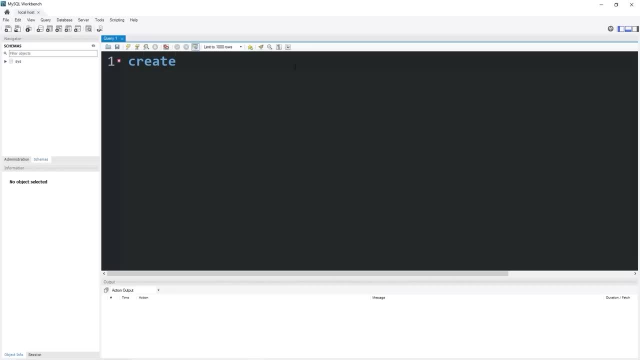 letter could be capital, Or you could do all lowercase With the keywords. I like to make them all uppercase, but that's just me. Create Database And then we'll need a unique database name. What about mydb? Then? it's important with all SQL statements to end each statement. 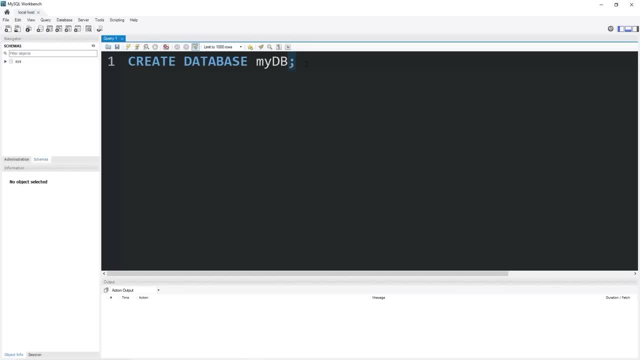 with a semicolon. It's like the period at the end of a sentence. That's how we know that the statement is complete, So you'll need these three words: Create Database, Then a database name. We just named our database mydb. Hit this lightning bolt button to execute. 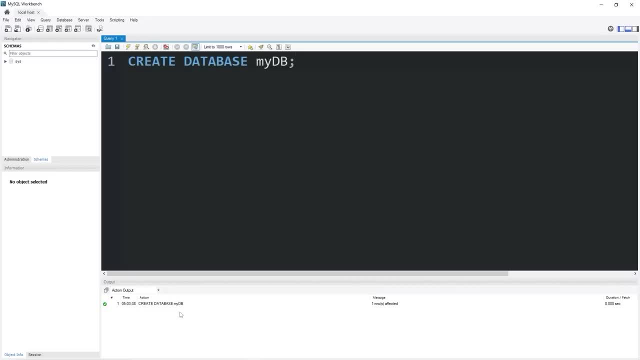 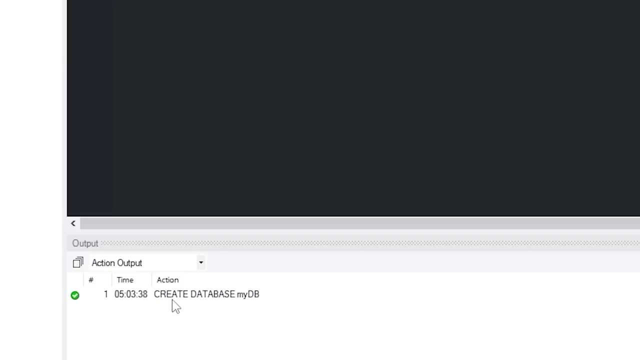 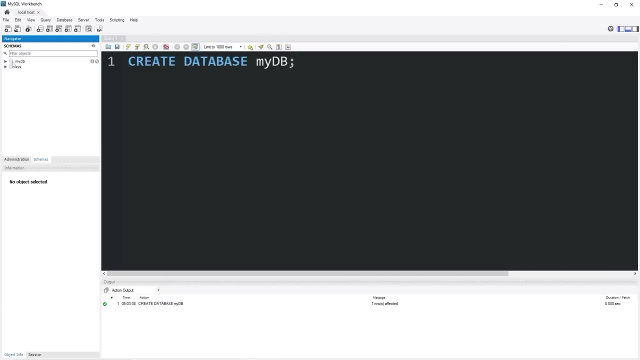 this statement And in my output window. Unfortunately I can't increase the font size, but I can zoom in. This action was successful. We have created database mydb. If you head to your schemas tab, then hit the refresh button. you should see a database in here named mydb. There's. 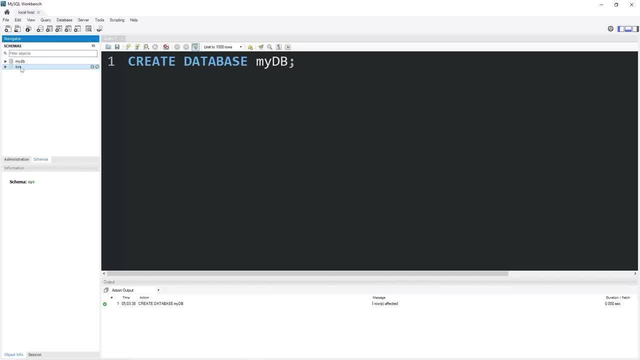 also a database for sys. Sys is the internal database that MySQL uses. We'll want to be sure that we're using the database that we just created. To use a database, we can either right click on the database, Then click on set as default schema. 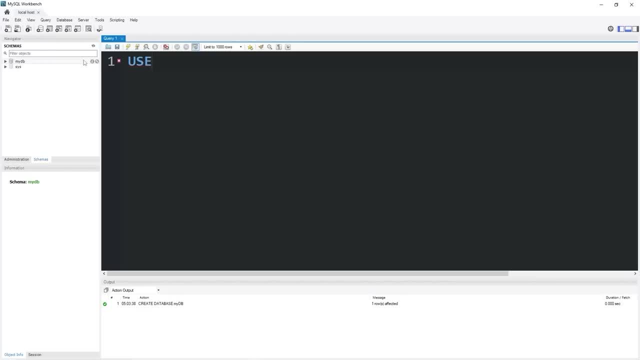 Or you could use a statement. Use Then the name of the database: Mydb semicolon. Execute this statement. We are now using my database To drop a database type: drop database, Then the name of the database And our database is gone. Unfortunately, we do need a database. 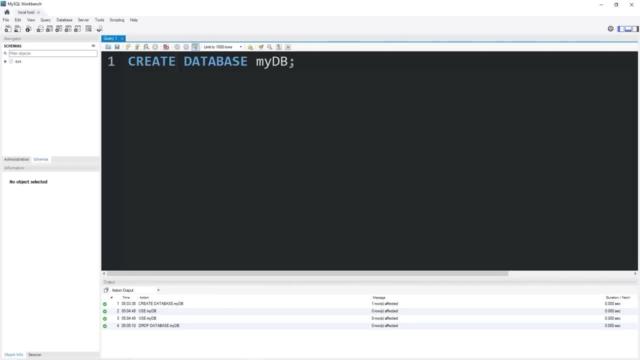 for this series. so let's go ahead and recreate our database. Create database, Then we'll type database: mydb. Refresh, Then, just to be sure we're using this database, we can either use that keyword use Or you can right click on the database and set as default schema. 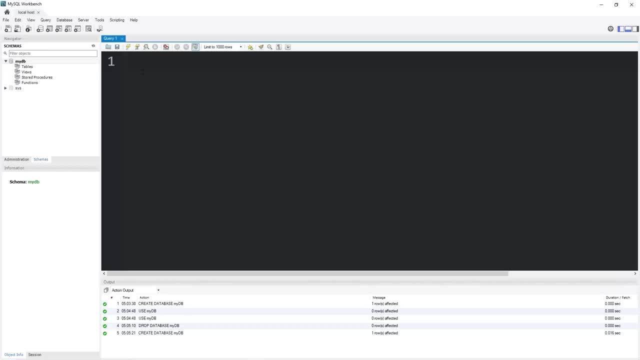 Alright, so we can create, use and drop a database. How about alter? There's two features for beginners. I'll mention Setting a database to read only. The other is enabling encryption. Let's set our database to be read only. Type alter. 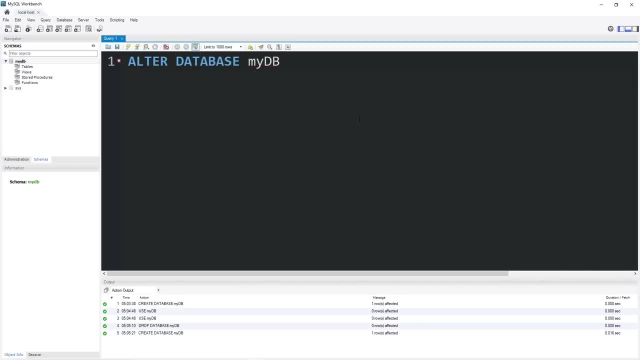 Database. The name of the database Read only equals one. This statement would make our database read only. If a database is in read only mode, we can't make any modifications to it, but we can still access the data within. Let's attempt to drop our database. Drop database. 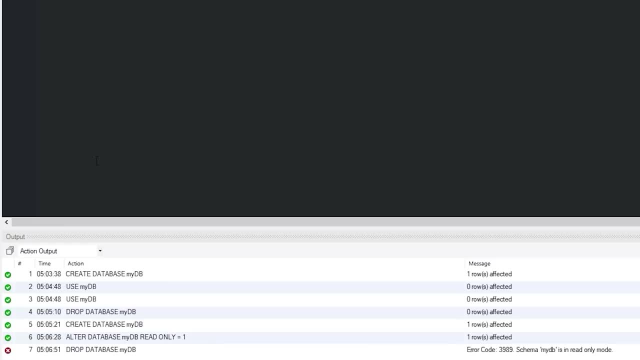 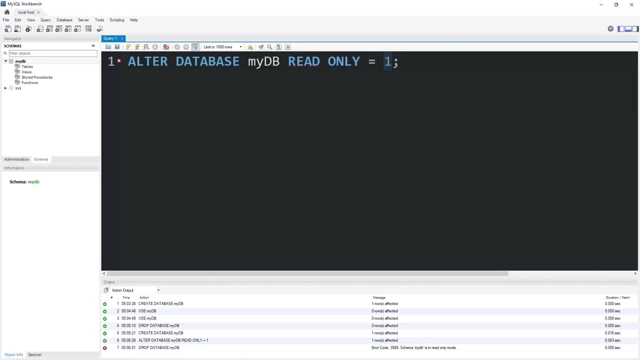 mydb, Then we have a red xray. That means we could not complete this action. Drop database- mydb Schema. mydb is in read only mode. To disable read only mode, you would set read only equal to zero. Now we 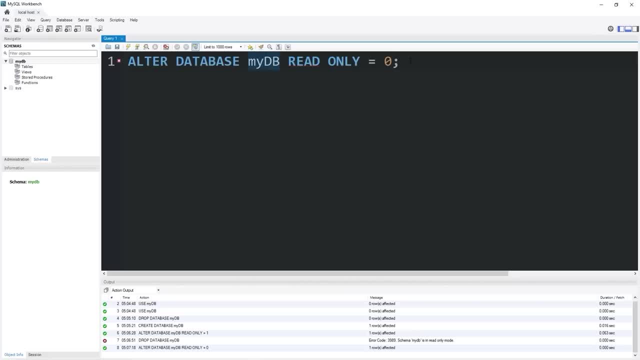 would be able to drop this database. Alright, everybody. that is how to create, use, drop and alter a database. Think of a database as just a folder. A folder can hold files. The files will be the tables that we'll create. 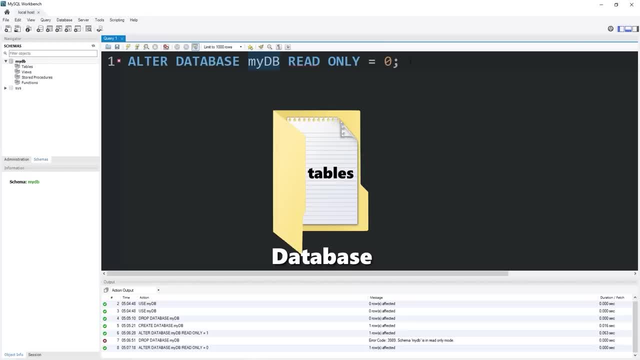 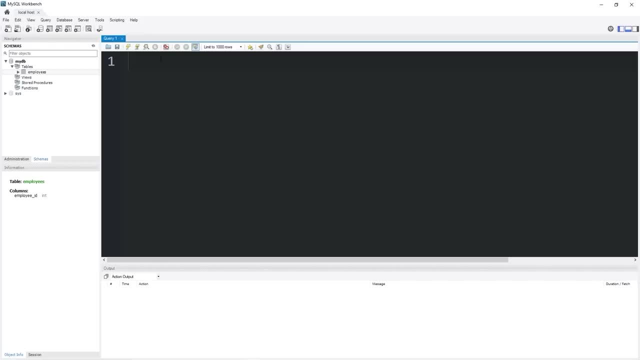 We'll store them within the database. This is exactly the case for the database, And in the next topic I'll show you how we can create some tables. Hey, welcome back everybody. In this video I'm going to show you how we can make some. 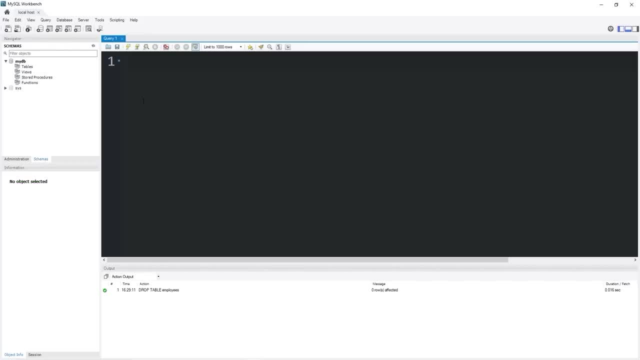 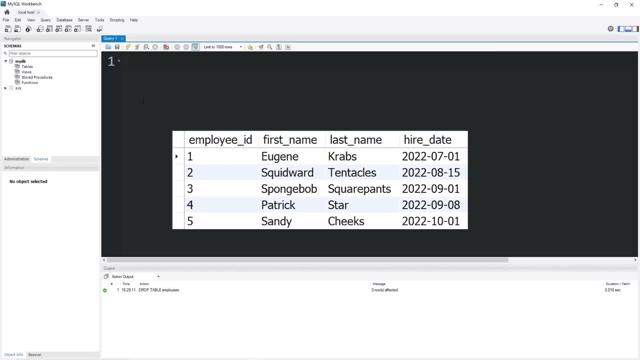 tables in MySQL, A table in a relational database. They consist of rows and columns, kind of like an Excel spreadsheet. In this topic we're going to create the table and the columns, But we'll be populating the rows in the next video. Create a table. You'll type Create, Create Wallet table, then the name of the table. I'll create a table named employees. Then add a set of parentheses- semicolon- at the end. Within the set of parentheses, we will list the columns. 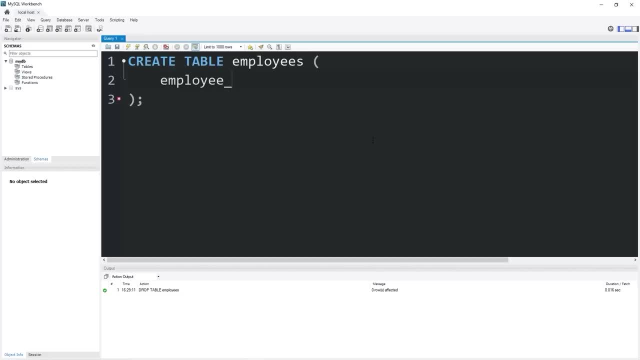 For employees, let's have an employee ID comma. Each column is separated with a comma, Then a first name, Last name. How about hourly pay? That'd be good. Hired date: Which date were they hired? There's one thing that's missing After each column. 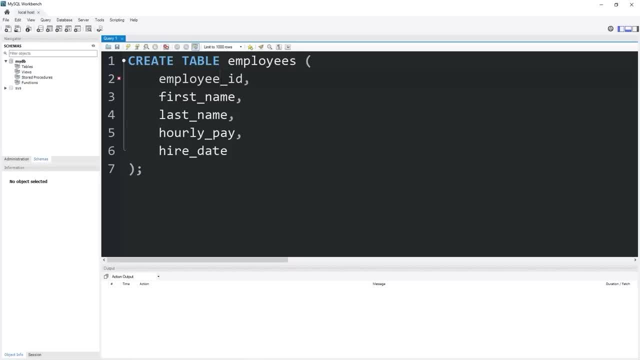 we need to set the data type of what we're storing within each column exactly. Is the data going to be whole integers, decimals, text, a timestamp- Those are data types. An employee ID comma- that could be a whole integer. The data type will be int- add int after the column name. 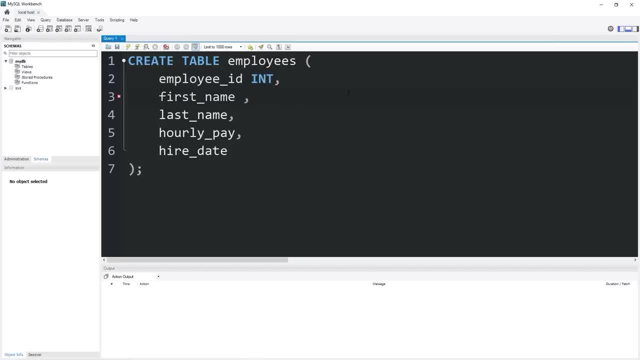 A first name that's a series of characters. The data type for some text would be var. char. then, within parentheses, the maximum amount of characters. I think 50 characters is enough for a first name. Last name, var char. 50 is good. Hourly pay: Maybe our hourly pay. 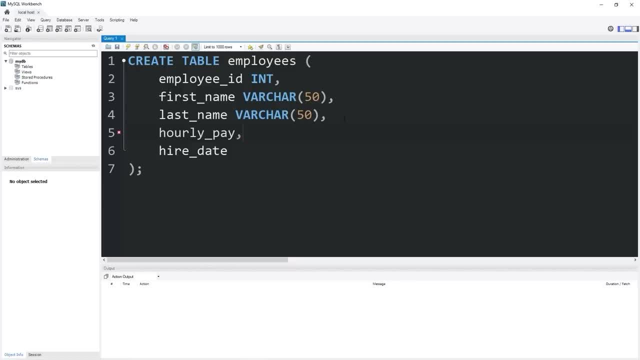 is in dollars and cents. We'll need a decimal portion. There is a data type That is decimal. Add a set of parentheses. We'll add the maximum amount of digits for our decimal. I think five should be good. Then a precision: Two for two decimal places. The reason that I set. 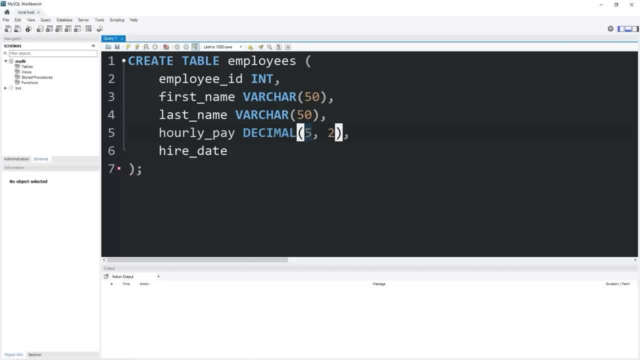 the maximum digits of my hourly pay to be five is that I don't anticipate anybody's hourly pay being over $999.99.. There is a data type which is date, if you need to work with dates. Otherwise, there's date time. if you need to include the time, Just the date, is fine, Let's execute this. 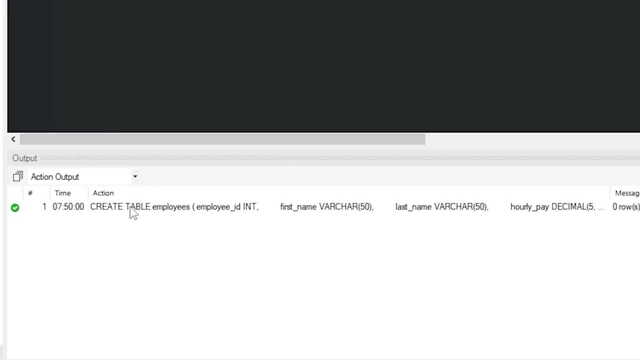 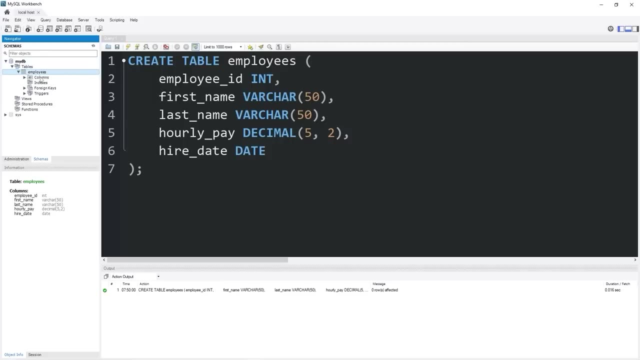 script. We have created our table Employees. If I were to refresh my schemas window, underneath tables we have our Employees table. Now I'll show you how we can select a table. If you. If you need to select your table, you can type SELECT asterisk FROM the name of the table. 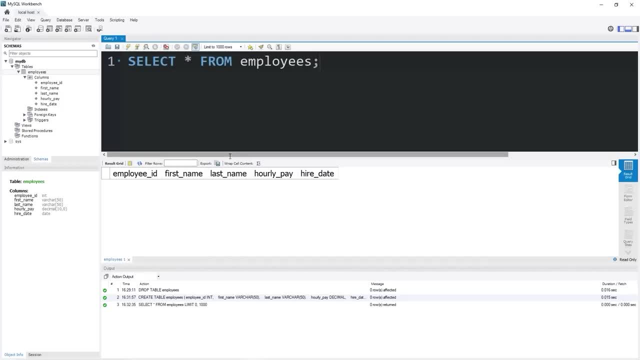 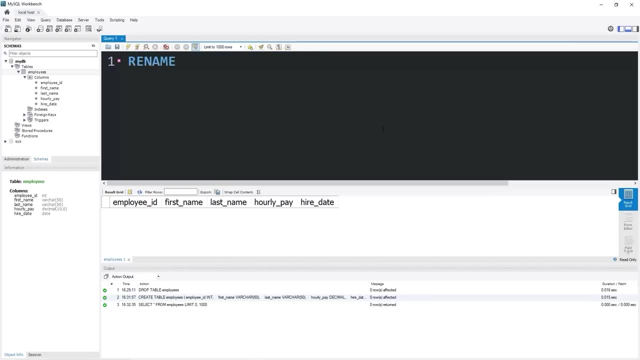 Employees. Let's take a look. Here's our table. so far There's no rows but there are columns. We have employee ID, first name, last name, hourly pay and hire date. If you need to rename a table, you can type RENAME TABLE. the original name, EMPLOYEES TO whatever the new name is, perhaps WORKERS. 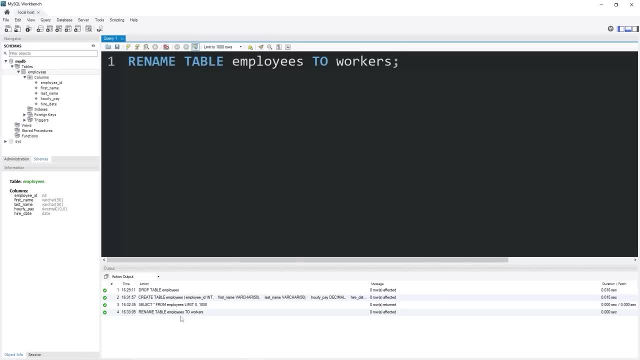 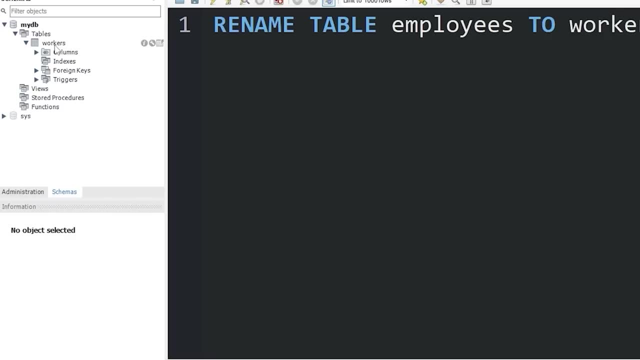 Let's try that. RENAME TABLE EMPLOYEES TO WORKERS was successful. If I refresh my schemas window, the table EMPLOYEES is now known as WORKERS, But I think that's stupid. Let's go back and change it. 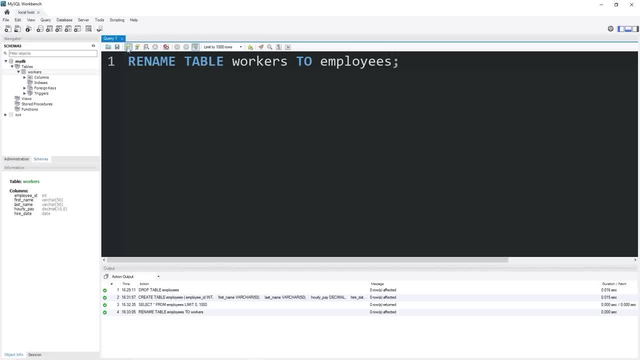 RENAME TABLE WORKERS TO EMPLOYEES To drop a table. I discussed this earlier. you would type DROP TABLE, the name of the table. I don't want to drop this, so I'm not going to execute this statement, but that's how you would drop a table. 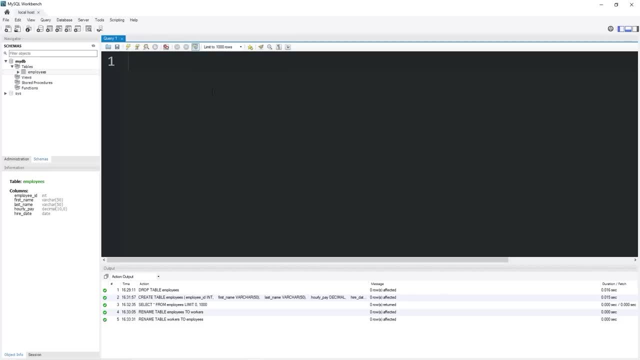 DROP TABLE- the name of the table. If you need to alter a table, there is the ALTER keyword. Let's add a phone number: ALTER TABLE EMPLOYEES. I'm going to write this next part of the statement on a new line. 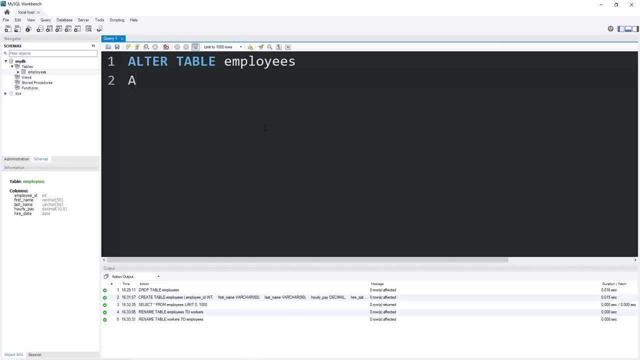 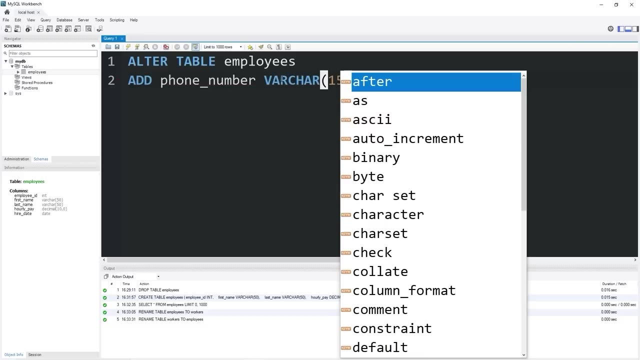 What do we want to add? What about a phone number? ADD PHONE NUMBER. Then we'll need to list the data type of this column. VARCHAR is good. Max size of 15 characters. Then we will end this statement. Execute the script. 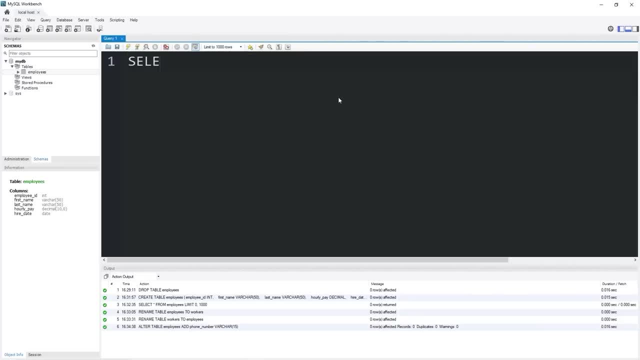 Alright, we have altered our table. Let's take a look at our table. Select asterisk. Asterisk means all. I don't know if I explained that. Select all from employees. We have employee ID: first name, last name, hourly pay, hire date. 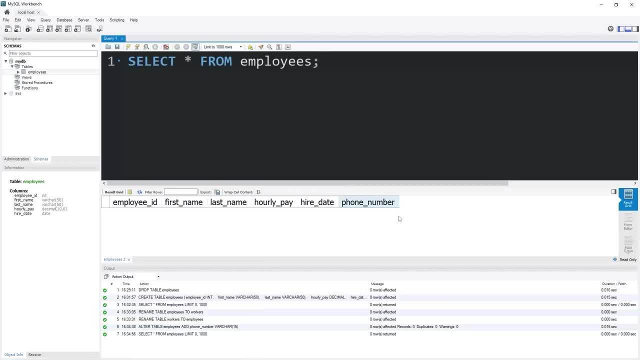 Then our column phone number. Let's rename phone number and change it to something else. We will again use the ALTER keyword: ALTER TABLE- EMPLOYEES. RENAME COLUMN PHONE NUMBER TO, let's say, EMAIL. 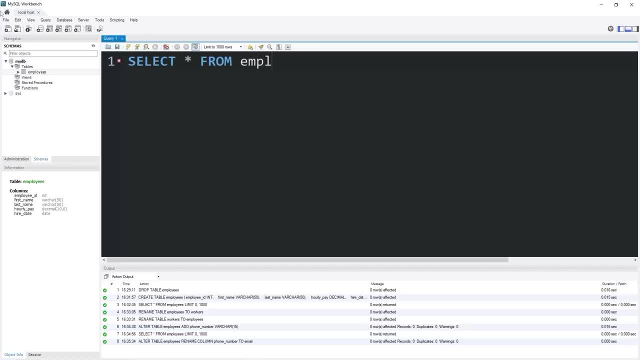 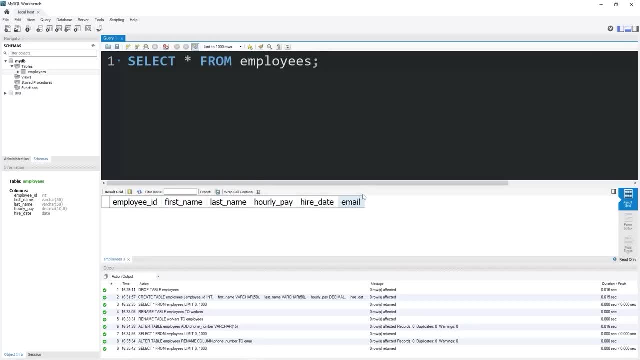 Okay, then let's take a look again. Select all from employees: Yeah, employee ID. first name, last name, hourly pay, hire date, then email. However, the data type has not changed for email. I'm going to refresh my schemas. then, underneath information, underneath employees: 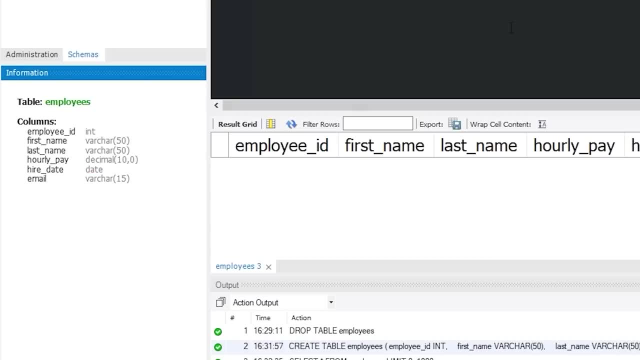 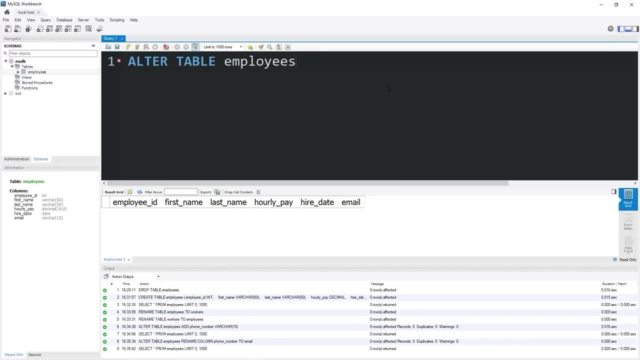 Our email column has a max size of 15 characters. Let's change that. ALTER TABLE EMPLOYEES MODIFY COLUMN EMAIL, Then the new data type: VARCHAR MAYBE 100 CHARACTERS FOR AN EMAIL. 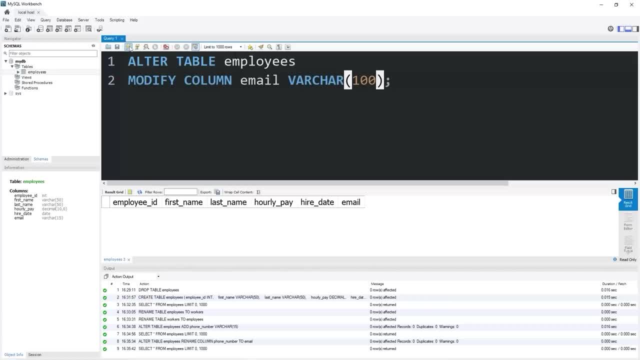 Let's execute this statement. Refresh our schemas. Yeah, now our email column has a size of 100 characters. Maybe we need to change the position of our email column. If you need to move columns around, this is how you can do so. 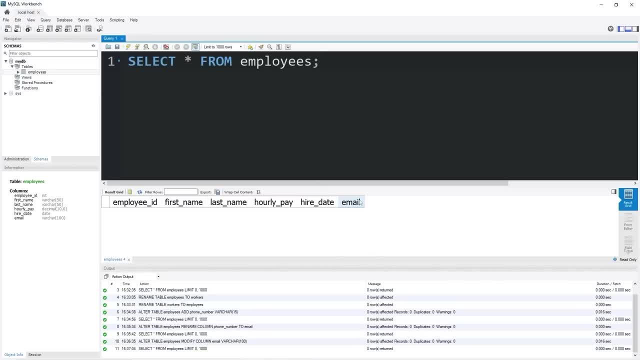 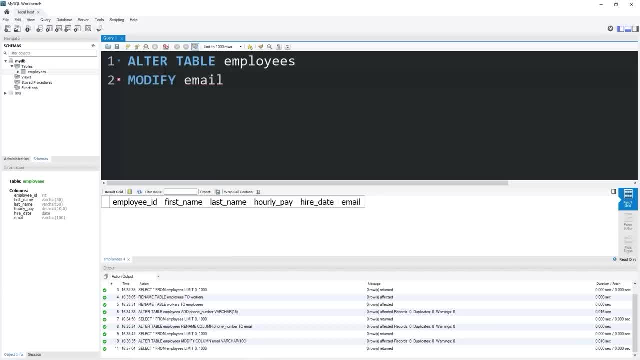 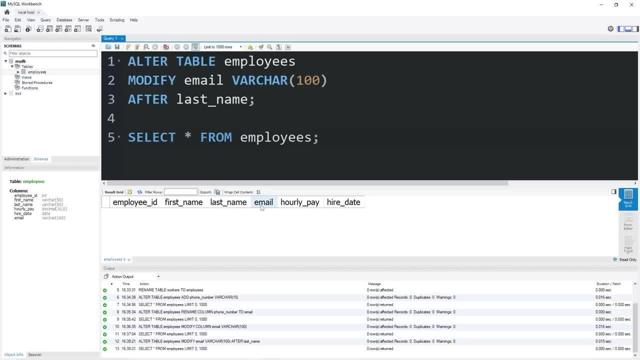 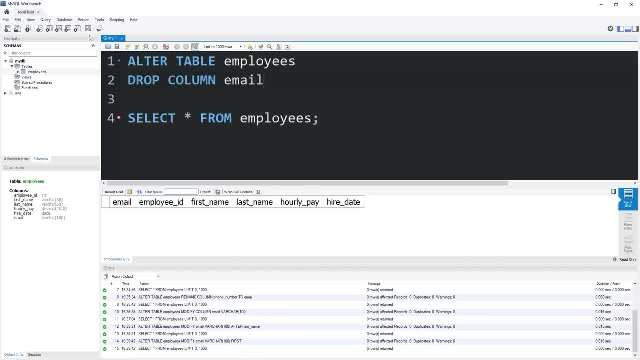 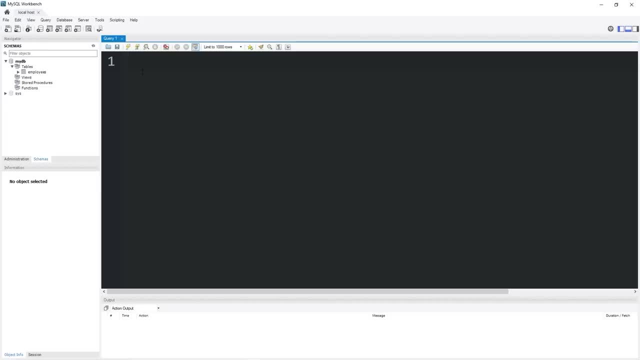 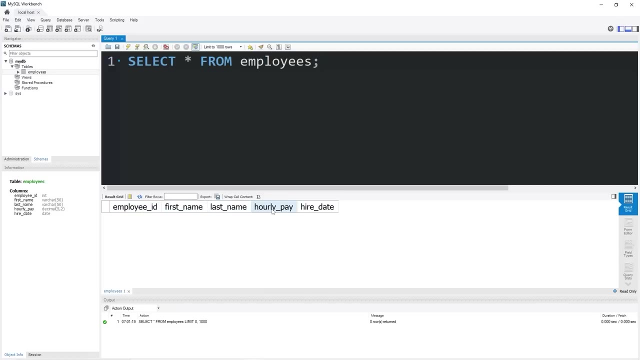 Hey everybody, in this topic I'm going to show you how we can insert rows into a table. We have a table named employees. I will select everything from my table employees. Here are the columns. We have an employee ID: first name, last name, hourly pay. 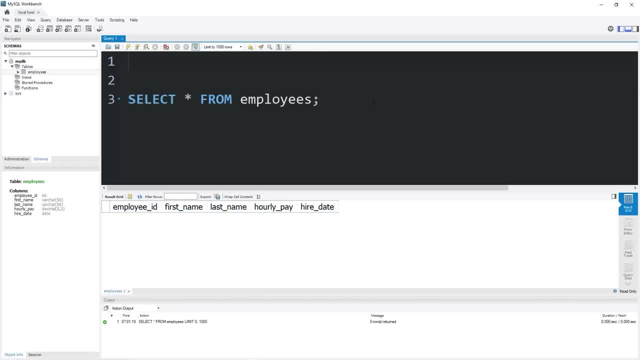 and hire date. To insert a row into a table, we would type: insert into the name of the table, followed by values, parentheses, semicolon. Between this set of parentheses, we will add all of the data for a row. We will follow this order, beginning with employees. 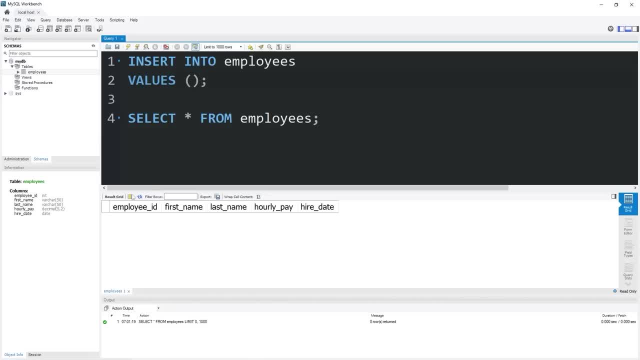 ID- first name, last name, so on and so forth. But we do have to pay attention to the data types too. Each piece of data will be separated with a comma. Let's begin with an employee ID. The first employee will be Mr Krabs. He's the first employee. I'll give him an employee ID of one. 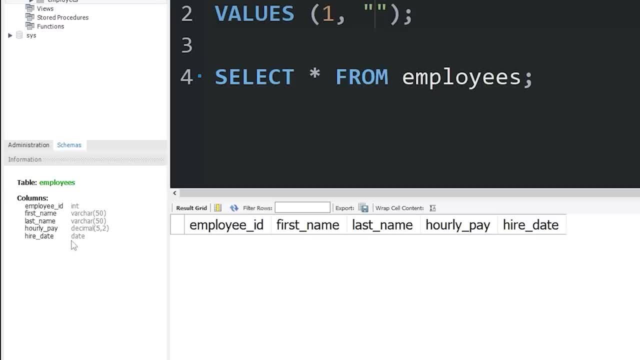 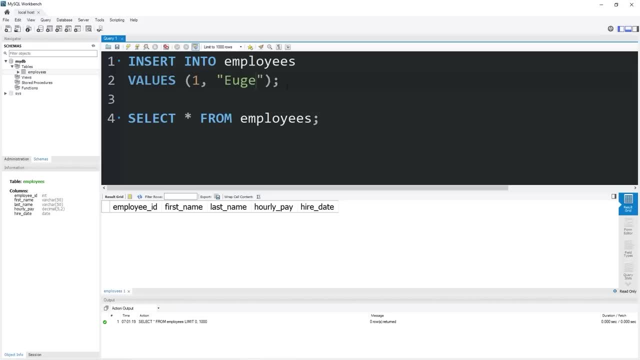 Then we'll need a first name. I'll put that within quotes because the data type of our first name is Varchar. Basically speaking, that's text: Mr Krabs first name. First name is Eugene, according to SpongeBob lore. Then we have a last name. 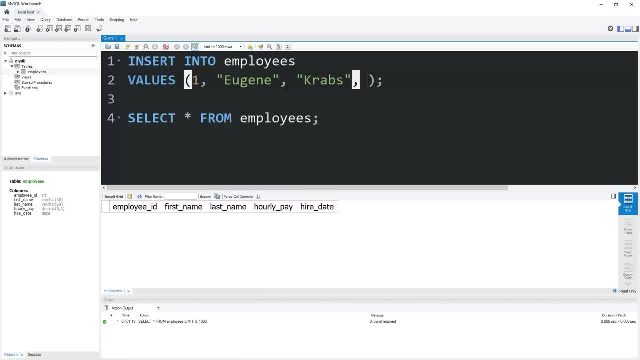 Last name, Krabs Hourly pay. This is a decimal. Mr Krabs hourly pay will be $25.50.. I'm just making up numbers here. Hire date. Here's the format for a date Within a set of quotes. 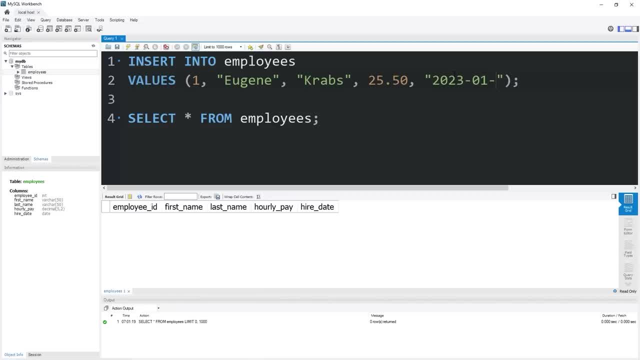 we will list the year, followed by the month, then the day. I'll set Mr Krabs hire date to be January 2nd 2023.. Now we can execute these statements. Yeah, here we go. Here's the first row Employee ID one. First name: Eugene. Last name: Krabs. Hourly: 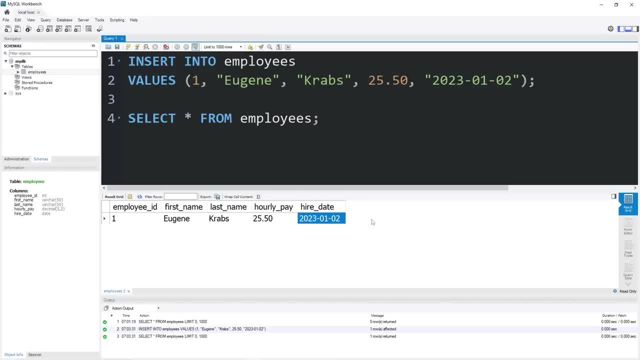 pay $25.50.. Hire date: January 2nd 2023.. It can be somewhat tedious to manually insert each row one statement at a time. Let's insert multiple rows at once. To do that after my set of parentheses. 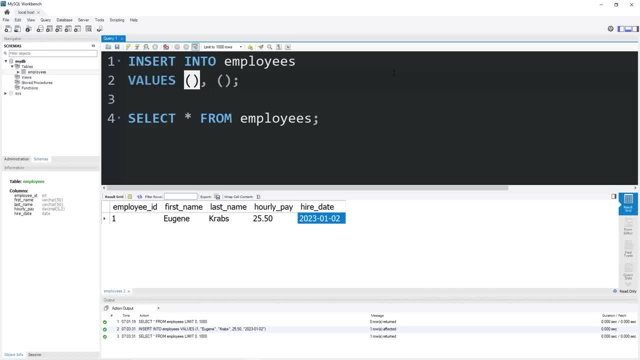 I will add another set of parentheses, each separated with a comma, depending on how many rows I would like to enter. So I have four employees I would like to enter. I will add four sets of parentheses, each separated with a comma, And let me just do some formatting to make this look pretty. 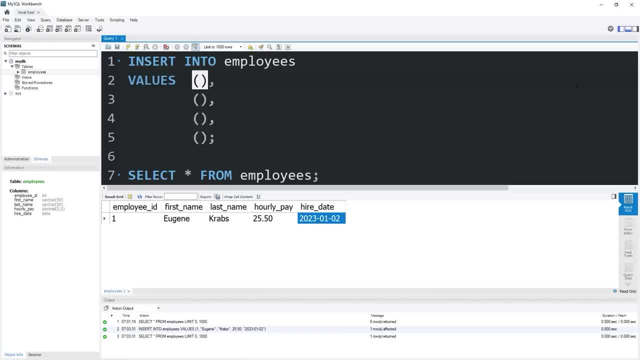 Each set of parentheses corresponds to a new row, So let's enter all the data that we'll need for this table. Employee ID number two will be Squidward tentacles. Squidward's hourly pay will be maybe a solid $15.. Squidward's hire date. 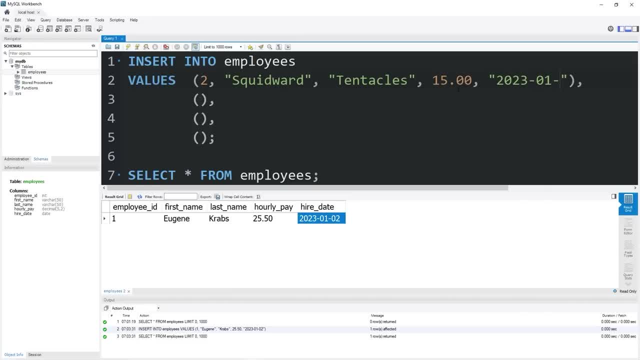 the year 2023, January. I think January 3rd is good. All right, so that is the next row. Let's work on employee number three. Employee number three will be Spongebob. Last name will be squarepants. Spongebob's hourly pay will be $12.50.. Spongebob's hire date is the year 2023, January 4th. 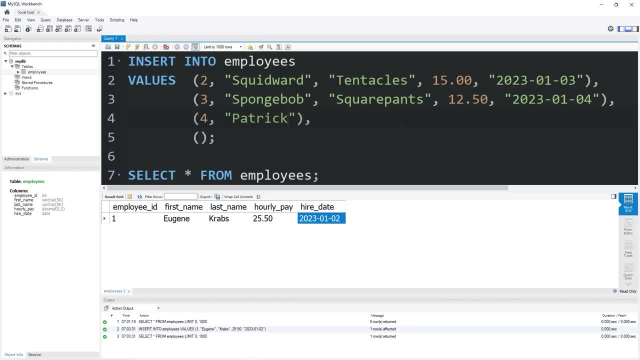 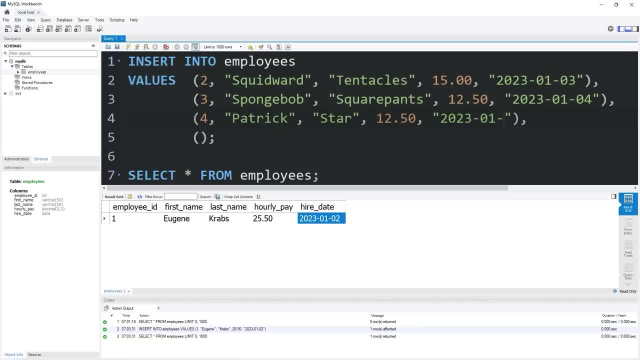 Hire date: 2023, January 5th. Okay, last employee, Employee ID number five: First name: Sandy. Last name: Cheeks. Sandy's hourly pay will be $17.25.. She'll be an assistant manager. 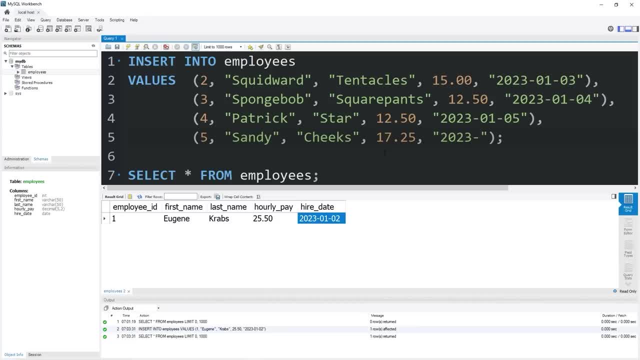 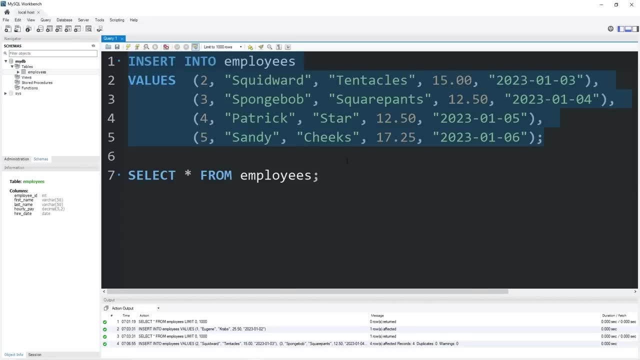 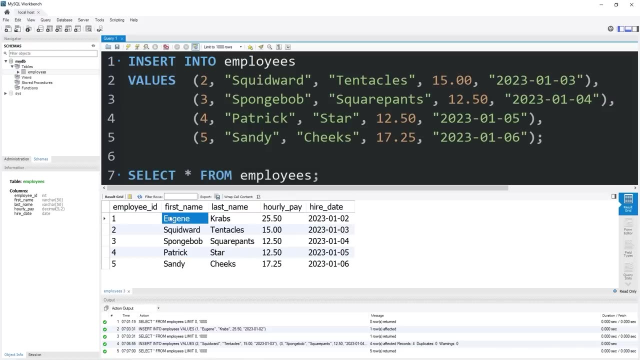 Sandy's start date will be the year 2023, January 6th. We can execute this statement to insert multiple rows all at once. Yep, here's our table. We have five rows, each corresponding to a different employee. We have Mr Krabs, Squidward, SpongeBob, Patrick and Sandy. 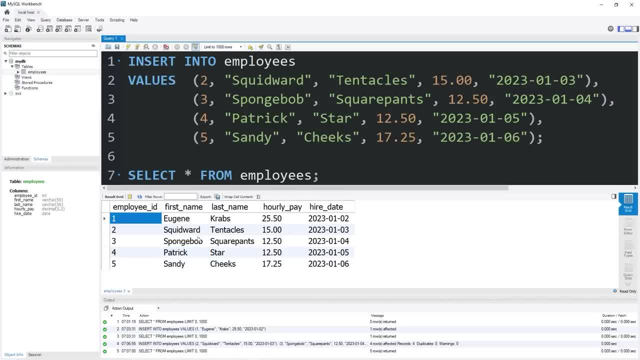 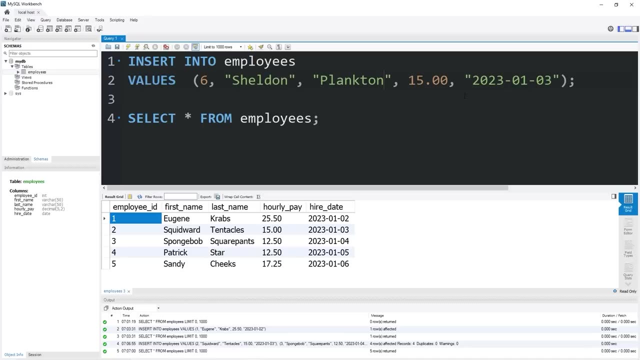 I'm going to demonstrate what happens when we attempt to insert a row with missing data. I will insert employee number six, Their first name. Their first name is Sheldon, Last name: Plankton. But we will not insert an hourly rate of pay or a hire date. 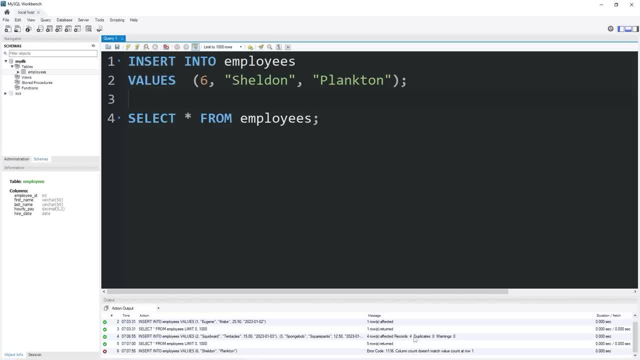 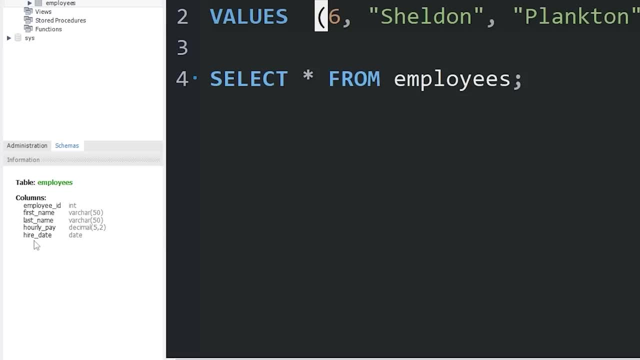 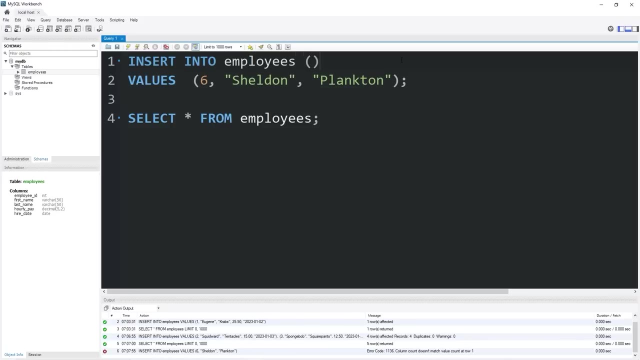 Here's what will happen. So we have an error. Column count doesn't match the value at count. at row one, We're missing data for our hourly pay and hire date. You could insert just select columns. That is done by adding: after the name of the table, add a set of parentheses. 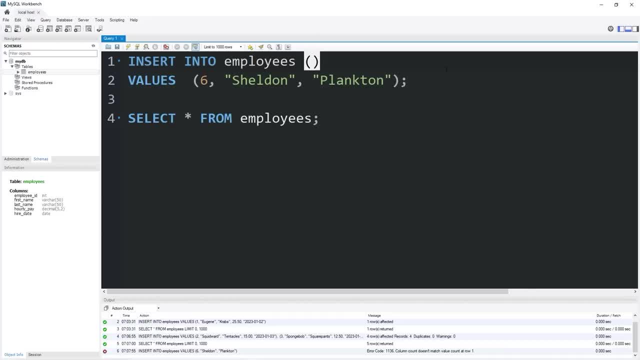 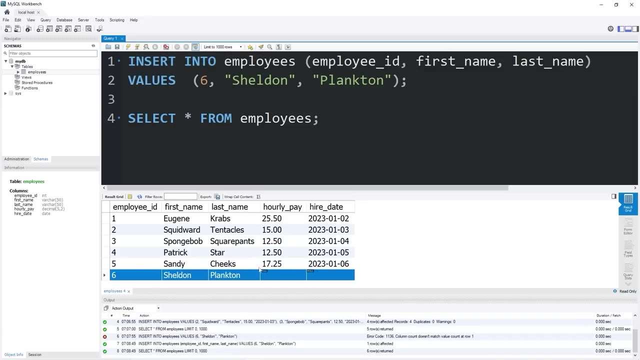 then name the columns you would like to insert. All we're adding is an employee ID: first name, then last name. Okay, now we've inserted a new employee, but there is data missing. and that's okay. We plan on hiring Mr Plankton, but we have not yet negotiated an hourly pay or start date. 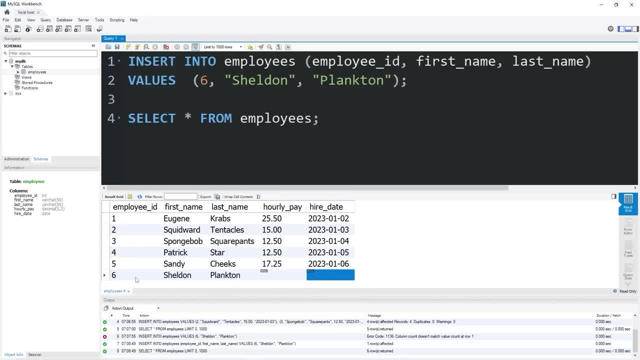 We still need to run a background check on him, but we want to add him to the system at least. So if you ever need to insert data, you can do that by clicking on the button on the right side of the screen. So if you ever need to insert data into a row but you need to omit certain columns, 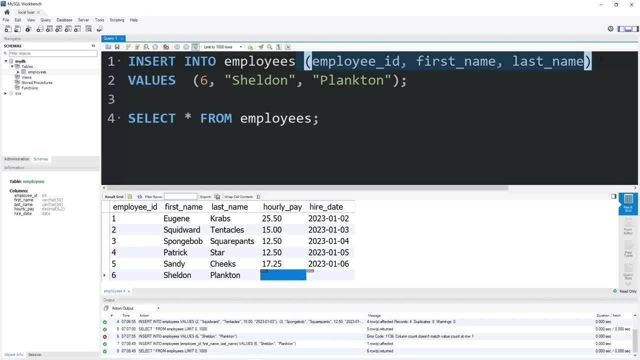 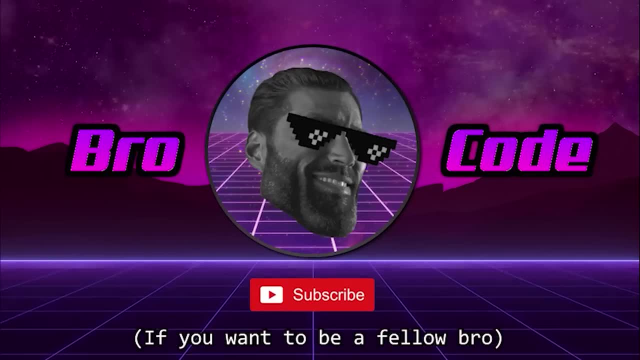 you can simply just list the name of the columns you would like to insert data into. All right, everybody. that is how to insert rows into a table in MySQL. Hey everybody, In this video I'm going to show you how we can select data from a table. 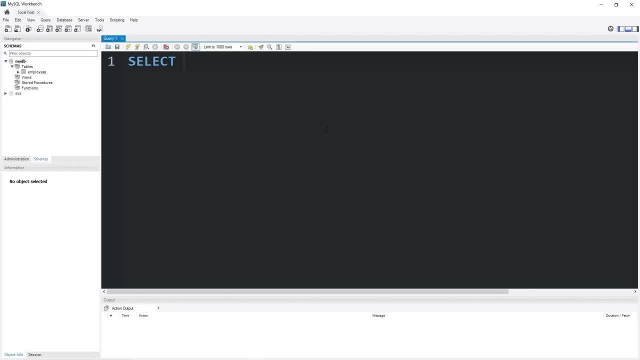 To query all of the data from a table, we would type select asterisk, meaning all from the name of the table. In my case, we have table. This statement- select all from employees- will give me all columns and all rows. 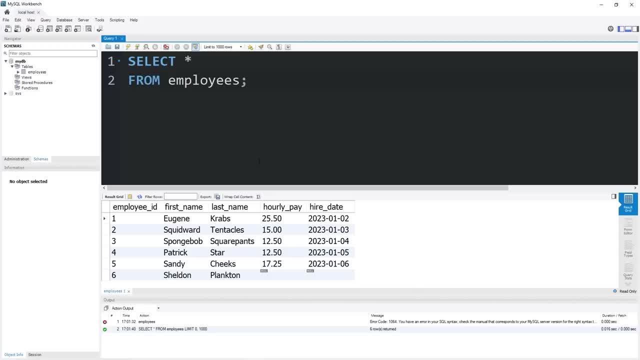 But sometimes you may not want all of the data. Here's a scenario: Your boss gives you a task of retrieving the full name of every employee. Well, we don't need employee ID, hourly pay or hire date for that right. 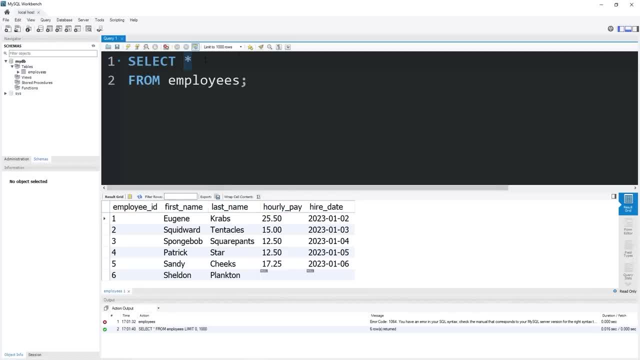 We just need a list of the first and last names of our employees table. In place of the asterisk, meaning all, we can select specific columns, such as first name and last name. We have all of the first and last names from our employees table. 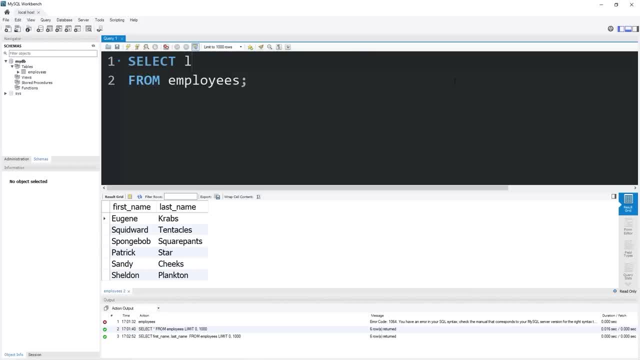 You can change up the order of the columns too. This time I would like last name, then first name. With our query, this returned all of the last and first names of all the employees, Point being, you can select specific columns depending on what you're looking for or 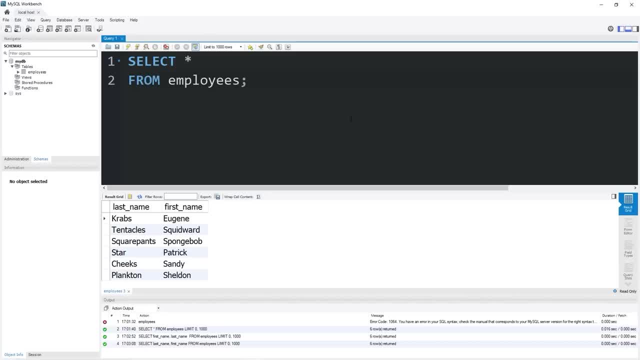 everything with the asterisk. There is a clause known as asterisk. There is a clause known as the where clause. If we're looking for something specific, let's add where. Then what are we looking for exactly? We can write some criteria. 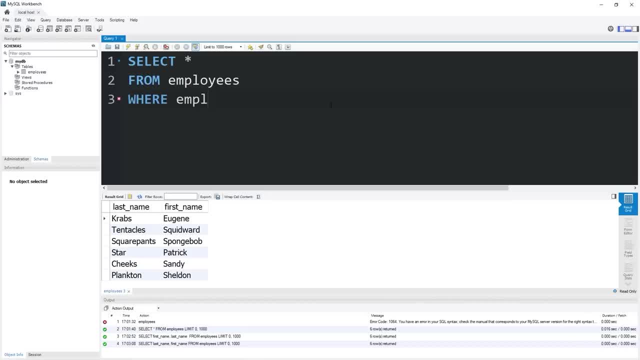 Let's select all from employees where employee ID equals 1.. Then end your statement with a semicolon. This will give us a specific employee: the employee that has an ID of 1.. If I set employee ID to be 2, that would give us Squidward. 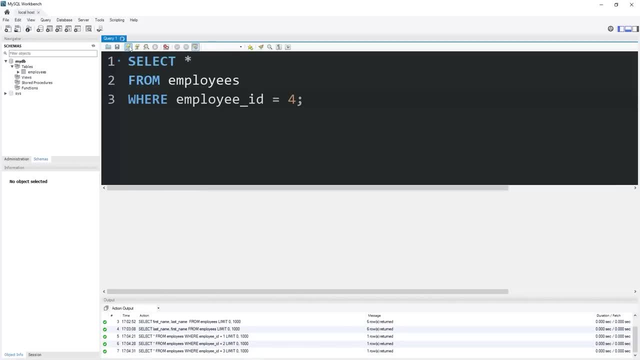 3 would be SpongeBob 4. Patrick. I think you get the idea. Here's an exercise. Let's find all the data from employees where the first name equals SpongeBob. Where first name equals SpongeBob, This query will return employee ID 3.. 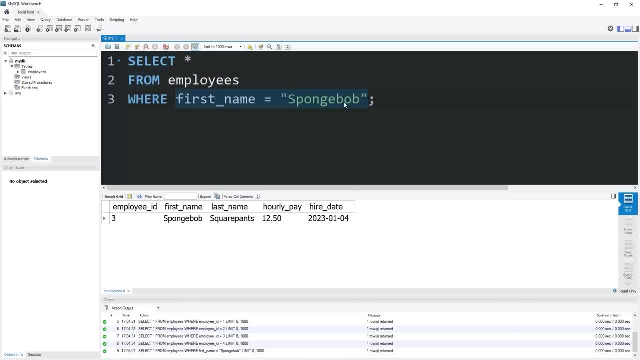 The first name, last name, hourly pay and hire date. Here's another example. Let's find all employees That have an hourly pay greater than or equal to 15.. Our criteria will be: where hourly pay is greater than, We'll use the greater than operator. 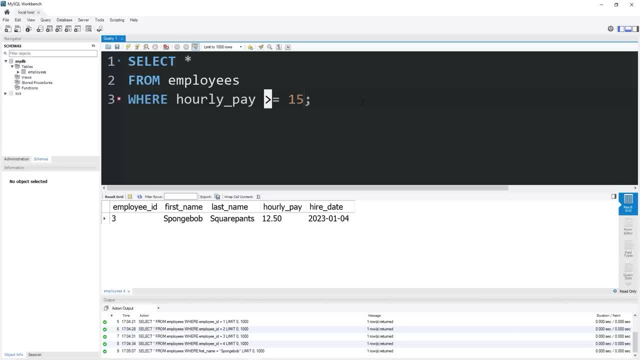 Or equal to 15.. This returns 3 employees: Mr Krabs, Squidward and Sandy. All 3 of them have an hourly pay of $15 per hour or greater. It is possible your query can return multiple results. 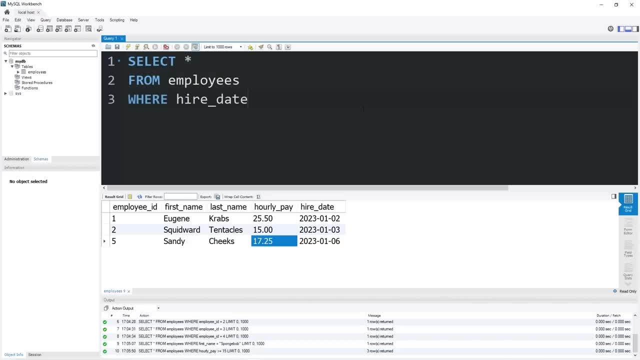 Let's find anybody that has a hire date less than or equal to perhaps the year 2023, January 3rd. This query returns 2 results: Eugene Krabs and Squidward Tentacles. They both match this criteria. In this case, we use the less than or equals to operator. 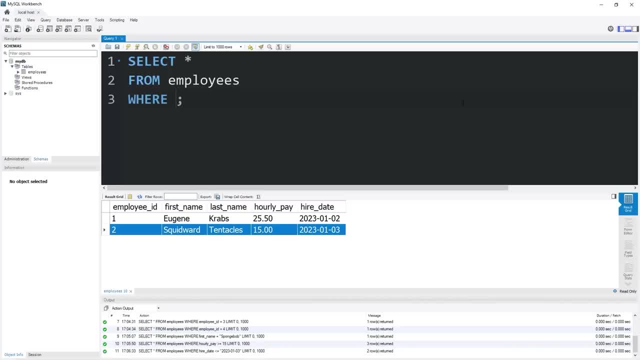 Another operator you should know about is the last comparison operator. It's an exclamation point and an equal sign. We will check if something is not equal. Let's find where employee ID does not equal 1.. Who are all the employees that have an ID not equal to 1?? 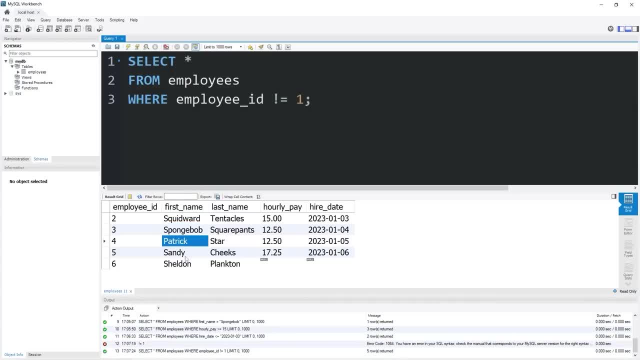 That gives us Squidward SpongeBob, Patrick, Sandy and Plankton. On the other hand, if I set this to 1, that would give us Mr Krabs. That is the not comparison operator If you need to check, if something is. 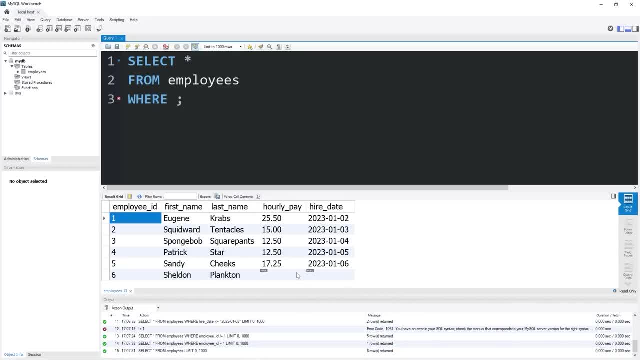 not equal. In this next example, let's pretend that we're human resources. We need to find any employees that do not have a hire date and then begin the paperwork for them. Currently, Plankton's hourly pay and hire date are both set to null. 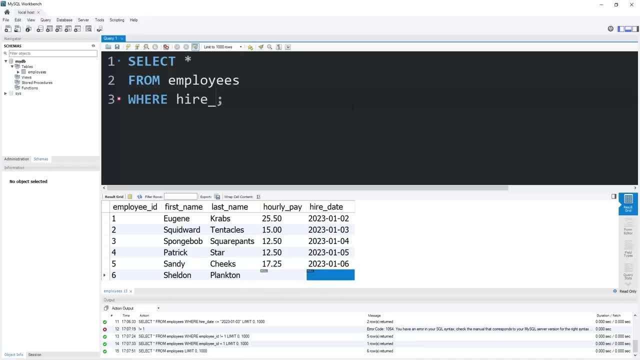 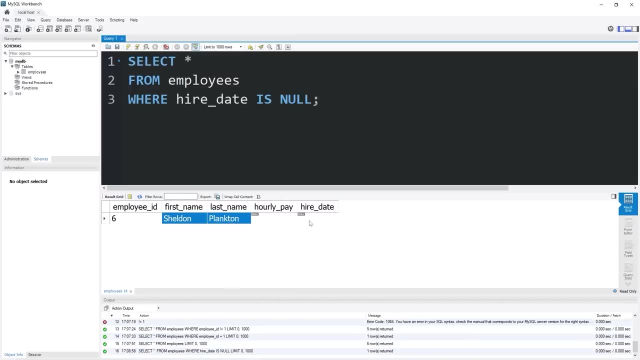 Null, meaning no value. In place of saying you know, hire date equals null. in place of using the equal sign we would type is select all from employees where hire date is null. That would return Sheldon Plankton because his hire date is null, Not equals null. 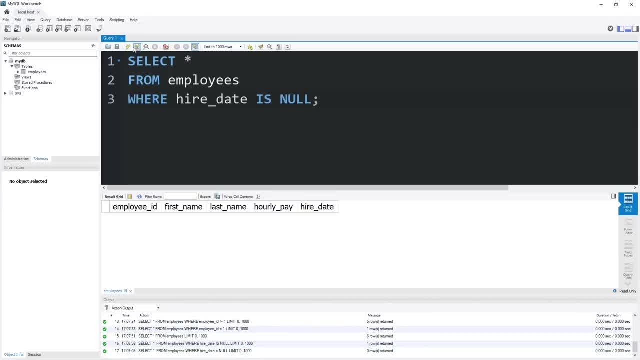 that doesn't work. It would be is null. You could even say is not null. That would return every employee that does have a hire date- Alright, everybody. so that is how to query data from a table. Select whatever you're looking for. 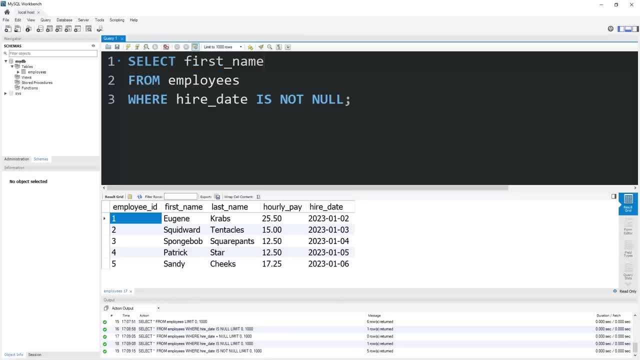 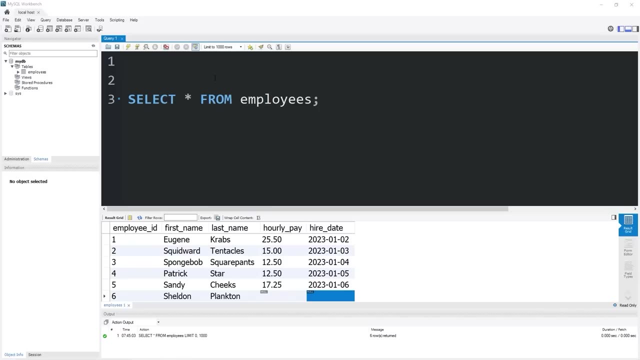 It can be everything or specific columns from a table of your choosing, where the results equal some criteria that you set. It really depends on what you're looking for, And that is how to query data from a table. Hey, everybody, in this video I'm going to show you. 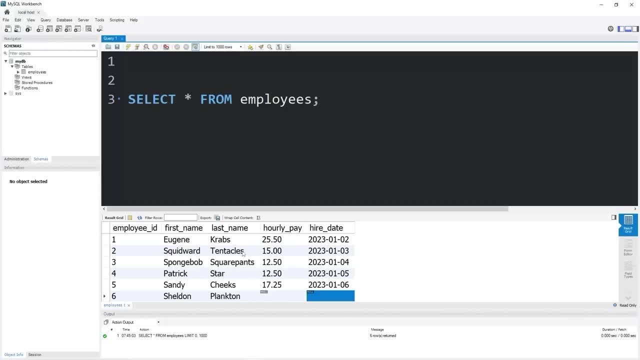 how we can update and delete data from a table. In my example, we have a table of employees. However, Sheldon Plankton is missing some information: An hourly pay and a hire date. Let's update those fields To update some data in a table. 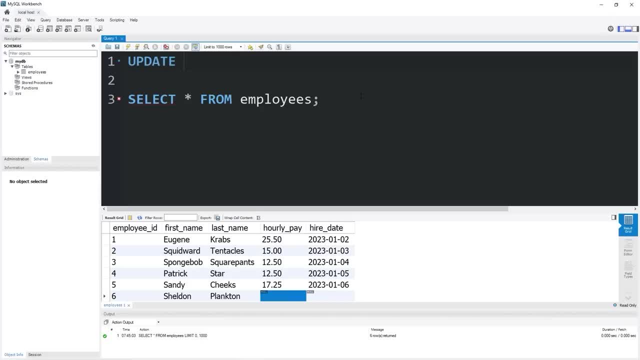 we would use the update keyword- The name of the table- Employees in my example- Then set which column would we like to interact with. first, Let's interact with hourly pay. Set hourly pay. Let's pay Plankton $10.00 and $0.25 per hour. 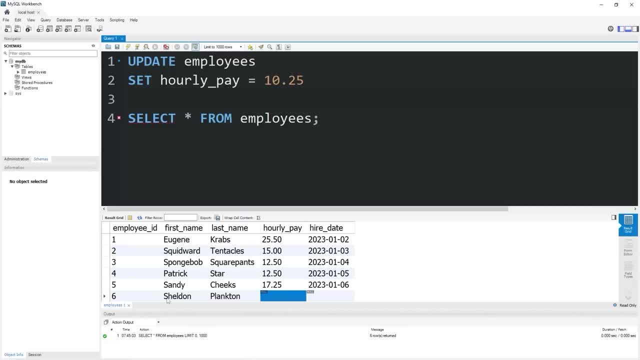 We should probably add a where clause. I need to specifically select Plankton where let's select his employee ID, Where employee ID equals 6.. Then semicolon to end the statement. You could also select Plankton by his first name or last name as well. 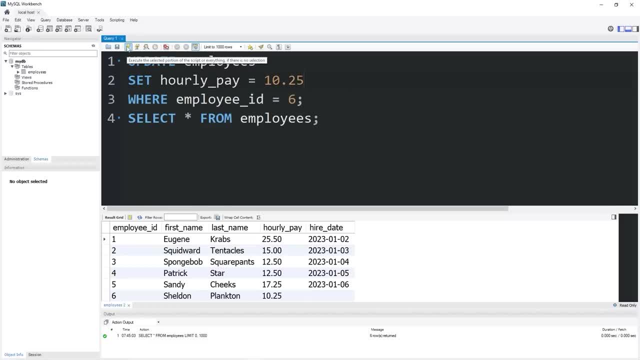 When I execute the script, Plankton's hourly pay is now $10.25 per hour. To update multiple columns, you can change more than one field at once. After your first change, you can add a comma, Then change another field. Let's change Plankton's hire date to. 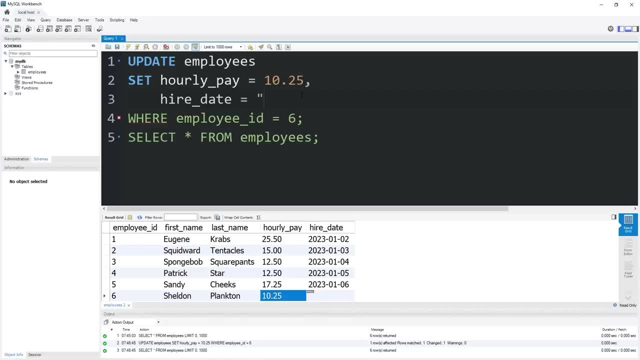 be the following: Hire date equals 10: 23 dash, 0 dash 07.. I'll make his hourly pay $10.50.. I'm feeling generous. Here we are. Plankton's hourly pay is now $10.50.. 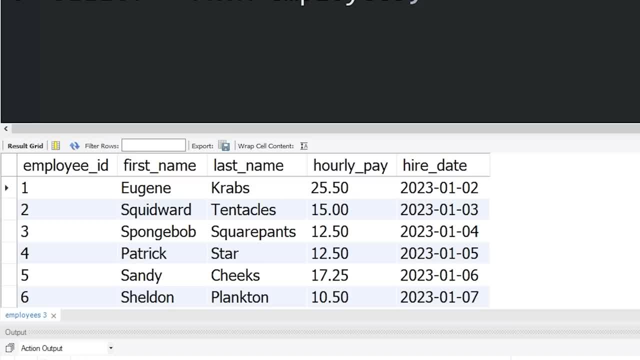 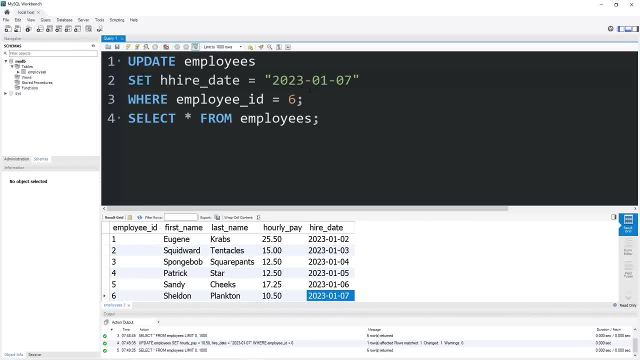 His hire date is January 7th 2023.. To set a field to null, meaning no value, you would just say equals null. For example, let's take Plankton's hire date. set the hire date equal to null. Plankton's. 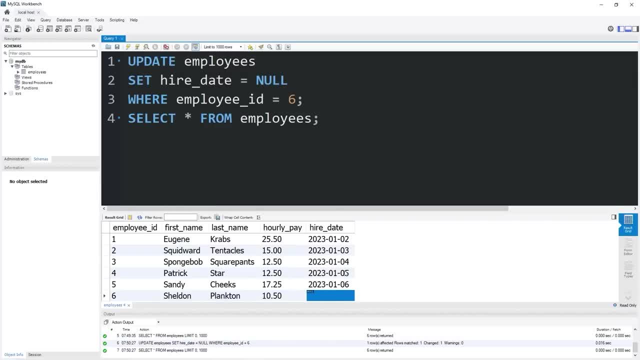 hire date is now null, So maybe we're going to fire him or something. In this next example I'll give you a demonstration, but you don't want to follow along. To update all of the rows within a column, you would exclude the where clause. 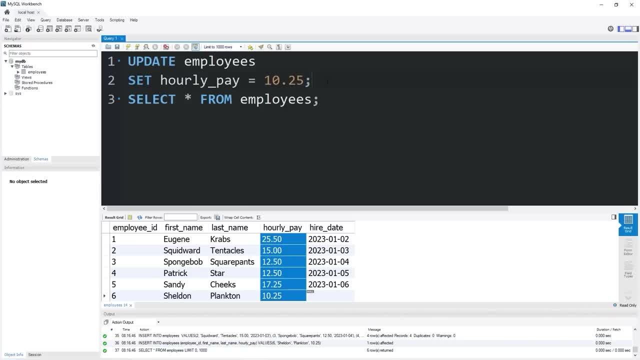 If I were to set hourly pay equal to $10.25, that would affect all of the rows. After executing this statement, the hourly pay for everybody is now $10.25.. That's an example of how you could set a column to be one consistent value. 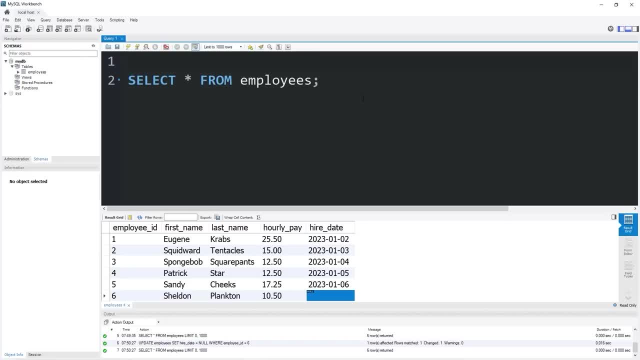 To delete a row from a table, you would type delete from the name of the table. Now, don't write just the statement. it will delete all rows in your table. Here's an example: do not do this. I will delete from employees There My whole. 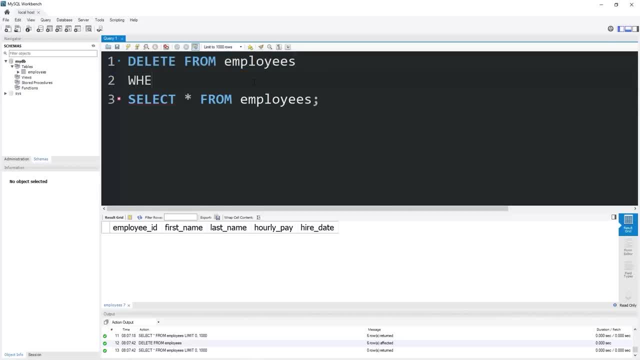 table is gone. Do not do this. Be sure to add a where clause when deleting from a table, Otherwise this will delete all your rows Where employee ID equals 6.. Plankton is no longer there. Alright, everybody, that is a super. 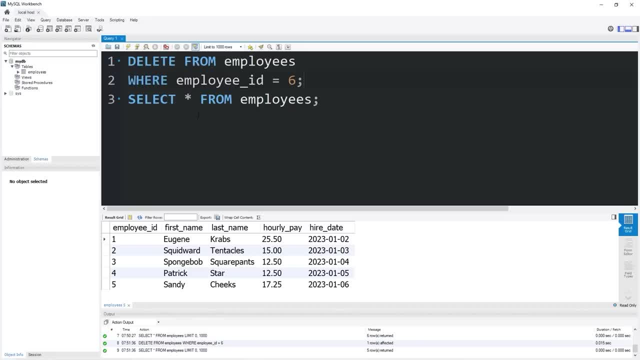 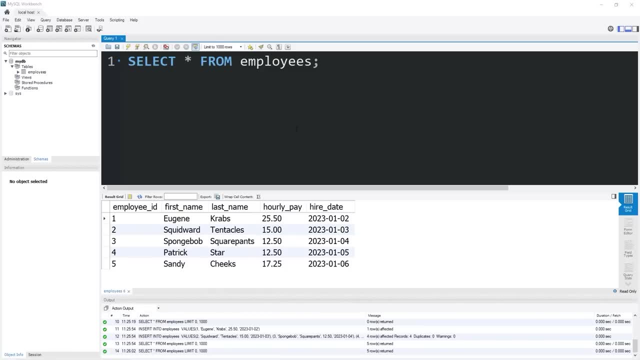 quick video on how to update and delete data from a table. Hey everybody, In this topic I'm going to explain auto commit, commit and rollback. Auto commit is a mode By default. auto commit is set to on Whenever you execute a transaction within MySQL. 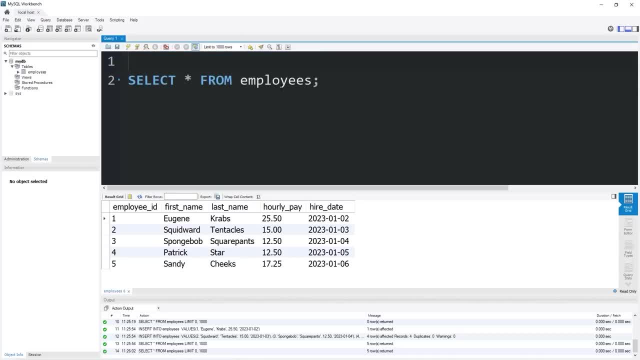 that transaction is saved. What if we were to make a transaction and we need to undo that transaction? For example, what if we accidentally delete all of the rows of this table? Don't do what I do, but I'll give you a demonstration. I accidentally type in: 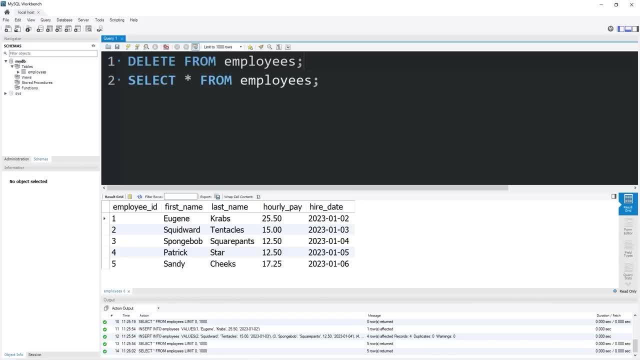 delete from employees, but I forget to add a where clause. Well, all my rows are now gone. How do I undo these changes? Well, what we're going to do is set auto commit to equal off. With this setting set to off, our transactions will not save automatically. 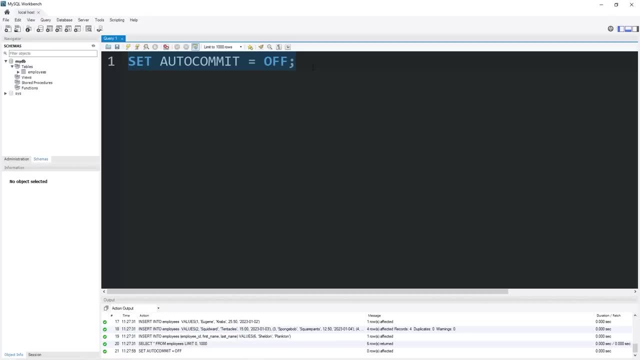 We would need to manually save each transaction. It creates a save point, so to say. I'm going to create a save point by typing commit, then execute. Now I'm going to select my table, select all from the name of my table. then I'm going to go ahead and delete all the rows. 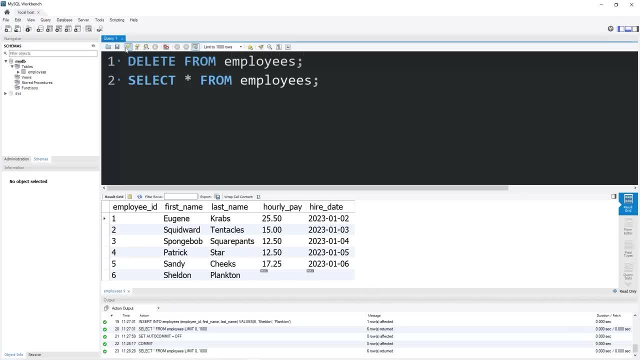 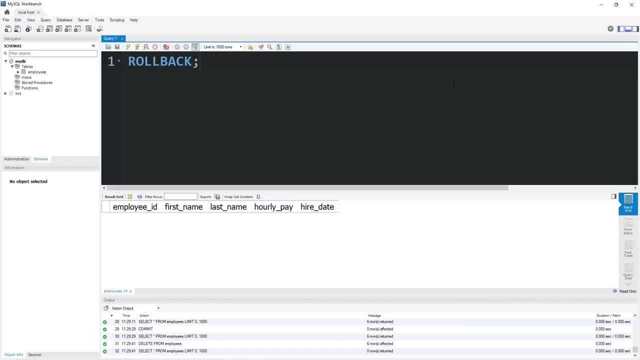 Delete from employees. Oh shoot, but I forgot to add a where clause. My whole table is gone now. Luckily, we created a save point with that commit statement To undo these changes. I can execute the roll back statement. This will restore my current transaction. 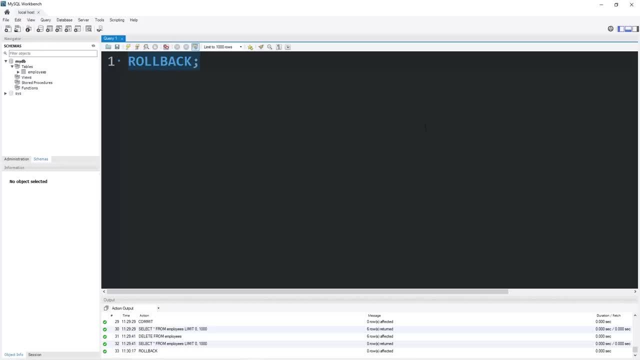 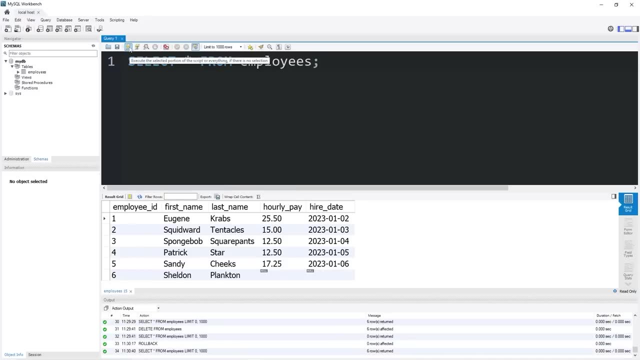 back to the previous save point where we used commit. Now, if I were to select all from the name of my table, our table is back to what it previously was. And again, to save any changes, let's say I delete my whole table again. delete from. 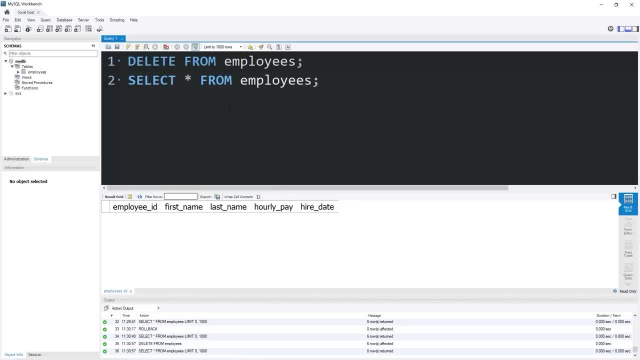 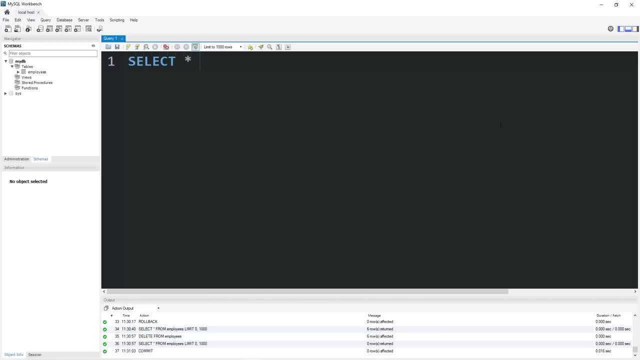 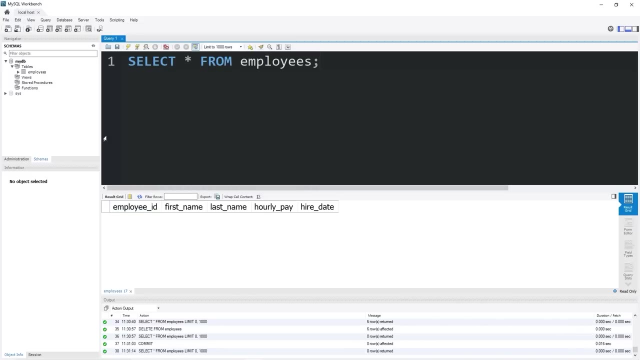 employees. if I want to save this change, I would commit. Then again I will select my table and that last change is now saved. My whole table is gone. So yeah, that is auto commit, commit and roll back. By default, auto commit is set to be on Any transactions. 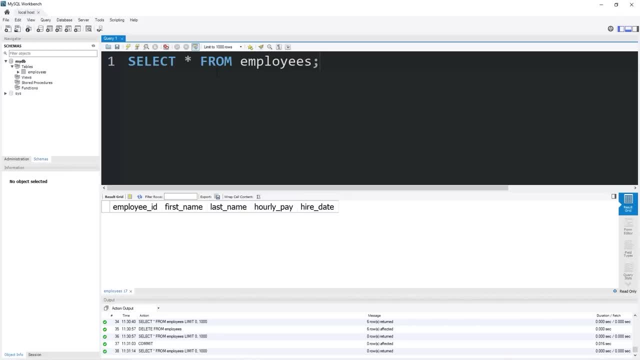 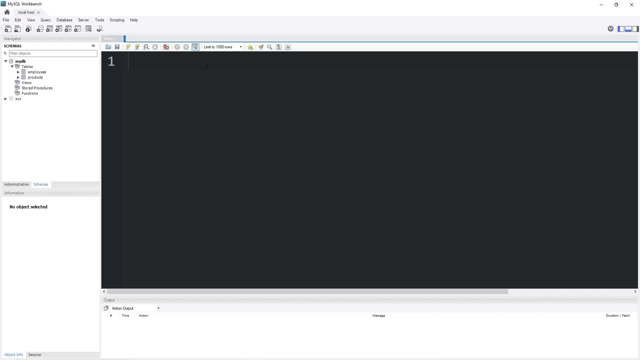 after executing are saved. If that mode is set to off, you can commit any changes manually. To undo any changes, use that roll back statement. So yeah, that is auto commit, commit and roll back in MySQL. Hey everybody in this topic I have a super quick. 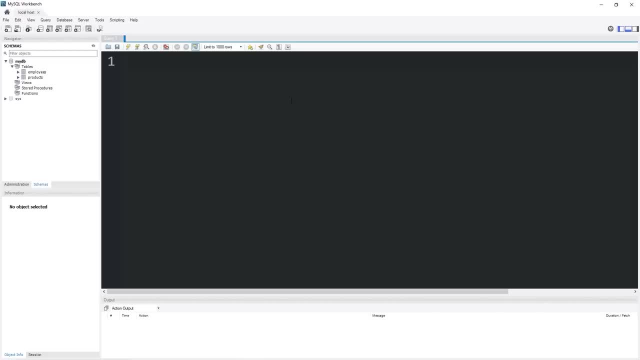 video on getting the current date and time in MySQL. Let's create a temporary table At the end of this topic. we will delete it. Create table. I will name this table test. We will have three columns: The current date. I will name the column my date. 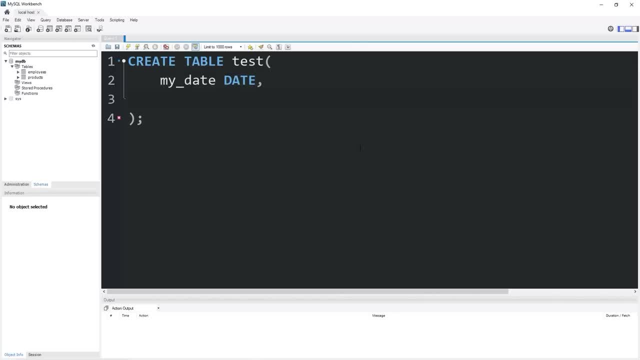 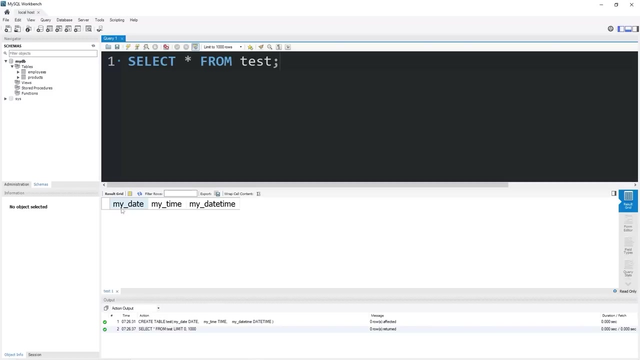 the data type is date, my time. the data type is time, then we will combine both: my date time, the data type is date time. Let's create this table. It was created successfully. Then I will select all from our table test. We have three columns A date. 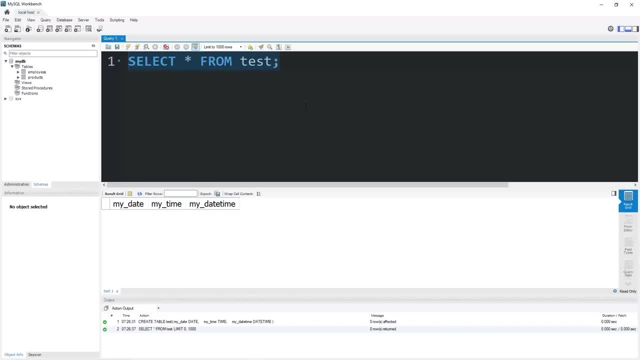 a time and a date time which combines both. So how do we get the current date? Maybe we need to create a time stamp of when some event happened, Maybe a higher date for our employees? So I am going to insert into the name of my table test. 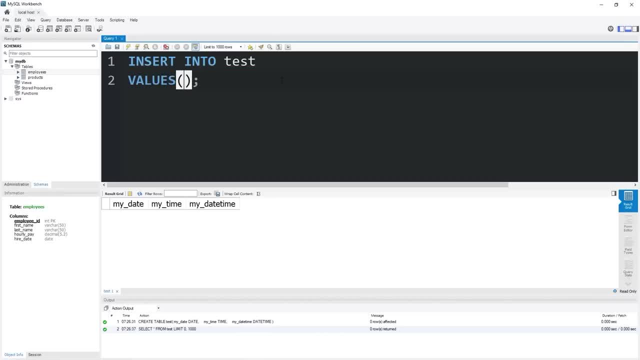 some values For the current date. there is a built in function. current underscore date. then add a set of parentheses. This function will return the current date. For the current time. there is a current time function. add a set of parentheses to the end of that function. 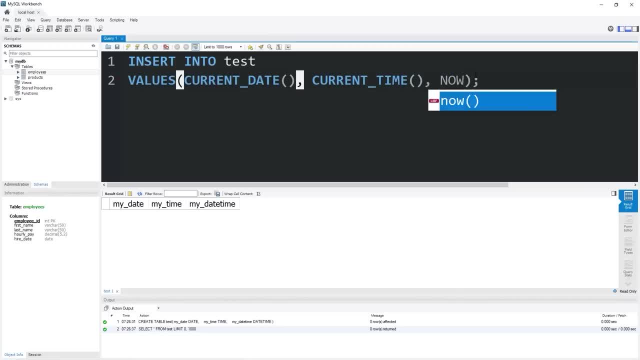 For the date time. you could just say now. then add a set of parentheses After inserting this row, let's select all from our table test. Here is the current date of me filming this video: October 21st 2022. the time is 7 in the morning. 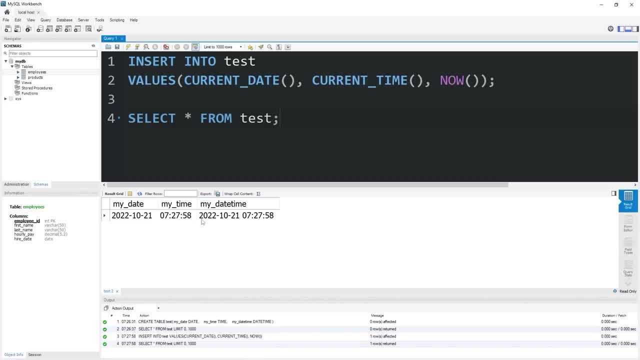 the current date time is October 21st 2022, 7 in the morning. A date time would probably be good for some sort of transaction you need to record. For the time being, I am going to set the current time to be null, as well as. 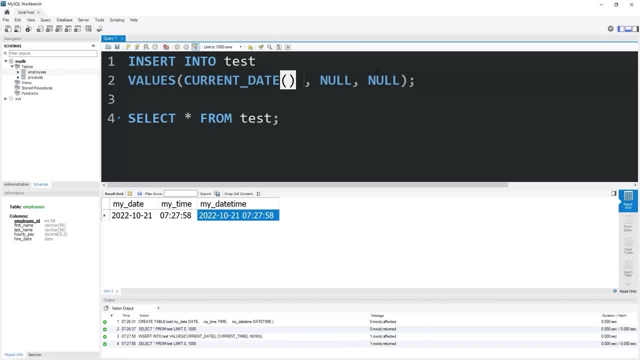 the date time to be null. Now, if you were to take your current date, then add plus one. This part of my statement would refer to tomorrow, October 22nd. If you were to take your current date minus one, that would technically be yesterday, October 20th. 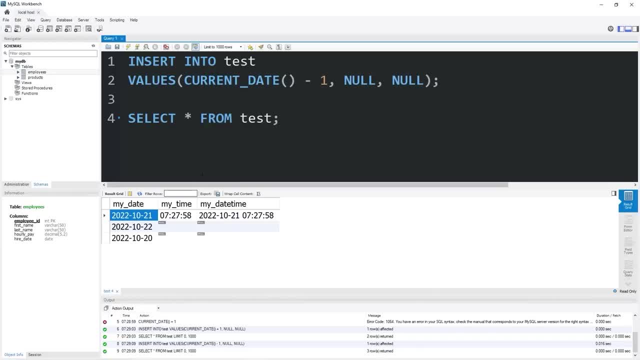 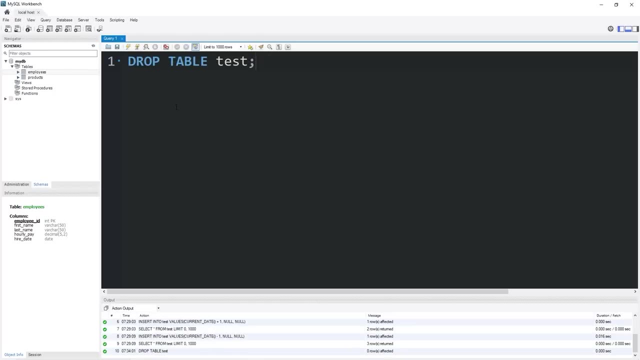 You could do something similar with your time and date time. You can add or subtract seconds, but I think that's pretty self explanatory. We don't need this test table anymore, so we can delete it. Drop table test And it's gone. Alright, everybody, so that was a super quick topic. 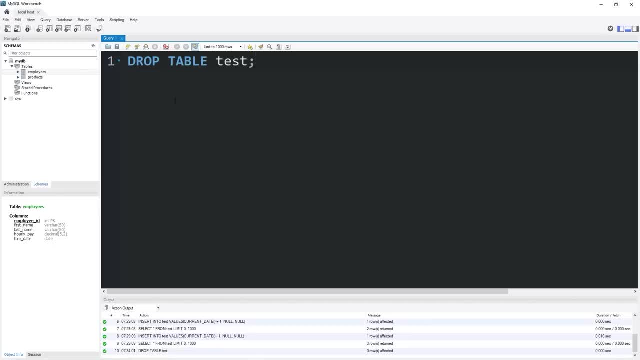 but I thought I needed to cover it. That is how to get the current date time and date time in MySQL. Hey everybody, I have a quick video on the unique constraint. The unique constraint ensures that all values in a column are all different. 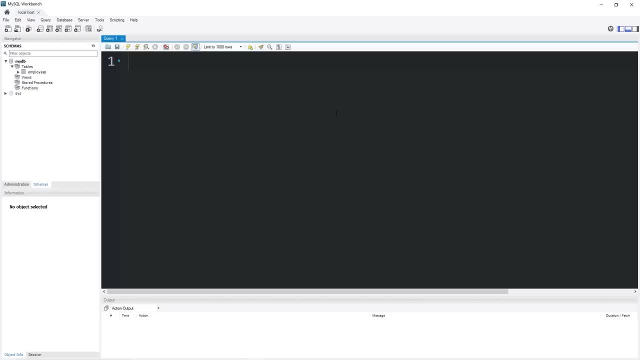 That's basically it. We can add this constraint when we create a table or after. Let's create a new table. Create a table. Let's create a table of products. What products do we offer? We'll list the columns. Let's add a. product id: The data type will be int. Product name: The data type will be varchar, maybe 25 characters, Then a price Price: The data type will be decimal. Our price will have a max size of 4 digits and a precision of. 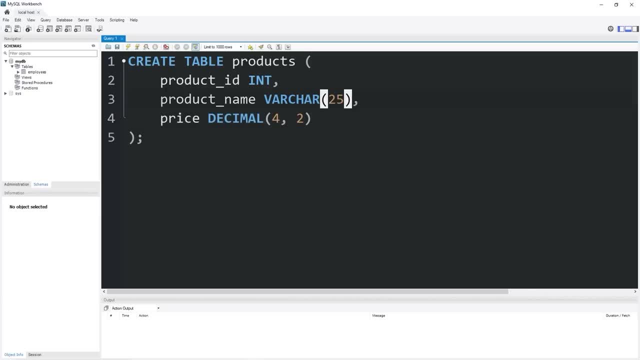 2 decimal places To add the unique constraint. select a column after the data type, add the keyword unique And that's all you have to do With this keyword unique. we can't insert any product names that are the same. They all have to be. 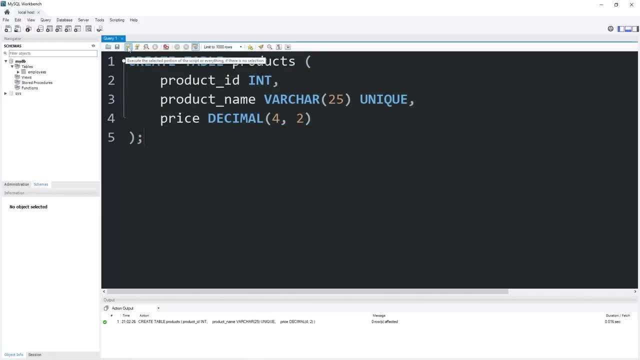 well, unique. Let's create this table. Let's say that you forget the unique keyword. Then you create the table. What you could do instead is type: alter table: the name of the table products which we just created. add constraint: unique: the name of the column within parentheses. 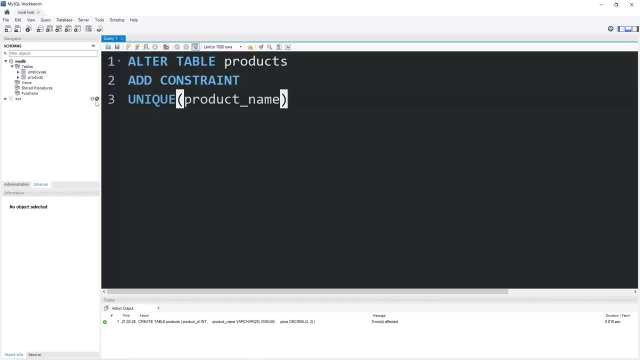 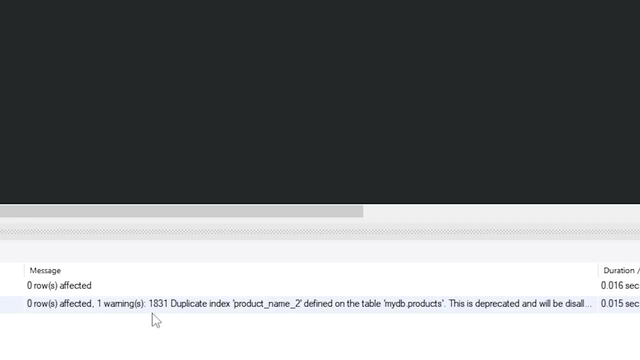 product name. If you forget to add a unique constraint to a column after you already create the table, that's what you can write. However, when I run this, I do have a warning. I already have a unique constraint on that column, But yeah, that's how you would add a unique. 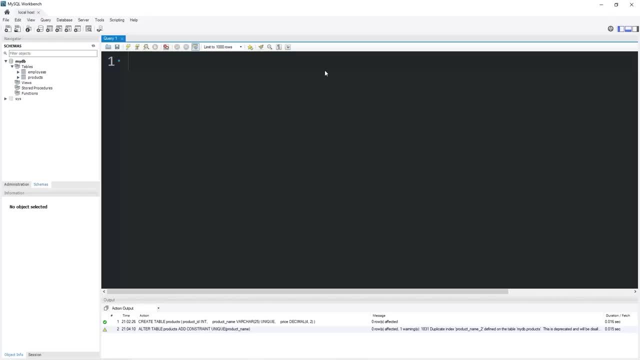 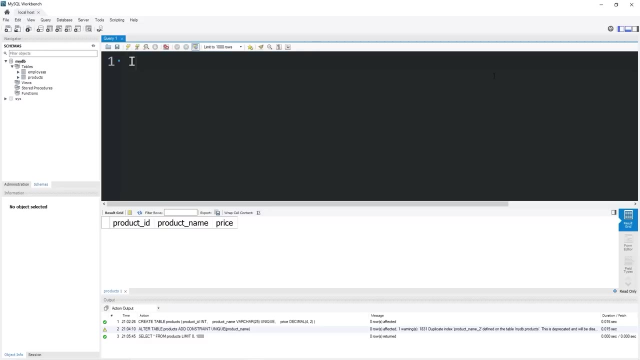 constraint to a column in a table you have already created. Let's select our table, Select all from products. We have a product ID column, product name and a price. Let's insert all of our values. Insert into the name of our table, which is products. 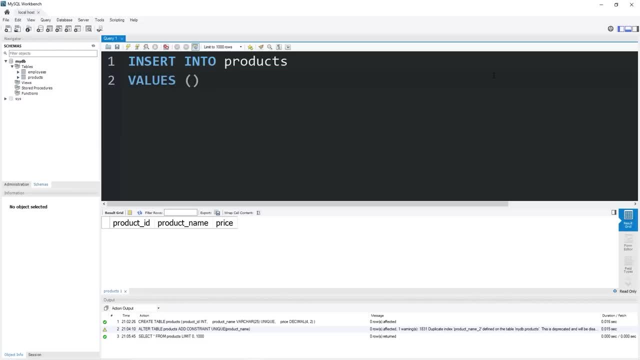 values. We'll insert maybe four rows. We'll need a product ID name, then a price For a product name. we have a hamburger and the product ID- I'm just making up a number- is 100, The name is hamburger, The price will be, The price will be. 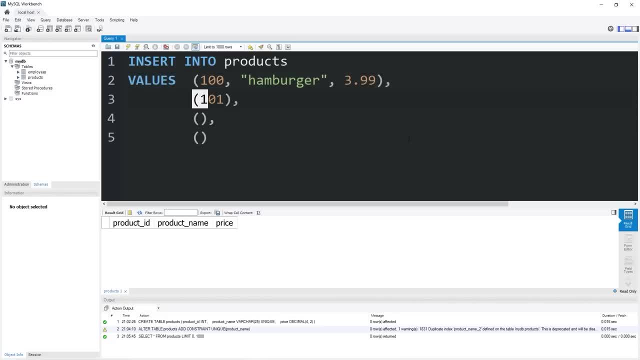 $3.99. Fries will be our next item. Then we have fries, The price will be $1.89. $1.02 Will be soda, The price is $1.00. even $1.03 will be ice cream, The price will be $1.49. 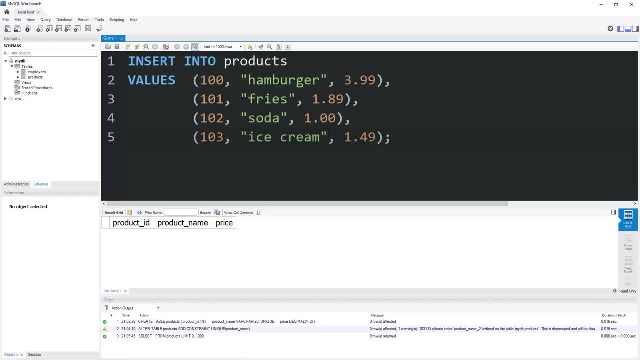 The price will be $1.49. The price will be $1.49. Let's test the unique constraint that we have added to the product name column. Suppose that I forget that I have fries on the menu already And I will add another row: $1.04. 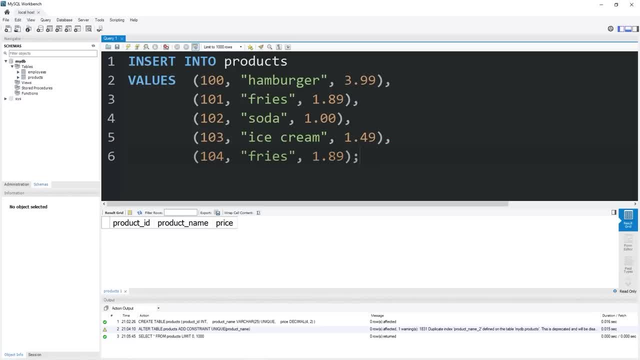 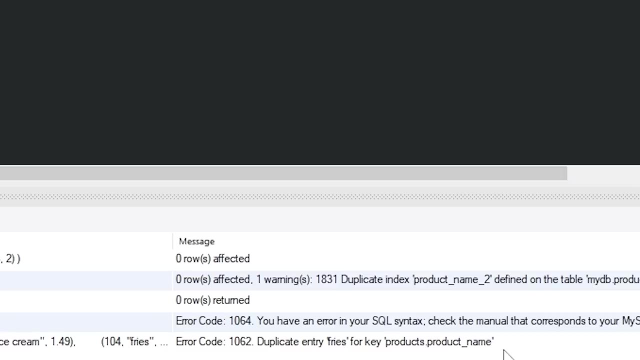 $1.04 fries- $1.89. Actually, let me change the price to maybe something different like $1.75. Here's what happens when I attempt to add two values that are the same. duplicate entry: fries for key products- dot product name. MySQL is telling us that we have. 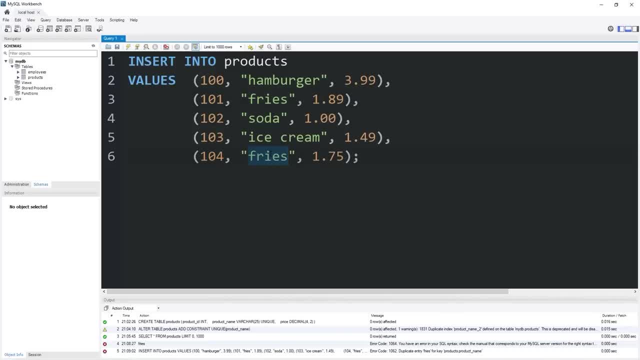 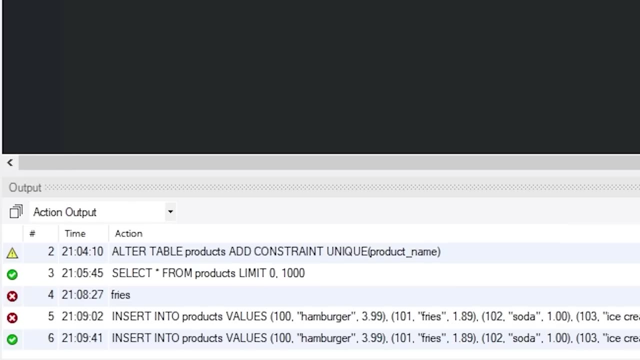 a duplicate under the product name column. We have fries twice. Since we added the unique constraint, all values in this column must be different. If I were to remove the last column where we have that duplicate, Well then this would run just fine. Now let's select everything from. 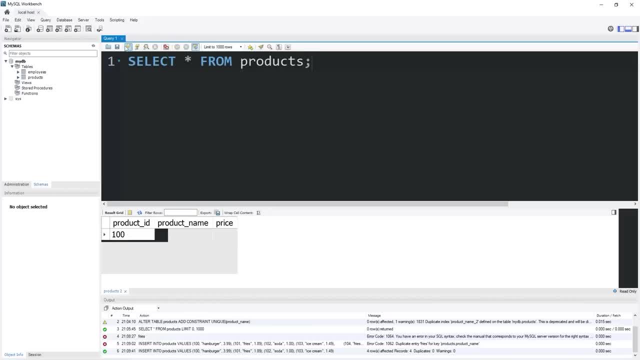 products. Yeah, there we go. here are the products. We have a hamburger, fries, soda and ice cream all on the menu. So, yeah, that's the unique constraint. You can add that constraint when you create a table or after Whatever column has that unique constraint: all the values need to be different. 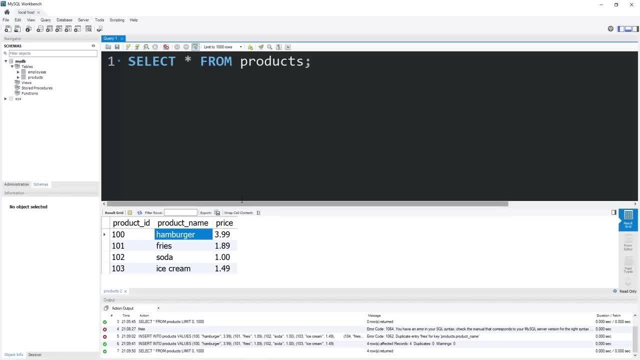 So yeah, that's the unique constraint in MySQL. Hey, everybody, in this topic I'm going to explain the not null constraint. The not null constraint can be added to a column when you create a table. Whenever we enter a new row, the value within that column can't be null. 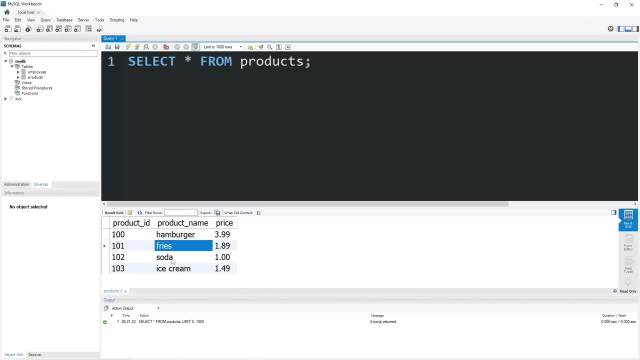 For example, I have table products. We have a hamburger, fries, soda, ice cream. If I were to recreate this table, I would type something like this: Create table products. I would list the columns We have products. product id: the data type is integer. 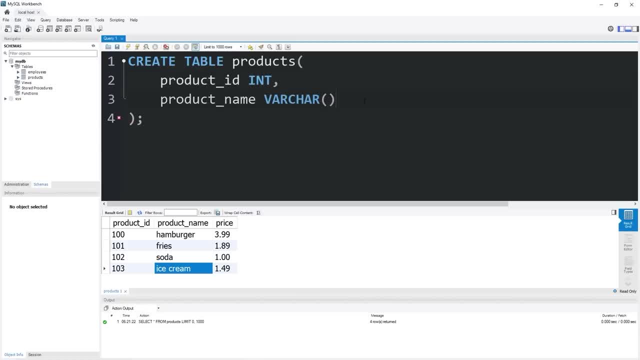 product name. the data type is varchar. I believe I set this to be 25 last time. then price: that is a decimal. We gave this column a max size of 4 digits and a precision of 2.. Any column that I do not want to have null values. 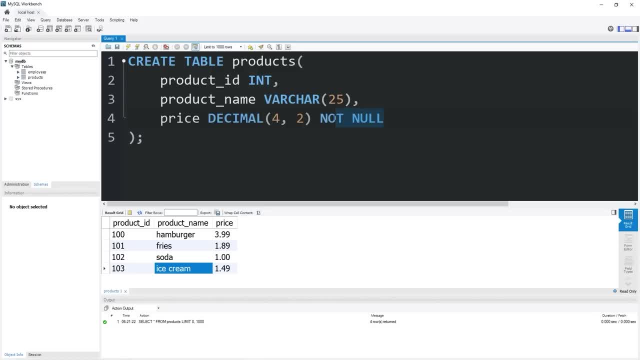 I will simply just add: not null. This is a constraint. Now I have already created this table, So I'm not going to execute this table. But that's how you would create a table that has the not null constraint After the column name. you just type: 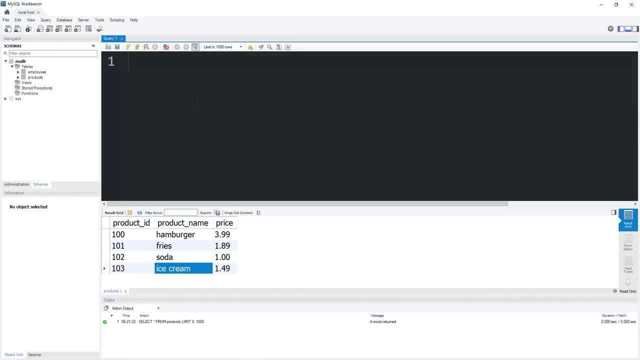 not null. To add the not null constraint to a table that already exists, you would instead type: alter table. the name of the table, modify the name of the column. the data type of the column, in this case decimal 4 comma 2, then not null. 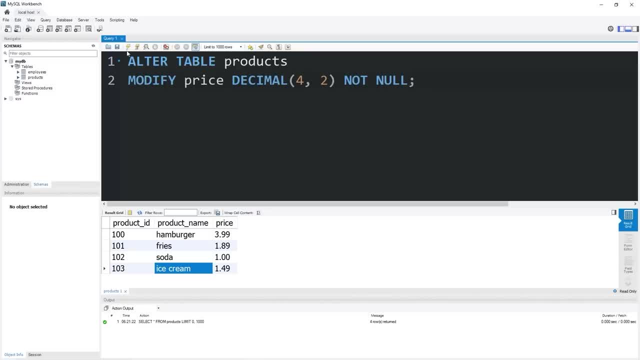 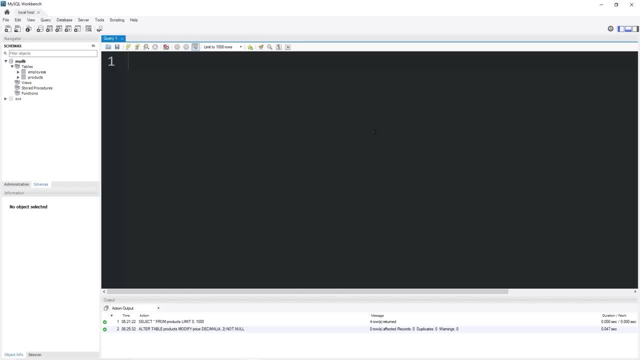 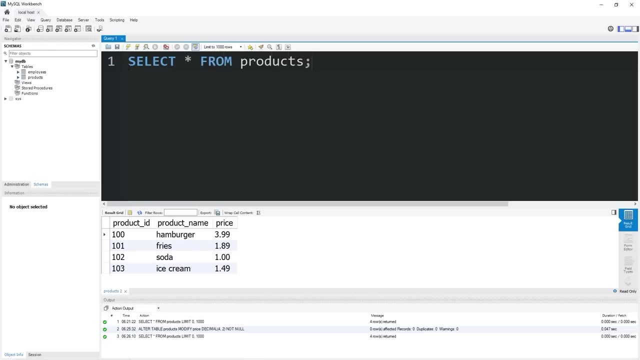 It's a little bit different than the unique constraint in the last topic, So let's execute this statement That seemed to work. Let's add a new item to the menu. I will select everything from my products table. select from products. Let's add a new item to the menu. 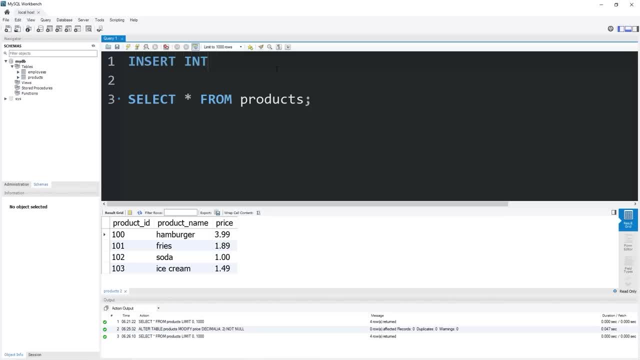 and we will test that. not null constraint. insert into products values. We have 104 Product ID. 104 will be. How about a cookie? I'm not going to set a price. I will say null for the price. Maybe I'm not decided on what the price is yet. 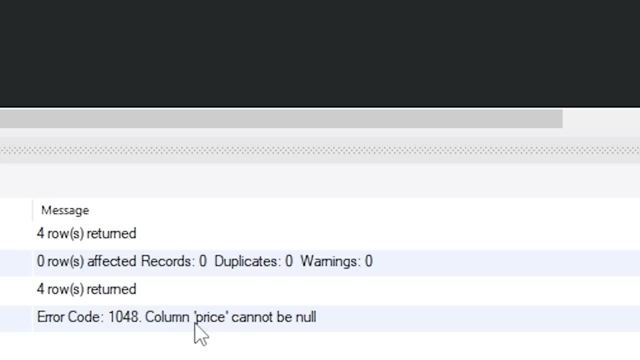 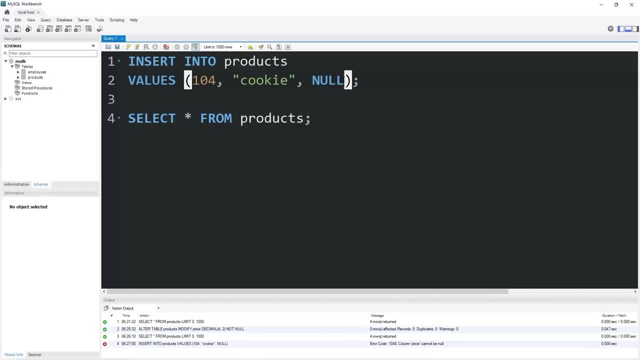 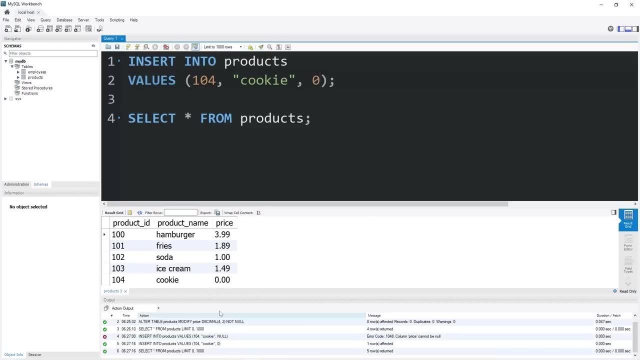 After executing this statement. Well, we have an error. Column price cannot be null. Since we set that not null constraint on the product price, We can't enter a null value. We could set this to be zero, That's acceptable, But it can't be null. So, yeah, everybody, that's the not null constraint. 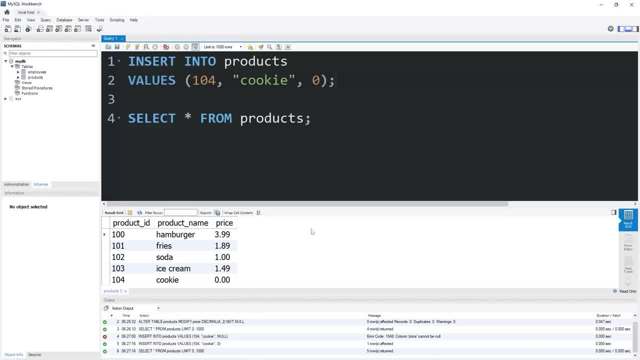 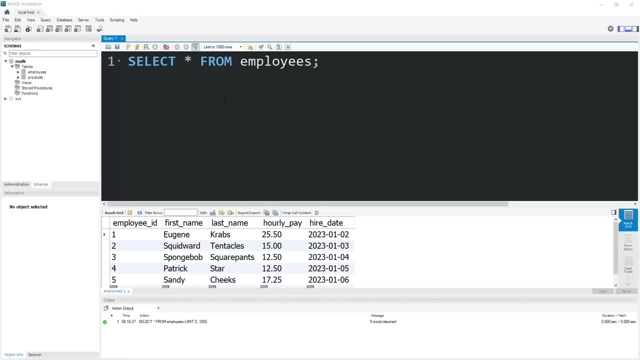 It's a useful constraint to verify input. If there's any column that you don't want to have any null values, Just add that constraint. And yeah, that is the not null constraint in MySQL. Hey, everybody in this topic I'm going to explain the check constraint. 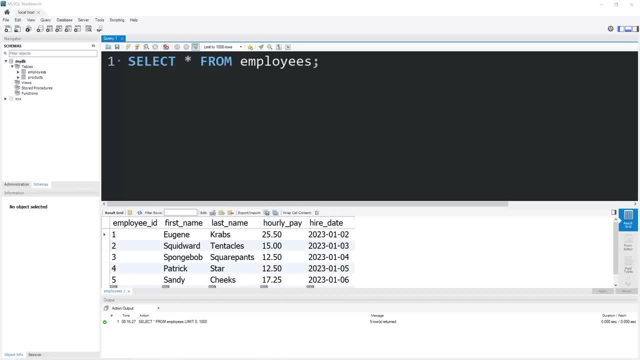 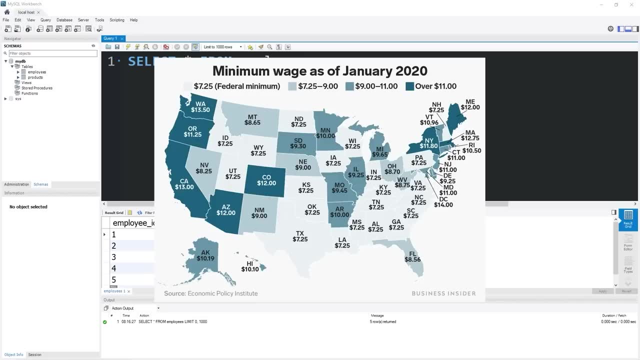 The check constraint is used to limit what values can be placed in a column. For example, I live in the United States. Depending on which state you live in, There is a minimum hourly wage that employers have to pay. In this example, let's set an hourly pay. 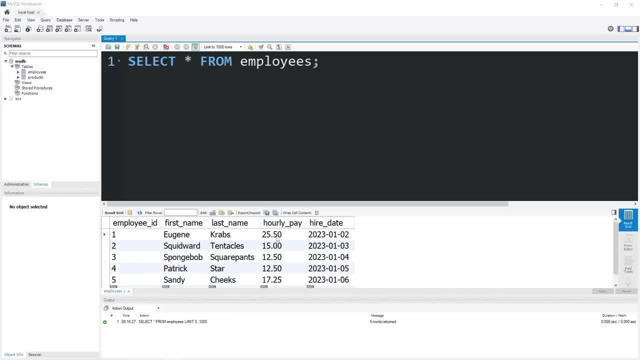 to our employees table. Every employee needs to be paid at least the minimum wage in that region And we can do that with the check constraint. We have our table of employees. If I were to recreate this table, It would look like this: I think that was pretty close. 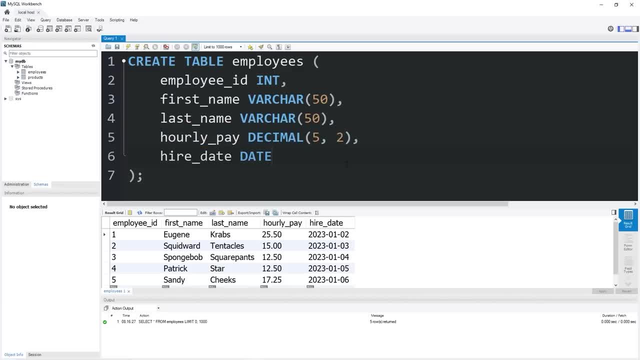 To add a check to a column At the end of our table. This is what we would write: Check. Then, within parenthesis, What sort of condition do we want? Let's check to see if our hourly pay column Is greater than or equal to, Maybe $10 per hour. 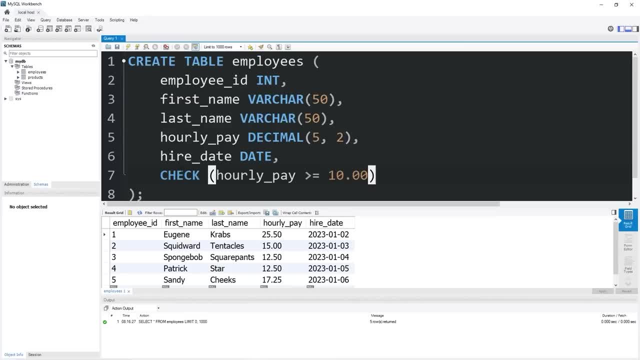 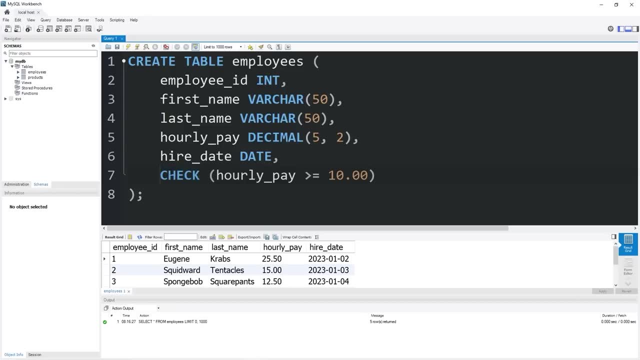 That will be the minimum wage in this region. This would work if we were to create this table. However, if we were to create this table, It's typically a good idea To give your check a name, Just in case you need to drop it later You can easily identify it. 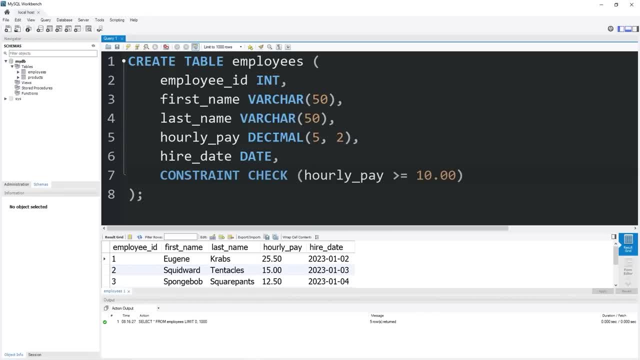 So precede check with constraint, Then a constraint name. What about CHK, meaning check Underscore, hourly Pay? This check will be known as Check hourly pay, So we can identify it. Then we can drop it or make any changes to it If we need to Execute this statement. 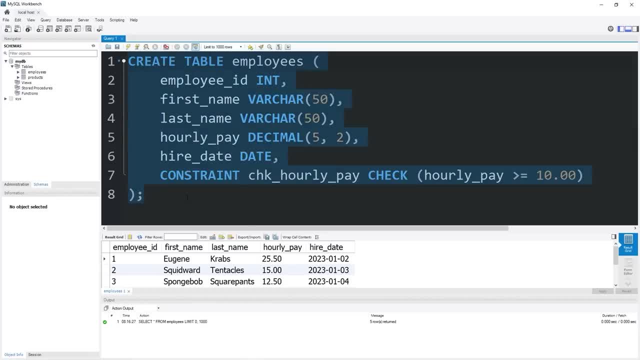 But to add a check constraint to a table, You would just add a row like this to the bottom. If you instead need to add a check constraint To a table that already exists, This would be the syntax Alter table, The name of the table: Add constraint. Then we need a unique name. 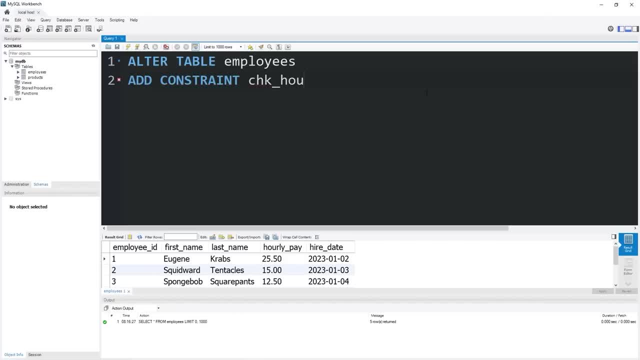 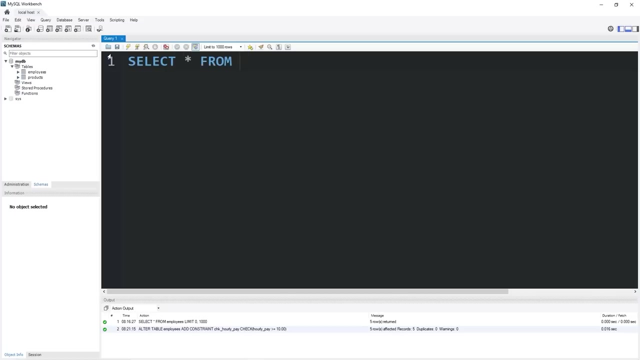 For this constraint. Check hourly pay. That's fine. Then the check within parenthesis: Hourly pay Is greater than Or equal to, Ten Ten dollars per hour. Okay, let's run this. Yeah, that appears to have worked. I'm going to select all From employees. Let's take a look at our table. 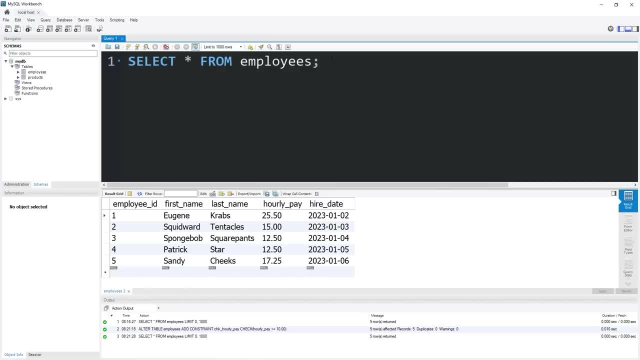 Then we will attempt To add a new employee Insert into Employees Values. We need an employee ID. First name, last name, hourly pay, Then a higher date Employee ID will be six. First name: Sheldon Plankton For hourly pay. Let's attempt to pay plankton. 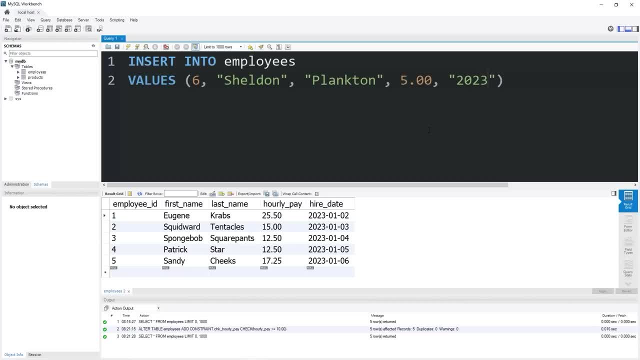 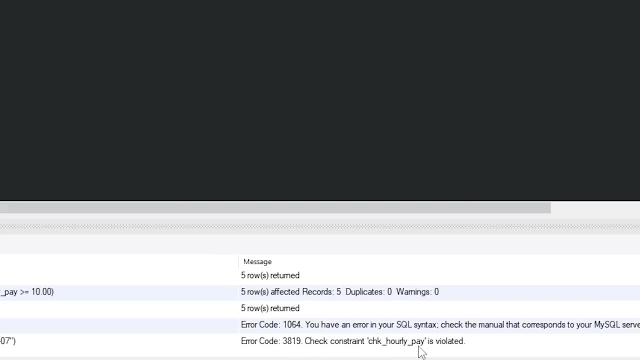 Maybe five dollars per hour, Then a higher date: Twenty twenty three. dash zero one, Dash zero seven. Let's see if that check constraint kicks in. We're paying plankton Under ten dollars per hour. Yeah, it doesn't appear that we can do so. Check constraint, check hourly pay. 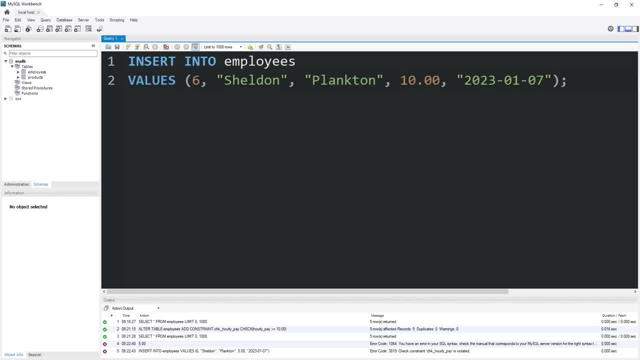 Is violated. Now let's pay plankton Ten dollars per hour. Yeah, that worked just fine. If you need to delete a check, You would type alter table, The name of the table, Drop Check, Then the name that you gave that check. In my case it was Check hourly pay. 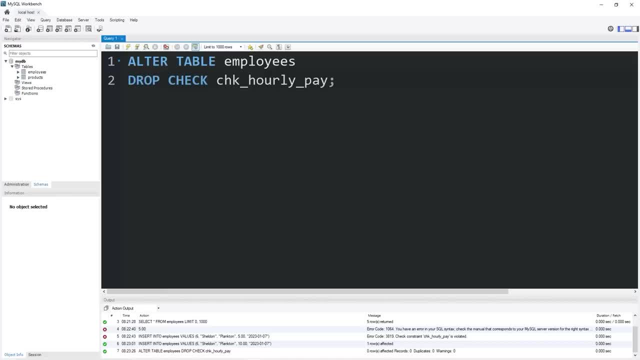 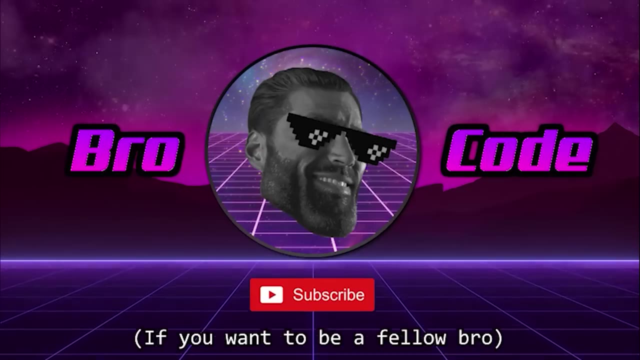 And that check Has been dropped. Yeah, everybody, that is the check constraint. It's used to limit what values Can be placed in a column. It's another useful method for checking input And that is the Check constraint in MySQL. Hey everybody, In this topic I'm going to explain the 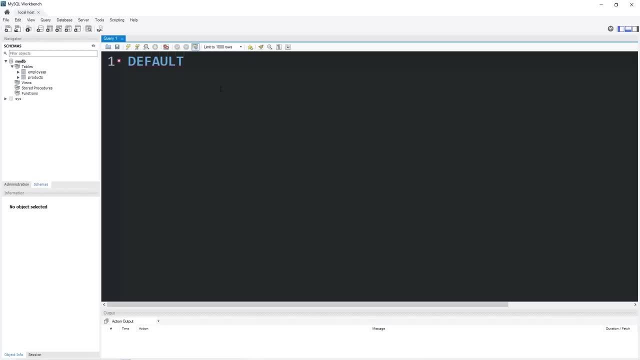 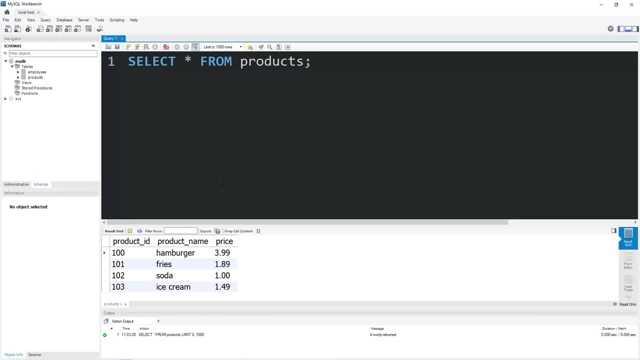 Default constraint When inserting a new row. If we do not specify a value for a column By default, we can add some value that we set. Here's an example: Select all from our products table. Select all from products. In an earlier example We have a table of products. 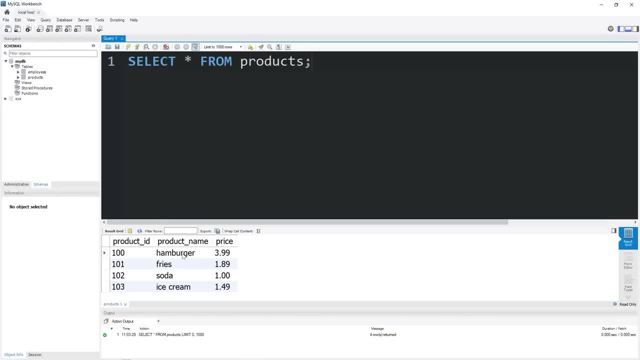 A few items on the menu for sale Are hamburgers, fries, soda and ice cream. Let's add a few items on the menu That would be free. This could include napkins, straws, Forks and spoons- Something you would commonly see At a fast food restaurant. 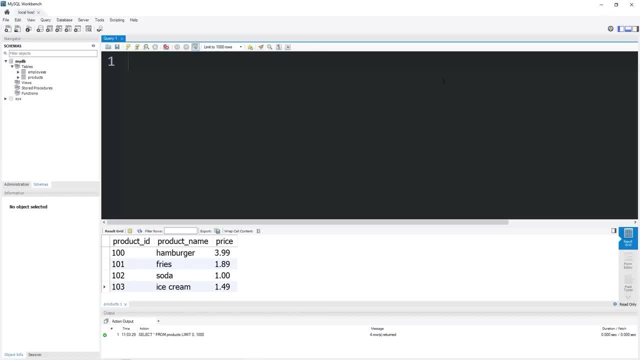 If we're not using the default constraint, We would have to enter in those prices manually. So let's insert Into our table Products Our values. Product ID 104 Will be A straw, The price will be $0.00. Let's do this all together, We have 105. 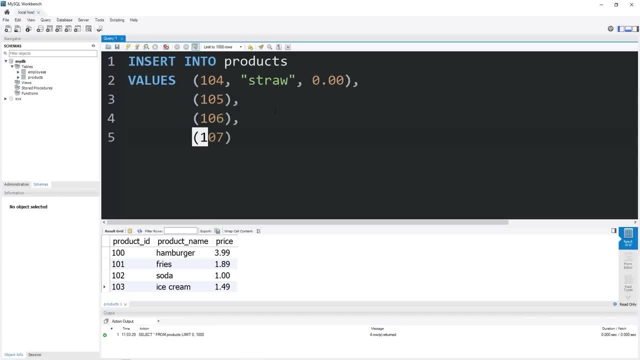 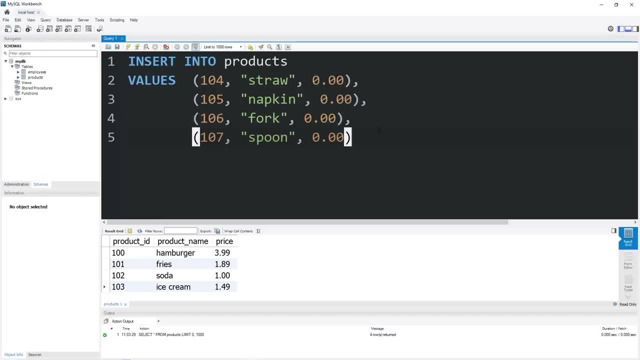 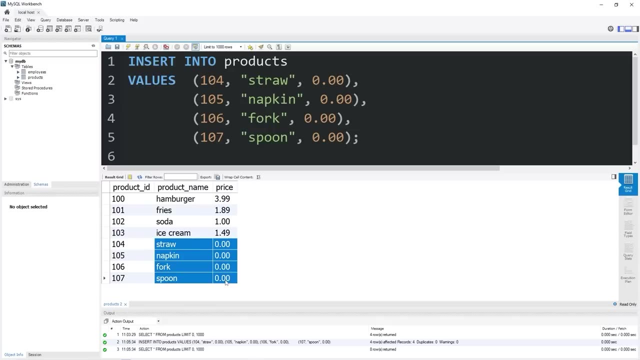 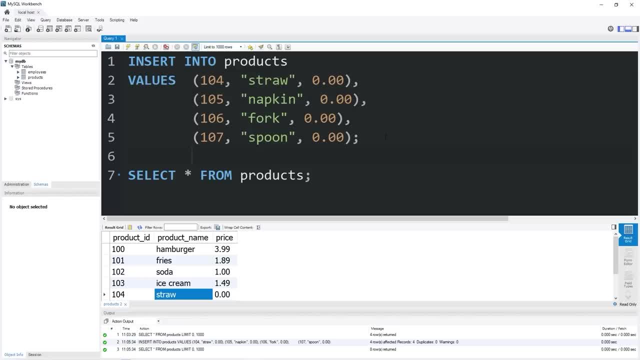 In place of explicitly stating a price. One way in which we can make our lives easier: If we're adding a bunch of free items To the menu, We could set a default constraint Where, if we don't explicitly set a price, The price will default to be $0.00. 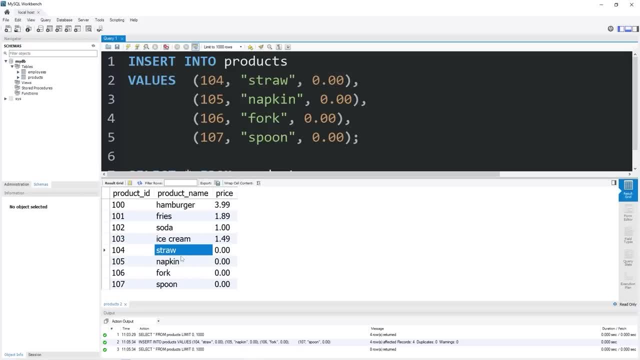 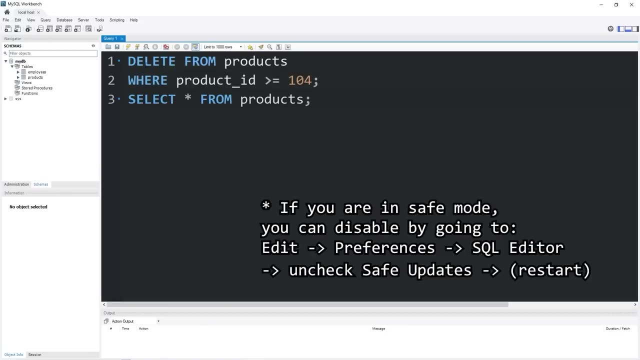 It will be free. So I'm going to undo everything that we just did. So I'm going to undo everything that we just did. Delete from Products Where Product ID is greater than Or equal to $104, And then we can Execute that statement. If we were recreating. 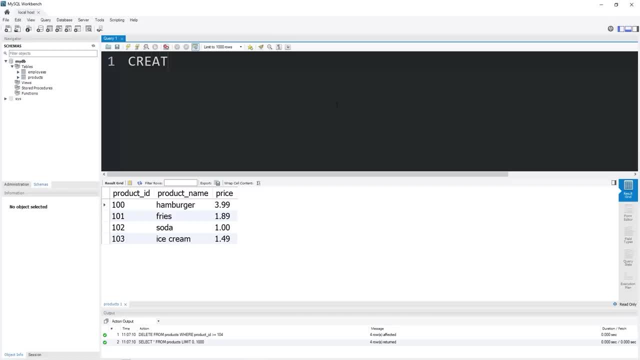 This table with the default constraint, We would type: Create table Products. in this case, Add our columns. We have a product ID. The data type is integer. We have a product Name. The data type is Varchar And I forgot what the size was. Looks like 25. 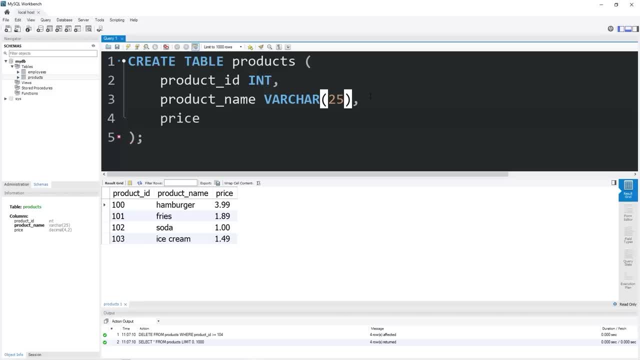 Then a price Which is a Decimal Max digit size of 4, Precision of 2. Now let's use the default constraint After the column. you would like to add that constraint to Then some value. I will set the default value to be $0.00, Or you could just say 0 too. 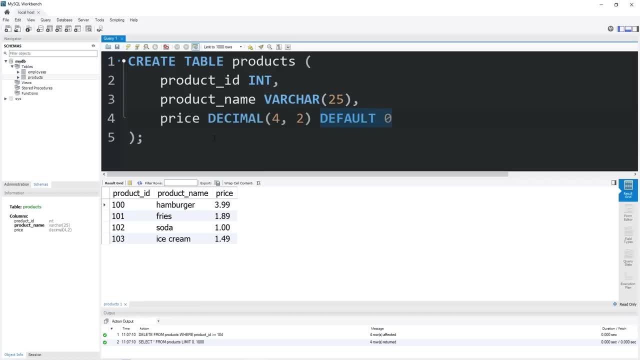 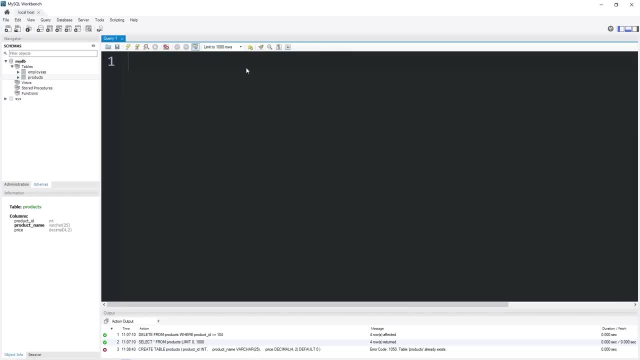 That would be fine. You would just add this constraint when creating a new table. However, I do already have a products table, So this technically wouldn't work Because that table already exists. Now to alter a table to include that constraint, You would instead type: Alter table- The name of the table. 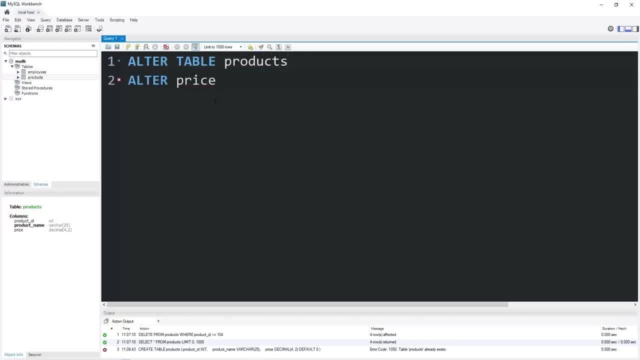 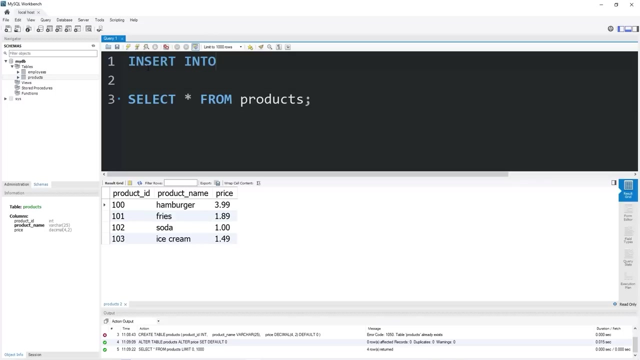 Alter the name of the column, Price, Set Default constraint, Then the value, So 0, And that appears to have worked. Let's select our products table. Select all from Products, Then we will insert some new rows. Insert Into Products, Then our values, So we had 4 rows. 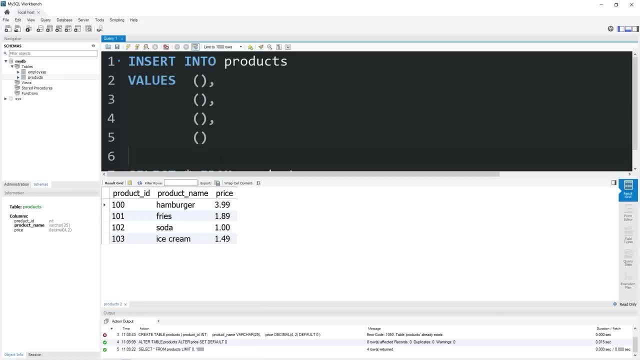 104 That was a straw, 105 Was a napkin, 106 Was a fork, 107 Is a spoon. Then finish the statement With a semicolon. So since we set that default constraint, We don't need to explicitly Set the default constraint. We can simply list the price. 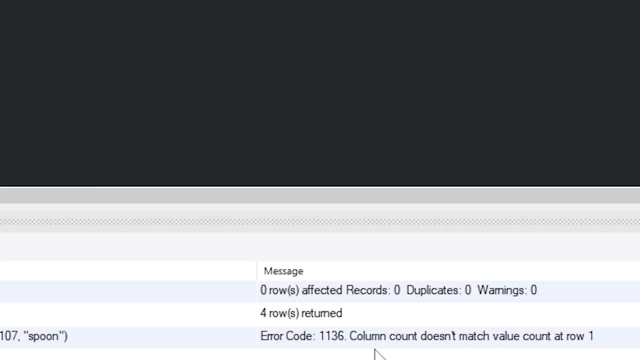 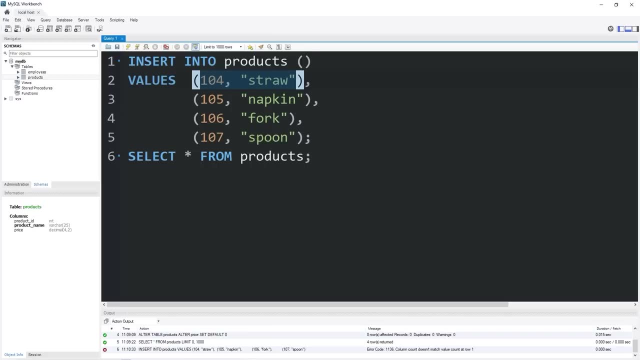 But we are missing one thing, though: When I execute this statement: The column count doesn't match. So when we insert into products, We will list what we are inserting explicitly: The product id And the product name After our table name, Within parentheses type: Product id, Then product name. 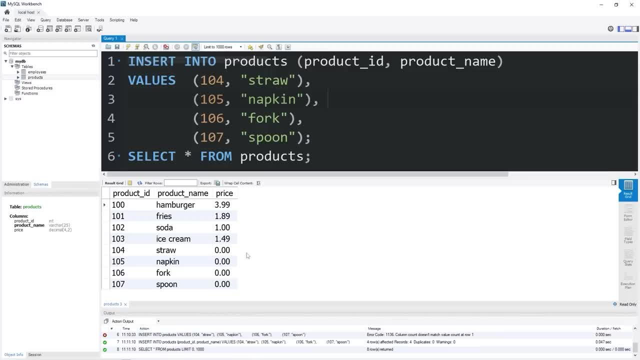 Now this should work. Yeah, and here is our products table After our table inserts. All of the prices were set to 0 And we did not need to explicitly state that this time. If you don't specify a value, You will use whatever the default is. Here is another example. 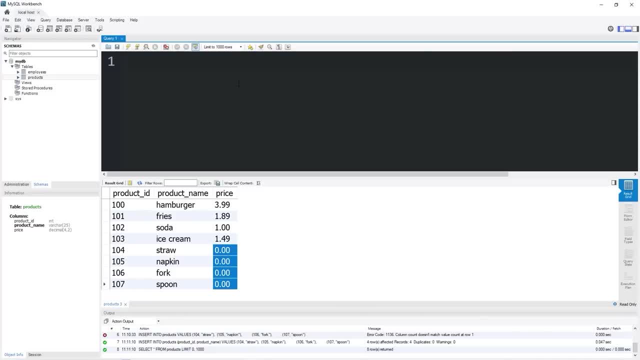 I think you will like this one. Let's say we have a table of transactions. After inserting a new transaction, We will insert a timestamp Of when that transaction took place And that timestamp will be the default Create table Transactions. At the end of this topic, We will delete this table. 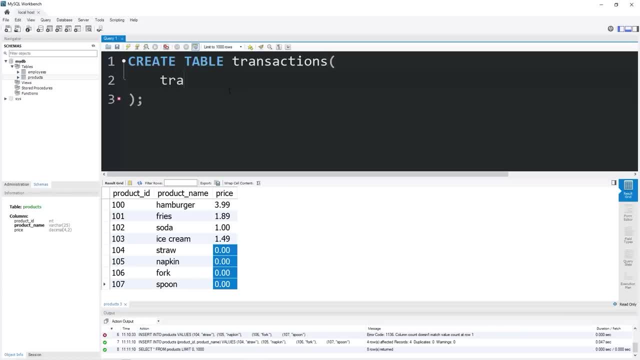 So don't get too attached to it. We will have three columns: Transaction id, Which will be Of the data type integer. A transaction amount, Let's just say amount. The data type will be decimal, Five digits, Precision of two is good. Then a transaction Date: The data type. 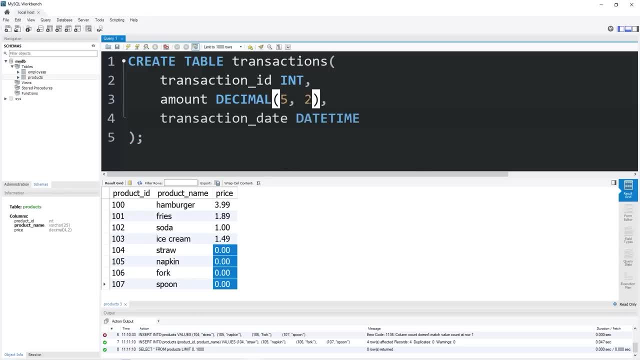 Will be date. Let's make this date time. I'd like to include the time of when this transaction happened. Now for the default constraint. After the date time. Let's add default, Then the now function. We don't need to explicitly add The date and time. That will be done automatically. 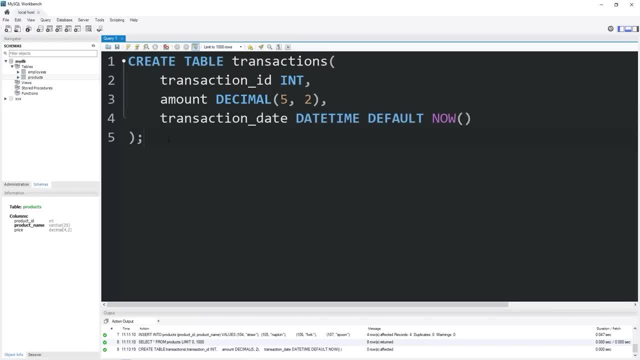 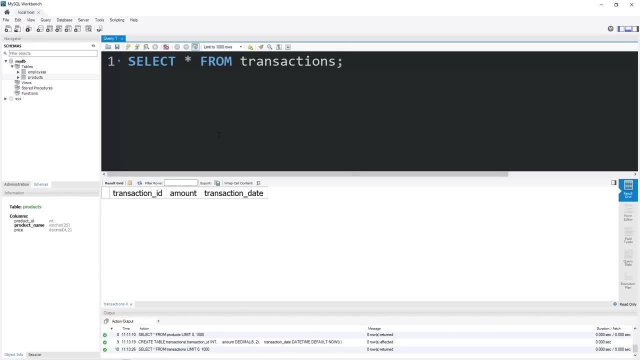 Which is kind of cool. So I'm going to create this table. Let's select all from Transactions. If we are going to insert Some values- At least a transaction id And amount, The transaction date will be included automatically. So let's insert Into Transactions Some values. Let's do one at a time. 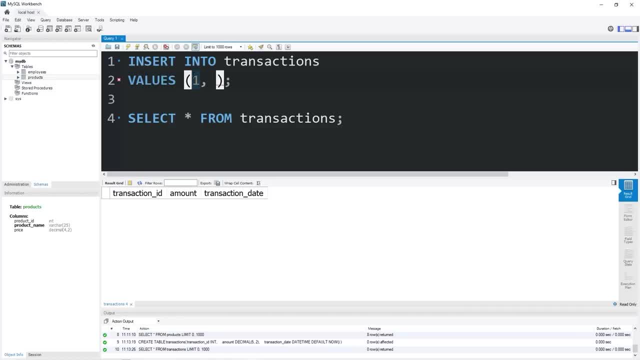 The first transaction of the day Will have a transaction id of one. I suppose A customer came in and bought a hamburger and a soda For a total of $4.99. Then we do need to list The transaction id After our table name. Add Transaction id, Then amount. 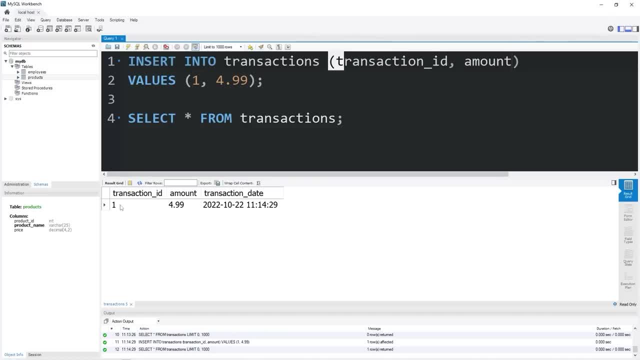 So let's run this. Yeah, cool. So there's our transaction id. This was order number one. The total amount was $4.99 And we do have a time stamp Of when this transaction occurred, So the second order of the day Will be for a total of $2.89. 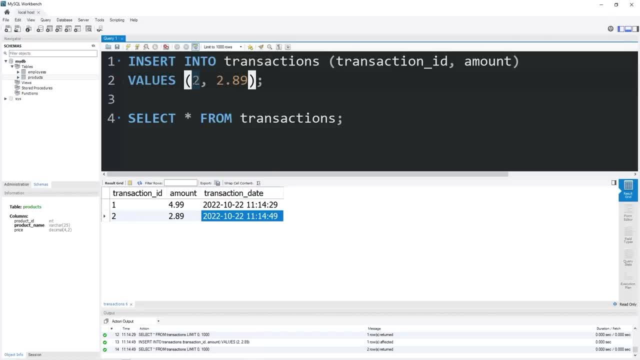 And that happened at this time. Then the third order of the day Will have a total price Of $8.37 Yep. there we are, So we don't need this table anymore. I'm going to drop Table transactions. We will recreate this table in the future, But I'd rather start fresh. 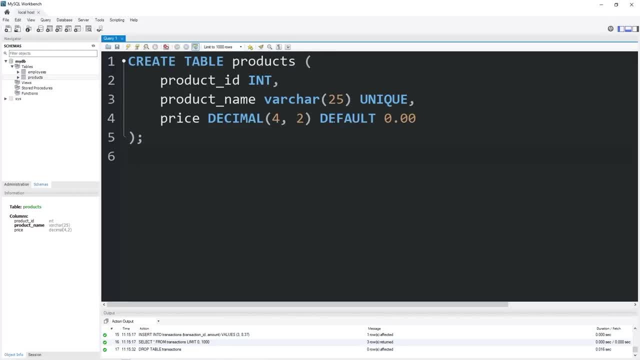 Alright, everybody, That is the default constraint. When you create a table Or alter a table, You can set a default value Of some value you specify. Then whenever you insert a row, A value will be included automatically, Which is pretty useful. But yeah, that is the default constraint In MySQL. 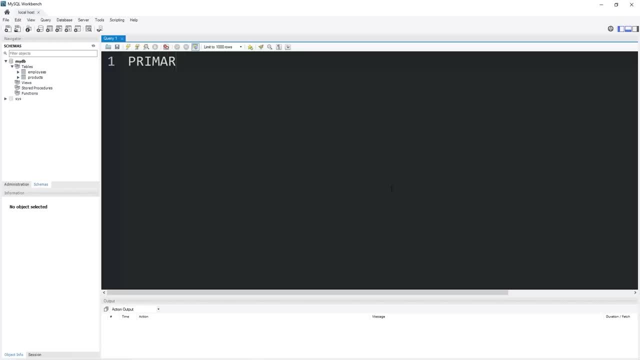 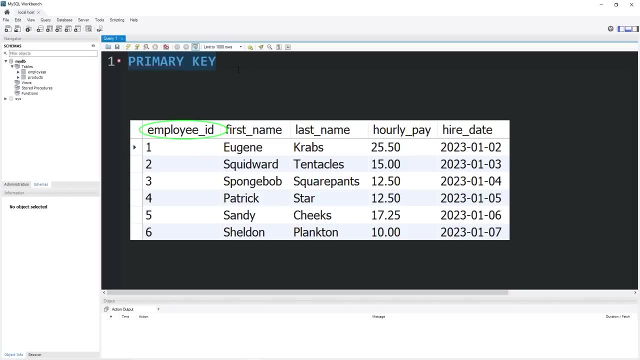 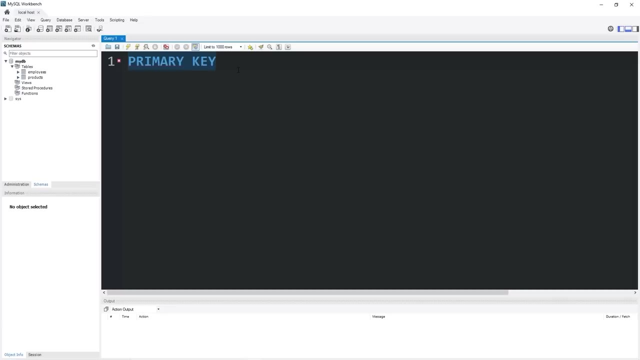 Hey everybody, In this topic I'm going to explain The primary key constraint in MySQL. The primary key constraint Can be applied to a column Where each value in that column Must both be unique and not null. It's typically used as a unique identifier. For example, I live in the United States. 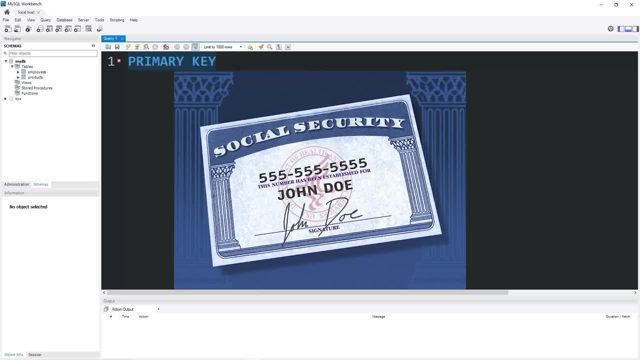 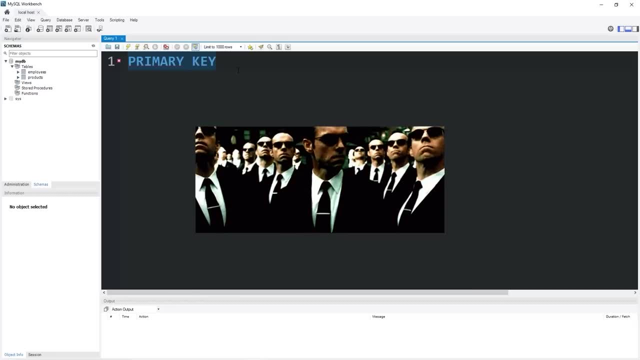 Each citizen within the United States Has a unique social security number. There is a strong possibility That two citizens in the United States Share the same first name and last name- John Smith, for example. If we're trying to find John Smith, Well, which one are we referring to? 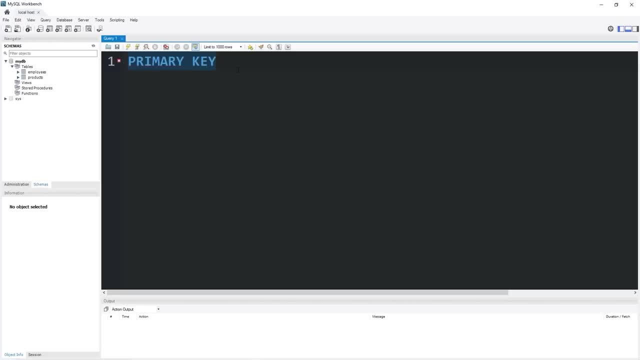 We could instead search for a citizen With a unique social security number. Then we know for sure we have the right person. That's kind of the same concept with the primary key. Also, a table can only have one Primary key constraint. Here's an example. Let's create a temporary table of transactions. 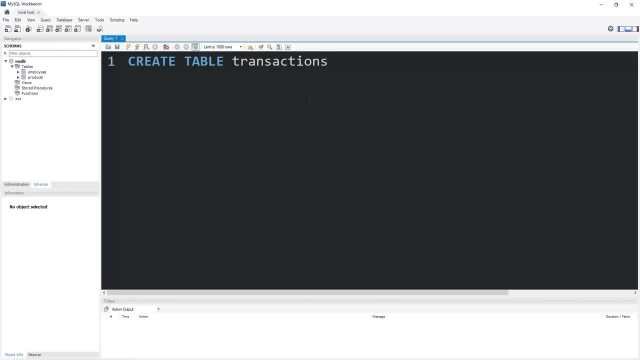 Let's create a temporary table of transactions. Let's create a temporary table of transactions. There will only be two columns: A transaction id, A transaction id. The data type is int. I will set the transaction id To be the primary key To be the primary key. There can be no duplicate transaction ids. 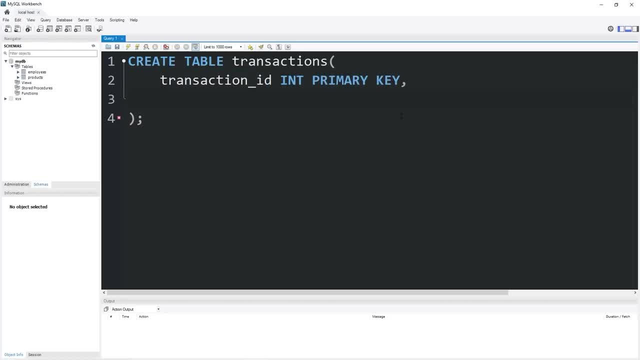 With the same value, And none of them can be null. Then we will also have an amount: How much was each transaction for? The data type will be decimal, Max size of five digits, Precision of two, And that is good enough. Then I will select all from our table. 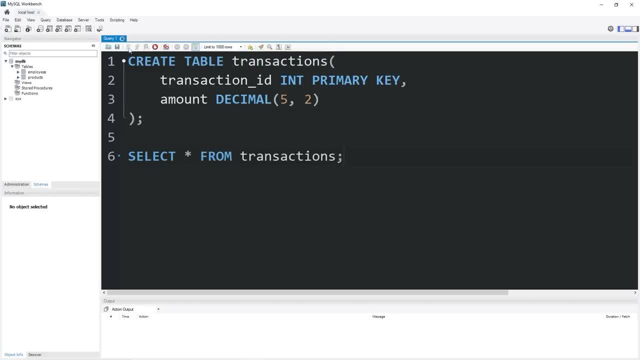 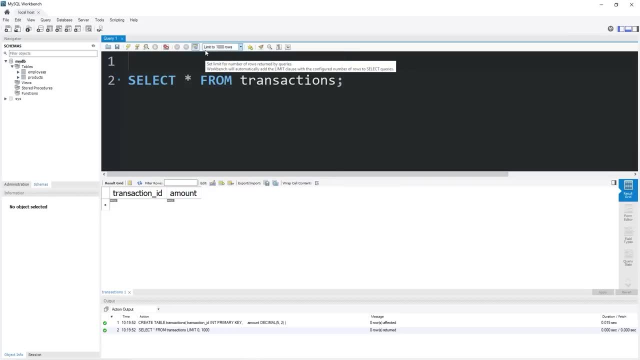 Then I will select all from our table Transactions. Here is our table Now to add a primary key constraint To a table that already exists. This is the syntax Alter table. The name of your table. Add constraint. The name of the constraint Primary key. In parentheses, The column we would like to apply. 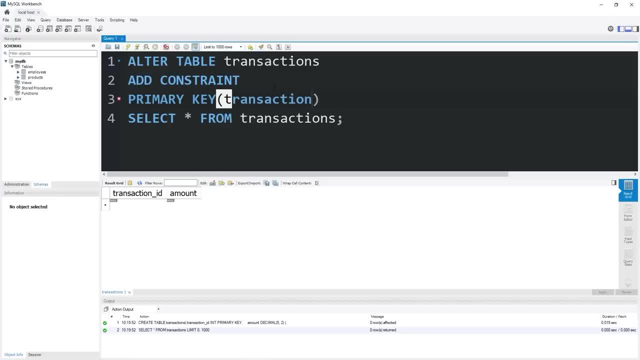 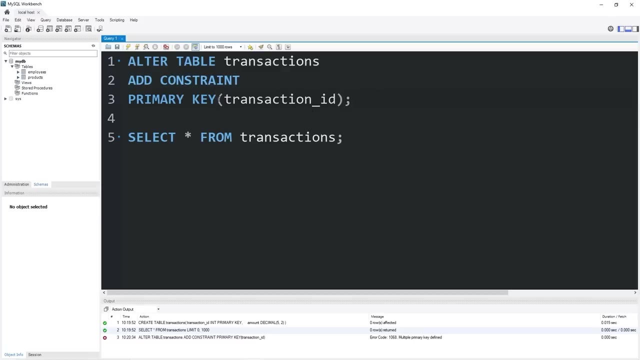 The primary key to Transaction id in this example, Then semicolon. However, we have already applied the primary key constraint To our transaction id column, So this isn't going to work, But that is how you would add a primary key constraint To a table that already exists. Let's test that theory. 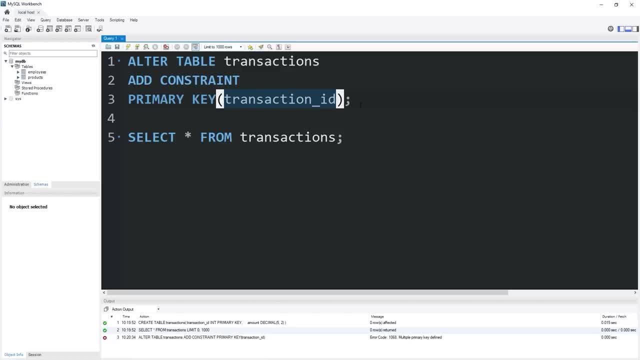 Of that limit of one primary key per table, I will attempt to add a Primary key to our Amount column And it does not appear we can do so. Multiple primary key defined. So, like I said, You can only have one primary key per table And that is typically used. 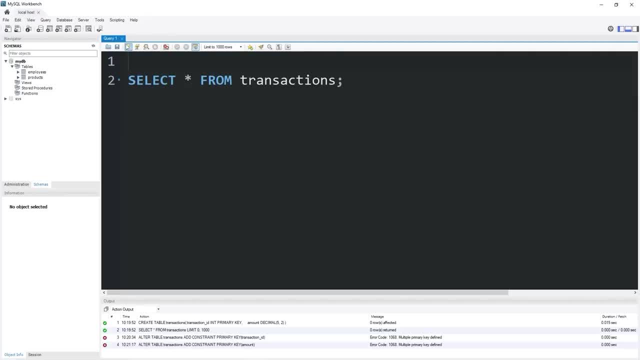 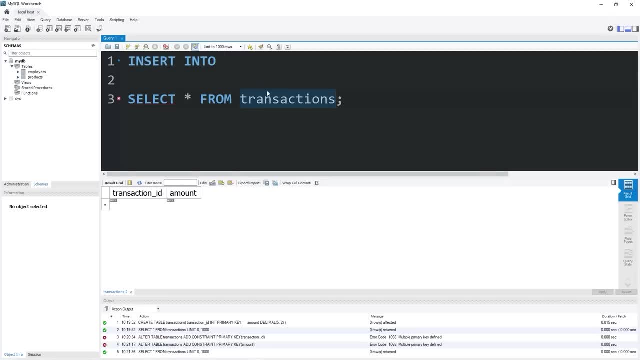 As the identifier. Let's take a look at our transactions. Let's populate this table with a few rows. We will insert Into our table Transactions- Some values. All we need is a transaction id and an amount For our transaction id. I will just make up a number. All transactions will start. 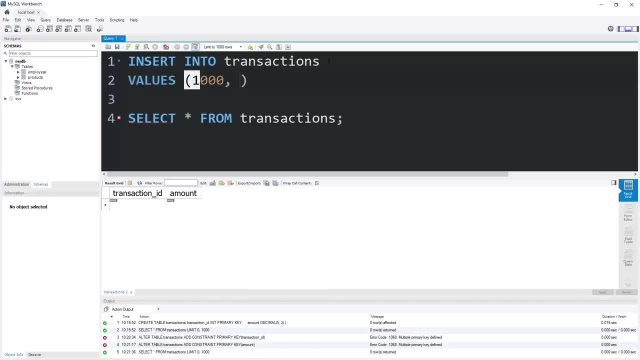 In the thousands. This will be our first transaction. So the amount A customer bought a hamburger and a soda. The total was $4.99. So let's run this. There is our first row. For the second transaction, The transaction id will be 1001. The customer bought fries and a soda. 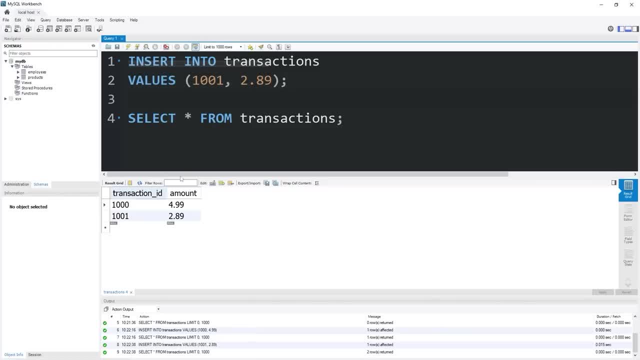 For $2.89, So that appears to have worked As well. The customer buys fries and ice cream For $3.38. Let's test that theory Of each transaction id having to be unique. I will attempt to insert this row With the same transaction id As the previous row. 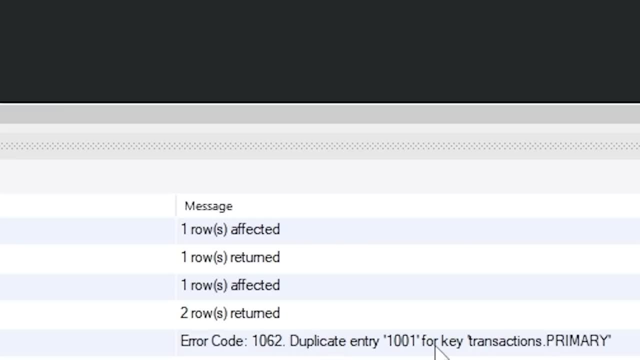 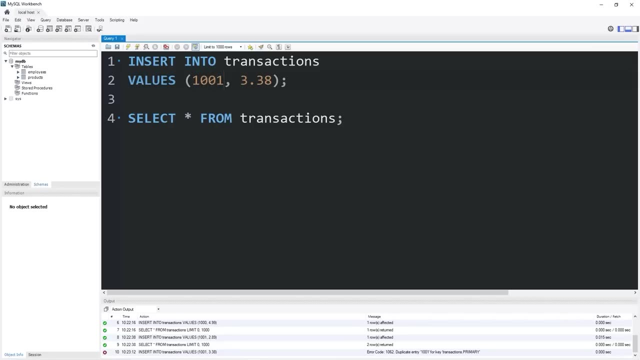 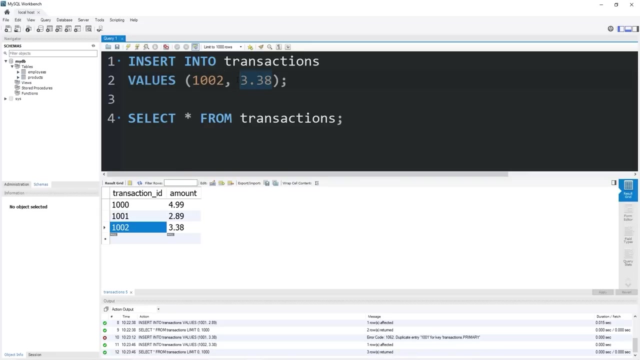 Then let's see what happens. Duplicate entry: 1001 For key transactionsprimary. Yeah, it appears that we cannot have Two rows with the same primary key. They each need to be unique. Let's change the transaction id to 1002. That appears to have worked. Now the next transaction. 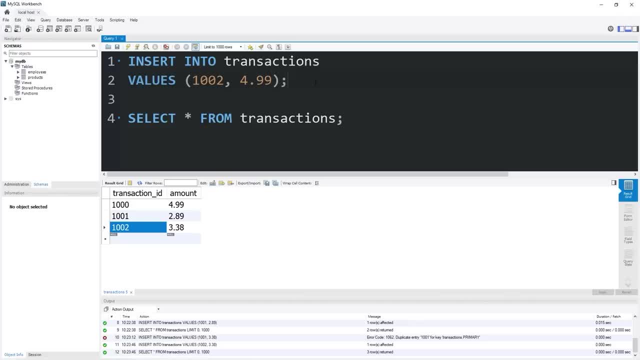 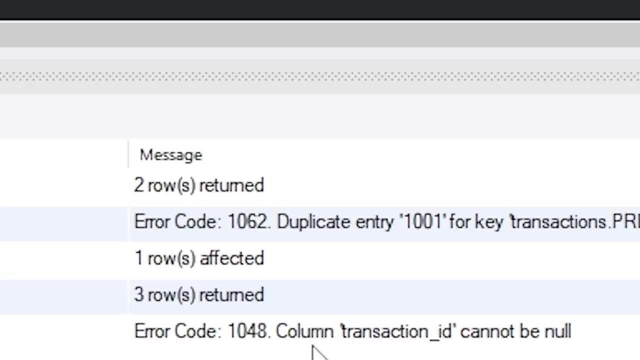 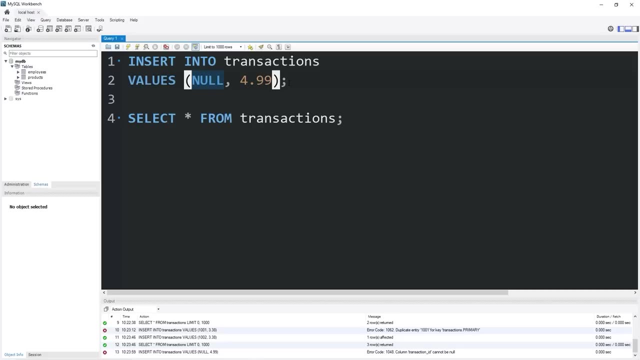 Will be a hamburger and soda For $4.49. I will attempt to set The transaction id to be null, Which we can't do either. Column transaction id cannot be null. Each value That's set as a primary key Can't be null and it needs to be unique. 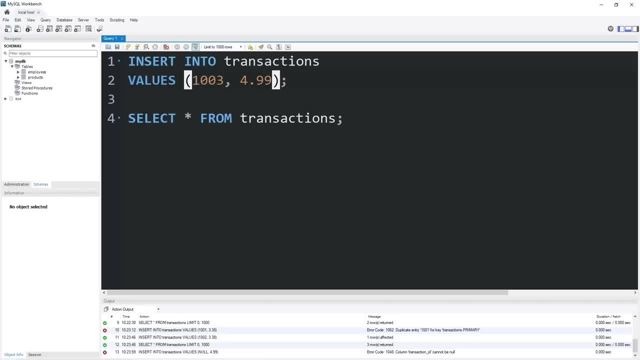 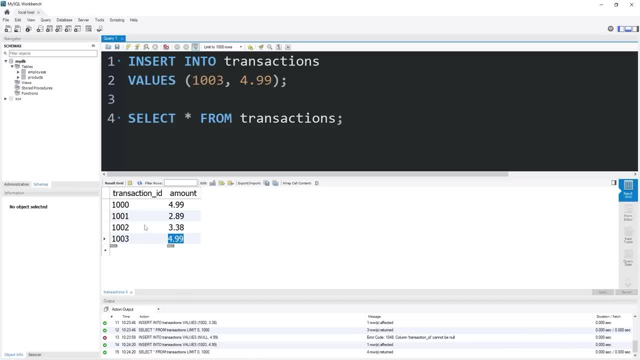 So this transaction will have A transaction id of 1003. Two rows Can share similar data. We have two customers that bought both A hamburger and a soda for the same price, But each transaction is uniquely identified By the transaction id, Which we set as the primary key. 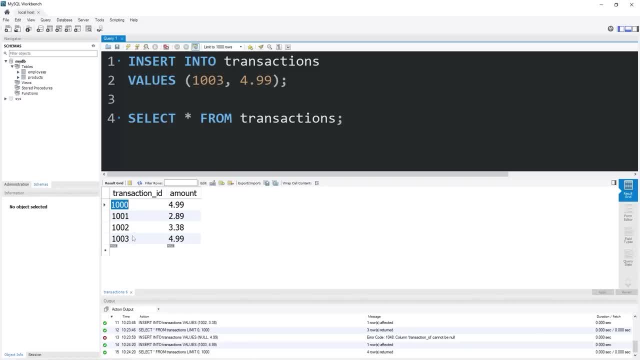 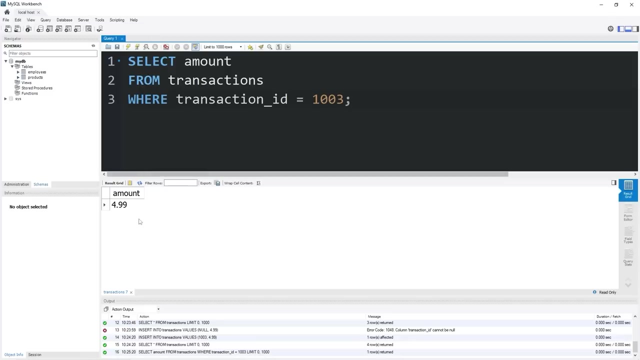 Let's say that somebody comes in to request a refund And they give us a transaction id. Well, we can easily look that up And refund them, whatever the amount was. Select Amount From Transactions Where Transaction id Equals 1003. So we are going to refund The customer $4.99. 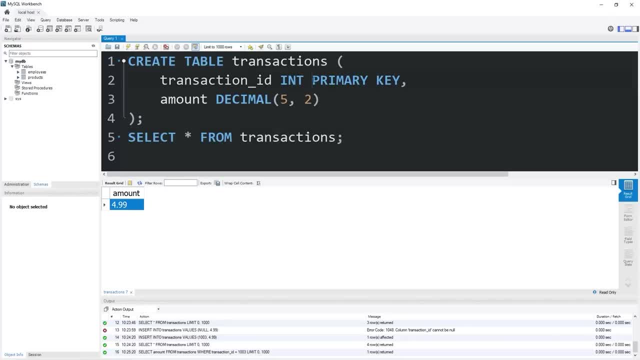 Well, alright then everybody. That is the primary key constraint. It's most commonly used As a unique identifier. You usually want a primary key in every table you make. Each value within a column That is set as the primary key Cannot be null And it needs to be unique. 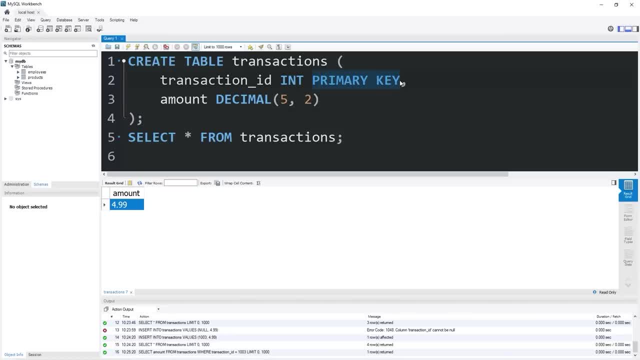 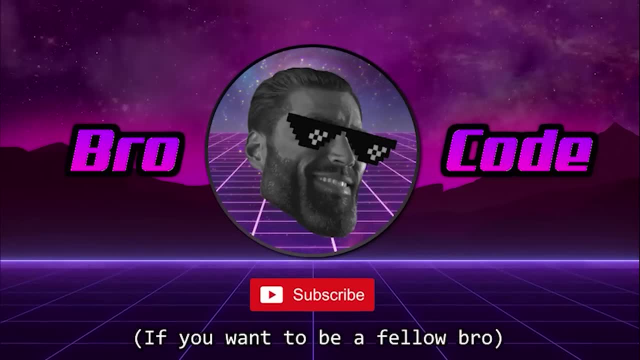 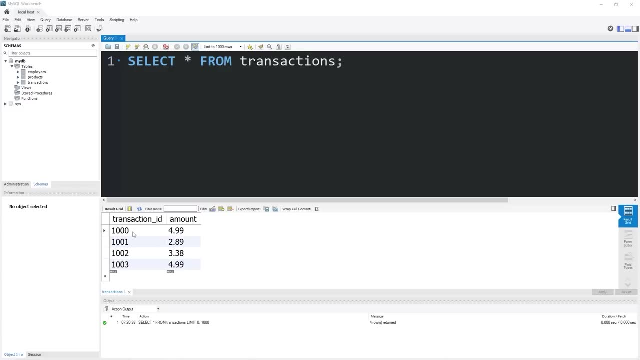 There can only be one primary key per table. Typically it's used as a unique identifier For each row. And, yeah, everybody. that is the primary key constraint In MySQL. Hey everybody, In today's topic I'm going to explain The auto increment attribute In MySQL. The auto increment attribute can be applied to a column. 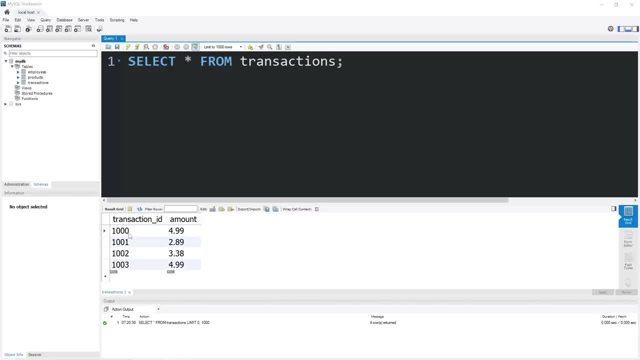 That is set as a key. Whenever we insert a new row, Our primary key can be populated automatically. Then each subsequent row Is auto incremented. I'm going to recreate this table transactions, But first I need to drop it. Drop Table transactions, Then we will recreate this table But apply that auto increment feature. 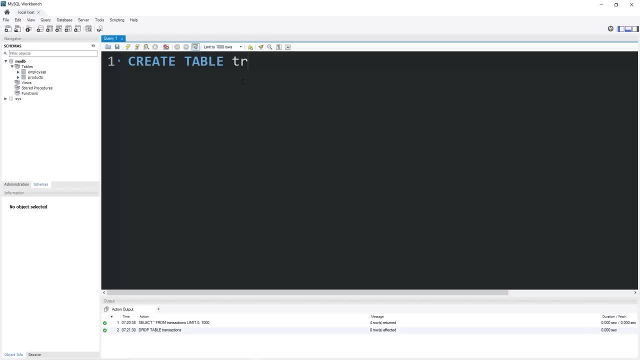 Create Table transactions. There were two columns, A transaction ID- The data type was int- And an amount. The data type was decimal, Five digits Precision of two. The auto increment feature Can only be applied to a column That is set as a key And the transaction ID Will set to be the primary key. 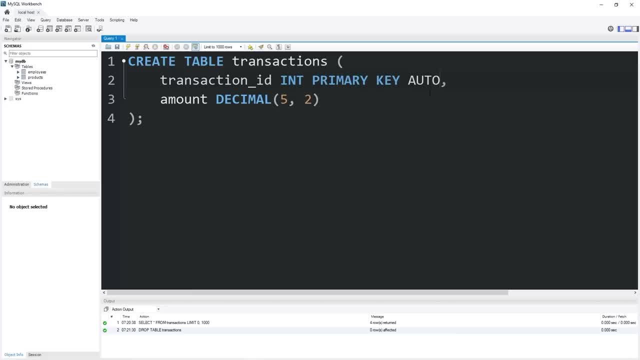 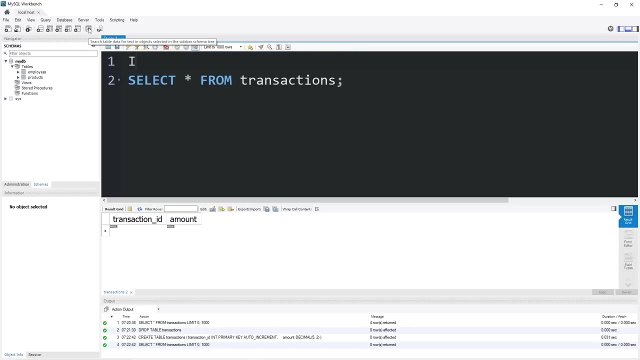 To apply the auto increment feature, Add the keyword Auto increment. Now, by default, The primary key is going to be set to one. So after creating this table, I will select all from Transactions. Okay, we have successfully Created our table. Then I will insert some values. Insert Into Transactions. 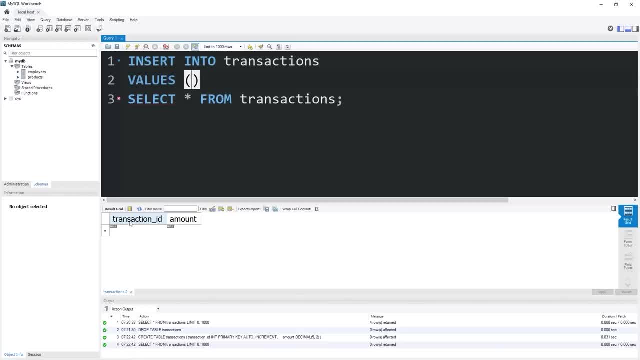 Our values, So we don't need to explicitly insert a Transaction ID. That will be done for us automatically, But we still need an amount. I will insert 499 for the first amount. Since we are not inserting All of the values into a row Explicitly, We would need to specify what column 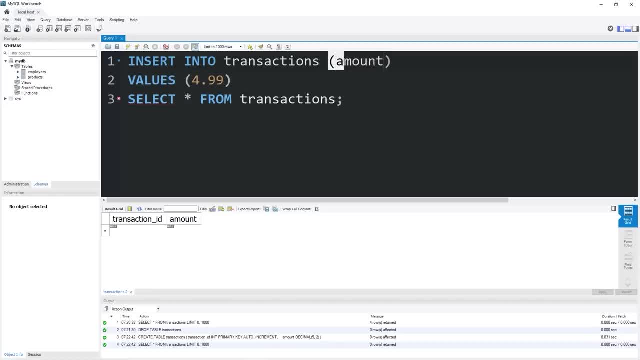 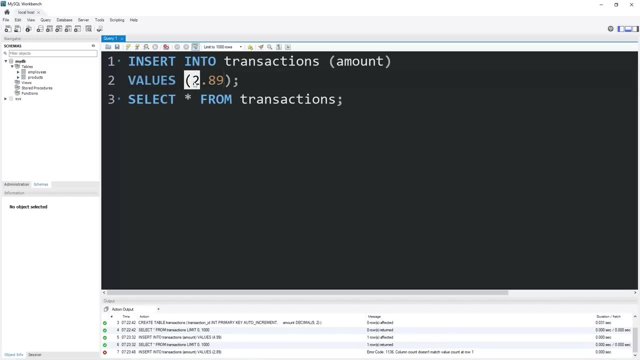 This value is for, That is for the amount. Okay, Let us execute this and take a look. Yeah, so the transaction ID Was set to one, Even though we did not manually insert that value. Let's insert the next amount. So we have 289. Yep. Transaction ID 2 is 289. 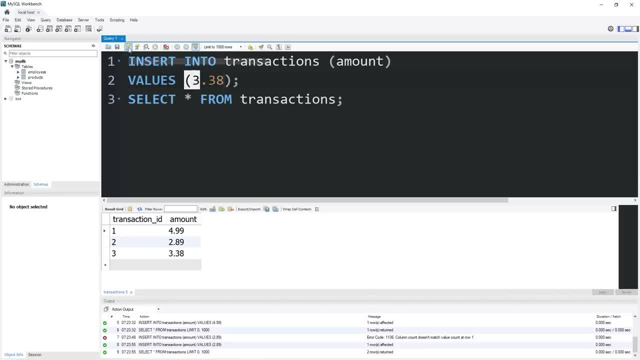 338 Transaction ID 3. 499 Transaction ID 4. We could set our primary key To begin at a different value. To do that, we would type: Alter table- The name of the table, Auto Increment. Let's begin at 1000 Instead of 1, Then I am going to go ahead and drop all the rows. 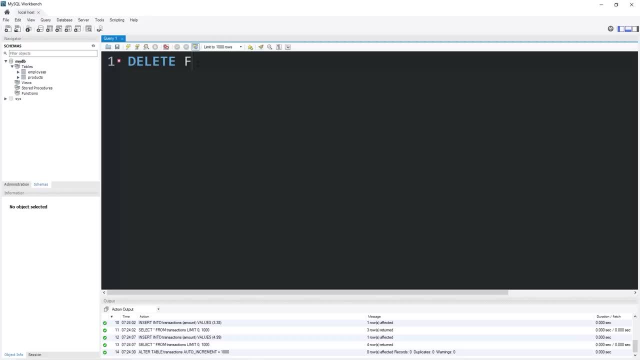 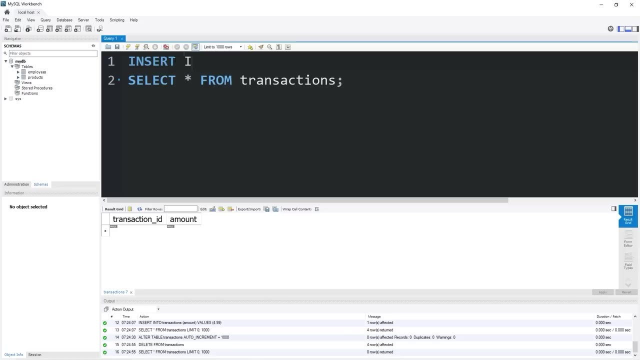 We will start fresh. Delete from Transactions. Select All from Transactions. Okay, then let's insert Those rows again and see what happens. Insert into Transactions Our values. 499 was the first amount. This value is For our amount column. Now this Transaction ID. It begins at 1000. 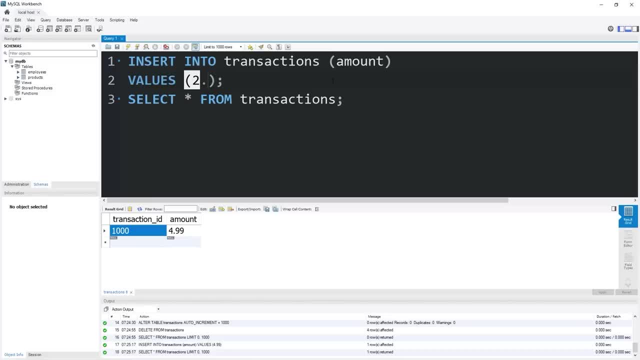 Then it should auto increment. The next value was 289. Our next transaction ID is 3001 338 1002, Then 499, 1003. Alright, everybody, That is the auto increment feature. It's a keyword that can be applied to A column that is set as a key. 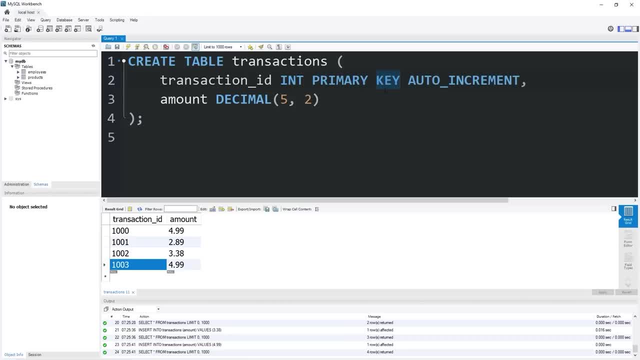 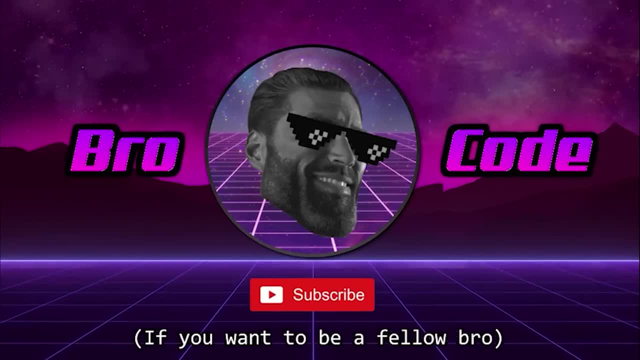 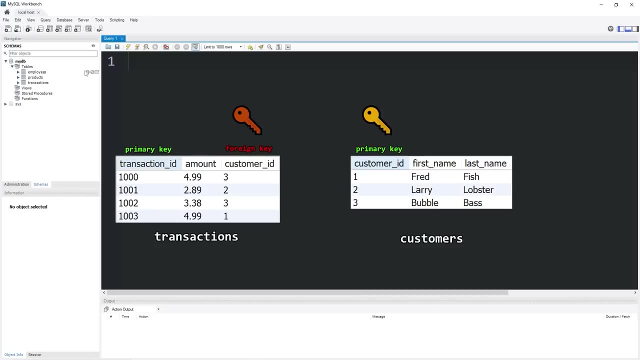 Whenever we insert a new row, Our key will be incremented by 1 For each row that we insert. But yeah, that is auto increment in MySQL. Hey everybody. so in this topic I am going to explain what the foreign key constraint is. A foreign key- Think of it as a primary key. 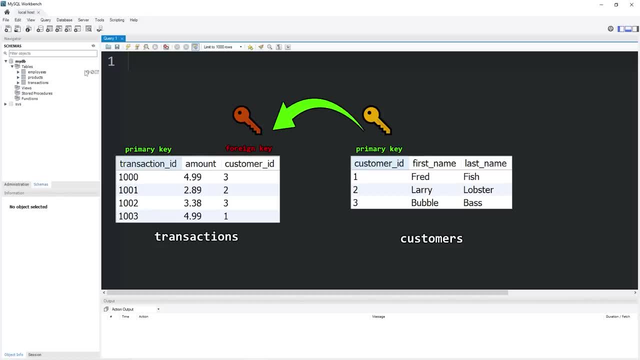 From one table that can be found Within a different table. Using a foreign key, we can establish A link between two tables. There is two primary benefits to this. In my transactions table, If I were to take a look at the customer ID Of who initiated this transaction, I could refer to the customers table. 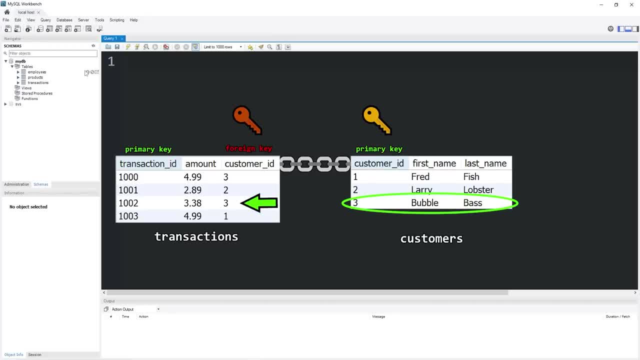 Then find the first And last name of that customer. We can do that when we reach the topic of Joins, but in this video We are going to focus more or less On just creating foreign keys. Another benefit: when you create a foreign key constraint That would create a link between 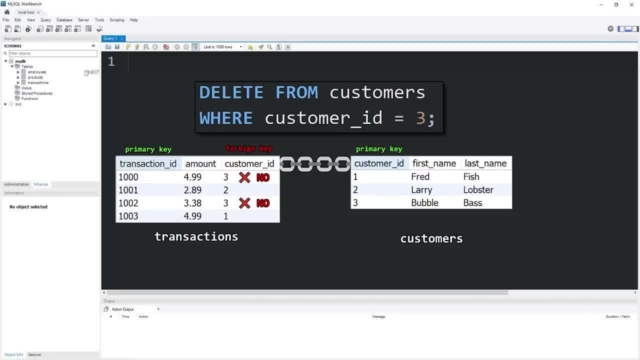 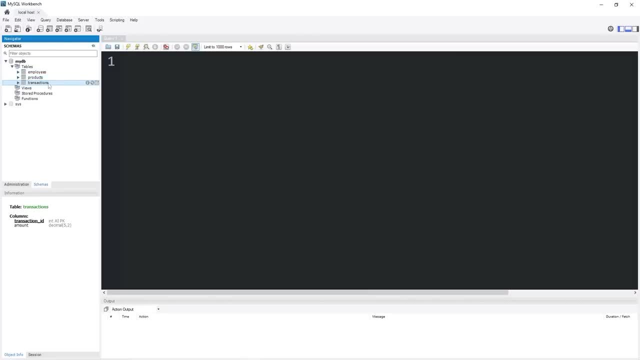 Two tables, which prevents Any actions that would destroy That link between them. So here is an example. I have three tables: Employees, products and transactions. I am going to create a new table, of customers. I am going to create this table and speed it up. Feel free to pause the video if you need to. 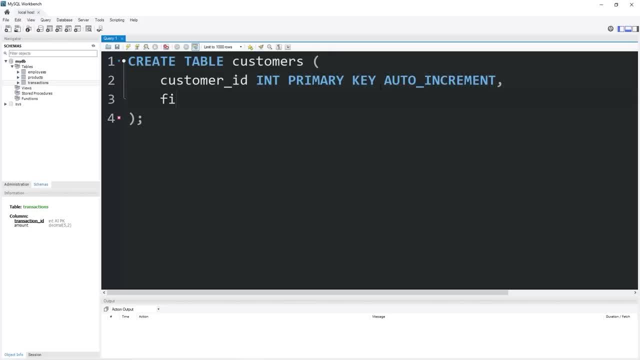 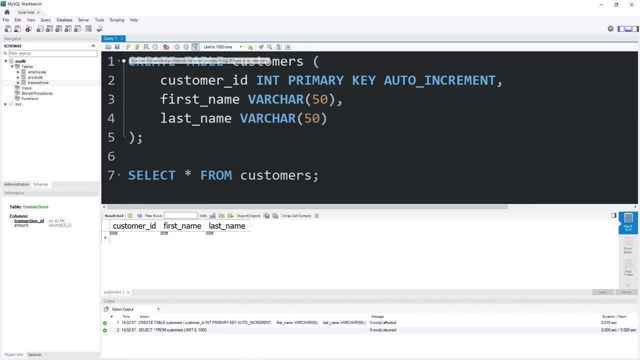 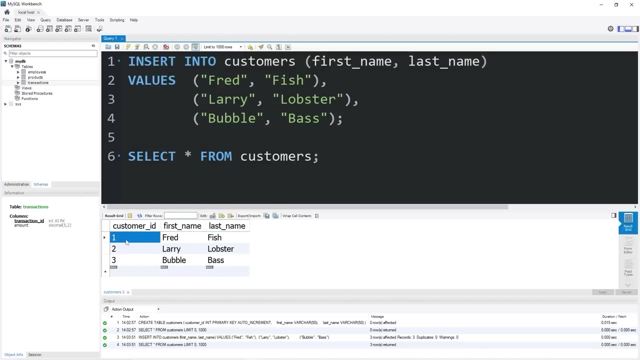 Here is my table. We have a customer ID, Which is the primary key: A first name and a last name. Let's populate our customers table. We have three customers: Fred Fish, Larry Lobster, Bubble Bass. Each has a unique customer ID. We are going to create a link. 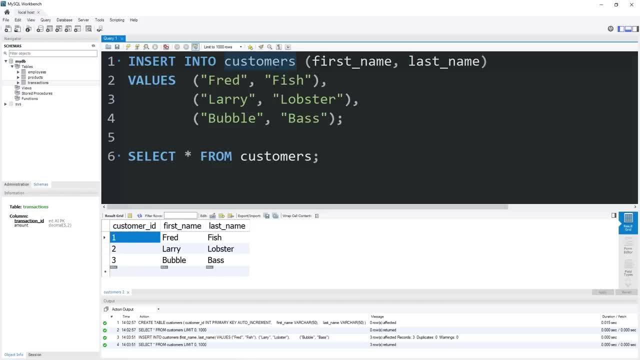 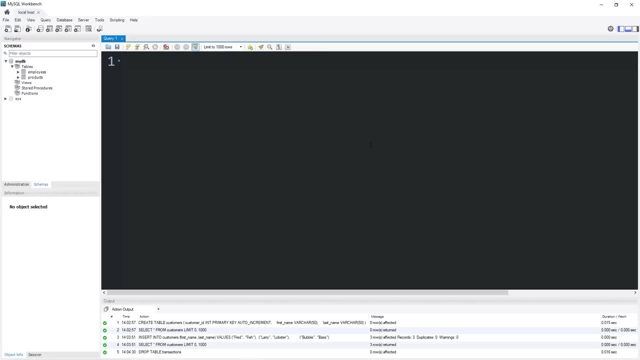 Between our customers table And our transactions table Via our customer ID. I am going to drop our table Transactions. Drop table Transactions. We will recreate this table But apply that foreign key constraint So again, I will speed up the footage. I am going to create a new table And speed it up. 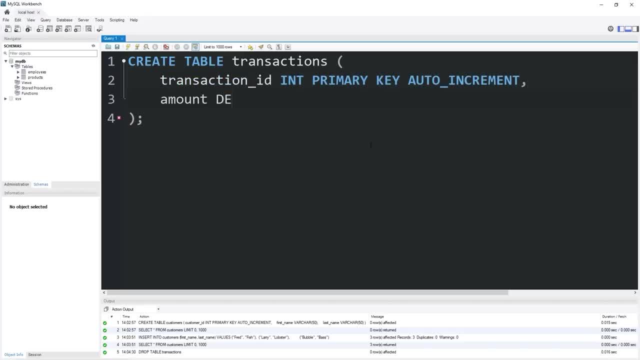 Feel free to pause the video. Feel free to pause the video. Feel free to pause the video. Now, what I am going to do Is create a third column To hold our customer ID, And the data type is int. I would like to add a foreign key constraint To our customer ID column. 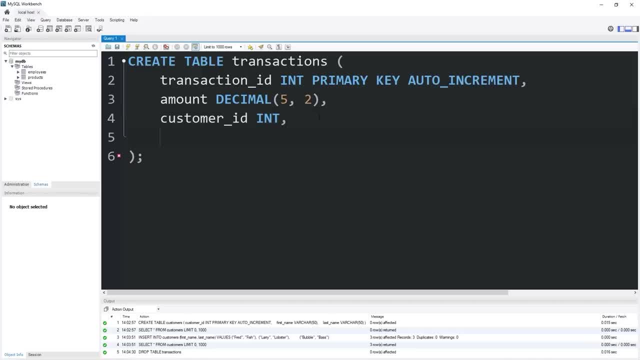 On the next line I will type: Foreign key List: the columns We are applying this foreign key constraint to, Within parentheses Customer ID References: Our second table, The customers table, Customers, Then the column of the primary key, Which was Customer ID. And that is all you need to do. 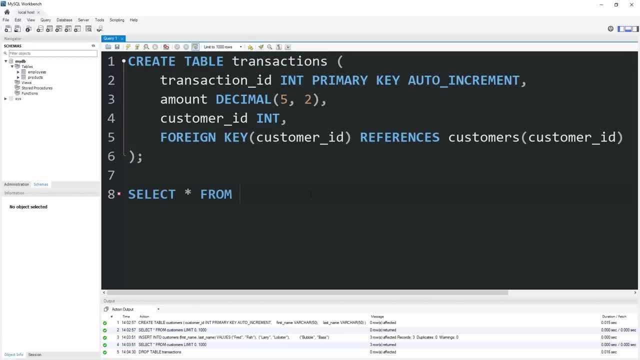 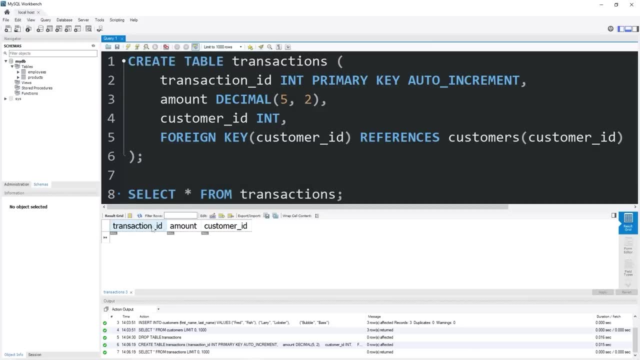 Then I will select all from my table Transactions. Here is our table. We have a transaction ID. This is the primary key- The amount of the transaction, Then the customer ID Of who initiated that transaction. Our customer ID column is the foreign key. It points to the customers table. 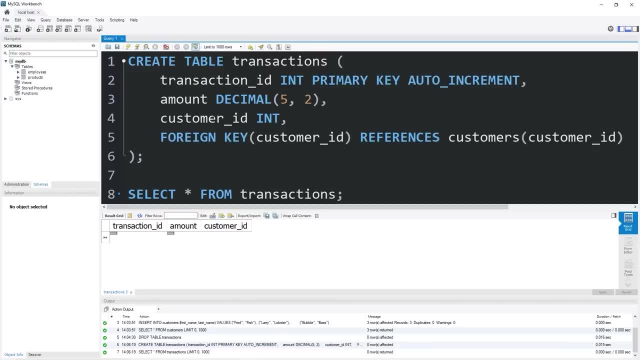 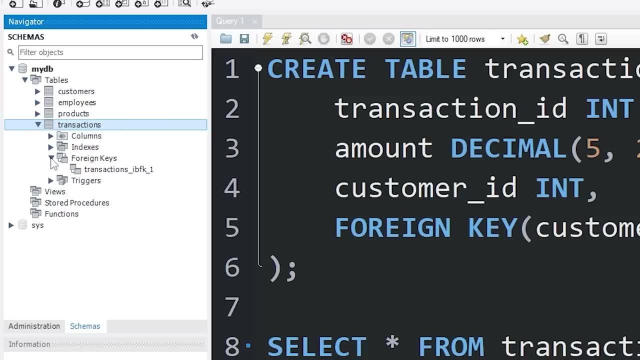 Based on what the customer ID is, We can find the first and last name of that customer. To find any active foreign keys, Go to your table, In this case, transactions Underneath foreign keys. This section will display any foreign keys. We currently have one Transactions underscore IBFK, underscore one. 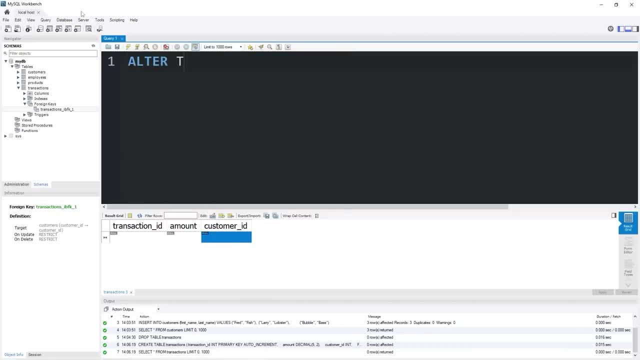 If you need to drop a foreign key, You would type Alter table The name of the table that has the foreign key constraint. That would be Transactions: Drop Foreign key. Then the name of this foreign key: Transactions underscore IBFK. underscore one That foreign key should be gone. You could also give your foreign key. 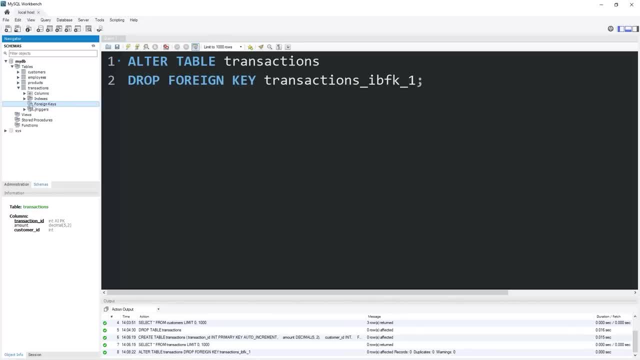 A unique name. Alter table. The name of the table. Add Constraint, Then some unique name. Let's rename that constraint As FK. Underscore: Customer ID- Foreign key. The name of the column: Customer ID References. The name of the second table: Customers. Then the column that has the primary key. 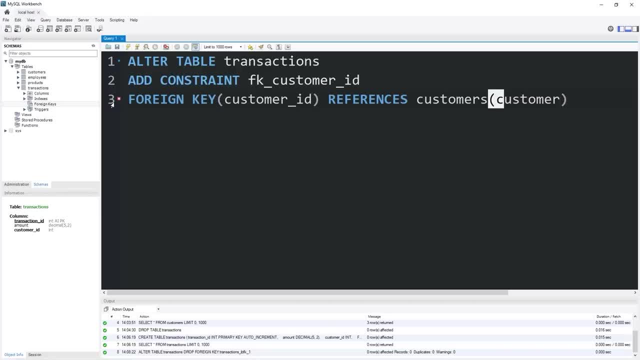 Customer ID. So to apply a foreign key To a table that already exists. This would be the syntax. You don't necessarily need to name the constraint, But if you would like to Just add the constraint, Add that line, Add constraint, Then some unique name. Let's add this foreign key constraint. 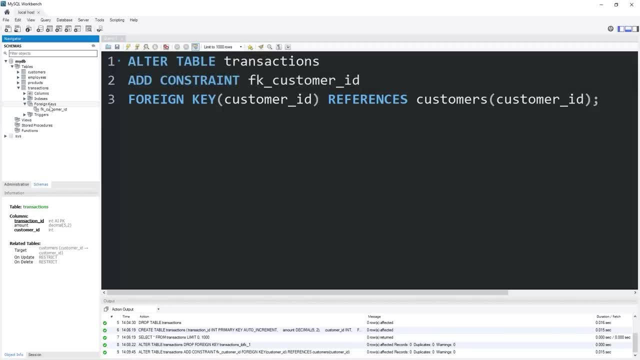 To a table that already exists. It worked If I were to refresh my navigator window. We now have a foreign key And it's the one that we gave a name to: Foreign key: Customer ID. What we're going to do is drop the rows from our transactions table. 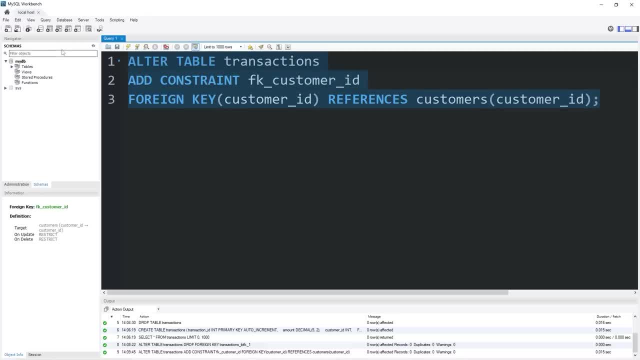 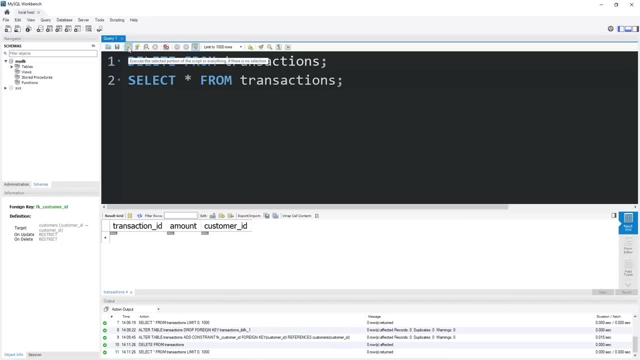 Then reinsert them, But we will add a value for each foreign key To this. Delete from Transactions, Then select all from Transactions. Here we are Ok, so let's insert some new rows. I do want to set auto increment To be 1000, So I'm going to do that before we insert some rows. 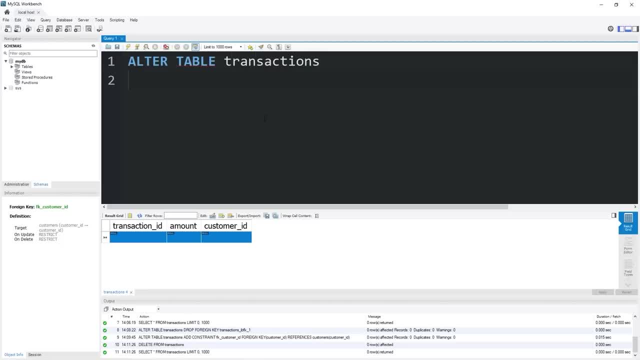 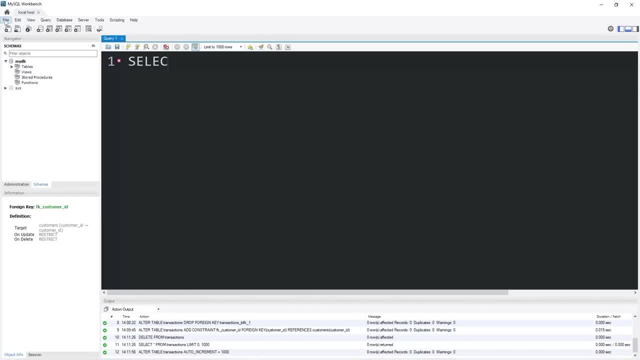 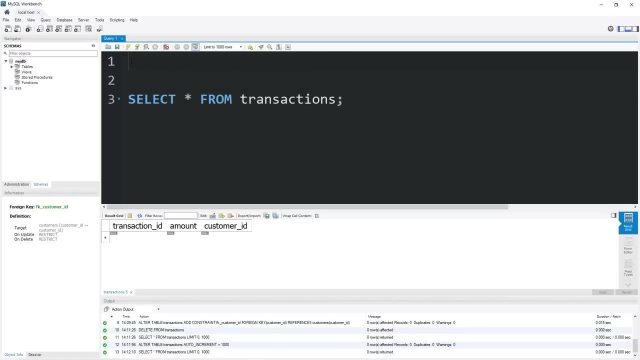 Alter table Transactions. Auto Increment Equals 1000. So let's take a look at Transactions. Then we will insert some new rows, Insert Into Transactions Our values. We had four transactions. We will need An amount And the customer ID Of who initiated the transaction. The first order is for $4.99. Customer number 3 Initiated this transaction. The second order is $2.89. Customer number 2 Initiated that transaction. $3.38- This is also customer 3. They returned back the same day. $4.99. Customer number 1 Initiated that transaction. 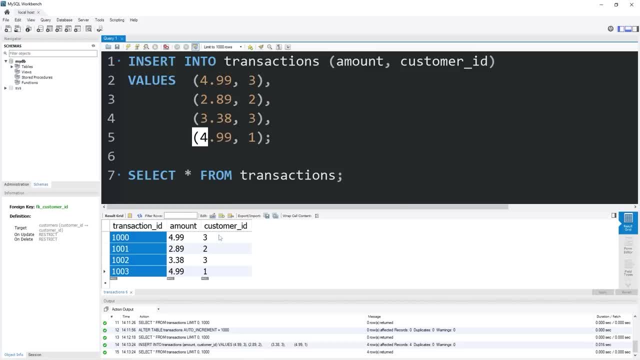 We have our primary key From the transactions table As well as our foreign key. Each of these customer IDs References the customer ID column From the customers table. We won't get to explore that Until we reach the topic on joins. So the other benefit of a foreign key constraint. 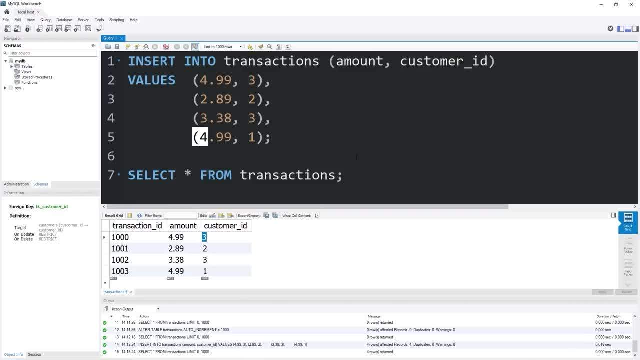 Is that we now have a link between Our transactions table And the customers table. MySQL will prevent any actions That link between them. Unless we explicitly drop that foreign key constraint, I'm going to delete some of our customers. Delete From Customers Where Customer ID Equals 3. We were right. 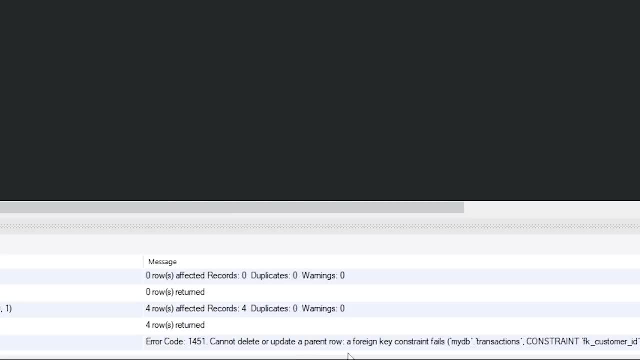 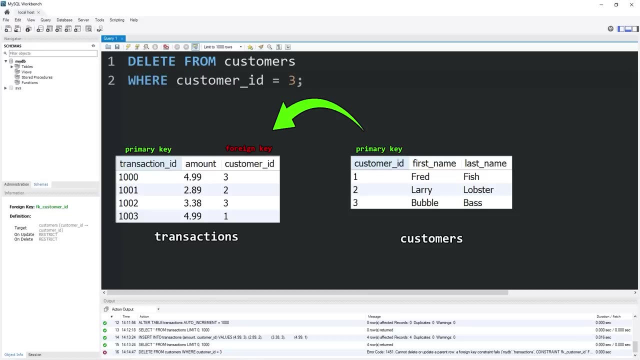 It doesn't appear that we can do so, Cannot delete or update a parent row. A foreign key constraint fails. So, yeah, that's the foreign key constraint. It's a primary key From one table That's found also within a different table, But when we're working with that different table, 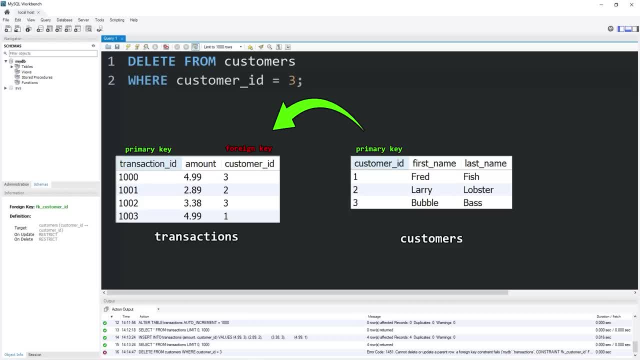 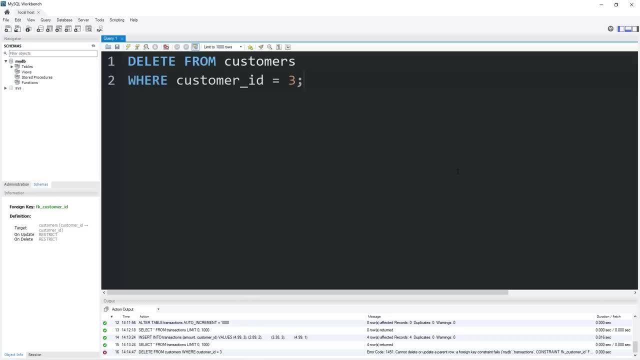 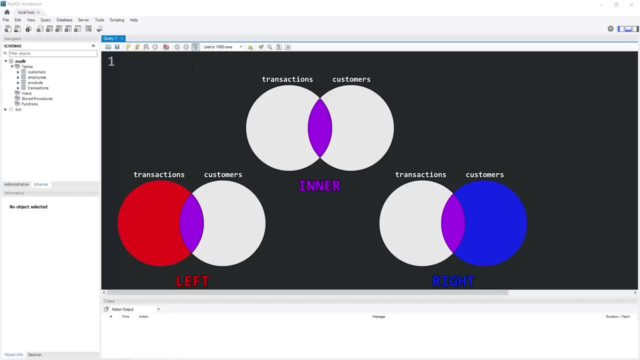 We would refer to that key As a foreign key. We'll have more practice with this when we reach the topic On joins. But yeah, that is the foreign key constraint In MySQL. Hey everybody, Welcome back again. In today's video I'm going to be explaining joins in MySQL. 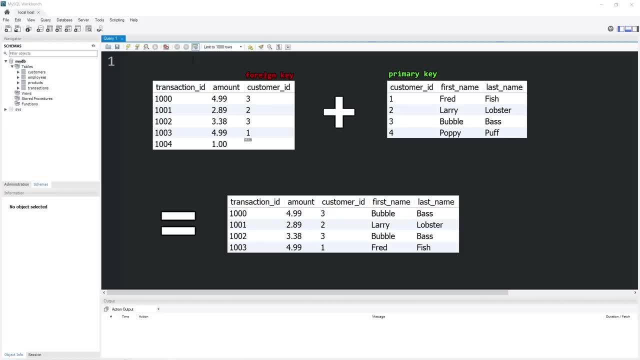 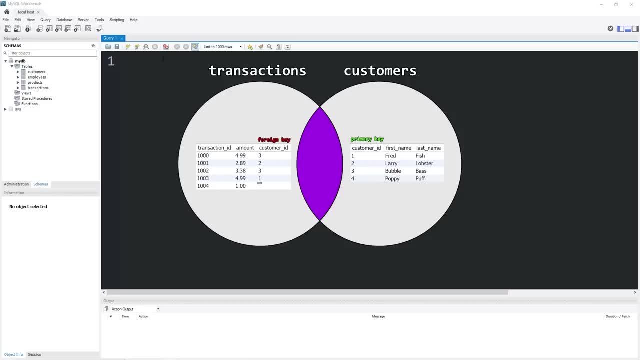 A join is a clause That is used to combine rows With two or more tables Based on a related column between them, Such as a foreign key. Here's an example: I have two tables, A table of transactions And a table of customers. Think of these two tables as a Venn diagram. 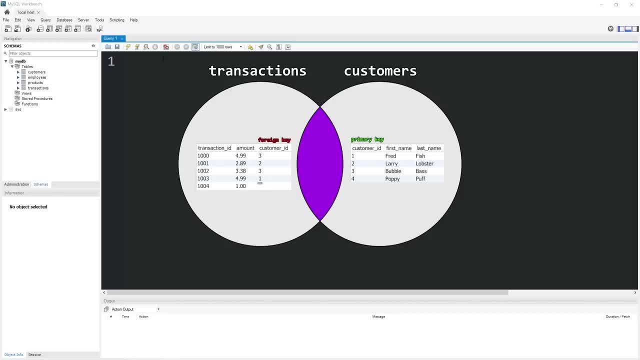 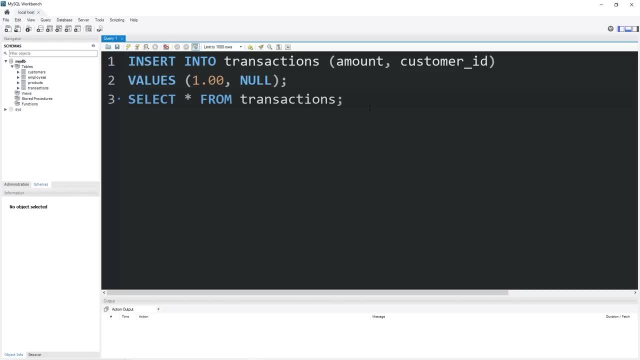 Transactions will be the table on the left. Customers will be the table on the right. Whatever data they have in common Is the middle part of our Venn diagram. For my demonstration to make more sense, I will need to add a few extra rows. Feel free to pause the video if you need to catch up. 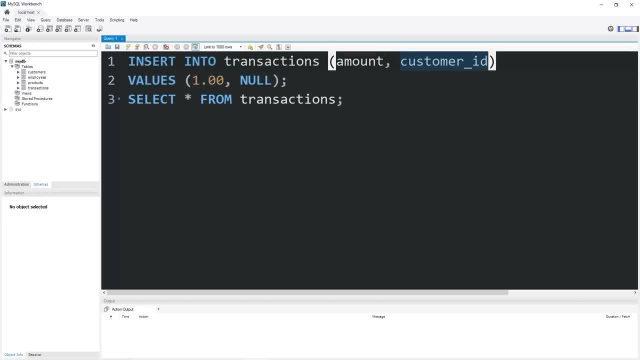 Here's a scenario: Suppose that somebody comes in Pays for a soda with cash. Well, we wouldn't have a customer ID right. If a customer instead Paid with a credit card, We could track who that customer was. There may be a customer ID Who initiated that credit card charge. 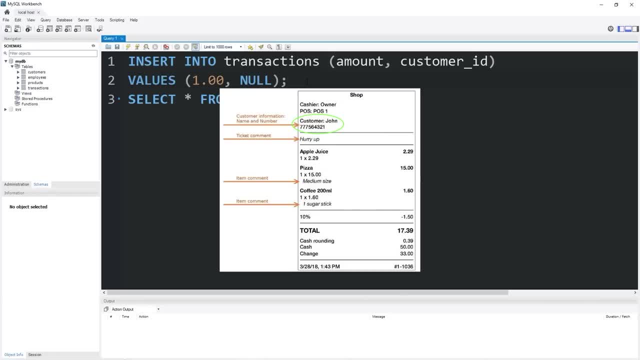 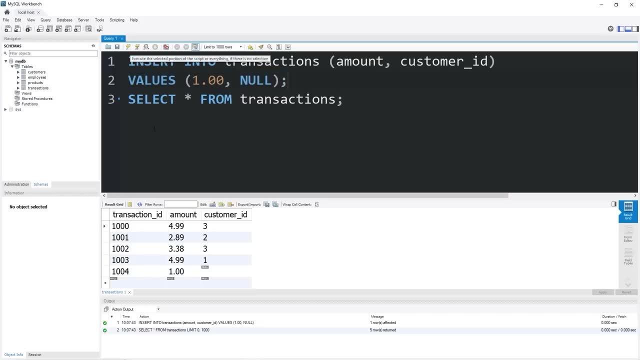 I'm going to insert this row And here's our new transactions table. I'm going to insert this row And here's our new transactions table. I'm going to insert this row And here's our new transactions table. Not all rows have a customer ID. Not all rows have a customer ID. 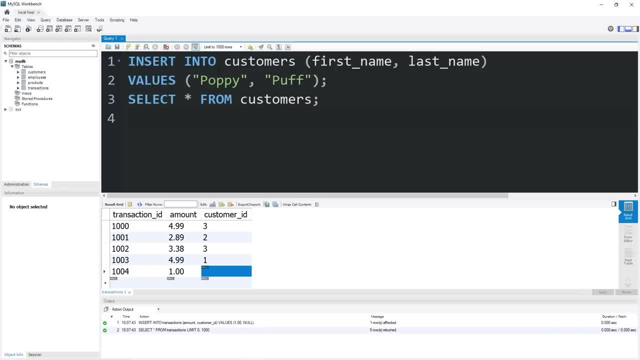 Then let's add one more customer. Insert into customers. Insert into customers: First name. last name will be PoppyPuff. Let's select all of our customers Now. not all transactions Have a customer ID And not all customers Have ever initiated a transaction. They could be registered as a customer. 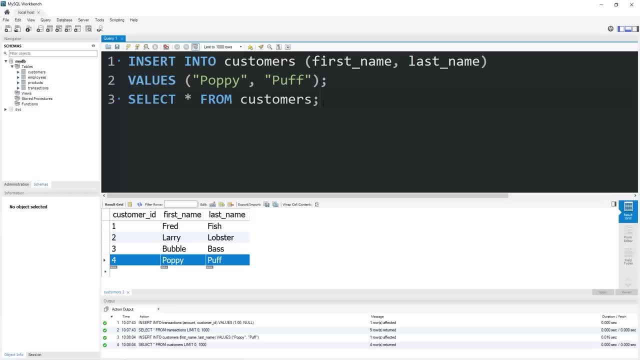 But they have never actually bought anything yet. But they have never actually bought anything yet. Let's take a look at what data These two tables have in common. We'll discuss inner joins, left joins and right joins. We'll discuss inner joins, left joins and right joins. 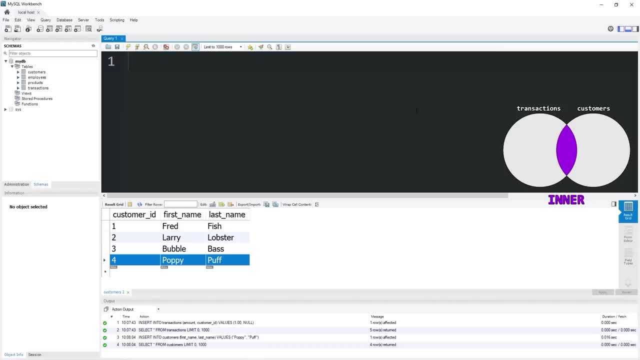 Let's begin with an inner join. To create an inner join between these two tables, You would type: Select all. from Which table would you like to be on the left? Think of that Venn diagram. Our transactions table will be on the left. Our transactions table will be on the left. 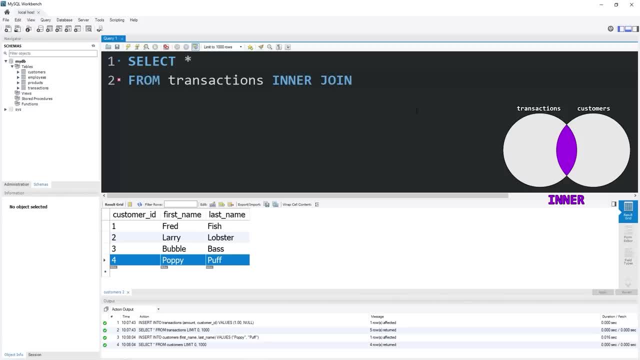 From transactions: Inner join Whatever table you would like to be on, the right, In this case customers On. We're going to join these two tables together By the foreign key from transactions. We'll take Transactions. dot The name of the foreign key column, Which was customer ID. 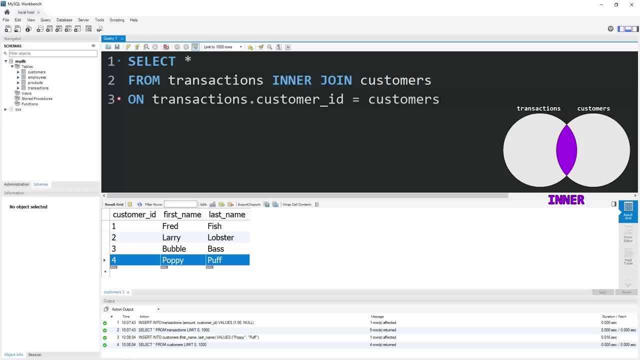 Which was customer ID Equals the table on the right. Dot the name of the primary key column, Dot the name of the primary key column Which was customer ID. Then we will execute this statement And here's our new table. We have created an inner join From these two tables. 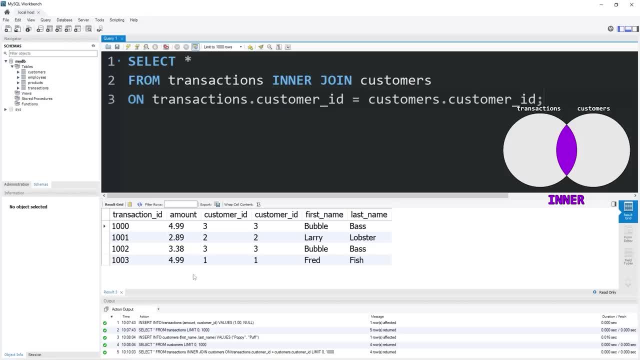 Based solely on what they have in common. If you remember, we don't have that row For that transaction for one dollar That doesn't have a customer ID, As well as our customer Poppy Puff. There's no row for her in this table. What we're telling MySQL is to select. 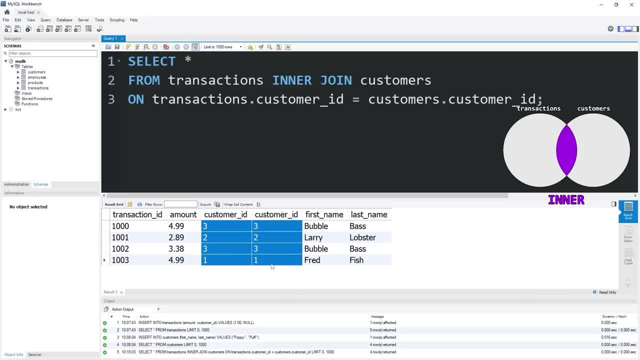 All rows from these two tables That have matching customer IDs. That have matching customer IDs. So that's why some data was excluded. One thing you could do with a join- This applies to left joins And right joins as well- You don't necessarily need to display Every single column from both tables. 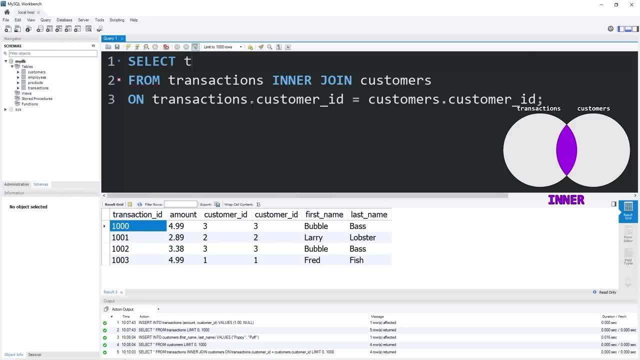 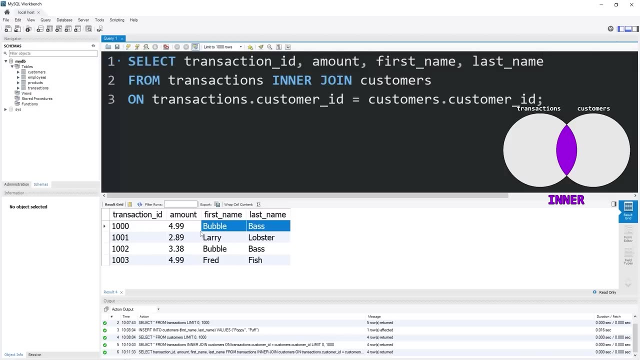 You can select specific columns. Let's select our Transaction ID, The amount, The first name, Then the last name. This would make it a lot easier To find the first and last name Of who initiated a transaction At a given time. So that is an inner join. Join together any matching rows. 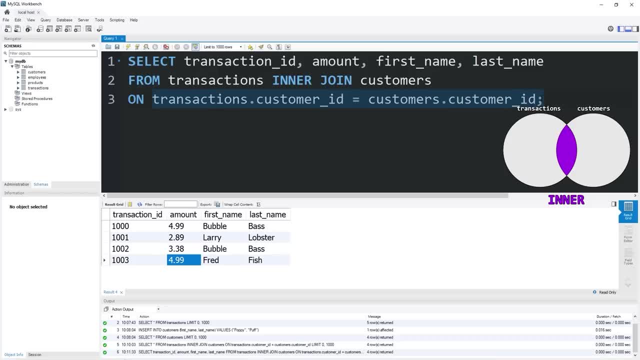 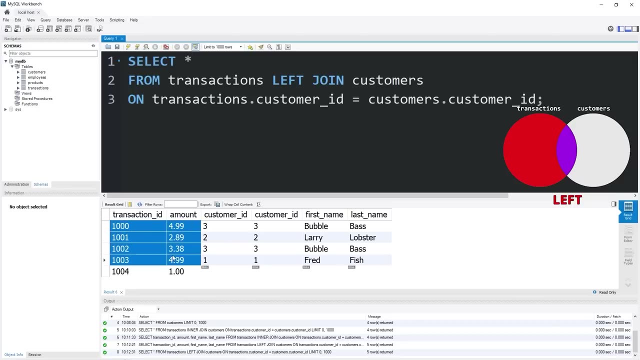 Based on some link. In this case, we're joining these two tables together By their customer ID. Now, with the left join, We are going to display everything From the table on the left, But let's select all. With the left join, We will display everything From the table on the left. 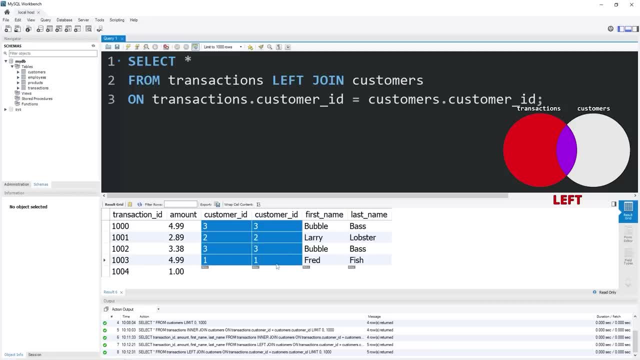 Our transactions. However, if there is a matching customer ID, Pull in any relevant data From the table on the right. Even though there is no customer ID With this latest row, We're still going to display it With the left: join, But there is no data to pull in. 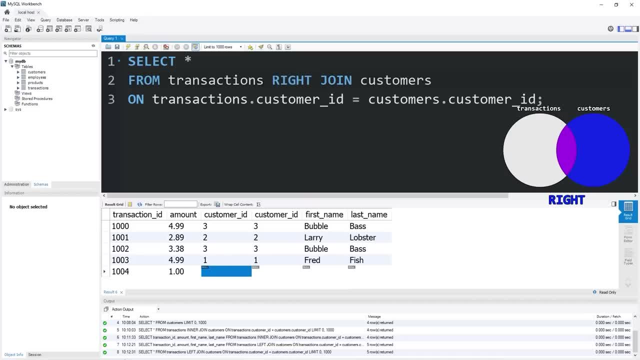 From the right table Because there is no registered customer ID With the right join. We will display the entire table on the right. If there is any matches, We will pull in any matching rows. From the left, We are displaying all of our customers. If any of these customers 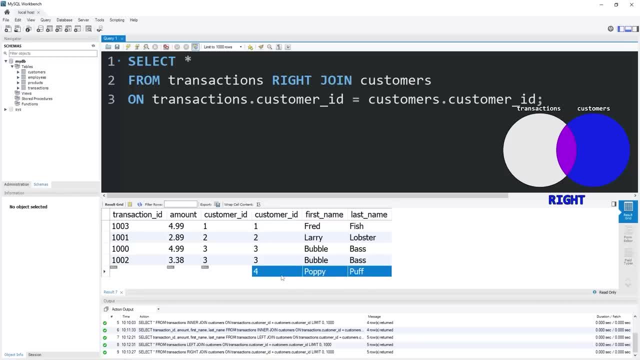 Do not exist, We will have them in the table, But no relevant transactions. She never initiated one. So yeah, everybody, those are joins. A join is used to combine rows From 2 or more tables Based on a related column between them, Such as a foreign key Like customer ID. 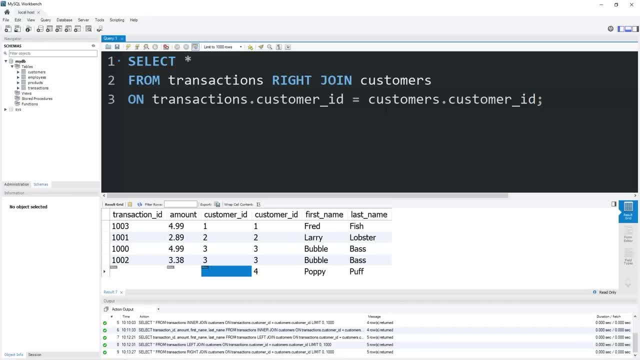 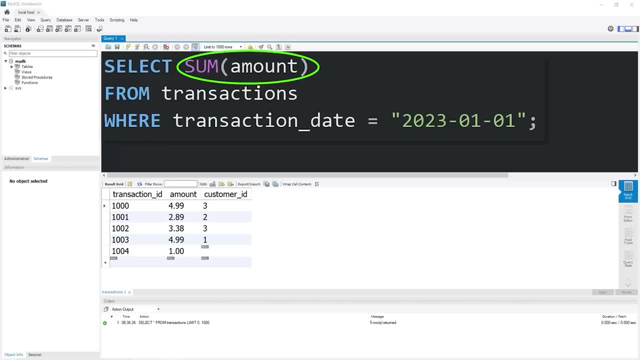 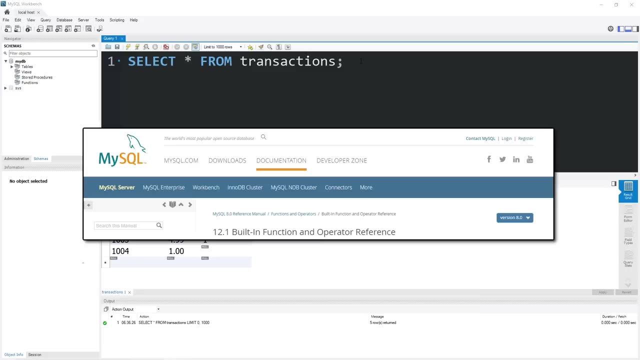 And that is a quick introduction To joins in mysql. Hello again everyone. Today I will be explaining functions. A function is a stored program that you can pass parameters into to return a value. If you look on MySQL's main website, there is a huge, comprehensive list of functions. 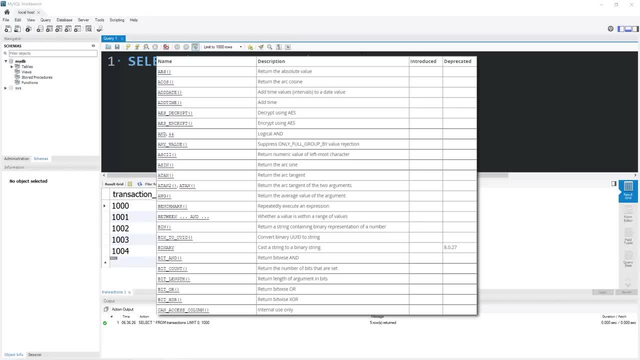 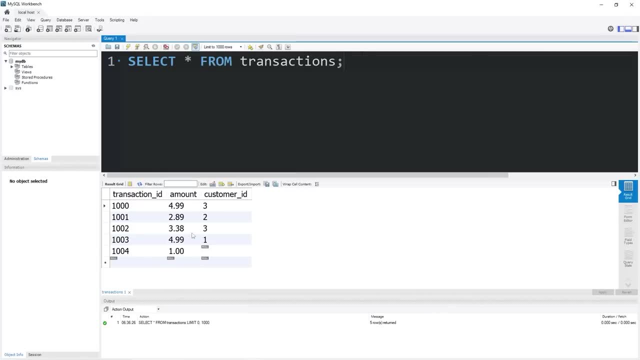 In this video I'll only be showing you a few of the more useful ones for beginners. But just so you know, there's a lot of functions out there that do all sorts of things. What if I would like to count how many transactions took place on a certain date? 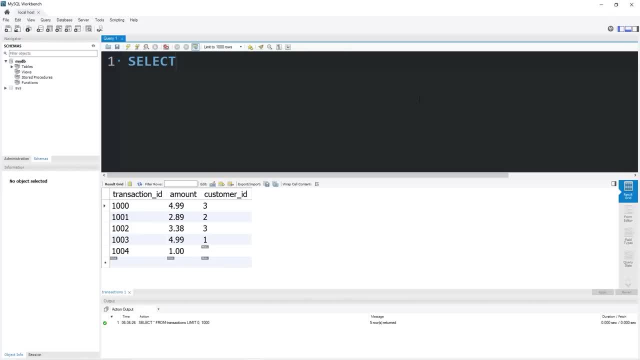 To do that we can use the count function: Select count parentheses. Within my set of parentheses I can place a column, then calculate how many rows are within that column. Let's calculate amount. We will count how many rows are within the column amount. 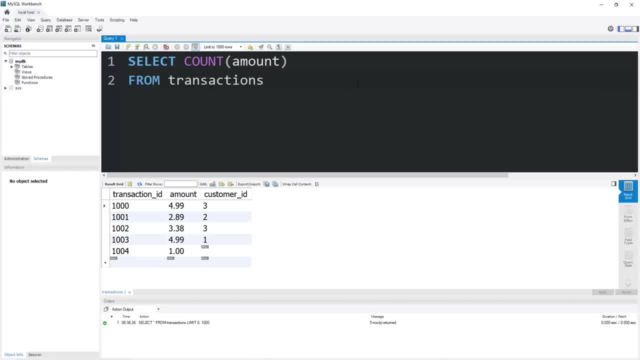 Then we will need a table From our table transactions, So you could add a where clause too, like where transaction date is on a certain date. But I want to keep this video as simple as possible. This function will return all of the rows within this column. 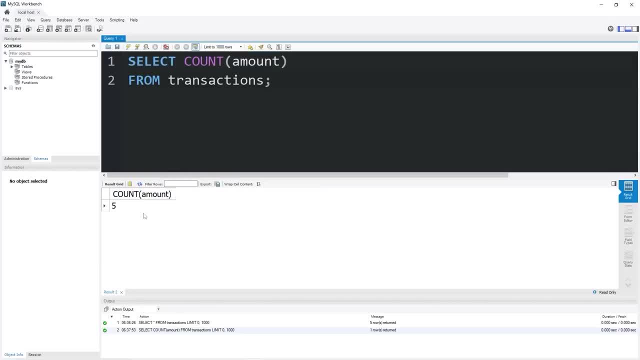 Amount, Which is 5.. We have 5 transactions within this table. Now this column header is kind of ugly. The column name is count, the amount column. You could give a column an alias by adding as then some nickname, Let's say count. 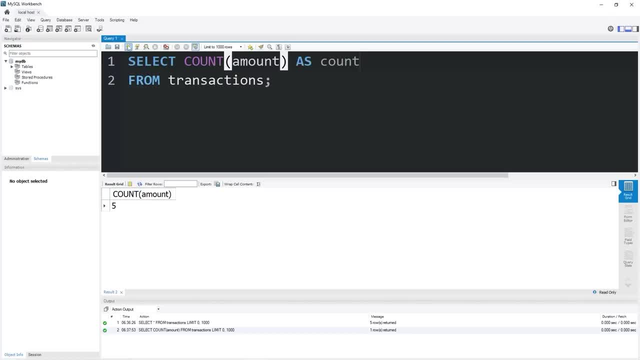 It's not necessary, but if you want to make the column header look pretty or rename it as something, you could do, that Count 5.. We could even rename this column as todayscom Transactions. That works too. Do whatever you want to do. 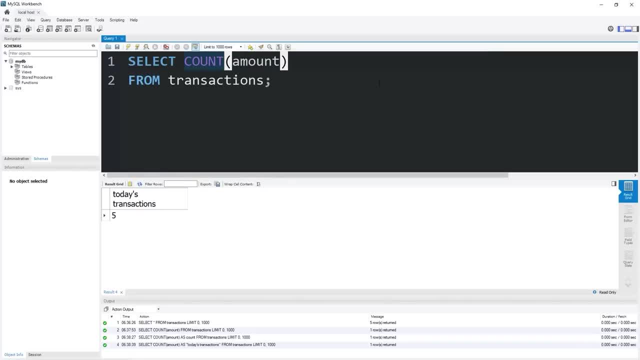 Let's find the maximum value of our column amount By using the max function. Within the set of parentheses, pass in your amount column. I will give this column an alias of maximum And that is the maximum amount. The largest order was $4.99. 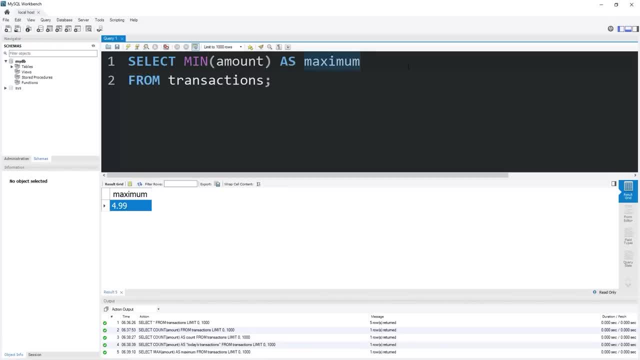 There's also min to find the minimum As minimum, The smallest order was for $1.. You could do average, which is AVG, As average. The average order is $3.45.. We can find the sum of a column by using the sum function. 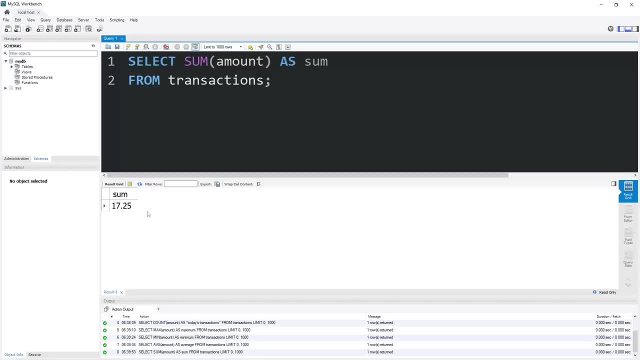 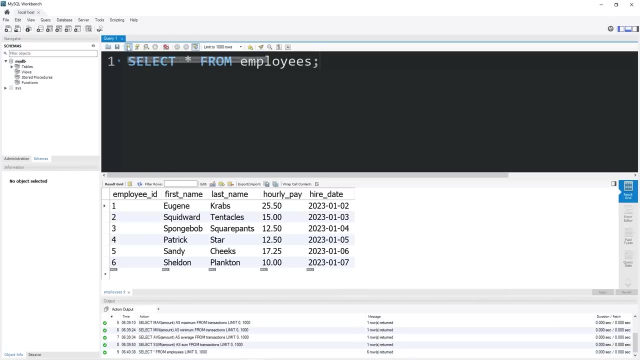 As sum. The sum of all of our transactions was $17.25.. Sum example: we're going to concatenate the first and last name of our employees, Select all from employees. We have two columns, one for a first name, the other 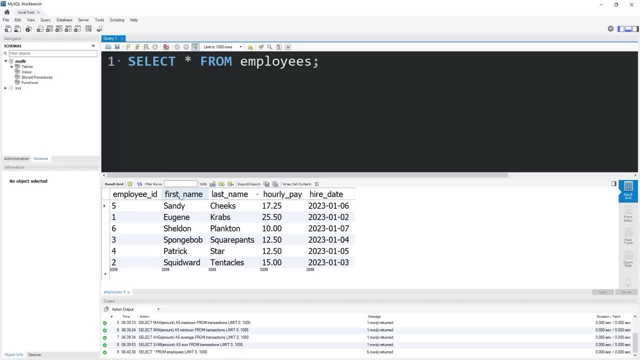 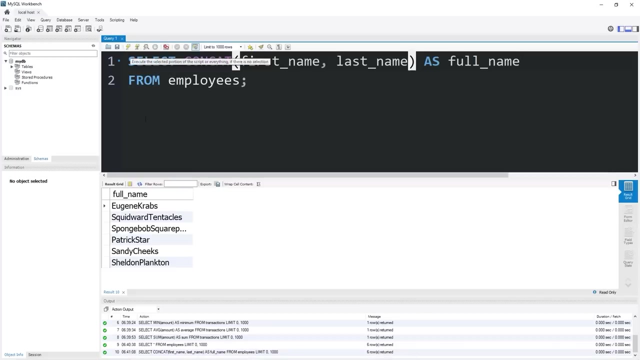 for a last name. We're going to combine these two columns together with the concat function, then create a new column named full name. Here's how to do that: Select concat- first name, last name. Then I'll add an alias as full name. Here's: 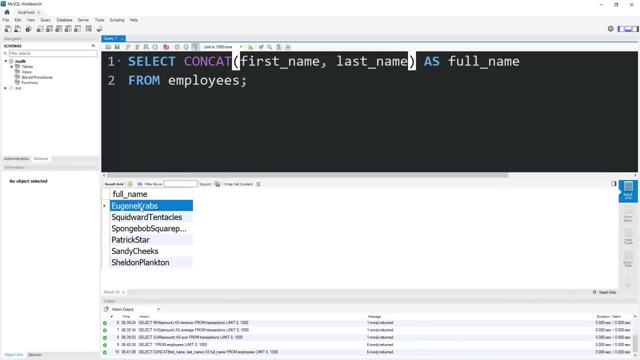 what we have so far. So we are concatenating the first and last names of our employees. However, we should separate each name with a space. Within our concat function, I'll add a space character surrounded with commas to separate each argument There. that's much better. So that is the concat function. We can concatenate. 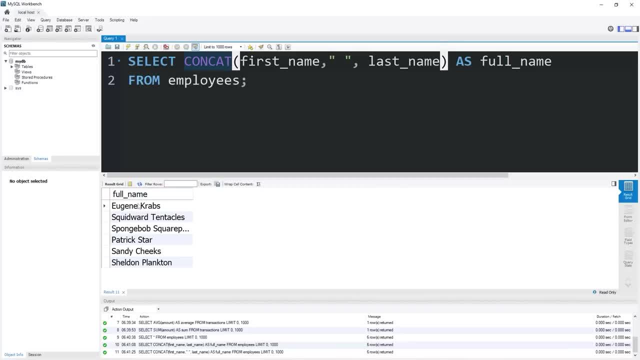 values together, such as if you need a column for somebody's full name. But yeah, those are just a few functions. There's still many more we haven't covered, but these are a few of the beginner ones you may be interested in. But yeah, those are. 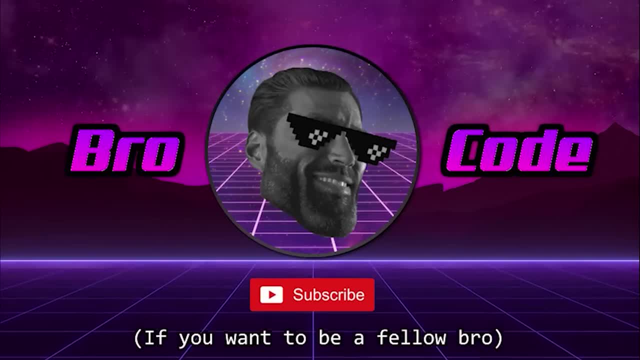 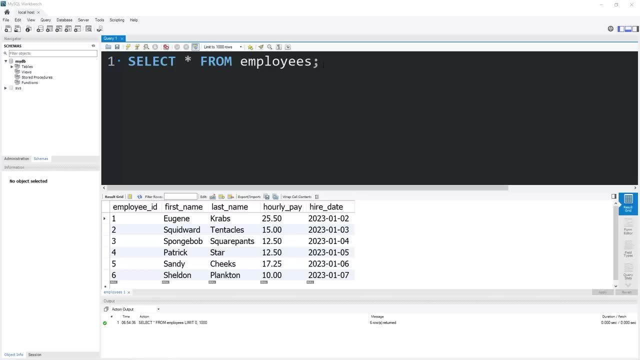 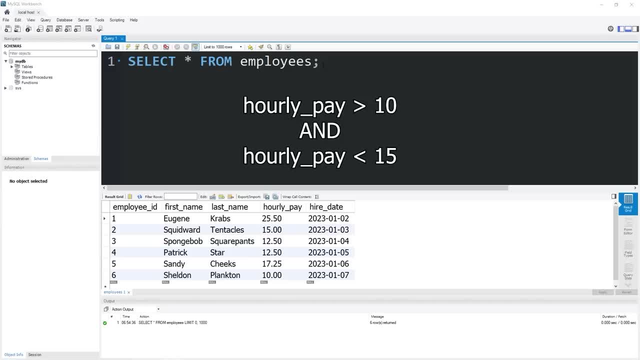 logical operators in MySQL. I would think of them as logical operators in MySQL. I would think of them as keywords that are used to combine more than one condition. For my examples to make more sense, I will add one more column, a job column. So let's alter our. 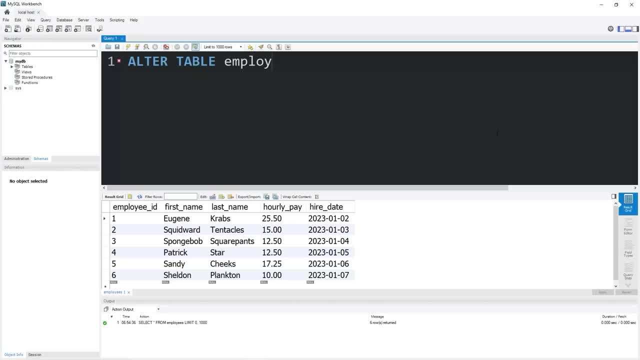 table of employees. Alter table employees. add column job. The data type will be varchar25.. I'll add this column after our hourly pay column. Then select all from my table employees. Here is our job column. Let's add some jobs to our employees. Let's. 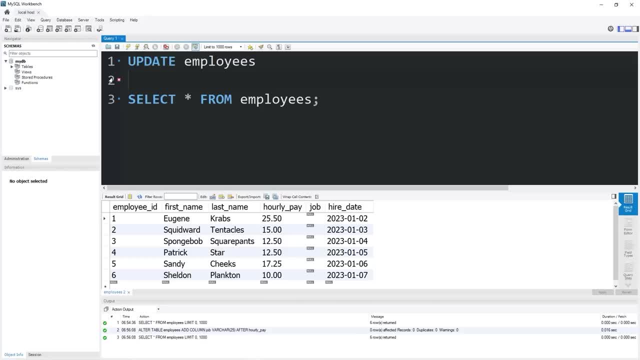 update employees. Set job equal to. let's select Mr Krabs, He will be a manager. Then be sure to add a where clause: Employee ID equals one. Mr Krabs is a manager. Squidward will be a cashier. Employee ID equals two- Spongebob Employee. 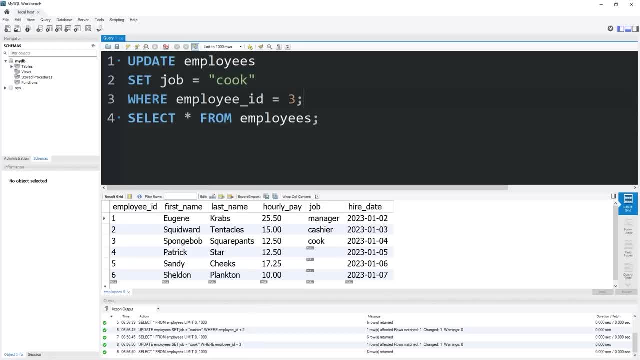 ID three. He will be a cook. Patrick will also be a cook. Sandy will be an assistant manager- Let's abbreviate the word assistant Assistant manager Plankton. Plankton will be a janitor. How is this related to logical operators? 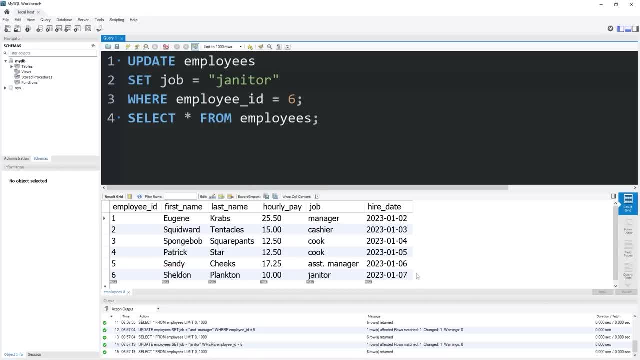 you're wondering. Well, using logical operators, we can check more than one condition. Suppose that our boss wants us to find any cooks that were hired before January 5th, How can we write a query that can satisfy those two conditions? Here's how We will use the and logical operator Select all from our 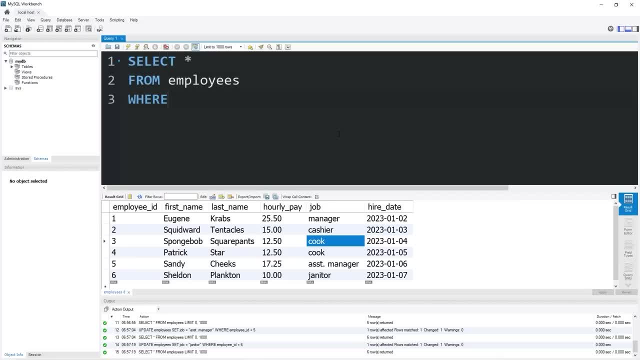 table Employees Using a where clause. we will write two conditions: Find any employees where the hire date is less than the year 2023, January 5th. So far, this would give us three results: Mr Krabs, Squidward and Spongebob. From these three: 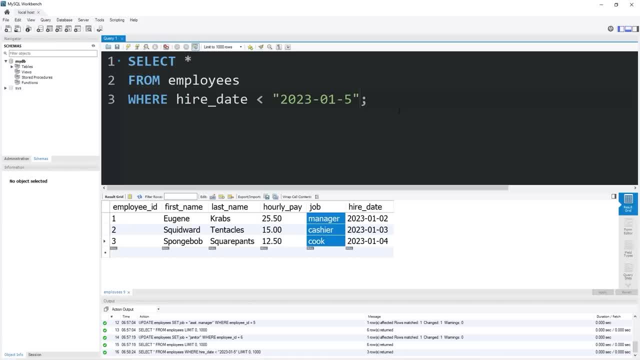 employees. how do we find any cooks? Well, we can add the and logical operator And we can write some other condition. Job is equal to cook. There we have Spongebob. He is a cook that was hired before January 5th, So that's the and logical operator. You will return any. 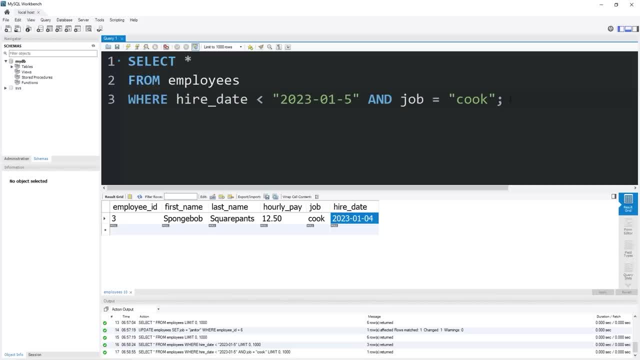 results that match these two criteria. Another logical operator is: or. You can check more than one condition. As long as one of those conditions is true, that row will be true. Let's find any cooks or cashiers. We can write some other. 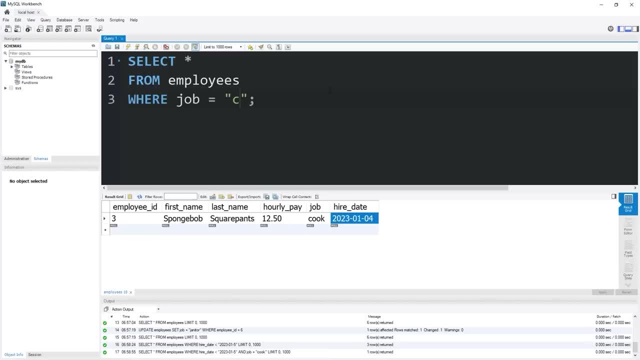 conditions. Job is equal to cook. That gives us both Spongebob and Patrick- They're both cooks- Or job is equal to cashier. That would also include Squidward. He's not a cook, but he is a cashier. With the or logical operator, only one condition needs to be true, Whereas 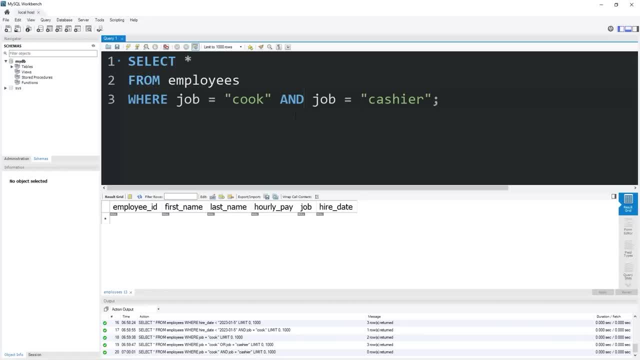 with the and logical operator. both conditions must be true. So that's the main difference between the and as well as or logical operators. With the not logical operator, not is a little different. Not basically reverses anything. you say. Let's find any employees that are not a manager Where not job equals manager. 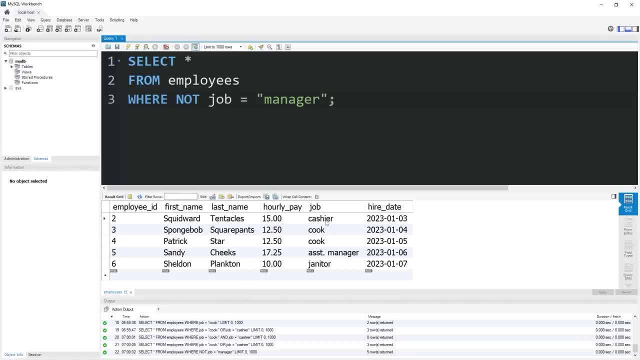 We have all of our employees besides Mr Krabs. We have cashiers, cooks, assistant managers and janitors. You can combine logical operators too. Let's find anybody that's not a manager and not an assistant manager, Let's add. 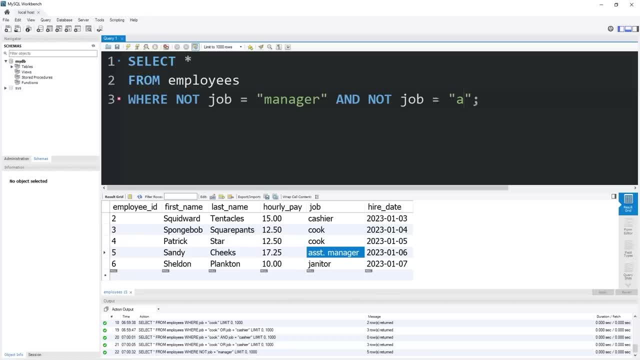 And not job equals assistant manager. We have everybody besides a manager and besides an assistant manager. Mr Krabs and Sandy are not within the results. So that is the not logical operator. It basically reverses whatever condition you write. There's also between Between. 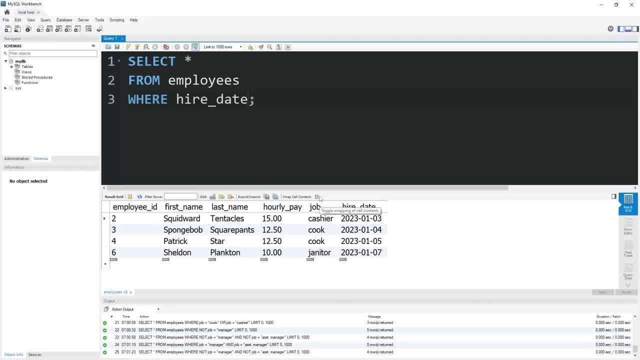 is used within a single column. It's very similar to the and logical operator, except people prefer to use the between logical operator when working with the same column, just because of its readability. Let's find any employees where the hire date is between January 4th and January 7th. 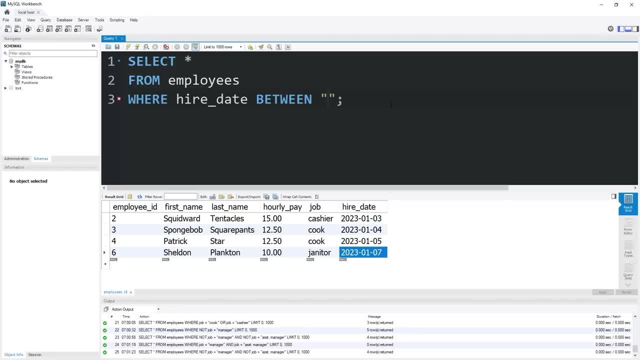 Where hire date between two values: 2023, 01, 04, and 2023, 01, dash 07.. So we have Spongebob Patrick, Sandy Sheldon. There's also the in logical operator We can find. 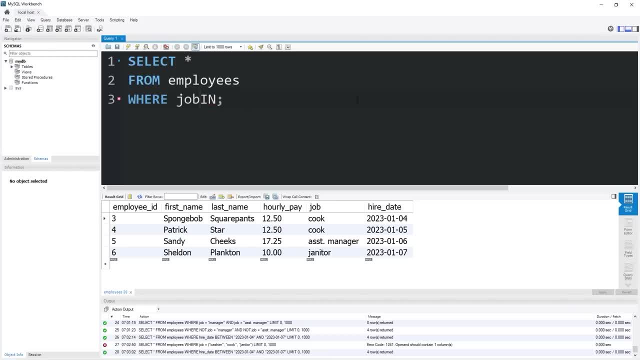 any values that are within a set. Let's find where job is in: Cook, cashier or a janitor. Yep, we have a cashier, a cook, a cook and a janitor. There is more than one way to write a query where you need to match more than one condition. 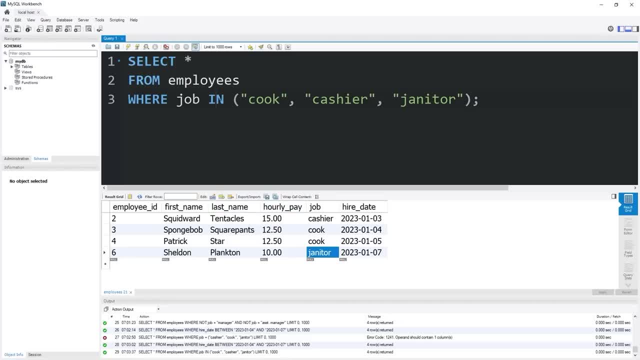 Really, the best way depends on your data set. Basically speaking, logical operators are used to check more than one condition, but they're done so in different ways depending on the logical operator that you're using. But yeah, those are logical operators in MySQL. 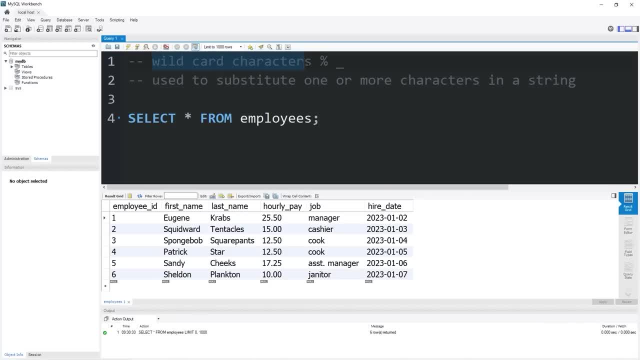 Hello again people. Today I'm going to be explaining wildcard characters. There are two: the percent and the underscore. Each of these is used to substitute one or more characters in a string. Here's an example: I have a table of employees. What if I need to find any employees? 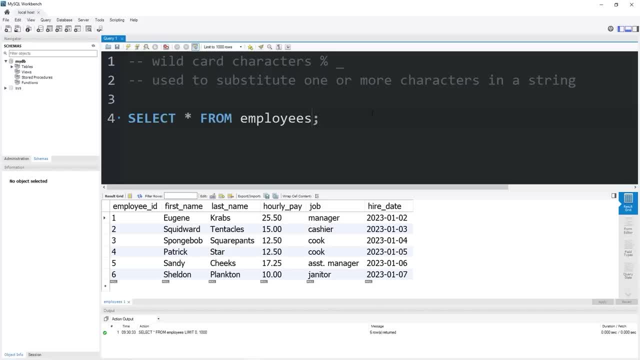 whose first name begins with an s. Well, you would think you could write something like this, Where first name is equal to s. Now, this technically doesn't work. Here. what we're doing is telling MySQL to find any first names that are equal to the character s. If I instead need to find: 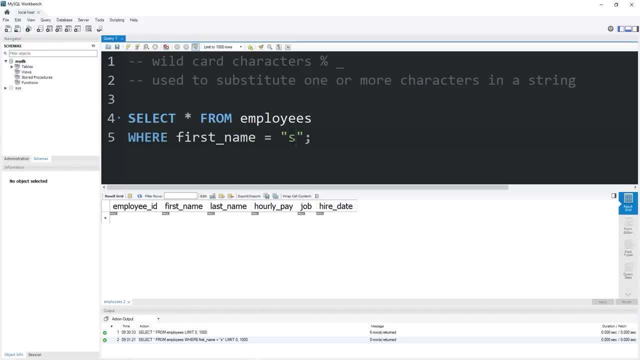 any first names that begin with the character s. I can type s, then the percent wildcard operator. the percent wildcard operator represents any number of random characters. But there's one more change we need to make: Replace the equals operator with the like operator, Like when used with an aware clause. 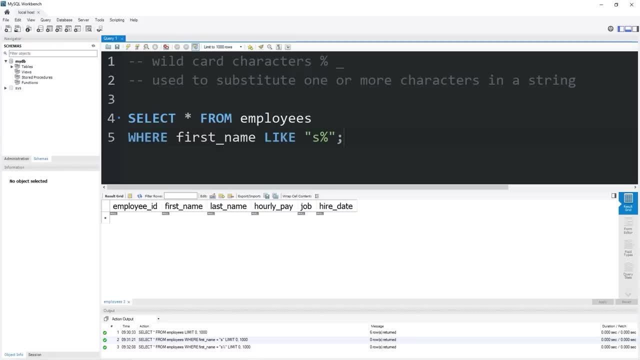 searches any patterns, We will return any first names that begin with the letter s. So the results are: Squidward, Spongebob, Sandy, Sheldon. Their first names all begin with the letter s. We could do this with dates too. Let's find any higher dates in the year 2023.. Technically, that 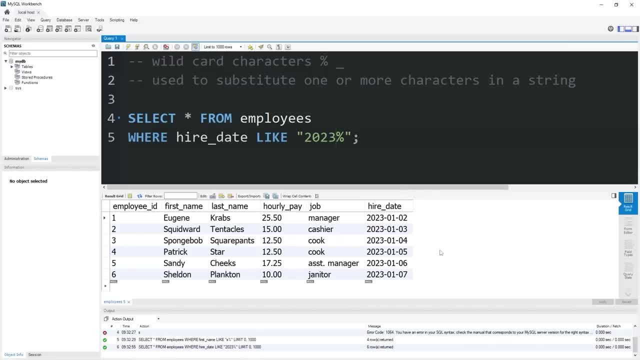 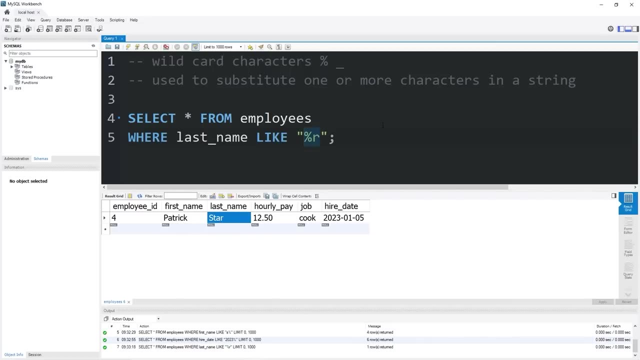 would return everything in my example, because all the higher dates are in 2023.. We can even find if something ends with a character. Let's find any last names that end with the character r. That would return Patrick star Star with an r at the end. You could add more than one character. 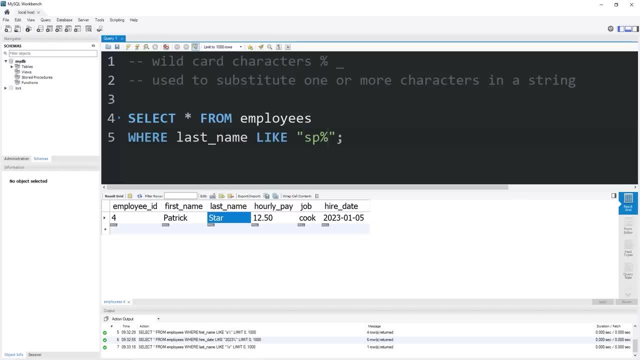 Let's find any first names that start with sp. Then change last name to first name. That would return one result: Spongebob, sp. On the other hand, we have the underscore wildcard character. The underscore wildcard character represents one random letter. Let's find any jobs that have one random character. 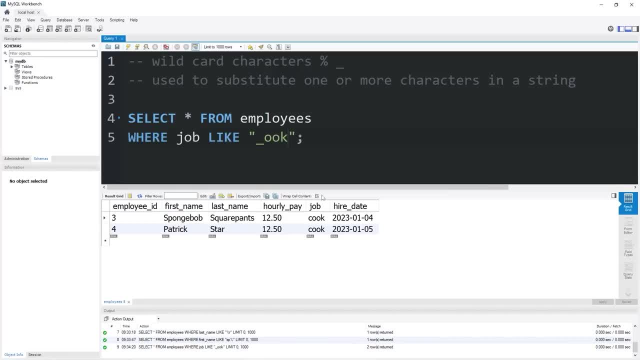 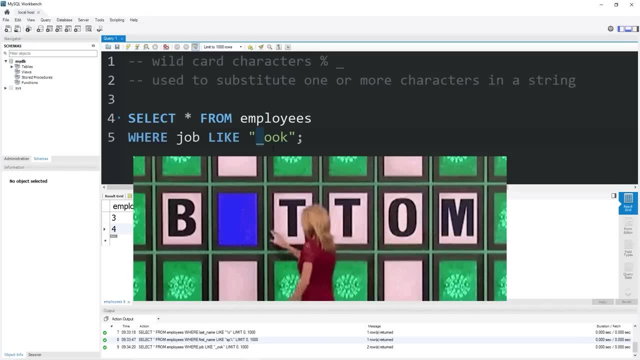 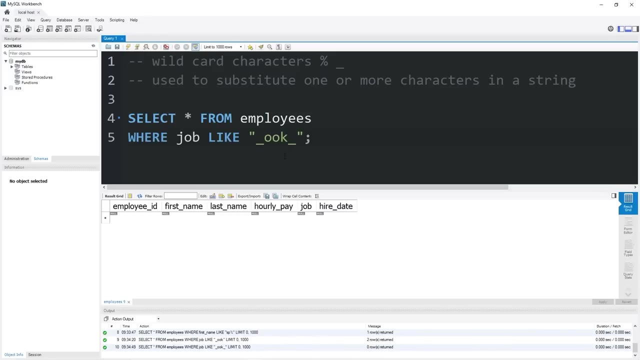 followed by o-o-k. That would return any cooks. The underscore kind of reminds me of that game wheel of fortune. My sql is going to attempt to fill in any blanks with a matching character. If we, If we had two underscores, well there technically wouldn't be any matches. 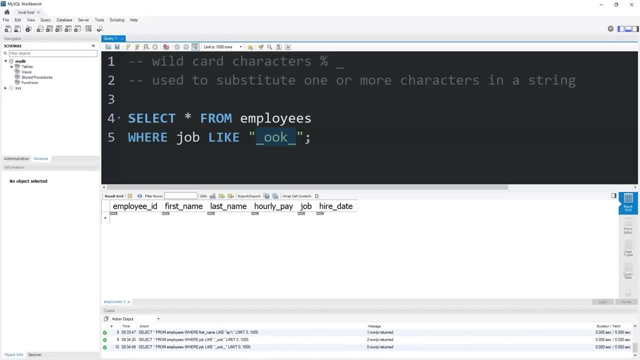 MySQL would technically be looking for a five letter word where the middle three characters are OOK, but there's no matches. Here's another example: Find any higher dates in January. Higher date is like the year is going to be random. 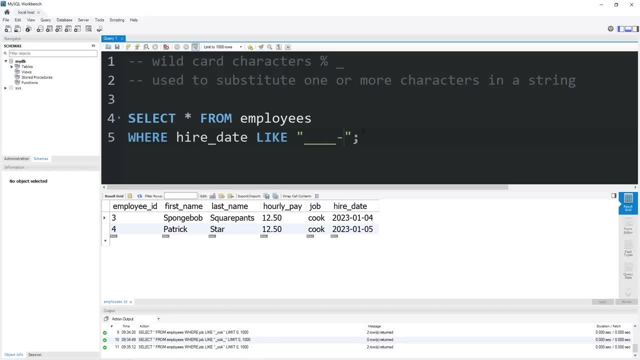 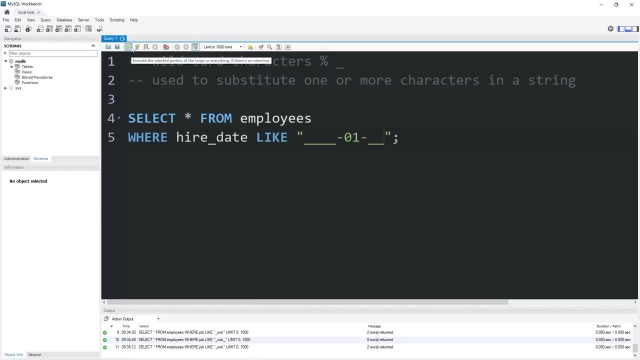 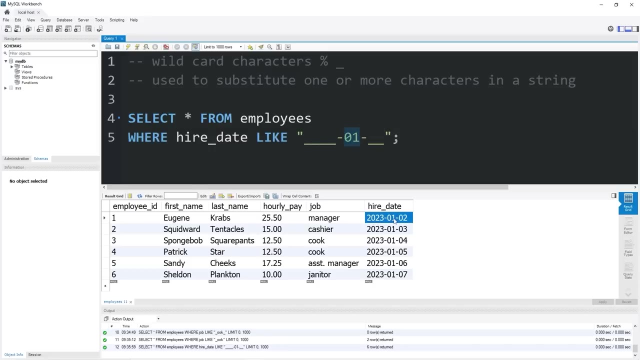 We have four digits, 1234, a dash, character 01, dash- then a day of the month. So two underscores Again. that would return pretty much all of our employees. they were all hired in January. Maybe we don't care about the year or the month, but we care about the day of the month. 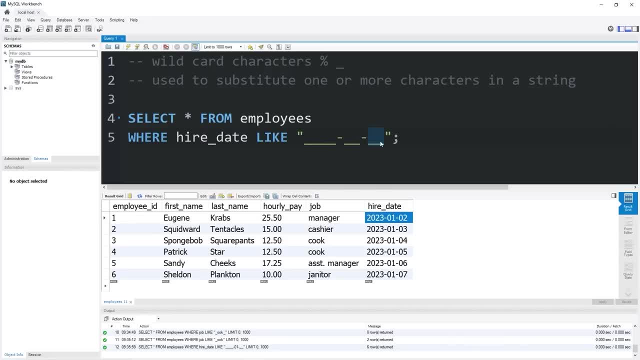 So let's replace the month with underscores: 02.. That would return, Mr Crosby Crabs 03.. That would be Squidward. Now you could combine these two different wildcards together too. Let's take a look at our jobs. 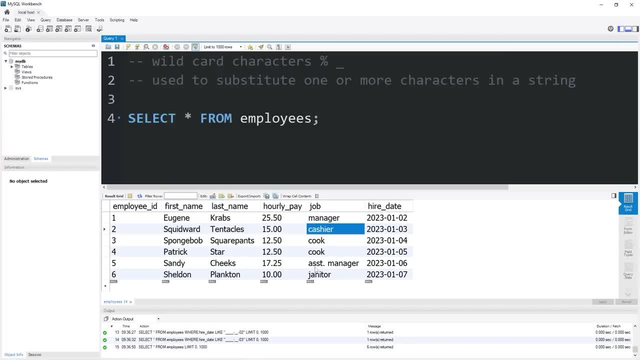 Let's find any jobs where the second character is an A. I know it's kind of a weird example, but hopefully it'll make sense. Select all from employees where job is like: Now we're going to combine these two wild characters: The second character has to be an A. 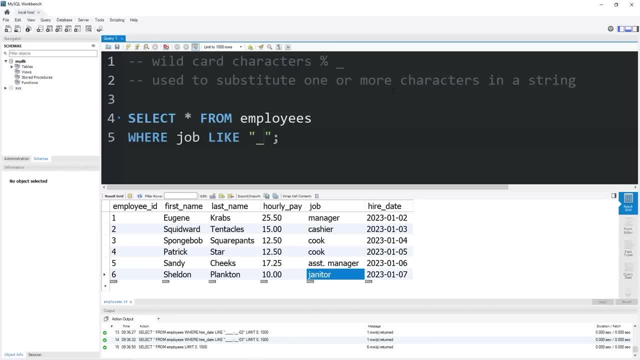 Okay, We could use the underscore for the first character A, then any amount of random characters afterwards. That would return a manager, cashier or janitor. So yeah, those are wildcard characters. You can use these to substitute one or more characters in a string. 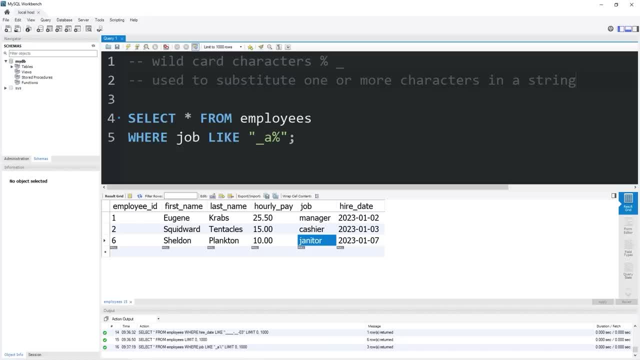 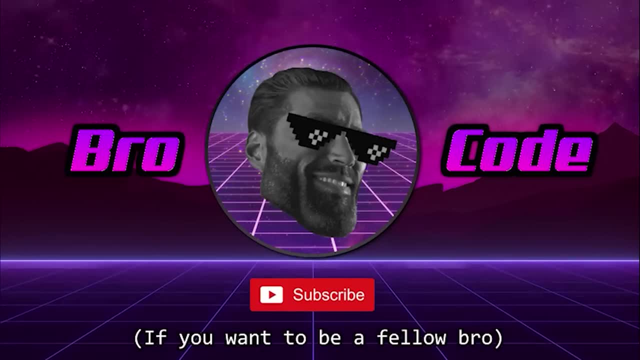 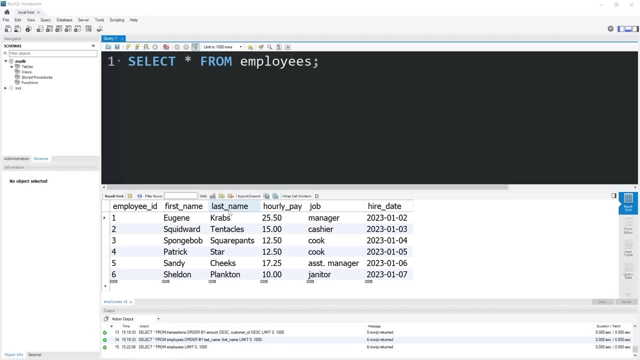 It's pretty helpful if you need to find if a string starts with some value or ends with some value, And those are wildcard characters in MySQL. Hey everyone, I have a super quick video on the order by clause. The order by clause sorts the results of a query in either ascending or descending order. 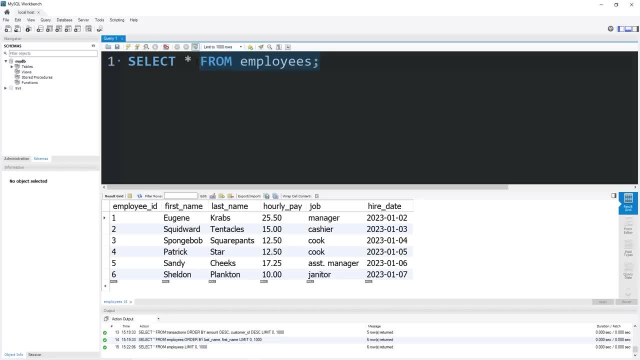 based on which column we list. Here's an example. I have a list of employees. How can I list all of these employees alphabetically? Currently they are listed by their employee ID. Well, at the end of my statement I can add an order by clause. 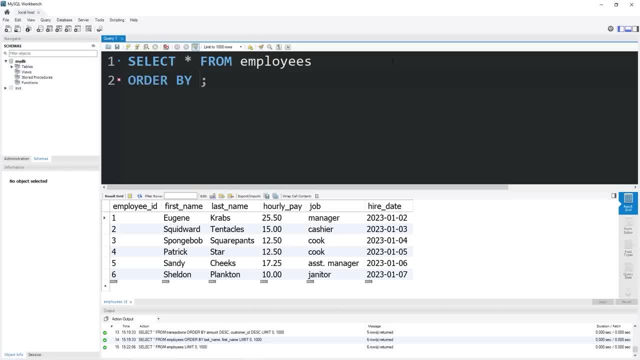 Order By Then a column to order our roses. Close by. Let's order all of these employees by their last name. Now, by default, they will be ordered in ascending order or alphabetical order. if you're working with characters For descending order or reverse alphabetical order, just add DESC for descending. 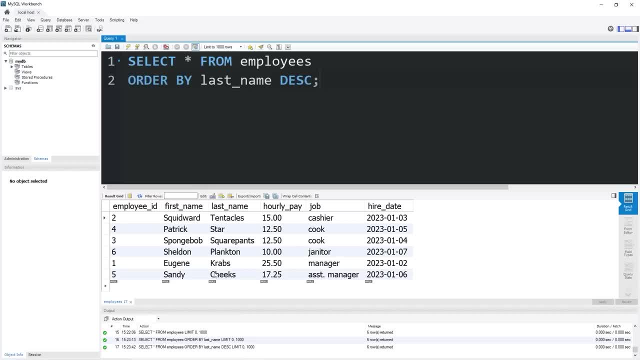 Now these employees are listed in reverse alphabetical order, or descending order. For ascending order, that would be A-S-C, but that is the default, So you don't explicitly need A-S-C. Let's order these employees by their first name. 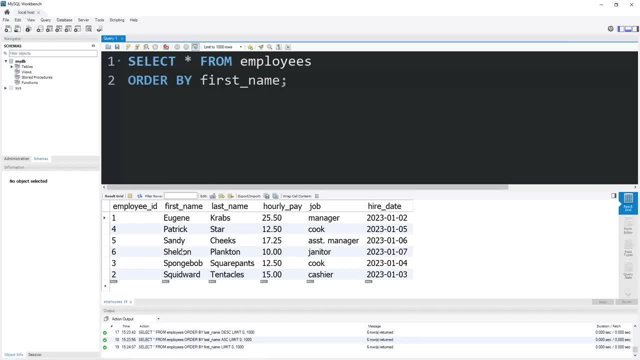 First name. These employees are listed alphabetically by their first name. Let's do reverse alphabetical order. Yeah, there we are. Let's order these employees by their hire date. Hire date in ascending order. You don't even technically need that keyword ascending, it would still work just fine. 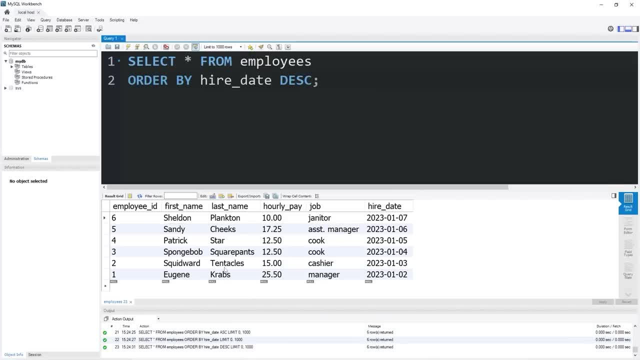 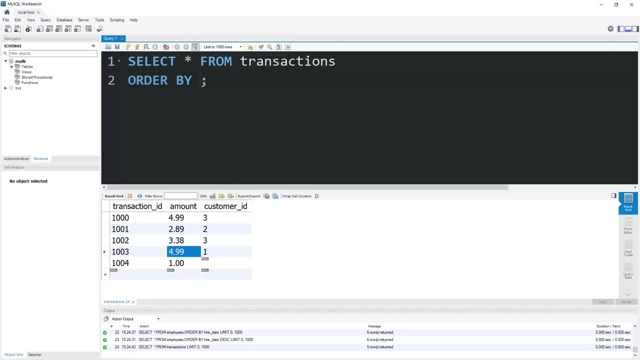 Now descending. I think we have the hang of it now. Let's select all from transactions. There's one more thing I want to show you: Select all from transactions. We have two transactions with the same amount. Let's order by amount. 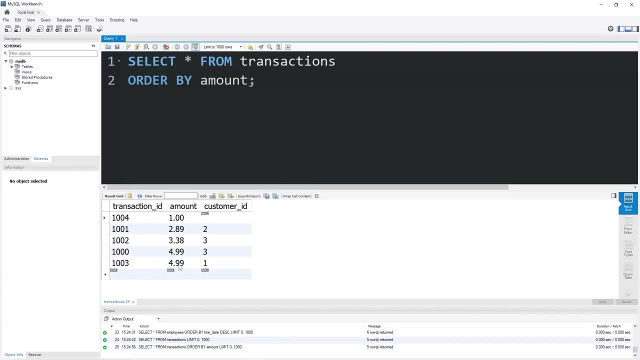 When ordering a column. if two values share the same amount, we can add an additional column to compare by Another. tunnels can be added from here. Now just screenshot the technique once again, so you follow me. All the results will appear automatically in the click add- 在₀. Well, Captioneafficlecom. 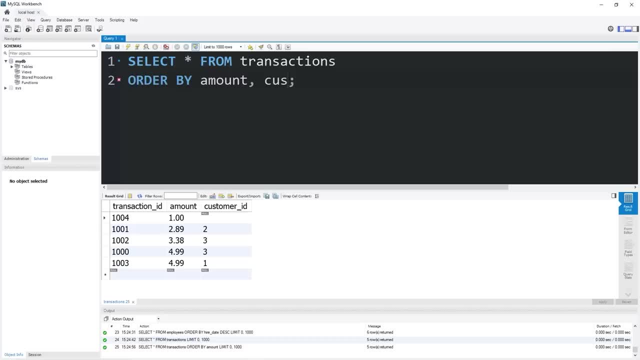 Mm. hmm, order by, maybe customer ID. these two rows are now flipped so you can order by more than one column. if two columns share the same amount, then order by some other column. then you can add ascending, descending, however you want to order your table. so yeah, that is the order by. 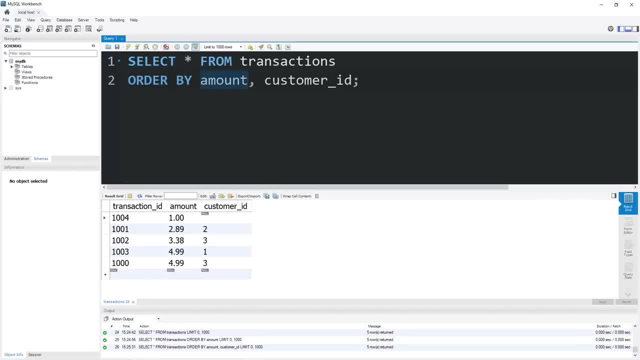 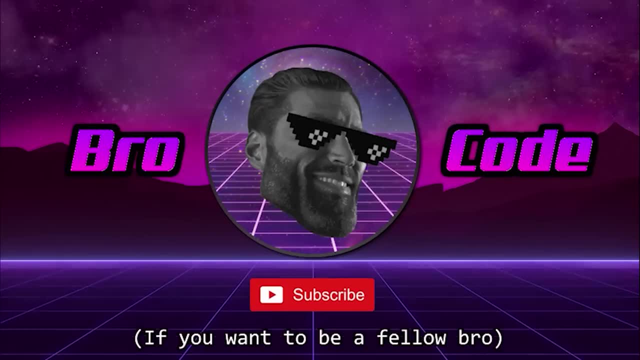 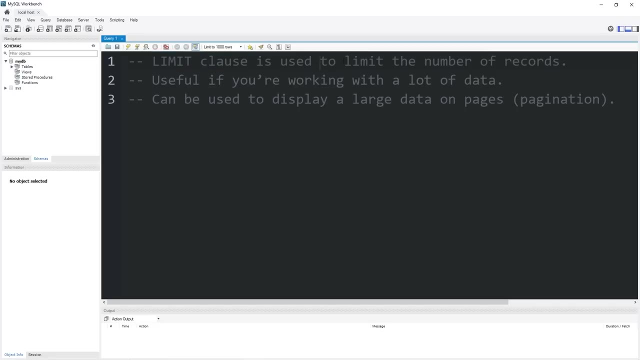 clause you can order your rows by some column you specify in ascending or descending order. but yeah, that is the order by clause in MySQL. hello, it's me again. today I will be explaining the limit clause. the limit clause is used to limit the number of records that are queried. 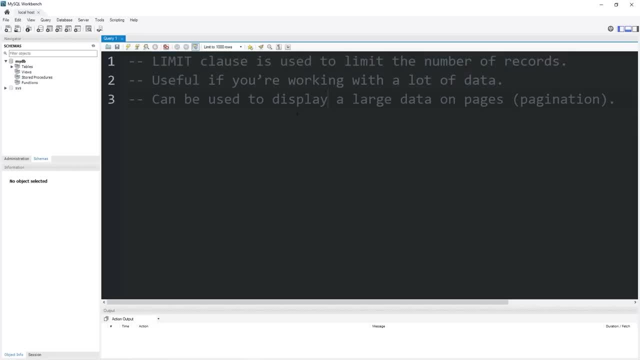 it's very useful if you're working with a lot of data. one use is that you can display a large data set on different pages, also known as pagination. here's an example. I have a few customers, not very many. I'm working with a small data set if 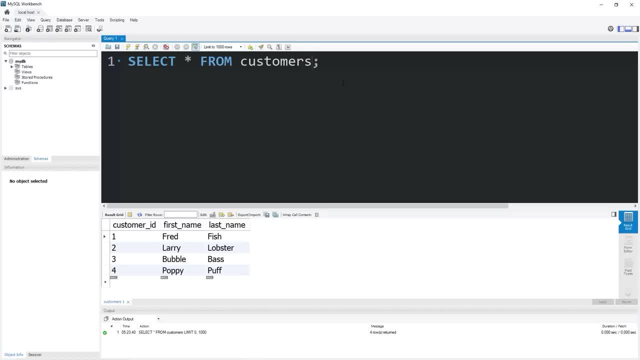 I would ever need to limit the amount of customers that are displayed. I can add a limit clause, then set how many I would like to display. I would like the first customer limit, one that would return Fred fish in my example. if I need the first two, that would be Fred, then Larry three. 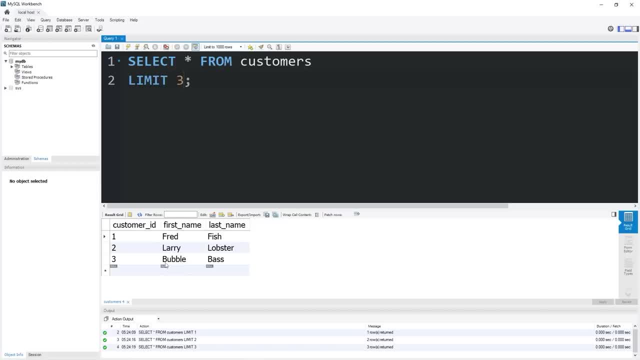 is Fred Larry bubble. that's kind of a weird first name, and then four would be poppy. currently these records are organized by customer ID. we could combine the limit clause with the order by clause. let's order by last name, then limit one. that would return bubble bass. it's an alphabetical order, or we? 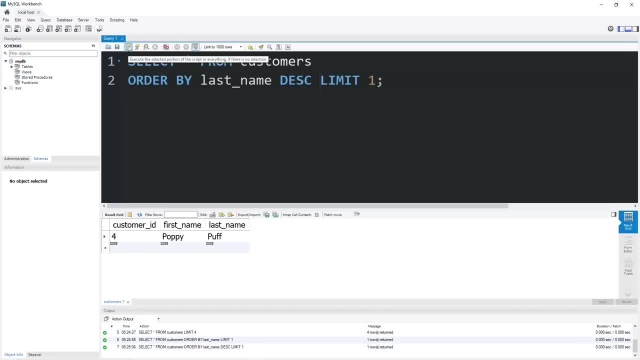 could do. last name, descending limit one: poppy puff has the name in least alphabetical order, I guess. basically speaking, limit limits the number of records that are returned. it's very useful in combination with the order by clause, which we learned about in the previous topic. now, with the limit clause, you can add an offset limit, one one, the first. 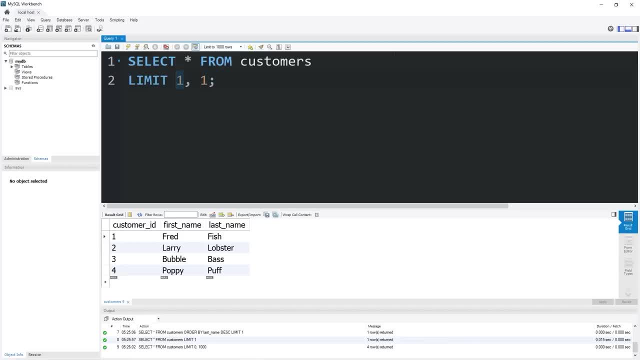 number is the offset limit to one record after the first. that should technically return Larry Lobster- yep, Larry. limit two would add an offset of two which returns bubble bass. limit three would return poppy puff. using an offset would be very helpful when working with a large data set, if you need to display your records on different pages. suppose that our 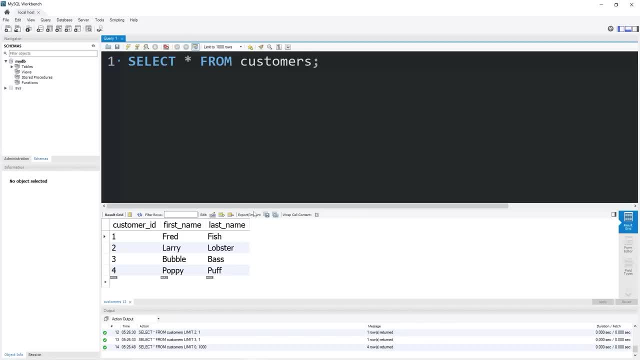 data set is maybe 100 customers. I need to display 10 customers per page, so the first 10 would be just limit 10.. but you know my data set's really small so it's not going to be apparent. if I need the next set of 10 customers, I can add an offset of 10.. although 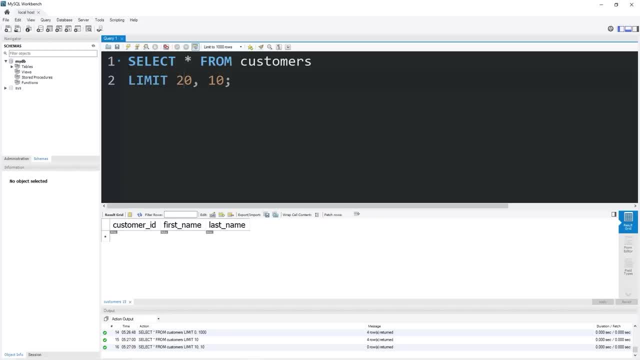 I don't have that many customers to begin with. the next set of 10 customers would be an offset of 20, then display 10, you know, then 30, 40, so on and so forth. so yeah, that's the limit clause. you will limit the results that are queried, type, limit, then some number. you could add an offset, so display. 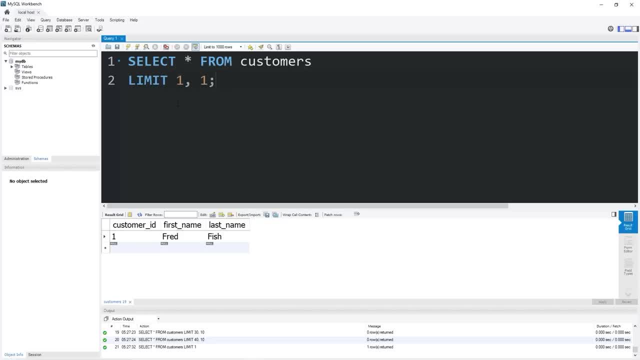 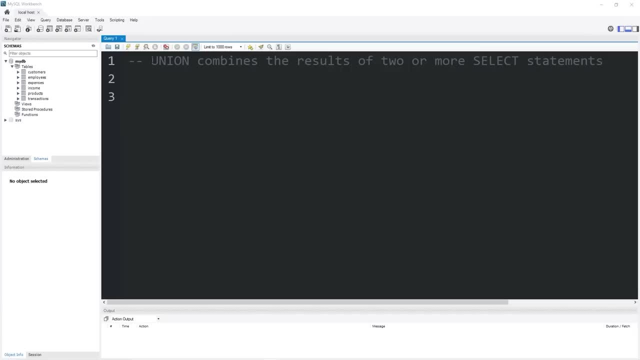 some number of records after an offset. but yeah, that is the limit clause in MySQL. hey, welcome back. today I will be explaining the union operator. the union operator combines the results of two or more select statements. I have created two additional tables. I'm only going to be using them temporarily. I'll delete them once we're done with this example. I have a table of 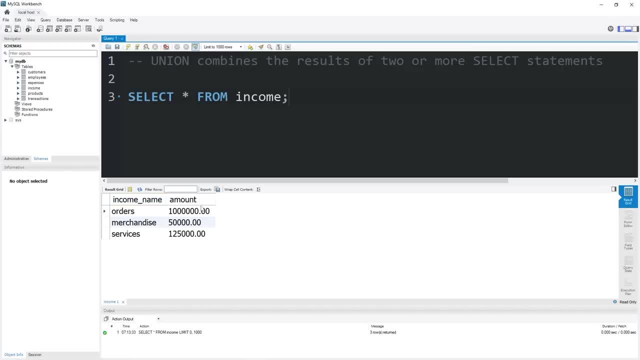 income. we have two columns: an income name and an amount. I just made up some numbers. they're probably not realistic. I also have a table of expenses. here's my table of expenses. we have an expense name and some amount. again, I just made up some numbers. suppose that our boss wants us to. 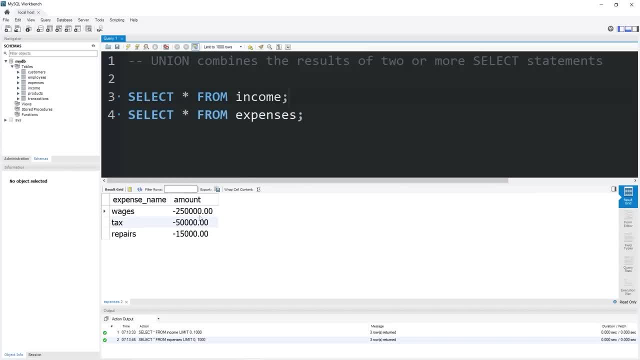 print a list of all of our different income versus expenses all in one window. well, we can easily do that with the union operator. after our first select statement, delete the semicolon add Union. We now have a window with the results of these two select statements. we have income and expenses. 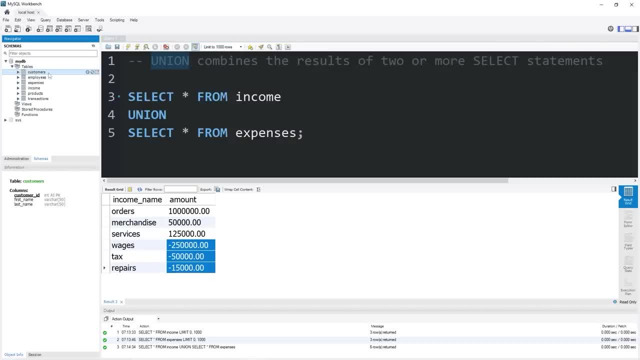 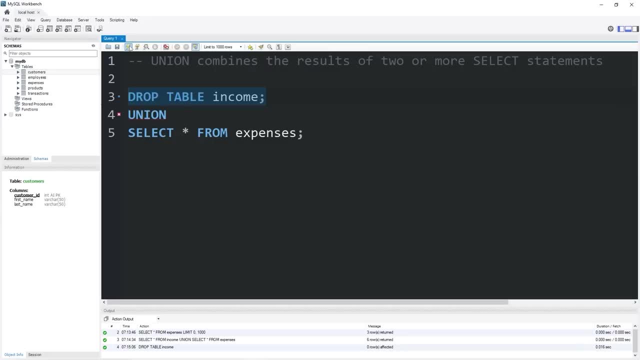 let's perform a similar operation with our employees and customers table. I'm going to drop these tables, though they were only temporary. drop table income, drop table expenses. let's begin. mr Krabs, our boss. he wants us to create a list of everybody that enters the store, all. 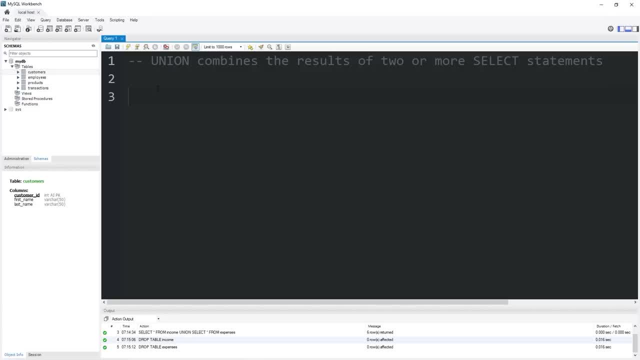 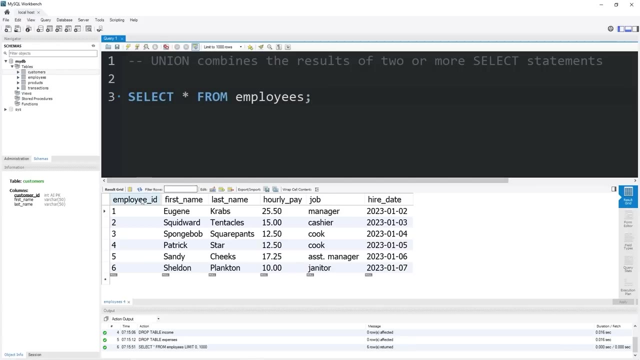 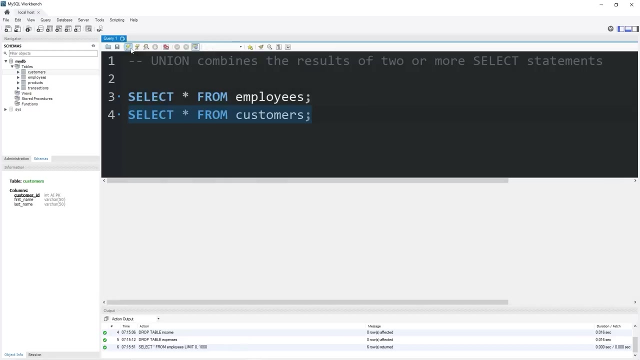 and all customers. Well, we can join together those select statements with the union operator. But first let's take a look at each of these tables, Select all from employees. We're going to have one problem: Our employees table has six columns, whereas our customers table- our customers table- has three columns. If 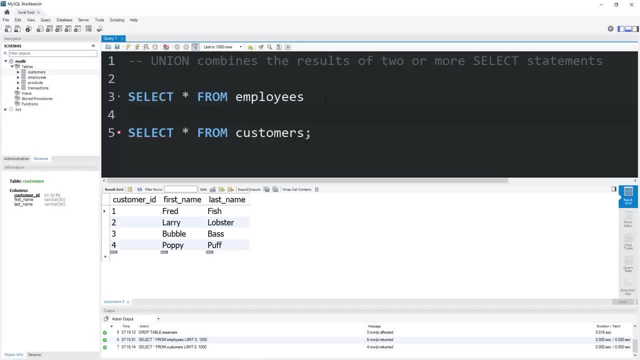 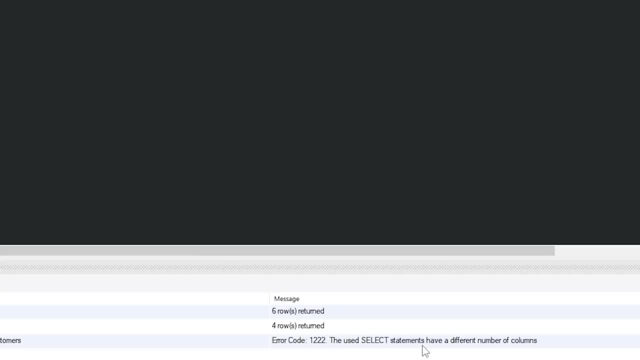 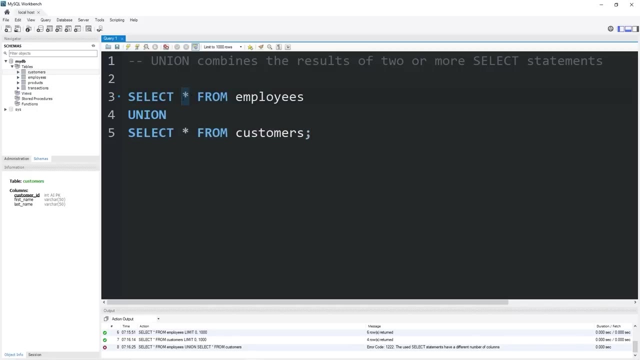 you're combining two different select statements that have a different amount of columns, a union isn't going to work. We have a problem. The used select statements have a different number of columns. In order to join two select statements together, they need the same number of columns. My employees table has 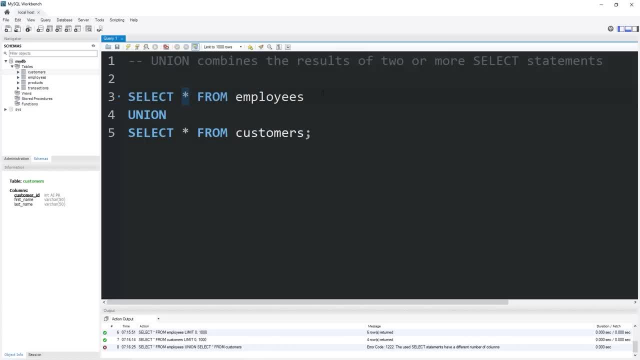 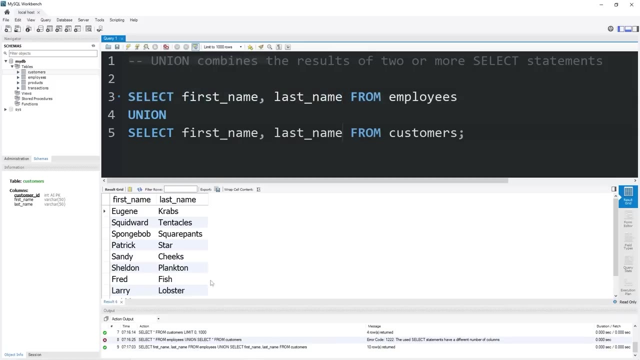 six columns. My customers table has three. Well, we could select distinct columns. All I need is the first name and the last name of each of these tables. First name, last name, And look at that. that works. We have now created a list of 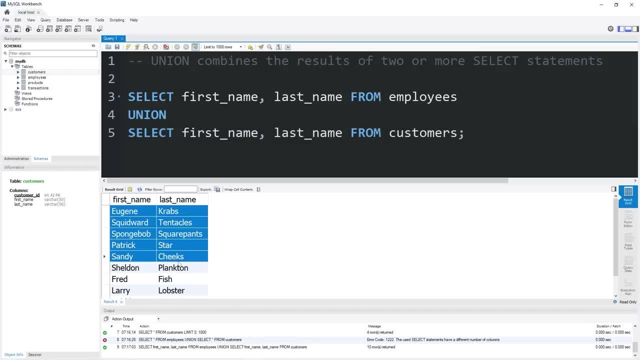 all of the different people that enter our store, both employees and customers. There is a different variation of the union operator. that is union. all That would include any duplicates if more than one value is found within each table. Just temporarily, I'm going to insert plankton into our customer. 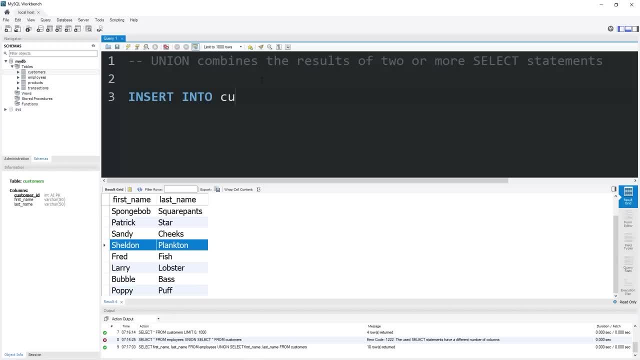 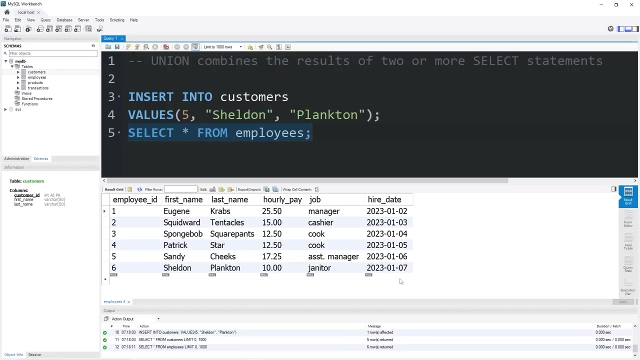 table. Insert into customers some values. Customer ID 5, first name Sheldon. last name plankton- Select all from customers. Plankton is both in our customers table and our employees table. Now what would happen if I add a union to those two? 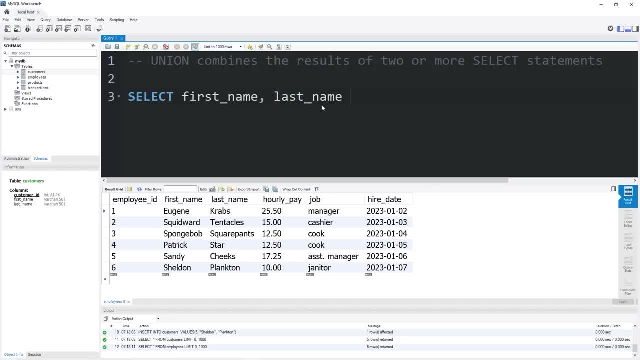 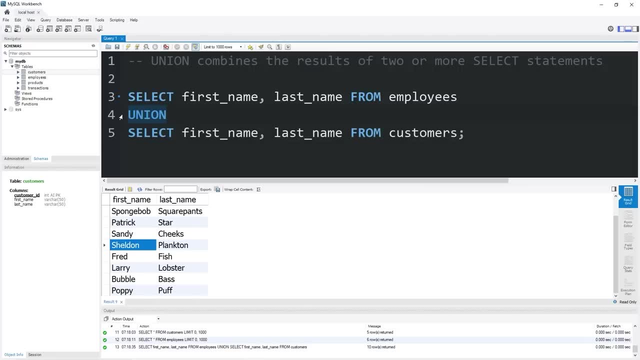 select statements With just union by itself. union doesn't allow duplicates. Sheldon plankton is only within our list once. With union, all you would include duplicates. Now Sheldon plankton is in this list twice. So use whatever is more fitting for your situation. I'm gonna go ahead and delete plankton from. 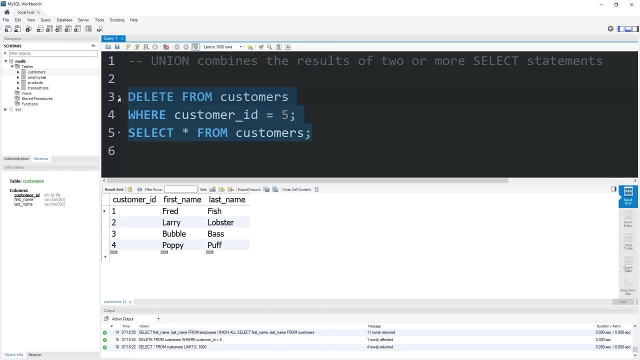 this table of customers. Alright, yeah, so that's a union, everybody. a union combines the results of two or more select statements. In order to do so, those two or more select statements need the same number of columns. But yeah, that is the union operator in MySQL. 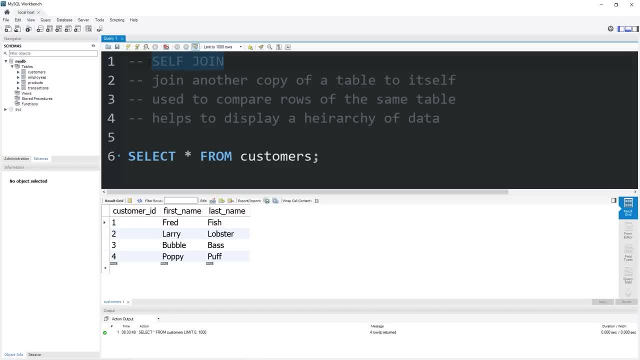 Hey everybody, Today I'm gonna be explaining self joins. A self join is really just any type of join where you join together another copy of a table to itself. They're used to compare rows of the same table. They really help with displaying a hierarchy of data. So a self join- 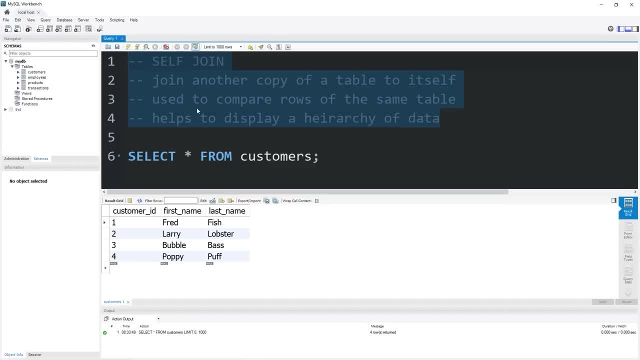 you just join another copy of a table to itself. So here's an example. I have a table of customers. I'm going to create another column named referred by. If a customer refers somebody and they register as a new customer, maybe they get like a free meal or something. Let's create a new column within our 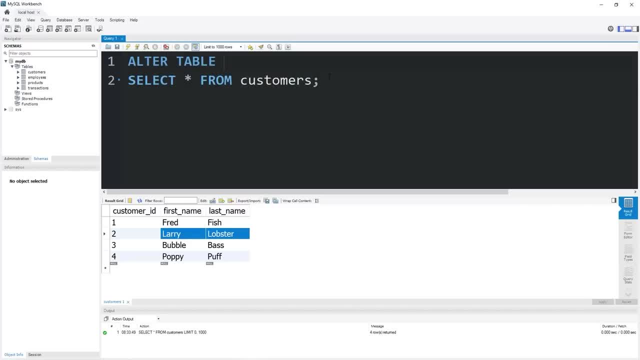 customers table: Alter table. customers add referral id. The data type will be int. Then select all from customers. Now let's populate this column: Update: customers Set referral id equal to one Where customer id equals two. Our first customer, Fred Fish. he was not referred by anybody. 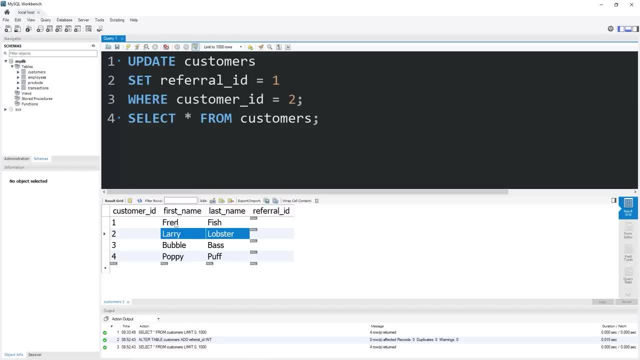 That value will be null. However, Larry Lobster was referred by Fred Fish. We'll set the referral id for him to be one. Larry Lobster was referred by Fred Fish, So Fred Fish gets a free meal at the Krusty Krab. Now Larry Lobster, he's going to refer both Bubble Bass and Poppy Puff, So he'll 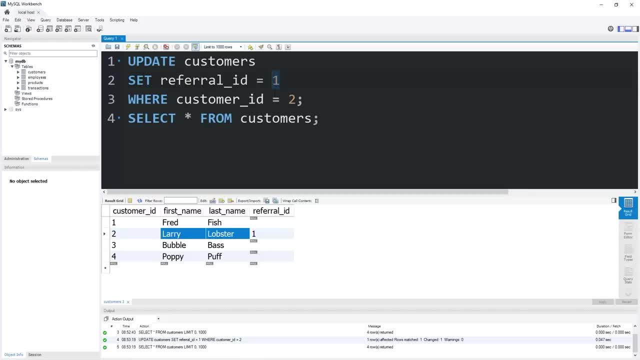 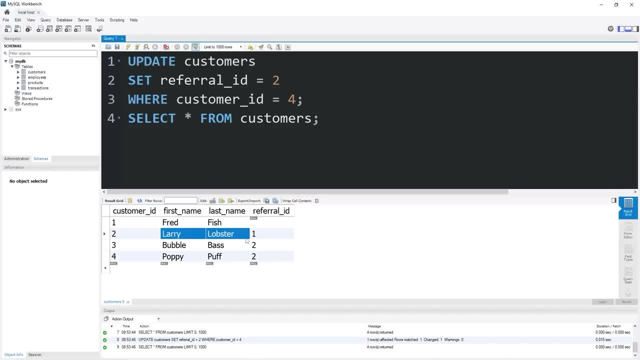 and four. Fred Fish referred Larry Lobster, Larry Lobster referred Bubble Bass and Poppy Puff. It makes me think of a pyramid scheme. I'm going to use a self join to replace our referral id column with the first and last name of the customer that referred one of these people. 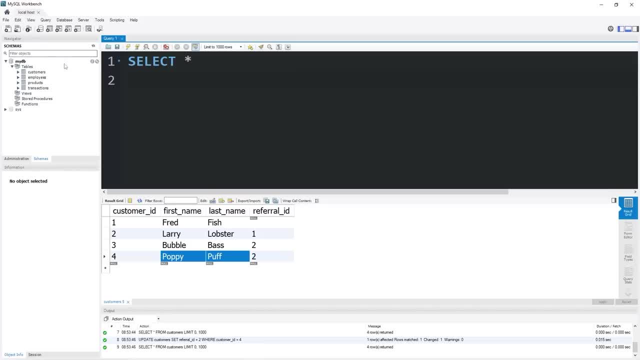 So I'm going to select all Now when, using a self join, we'll take from our table customers, then interjoin customers. Basically, we're just joining another copy of a table to itself, but we'll need to give these tables what's known as an alias, a nickname. 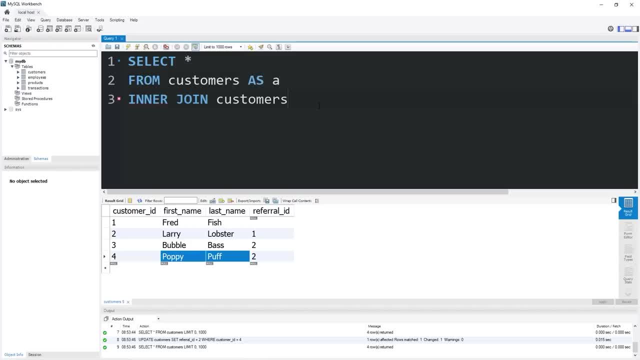 Let's say from customers, as maybe a- that's the nickname- Interjoin customers as b. The original copy of our customers table will be referred to as a. The copy will be b. They are the exact same table but we have two of them and we'll stitch them together with a join. 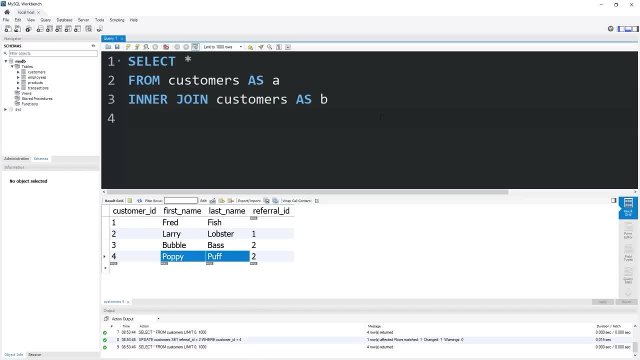 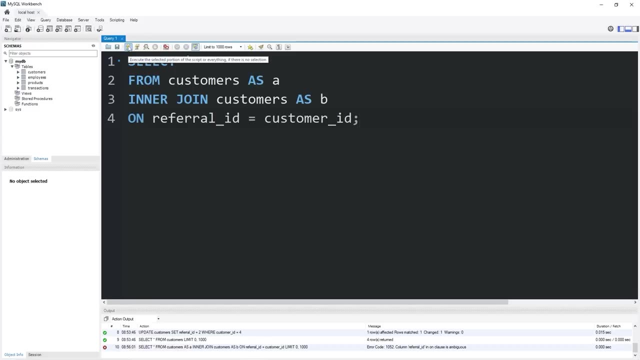 To link these tables by the referral ID and the customer ID, I'll add this additional line on referral ID equals customer ID. Let's take a look to see what we have so far. Column referral ID in on clause is ambiguous. Am I referring to the referral ID of table A or table B? 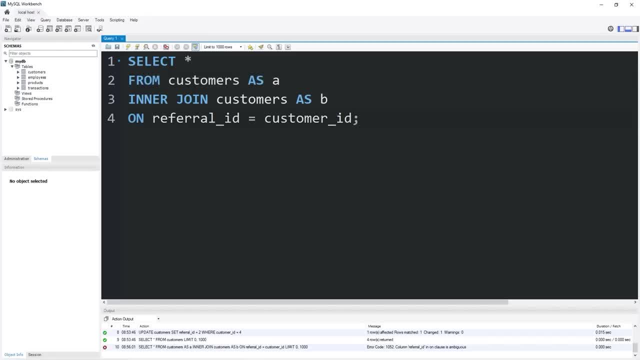 I'm referring to the referral ID of table A. What I'll do is prefix this column name with the name of my table, followed by dot. A dot. referral ID equals. I need the customer ID from my table copy, which is known as B. 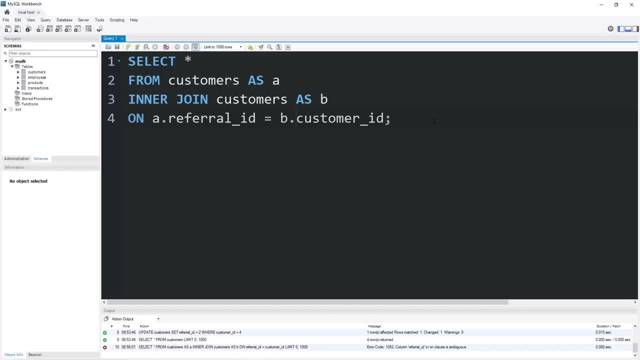 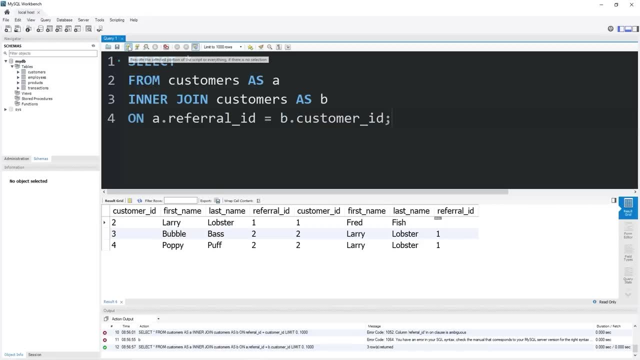 I will prefix B to this customer ID column. The referral ID of table A is linked to the customer ID of table B. Oh yeah, look at that, We have joined these two tables. The referral ID of table A is linked to the customer ID of table B. 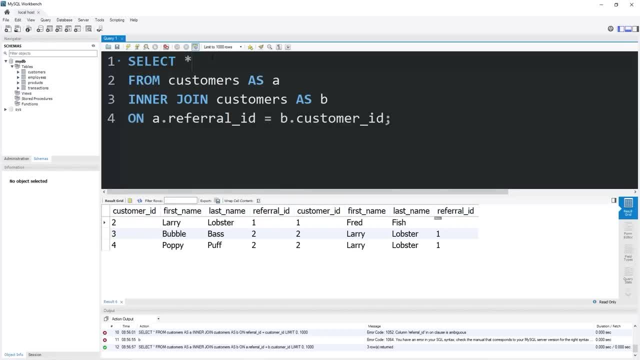 I don't necessarily need all of these columns. We're displaying everything. Let's select only specific columns. I would like a customer ID, first name, last name. Now we have one problem With our first name and last name. do we mean the first and last name? columns of table A. Or table B. Let's prefix these columns with the name of our table, the alias we're using. I would like the first name from table A, the last name from table A, followed by- I'm going to put this on a new line, just for readability. 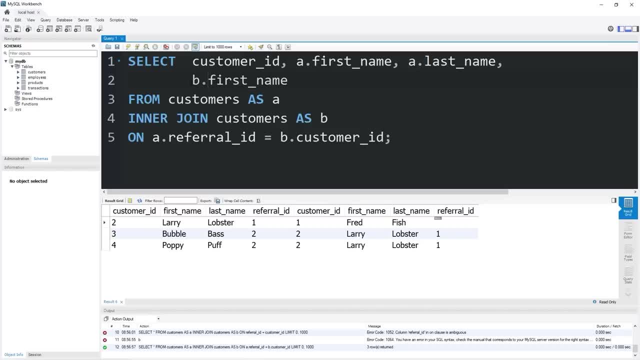 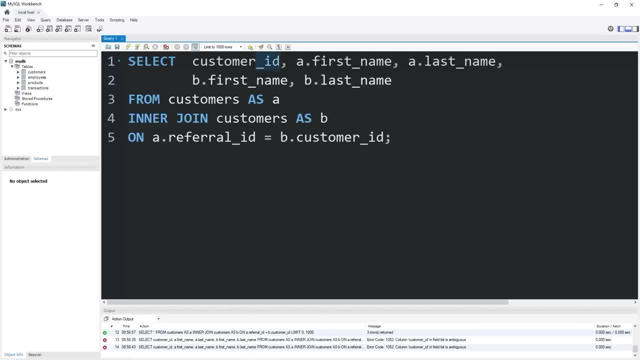 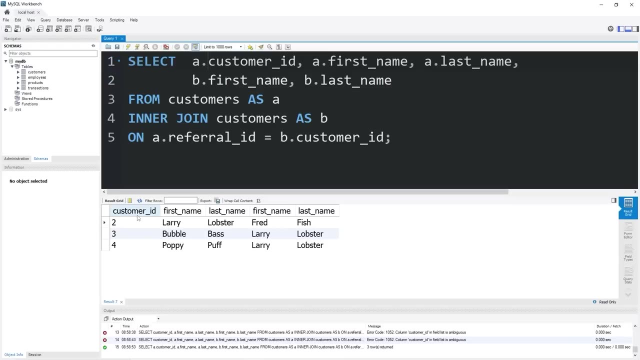 the first name of table B, then the last name of table B, Then be sure to include that within the customer ID too, So the customer ID of table A. Okay, we're getting somewhere. Customer ID: first name, last name. first name, last name. 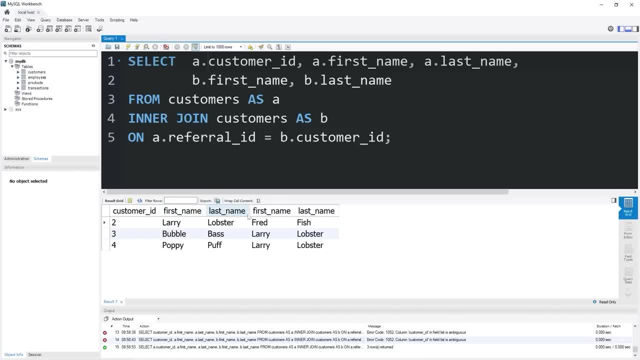 Okay. so if somebody were looking at this table they would think: why are there two columns for both first name and last name? Let's concatenate these two columns: Concat: first name, last name. I'll add a space in between the first name and last name. 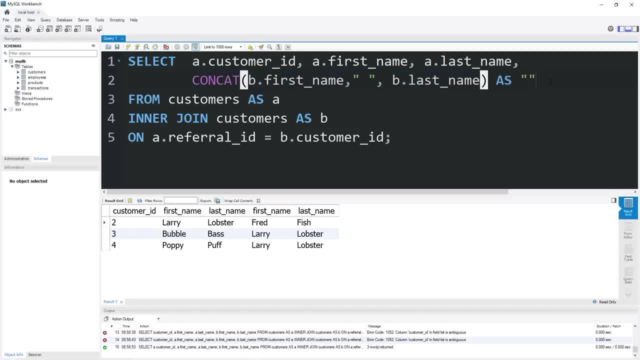 I'm going to give this column an alias, as referred by. All right, there's our table. We have all of our customers who were referred by another customer. Larry Lobster was referred by Fred Fish. Bubble Bass and Poppy Puff were both referred by Larry Lobster. 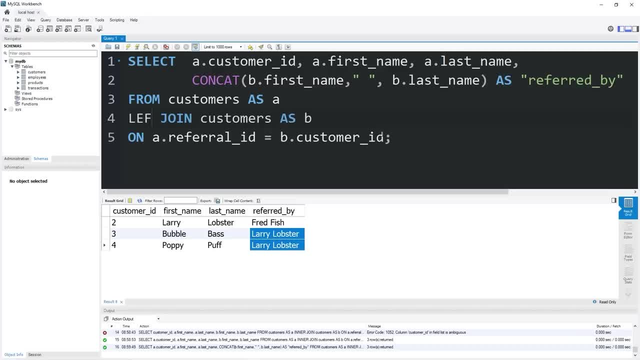 You could use a different type of join. besides an inner join, We could use a left join. What we're telling MySQL is to display all of our customers on the left table. If one of these customers was referred by another customer, join those rows as well. 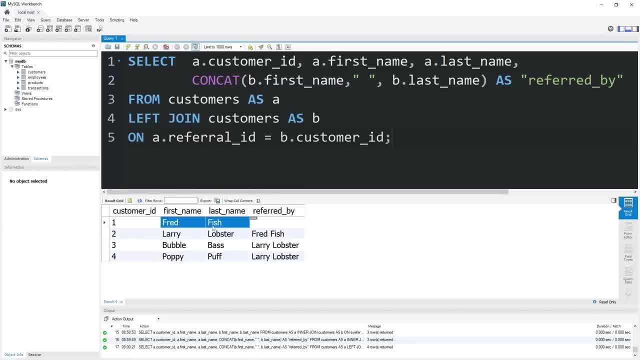 You can see that with the left join that Fred Fish is still within our table, but he wasn't referred by anybody. That value is null. So that's one example of a self-join. We're creating another copy of the same table. 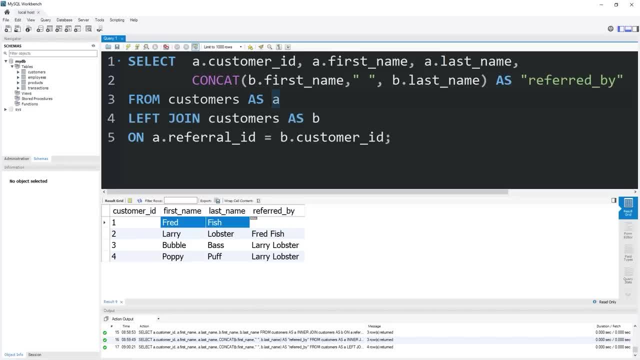 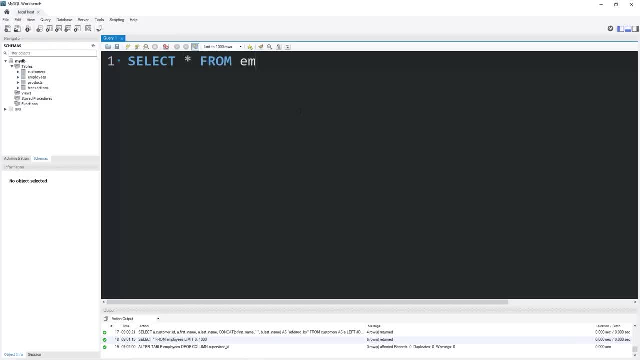 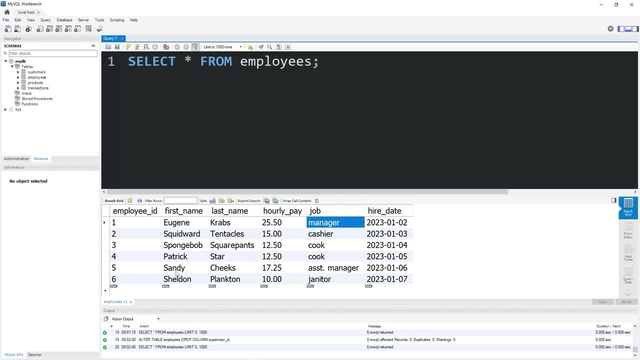 then joining it together to the original, But you'll need to give each table an alias, a unique nickname. Here's another example of a self-join: Let's select all from our employees table. In our employees table, Mr Krabs is a manager. 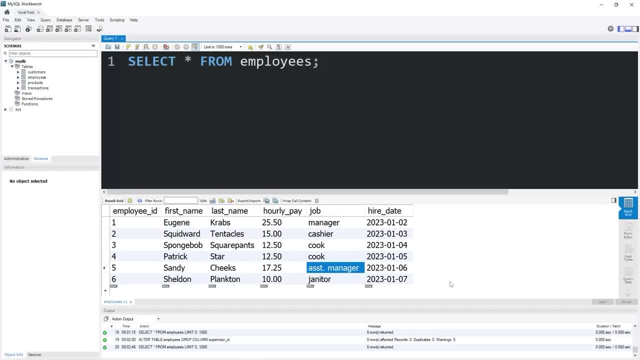 Sandy Cheeks is an assistant manager. Let's add an additional column named Supervisor ID. To who does each of these employees report to? Squidward, SpongeBob and Patrick and Sheldon. they will all report to Sandy, who's an assistant manager. 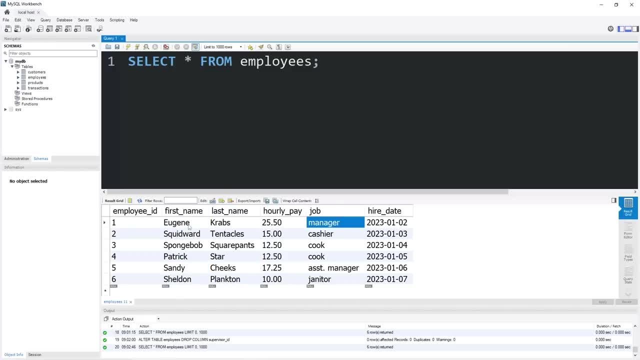 Sandy will report to Mr Krabs. He's the main manager And Mr Krabs doesn't report to anybody. Let's add another column: Alter table employees. add Supervisor ID. The data type is int And there's our new column. 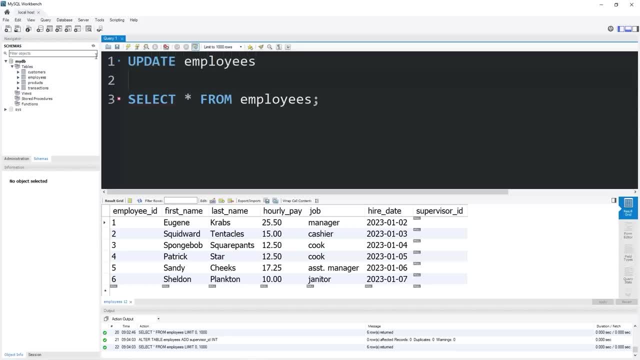 Update employees. Set Supervisor ID equal to five, That would be Sandy. She's the assistant manager. Where employee ID equals two, That would be Squidward. That would be Sandy. Squidward is now supervised by Sandy. 3, that's for SpongeBob. 4 is Patrick. 6 is Sheldon Plankton. 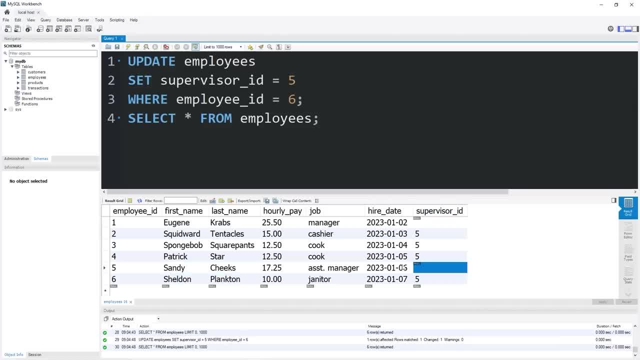 Now Sandy, her supervisor ID is going to be 1,. she is supervised by Mr Krabs. Set supervisor ID equal to 1, where employee ID equals 5.. And here we are Using a self-join. we are going to display the first and last names of all of our employees. 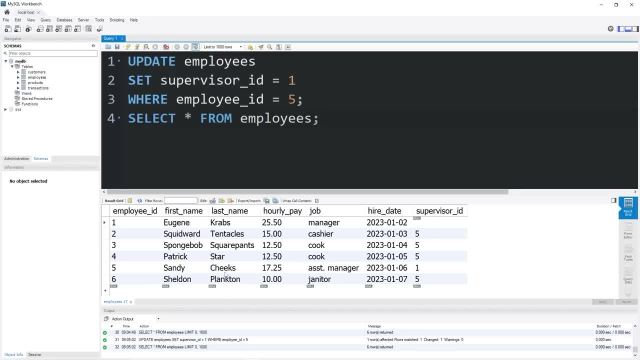 along with the full name of the person that's supervising them. because currently we only have supervisor ID, Let's utilize a self-join First. let's select all from our table employees. We'll need to give this table an alias as a. that's the original. 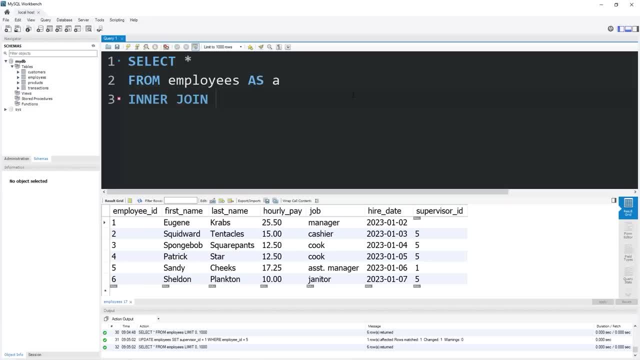 Let's do an inner join. Inner join Employees as B. B will be the copy. How are we going to link these On? the supervisor ID of table A equals the employee ID of table B. All right, we still have one massive table. 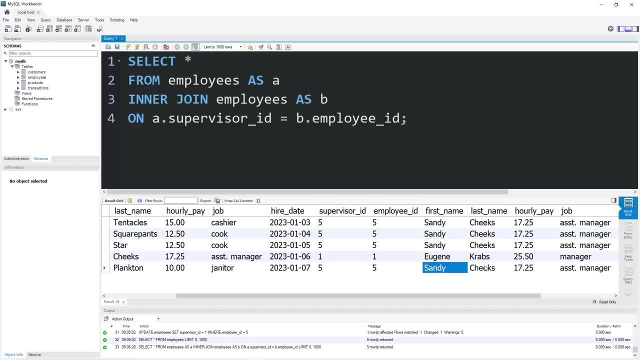 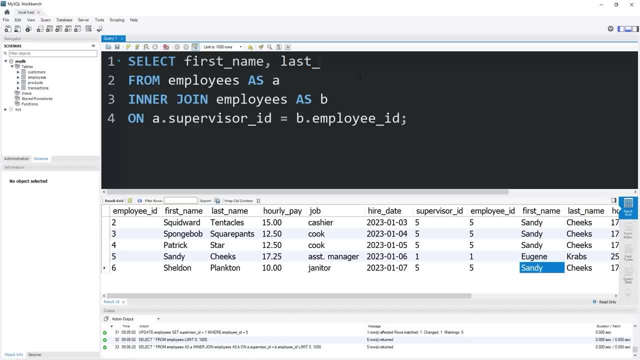 but we can see here that Sandy appears in multiple rows, which is a good start. We don't necessarily need all of this. Let's select the first name and last name of table A: A dot first name. A dot- last name. Then I'm going to concatenate the first and last name of table B. 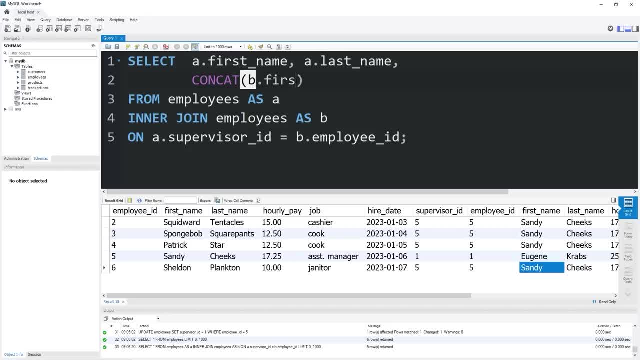 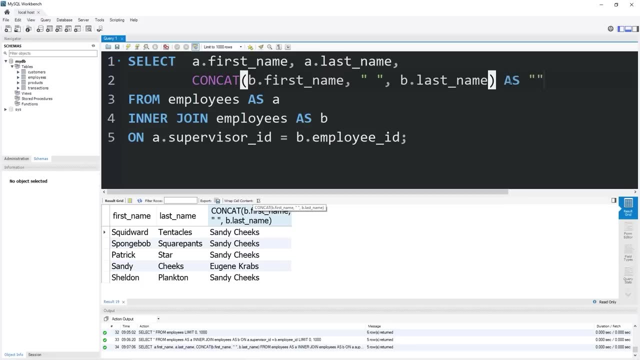 So concat: B dot first name. I'll add a space between the first name and last name. B dot last name. I'm going to give this column an alias. That's really ugly, As reports to. That's much better. All right, we have our hierarchy of data. 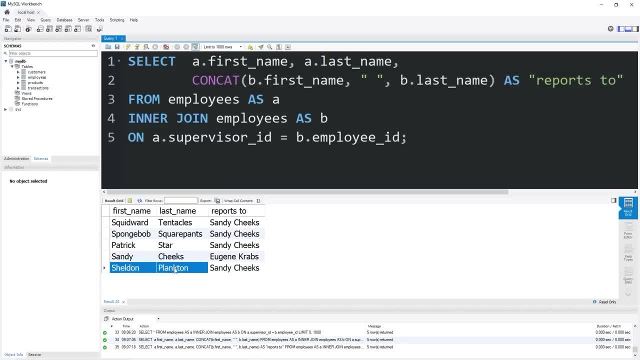 Squidward, SpongeBob Patrick and Sheldon Plankton- they all report to Sandy. Sandy, she reports to Mr Krabs. Then Mr Krabs doesn't report to anybody. If you would like all of your employees. 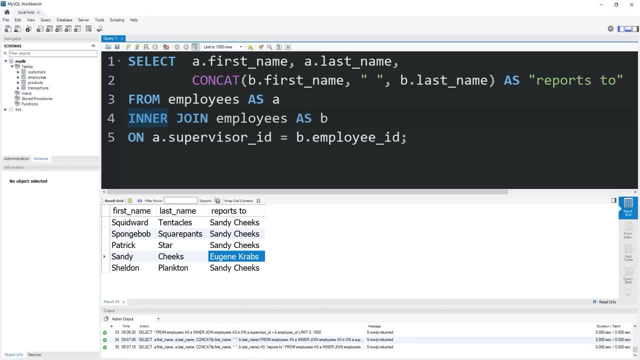 even if they don't report to anybody. you could instead use a left join. because a left join, we will display all of the rows from our table on the left. So Eugene Krabs is here, but he doesn't report to anybody. 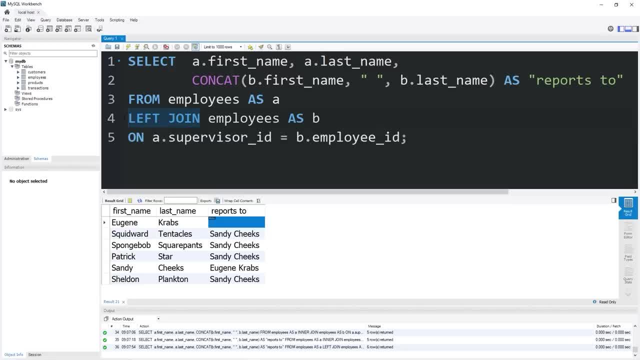 So yeah, basically speaking, that's a self join. You can use any type of join, but the tables you use are the same one. You use the original table, then a copy of that table, but you'll need to give them an alias to distinguish them. 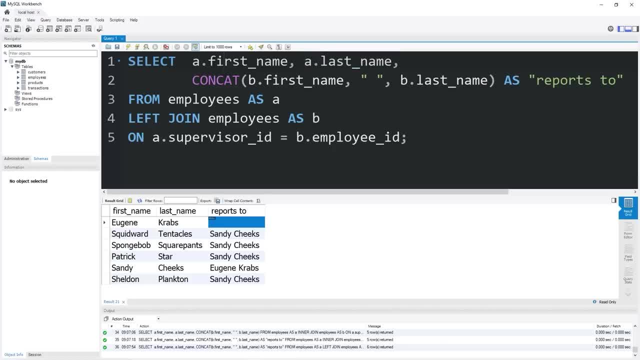 When we're selecting the first and last names of our tables, are we referring to the original table, which I named as A, or the copy, Because that makes a difference With self joins? they're great if you ever need to display a hierarchy of data. 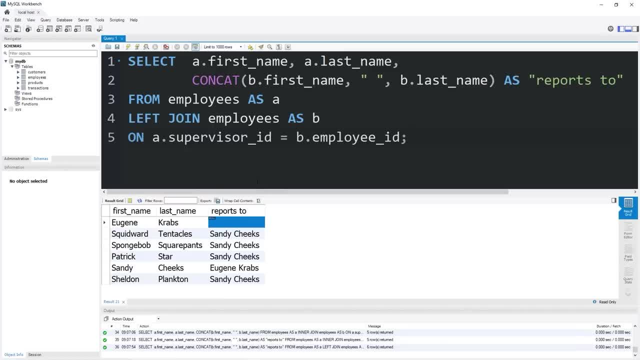 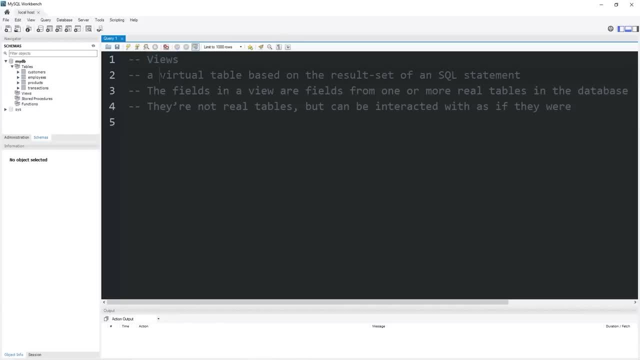 involving the same table. But yeah, that is a self join in MySQL. Hey everybody, today I'm going to be explaining views. Views, they're virtual tables. They're not real. They're made up of fields and columns from one or more real tables. 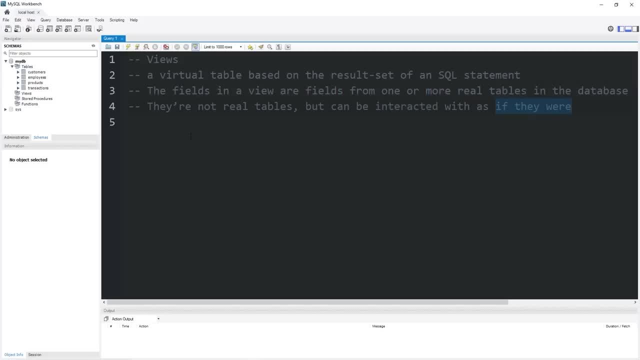 and they can be interacted with as if they were a real table. So here's an example. I'm going to select all fields from my employees table, Our boss, Mr Krabs. he would like us to create an employee attendance sheet. 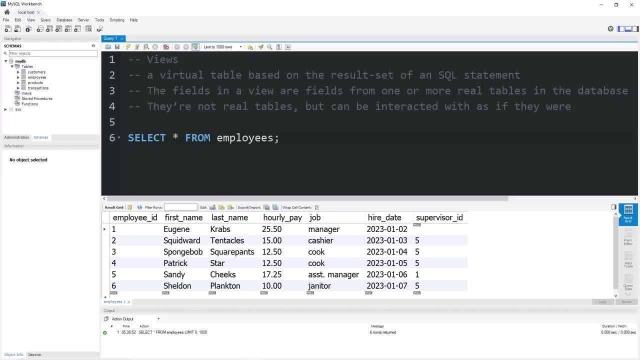 made up of just the first and last names of all the employees. Well, I could create a view that is made from the first and last name columns of the employees table. Now, a view isn't a real table, but it can behave as if it were. 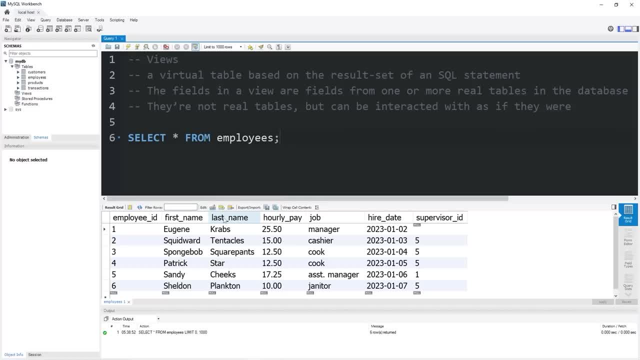 I may want to create a view of the employee first and last names instead of another table, because we try not to repeat data if we don't have to. If I had two tables, one of employees and another of employee attendance, if I need to remove an employee, 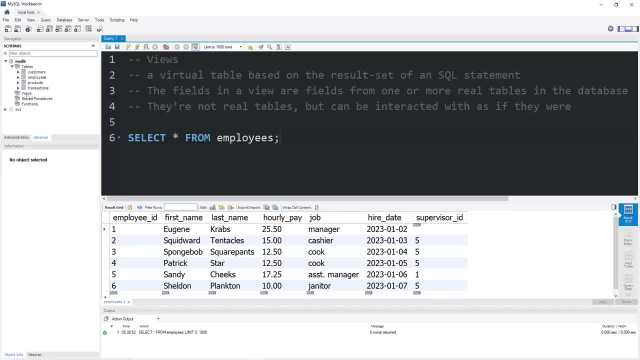 I would need to do so in two places. With a view, it's always up to date. Any changes to one or more of these real tables will also update the view. So let's create a view of the first and last name of our employees table. 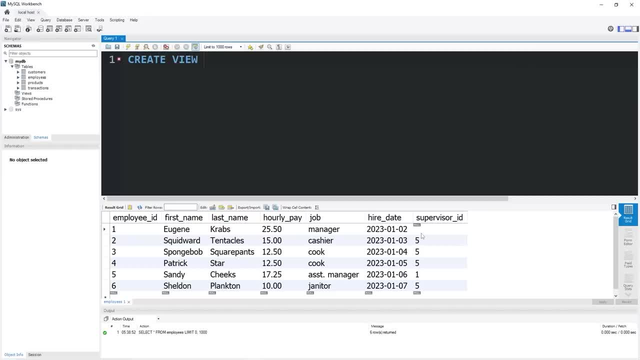 To create a view, you would type create view, then the name of the view, Let's say employee attendance. then, as I'm going to zoom in a little bit, what would we like to select? Let's select first name, last name from a real table. 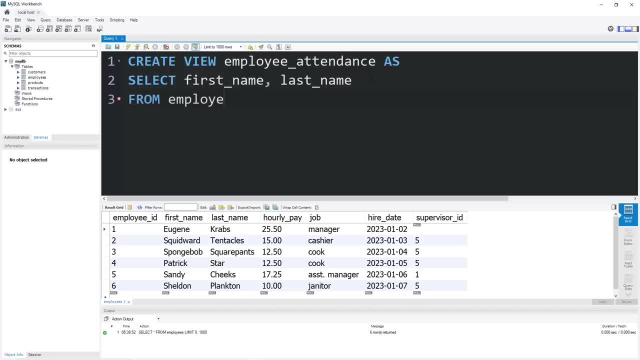 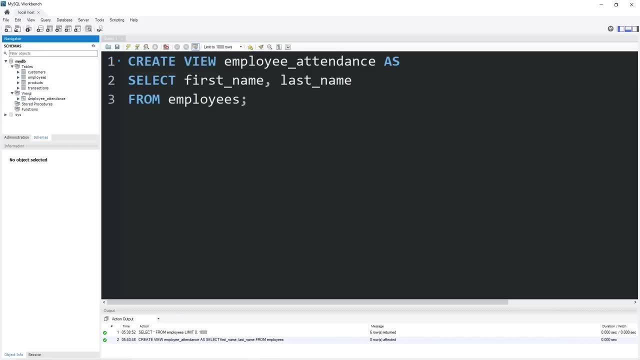 Let's say, from employees. So everything was successful. Let's refresh our schemas window. Underneath the views category we have a new view: Employee attendance. I'm going to select all from that view name- Employee attendance- And let's see what we got. 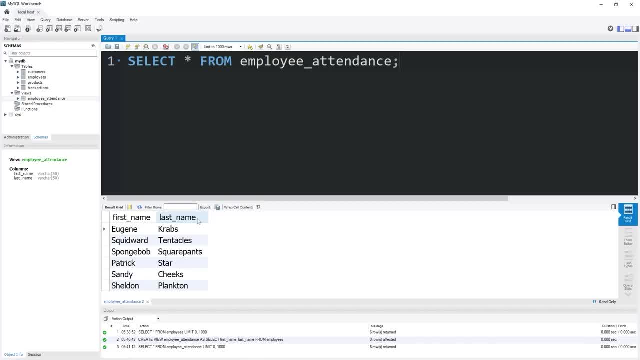 Yeah, here's our attendance sheet. We have the first and last name columns from the employees table. This view can be interacted with as if it were a real table. I will add order by last name ascending. You can use keywords and operators. 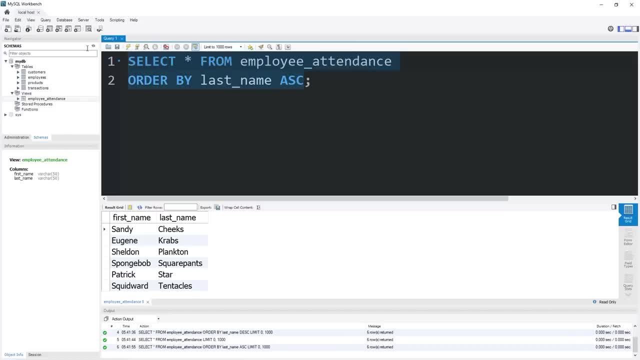 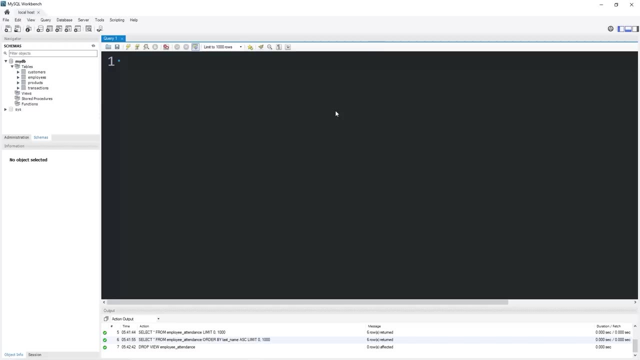 that we've learned about in previous lessons. on a view, To drop a view, you would type drop view- the name of the view- Employee attendance- And it's gone. Alright, here's another example. So views, they're always up to date, right. 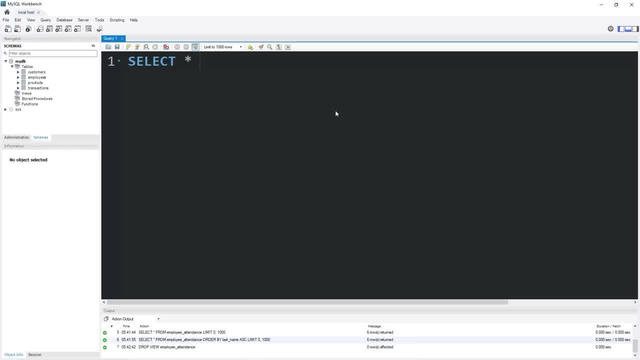 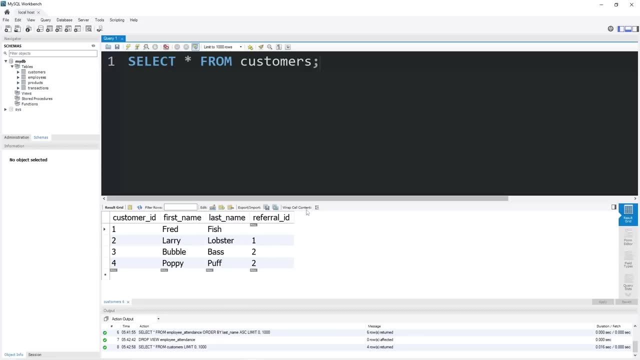 Let's create a view of customer emails, Select all from customers. Let's take a look to see what we have so far. I'm going to add one more column, A column of customer emails. Alter table customers. add column. email data type will be: 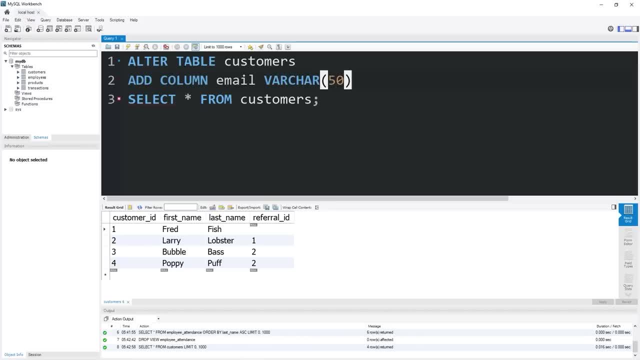 varchar. I think varchar 50 should be enough space. And there's our new column. Let's update these rows, update customers. set email equal to The first email will be for Fred Fish. f fish at gmailcom. Then we'll need a where clause. 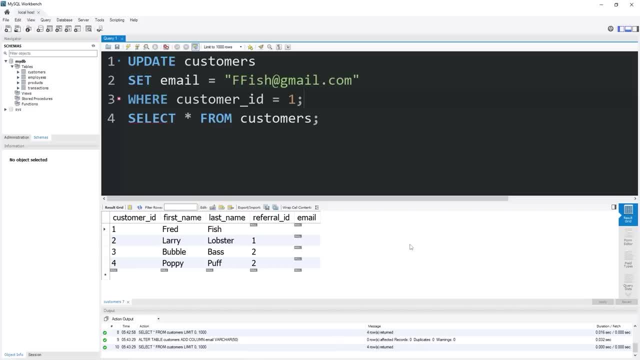 where customer id equals 1.. That's our first email Customer id. 2 will be l lobster at gmailcom. 3 is b bass at gmailcom. 4 will be p puff at gmailcom. Everybody really likes Gmail. I guess Let's create a view from these customers. 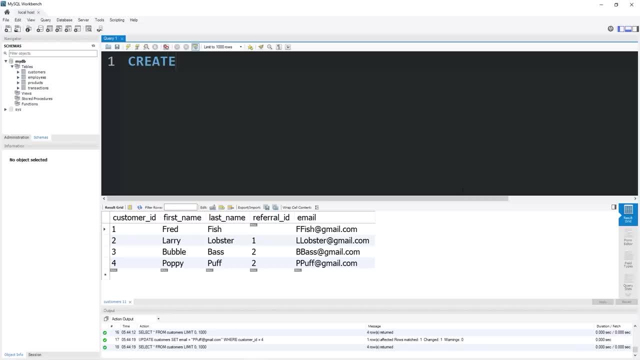 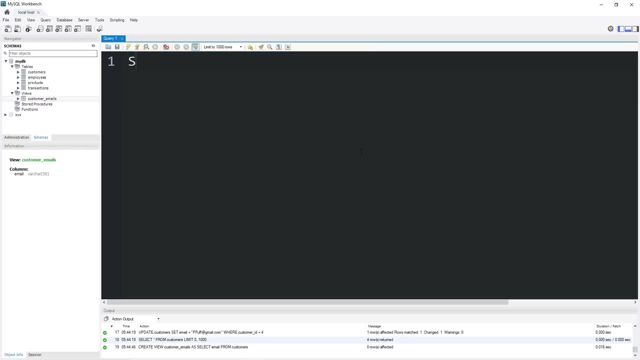 Create a view from these customer emails. Create view customer emails as. what are we selecting? Let's select the email column from our customers table. Let's refresh our schemas window. Yeah, we have a customer emails view. Then I will select all from customer emails. 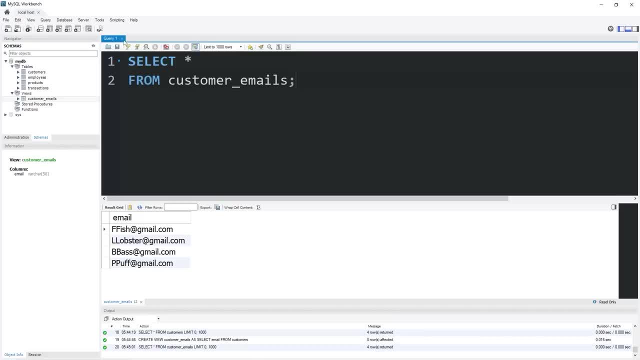 Customer emails And look at that, We have a listing of all the customer emails And we're going to spam these people with coupons or something I don't know. When you update one or more of the real tables in your database, those views would reflect any changes. 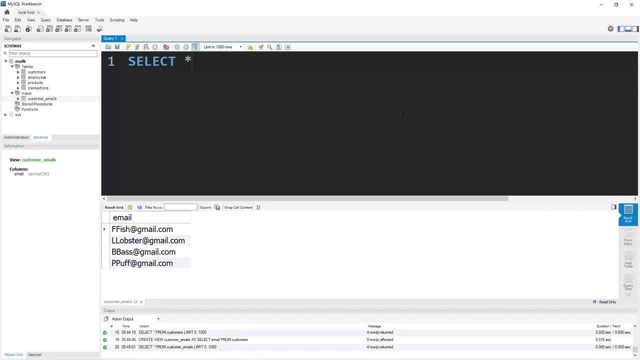 Let's add one more customer. So let's take a look at our customers table. Select all from customers. Let's add one more customer. Insert into our customers table Some values. We have five columns. A customer ID, First name. 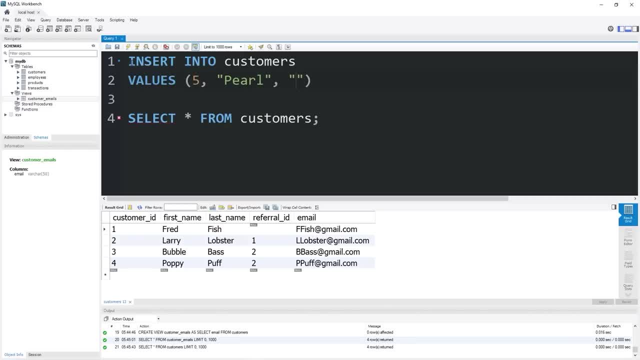 First name will be Pearl. Last name is Krabs. Referral ID: Let's say null. Email will be p krabs at gmailcom. Okay, there's our new customer. Let's take a look at our view. Let's see if it updated. 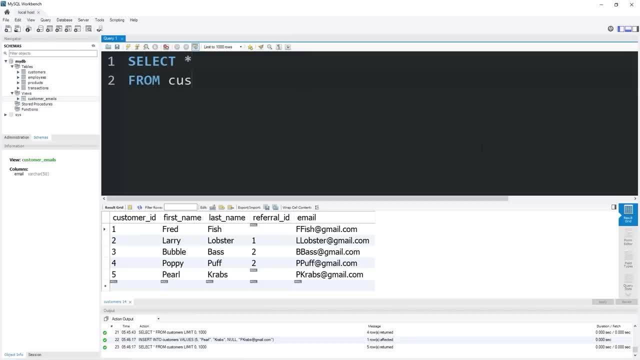 Select all from customer emails. Yeah, look at that, It's up to date. That is one of the benefits of a view. It will update automatically. because we're using components from real tables, Any views that use that data will also be updated. 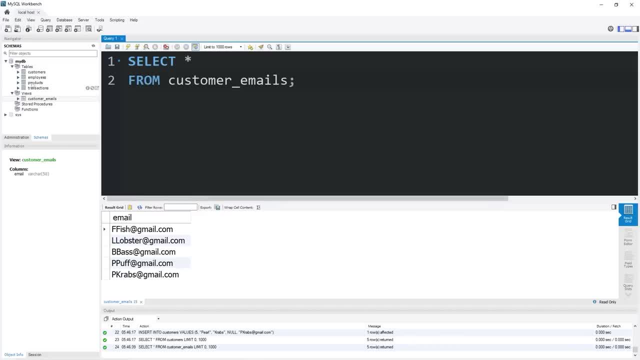 The other benefit of a view is that we don't have to repeat data in a real table. Ideally, we'd only want to make a change in one place rather than across the table. All right, that's a view everybody. A view is a virtual table based on the results of an SQL statement. 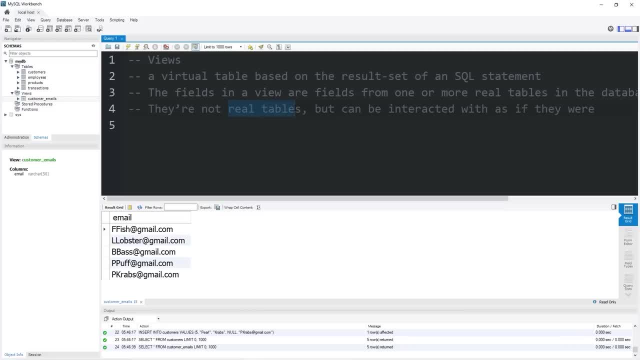 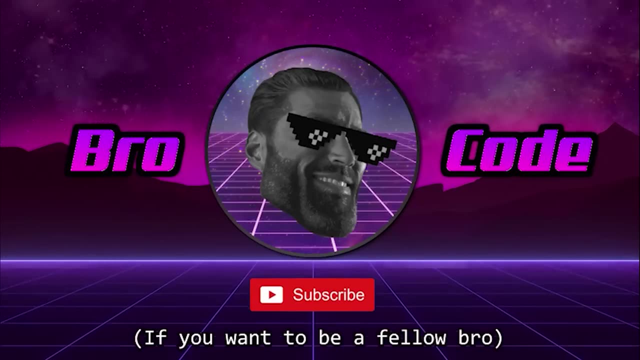 They're not real tables, but they can be interacted with as if they were real. The fields found within a view are fields from one or more real tables in the database. So, yeah, those are views in MySQL. Yeah, it's me again. 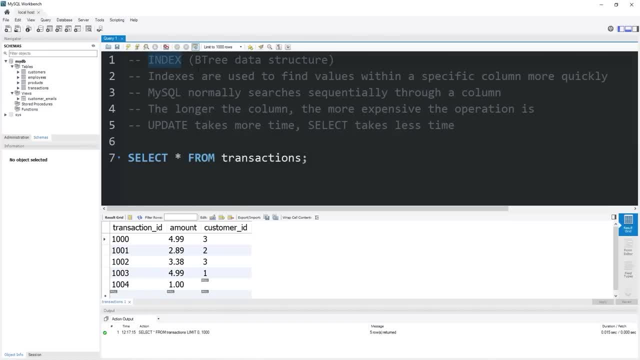 And in today's video I need to explain what indexes are in MySQL. An index is the number of rows in a table. An index is the number of rows in a table. An index is a type of data structure. They are used to find values within a specific. 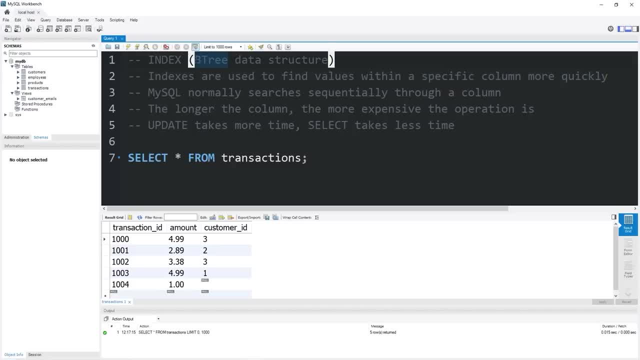 column more quickly. It's technically a B-tree data structure, if you're familiar with what that is, but if you don't, don't worry about it. MySQL normally performs searches sequentially through a column. If I'm looking for some specific value, just scan each value on the way down to see. 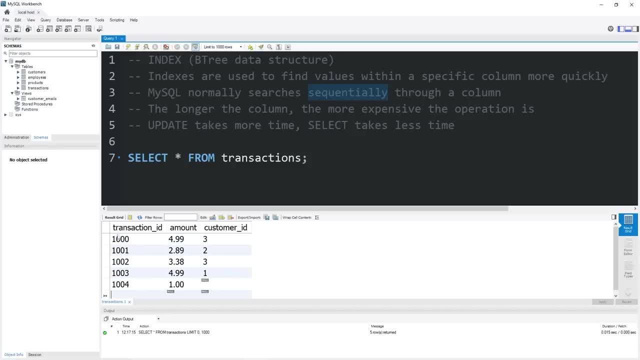 if those values match, depending on what I'm looking for, It doesn't really take much time if you have a small dataset, like I do. but imagine if you have millions of transactions. Searching each transaction one by one is gonna take a long time. We can speed up that process. 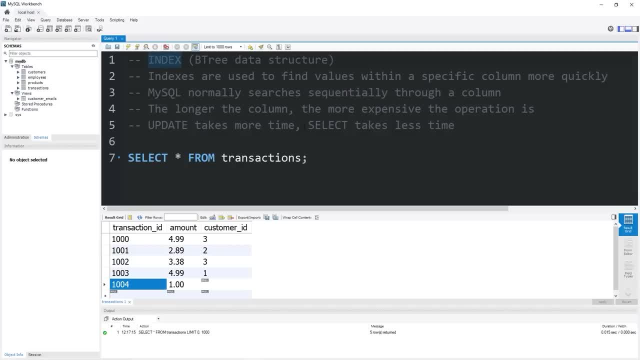 by using an index. By applying an index to a column, selecting or searching takes less time. However, updating takes a lot more time. So there's some pros and cons with using an index. It really depends on the table. If I'm working with a table of transactions, 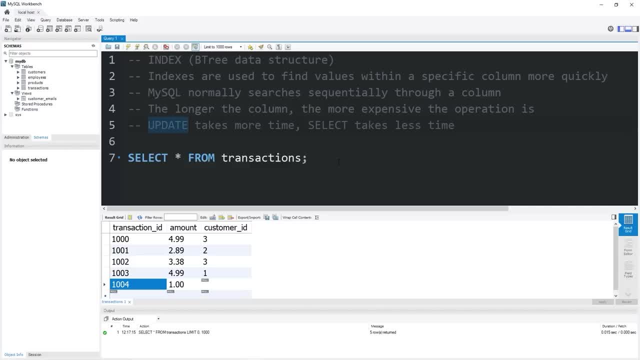 transactions are being updated all the time. People are constantly making purchases. I don't think our transactions table would be a good candidate for an index. We'll be doing a lot of updating but not a lot of searching. However, with our customers table, I think our customers table could benefit. We don't update our customers. 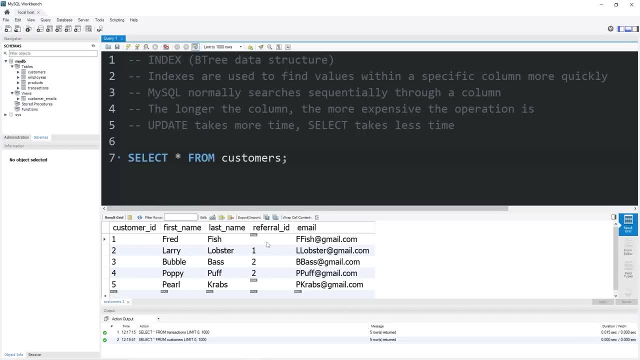 table. very often, Only a new customer comes in every once in a while. Let's reduce the time it takes to search for a customer With creating an index. how exactly do we want to find the customer? Believe it or not? we do have an index with our customer ID already. 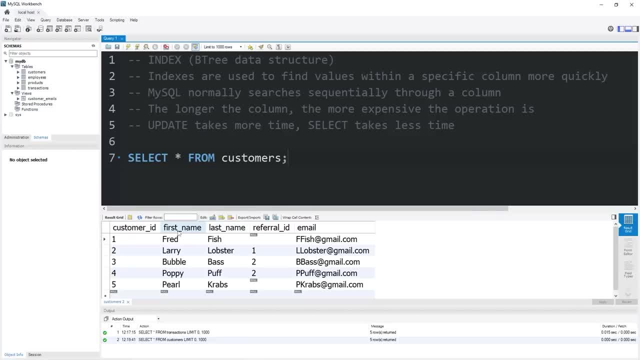 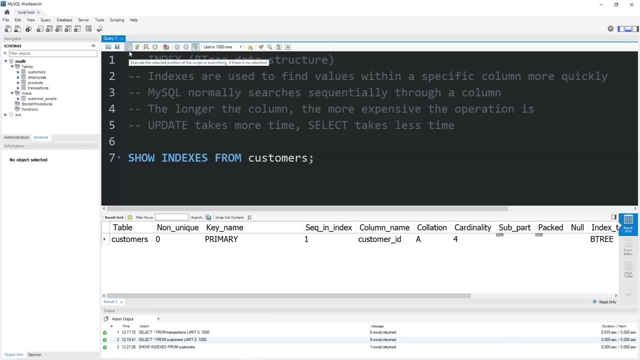 A customer may give you their last name and or first name. Let's create an index for these. We'll start with last name, though To show the current indexes of a table, you would type: show indexes from the name of the table. Here are the current indexes for our customers table. 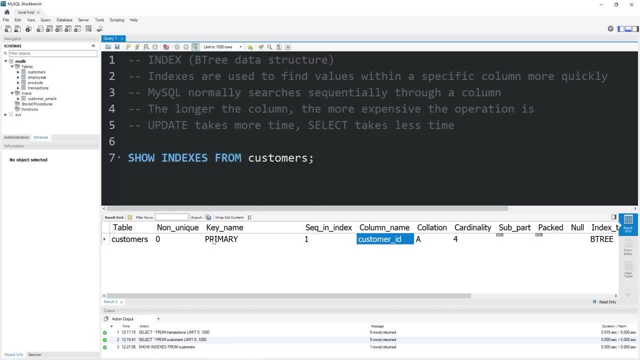 We do have one already, and that's for our customer ID. That is the primary key. We can search for a customer by their customer ID fairly quickly, but not so much by their last name or their first name. Let's apply an index to those columns. 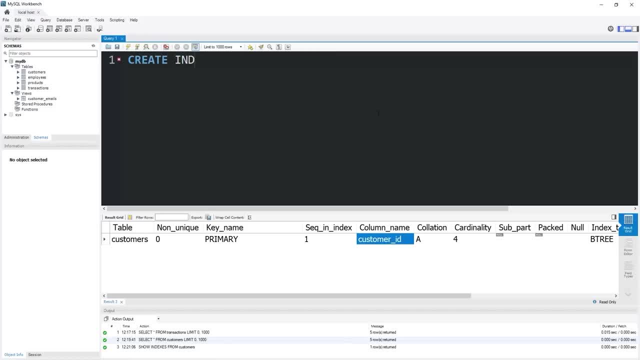 To create an index. you would type create index, then a name. I will apply an index to our last name column. I will name this index Last name, IDX, meaning index On the table, customers in this case. then list a column. I will apply an index to our last name. We will be doing a lot of. 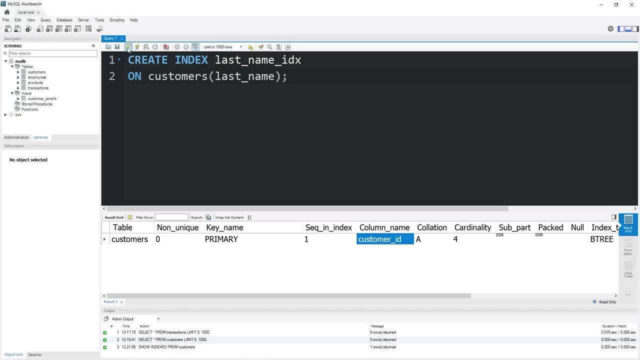 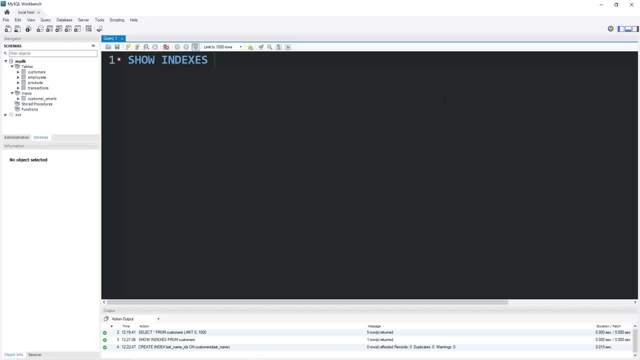 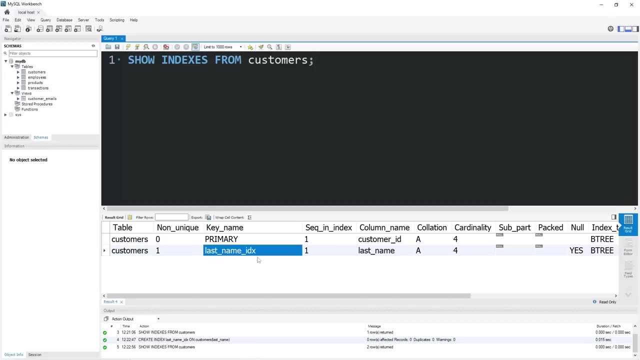 searching by a customer's last name. So I might as well apply an index. So let's execute the statement. Let's show our indexes again, Show indexes from customers. And here is our new index: last name index. It's applied to our column last name. If I were to search for a customer by last 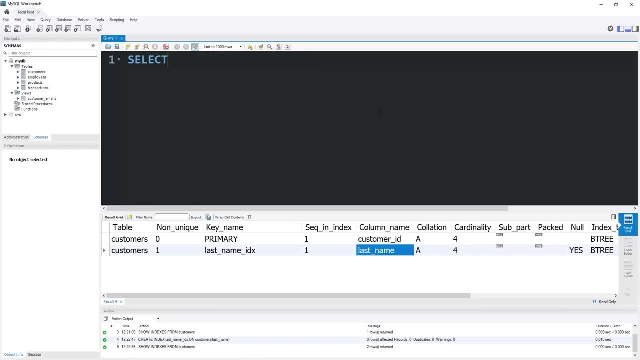 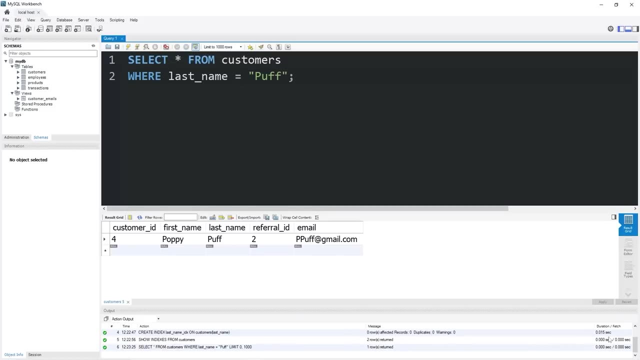 name, that process will be sped up. now. Select all from customers where last name is equal to puff. So my data set is already very small. to begin with, There's not going to be a noticeable difference in this example, but if I'm working with a million customers, using an index would. 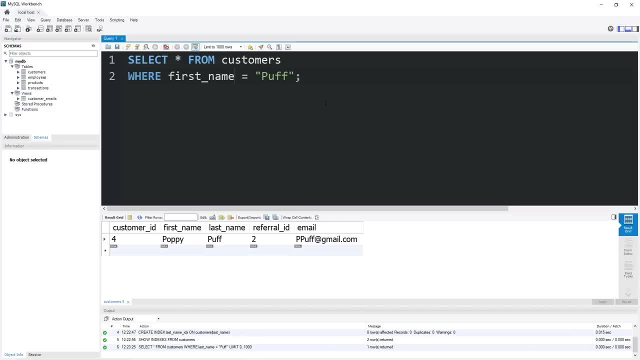 be a lot faster If I were to search by first name instead, where first name equals poppy. uh, I spelt poppy wrong. Well, we don't have an index applied to our first name. As of now, it would be slower to search for a customer by their first name compared to their last name. 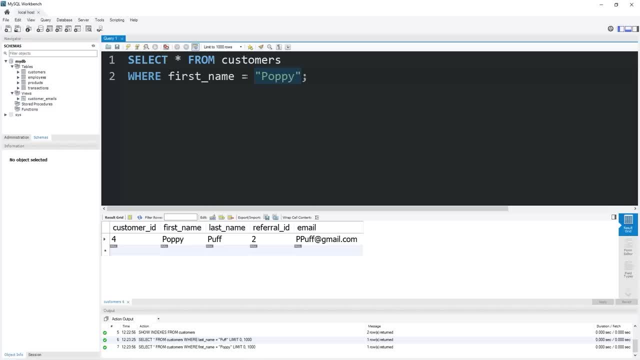 That first name doesn't have an index. Realistically, we wouldn't search for a customer just by their first name. We would do a last name or a last name and a first name. That's where multi-column indexes come in. To create a multi-column index, you would type: 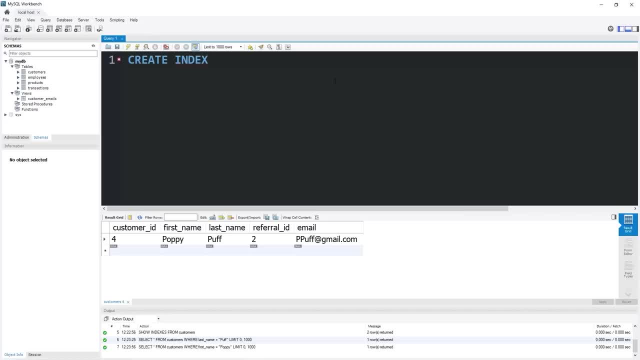 create index a unique name, let's say last name, first name, IDX on our table. customers then list the columns in order. The order is very important. MySQL has what's known as a leftmost prefix with indexes, So we will search by last name, then first name. 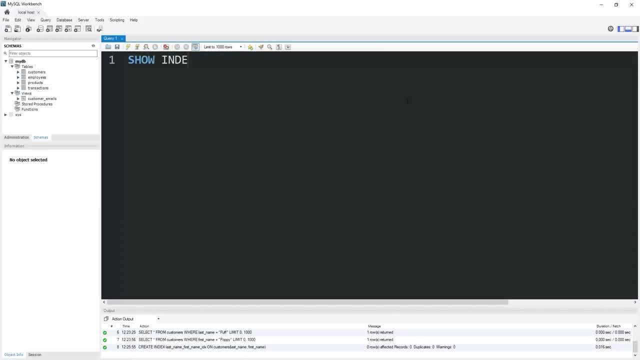 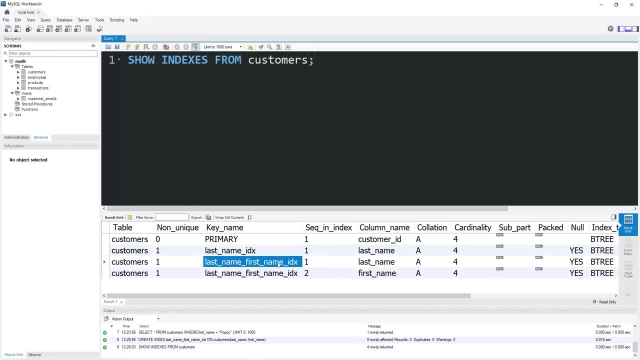 Let's execute the statement: show our index indexes. show indexes from customers. Here's our last name. first name index. There's a sequence. We're telling MySQL to search by a last name. However, if there's also a first name, include that too. There needs to be a last name to utilize this index. 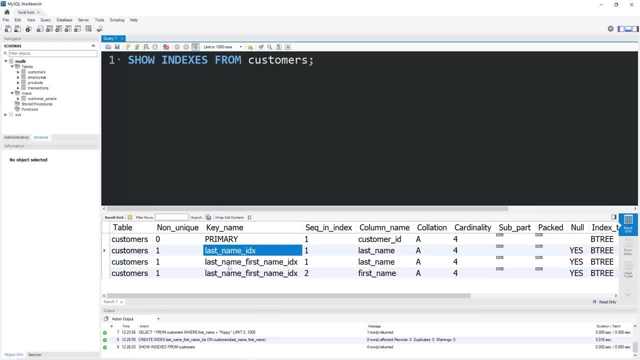 If I want to, I can get rid of this last name index, because our last name first name index would do the same thing. We can search for a last name as well as a first name index would do the same thing. We can search for a last name as well as a first name. 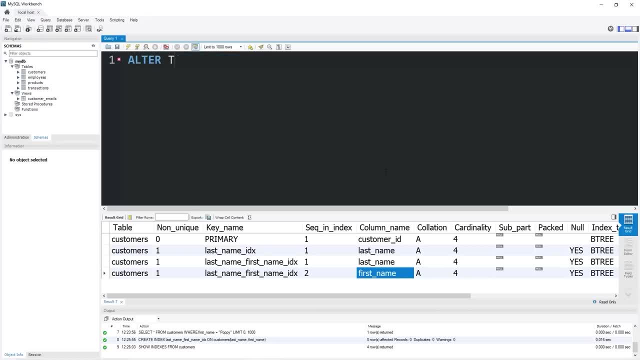 If we would like to drop an index, you would type: alter table: the name of the table. drop index: the name of the index, last name index. Then I'm going to go ahead and show indexes from customers And the last name index is gone. 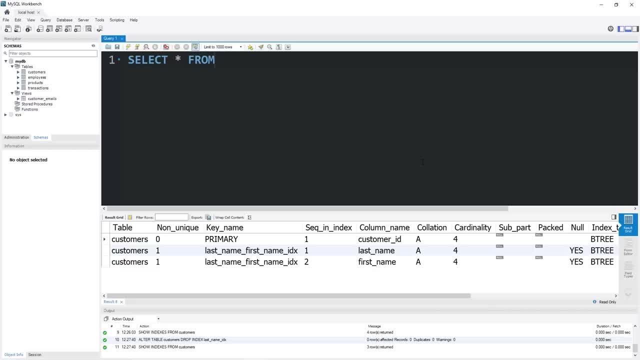 Now, if I was to search for a customer- select all from customers Where, if I were to search for a last name, we would benefit by using this multi-column index. If I looked for a last name and a first name, we would also benefit. 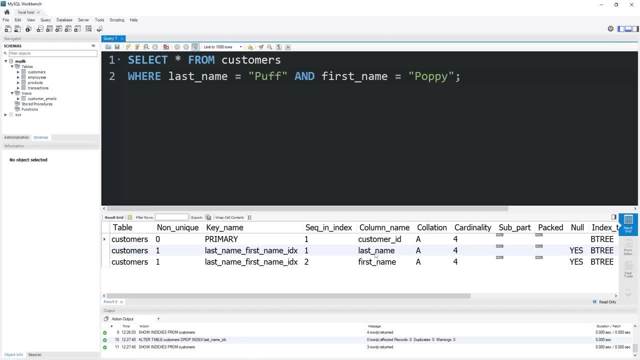 There's a sequence. We would search through any last names first because that's first in the sequence, But if I was to search for just a first name, we would not utilize this index. Well, everybody that's an index. It's a type of data structure that is used to find values more quickly within a specific column. MySQL normally searches through a column sequentially. The longer the column, the more expensive the operation is going to be. If you were to apply an index to a column, searching and selecting a value takes less time, But updating that table takes longer. Use it if you think a table is a good candidate where you don't update it very often. 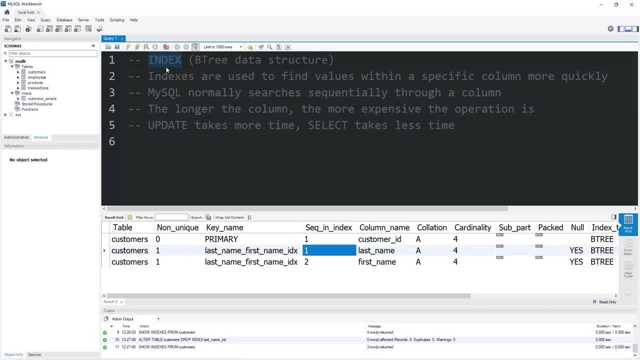 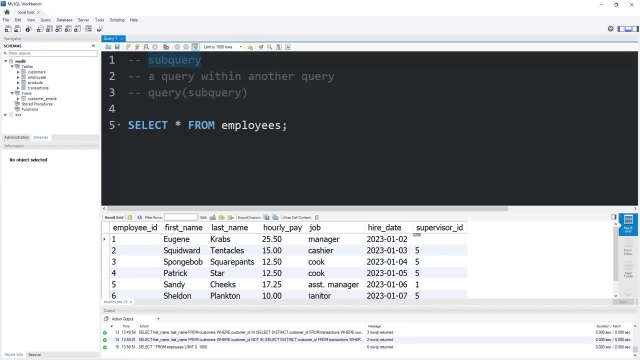 And well, yeah, those are indexes in MySQL. Well, hello again everybody. Today I need to explain subqueries. They can be pretty complicated, but I'll try my best to explain it simply. A subquery is just a query within another query. 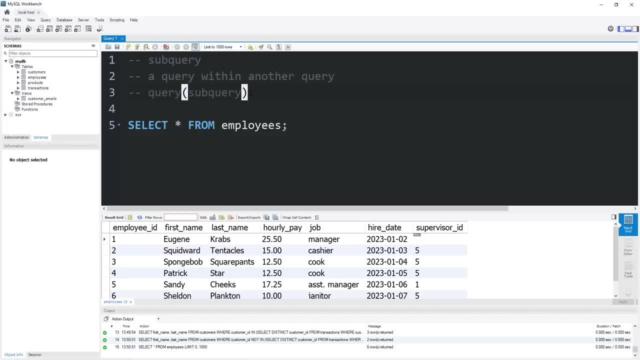 You write a query and close it within a set of parentheses. Whatever value or values are returned from the subquery you would use within an outer query. I'll give you a few demonstrations. I have an employees table- Our manager, Mr Krabs. he needs us to compare every employee's hourly pay. 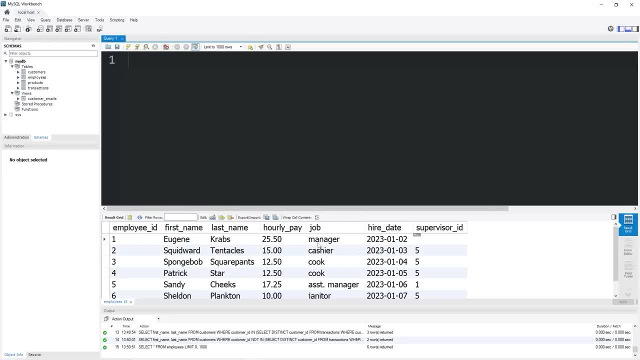 With the average hourly pay of our employees table. Maybe Mr Krabs is going to give people a pay reduction, Not an increase, a pay reduction- But he needs to compare the hourly pay of every employee versus the average. How can we write something like that? 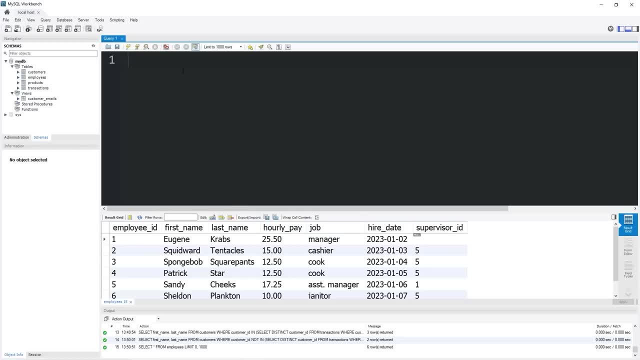 A task like that, I would say, involves at least two steps. We need to find the average hourly pay first, And then display every employee's first name, last name, hourly pay, Then the average pay. Let's begin with the average pay. 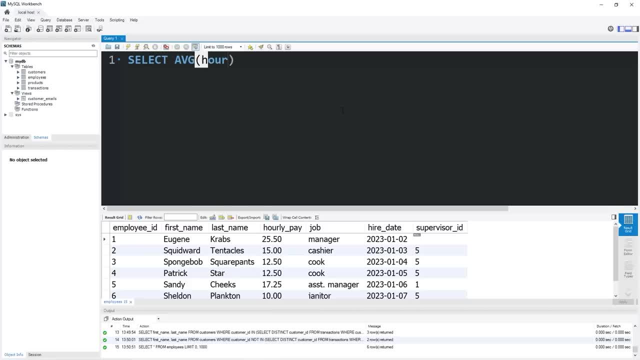 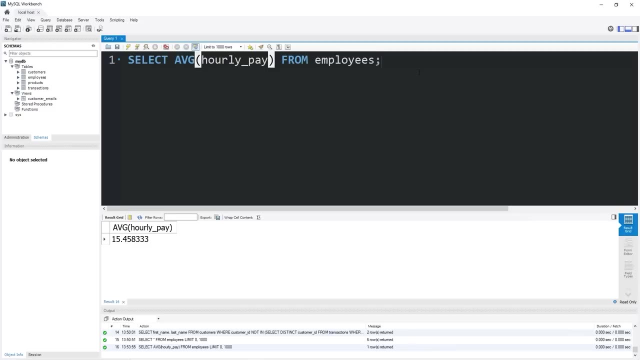 Select Average function Hourly Pay From My employees table. So far, so good. $15.45 is the average hourly pay of an employee. How do I use this number? Whatever value or values are returned from a subquery we can use within a larger outer query. 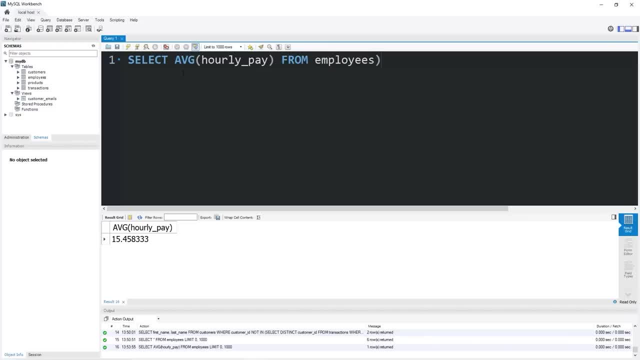 Let's delete this semicolon. I will surround this statement with a set of parentheses. I will then write the outer query. Let's select the first name, last name, the hourly pay, then comma our subquery from employees. There we are. 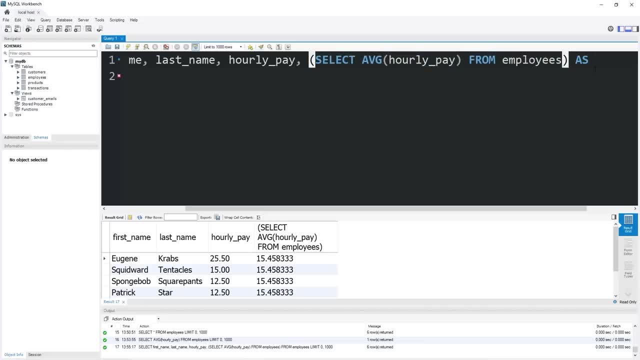 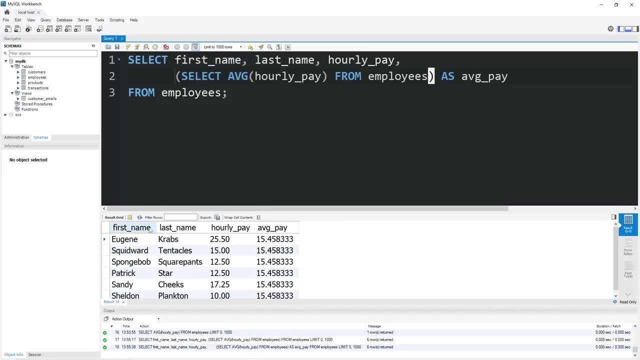 Although I'm going to give the subquery an alias as average pay, And I think I'm going to move this to the next line. That is much better. So We have accomplished our task. We have compared every employee's hourly pay versus the average. 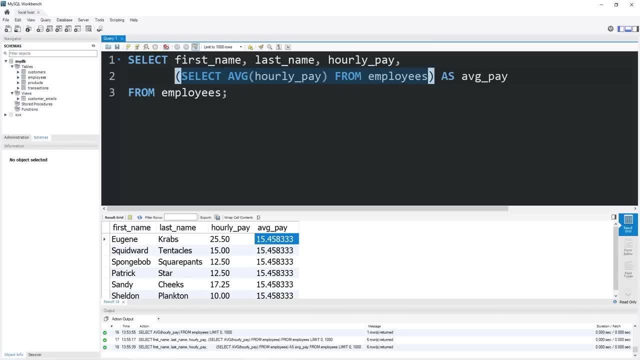 Once we complete the subquery, whatever value or values are returned from the subquery, we would use within the larger picture, the outer query. Just imagine that we replace the subquery with $15.45.. This value is what was returned. 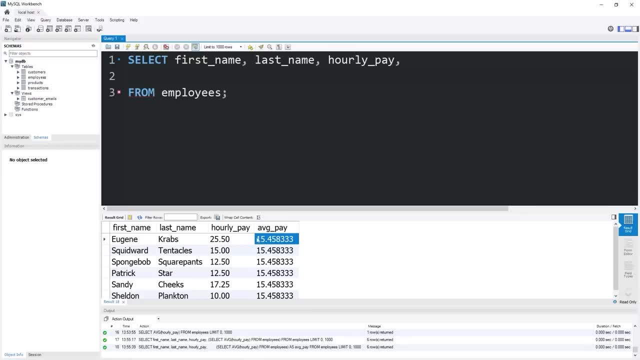 Although you don't want to write a concrete number like this, just because the average pay is bound to change, writing a subquery like this would calculate our average pay regardless if we add or remove employees. Let's try a different example. 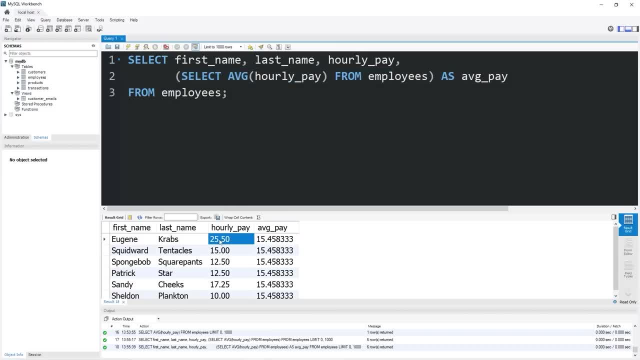 Let's find every employee that has an hourly pay greater than the average pay. So again we can begin with the subquery. We need the average pay, Select average function Hourly pay From employees. So again we return $15.45.. 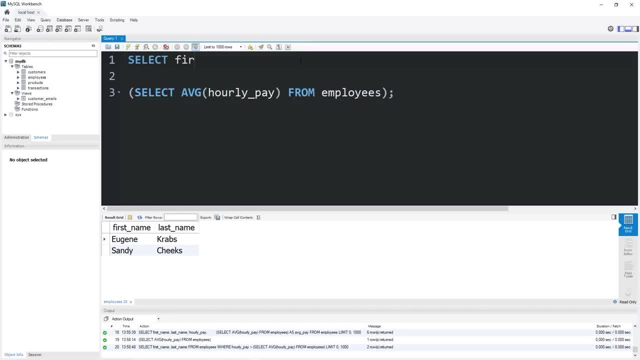 I'll use this within a moment where clause: Let's select the first name, last name, hourly pay from our employees table where the hourly pay is greater than our subquery. Mr Krabs and Sandy Cheeks are both making more than the average hourly pay. What was returned was: 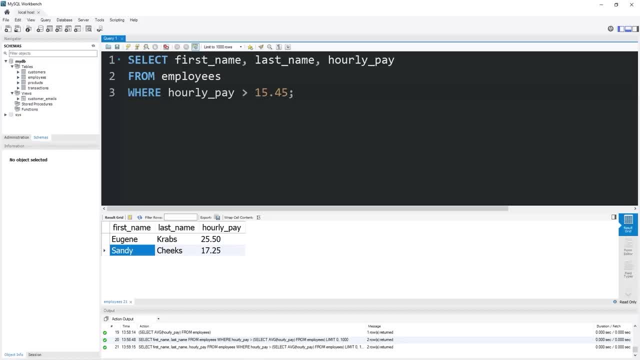 fifteen dollars forty-five cents. Then it's just a matter of completing the outer query. Select the first name, last name, hourly pay from employees where hourly pay is greater than 1545.. It looks complicated, but when you break it down into steps it's a lot easier to visualize. We're going to cover a. 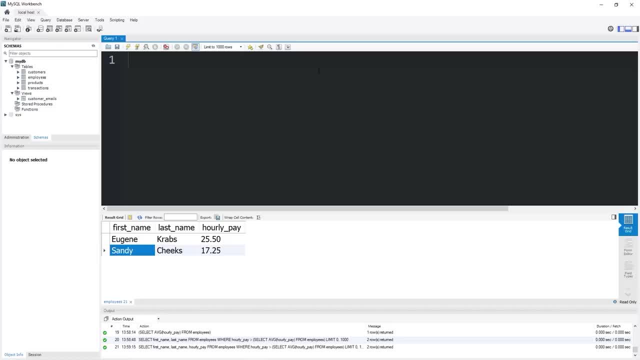 completely different example. We will be working with customers and transactions. I'm going to select all from my transactions table. We have a few transactions. I would like to find the first name and last name of every customer that has ever placed an order. We can do this step-by-step. Let's select. 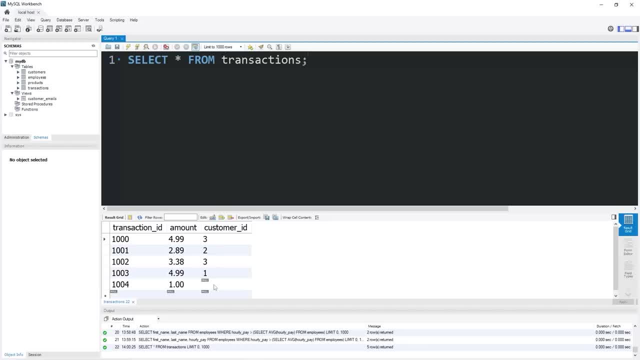 every customer ID from transactions that's not null. Select customer ID from transactions where customer ID is not null. Let's take a look. So we do have a few repeats. We have one, two, three and three. You can add this distinct keyword. if there's any repeats, That would eliminate. 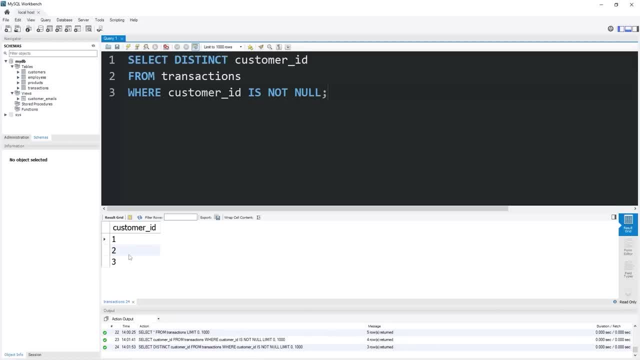 them. We have three registered customers that have placed orders in the past: Customer IDs 1,, 2, and 3.. But we don't know who these customers are. We will use these values within a larger outer query. I will surround this query within a set of parentheses. 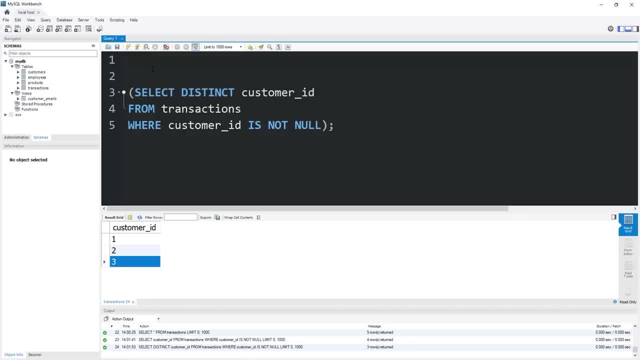 Eventually, we'll use this within aware clause. Let's select the first name and last name from our customers table where customer ID. I will then use the in operator, Then add my sub query. There we are. There's our three customers that have placed orders in the past: Fredfish. 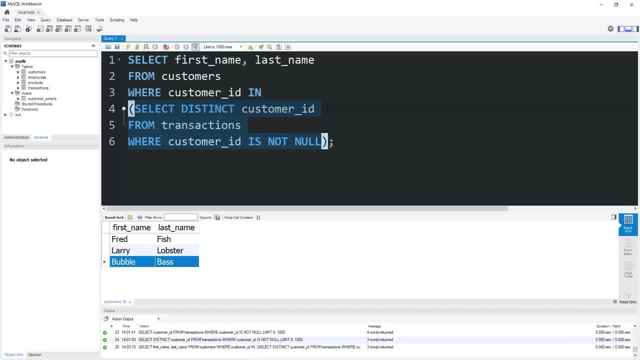 Larry AREa, Lobster Bubble الي. This subquery returned the values 1,, 2, and 3.. Imagine that once this query resolves, we are left with the values 1,, 2, 3.. So this outer query makes a lot more sense. 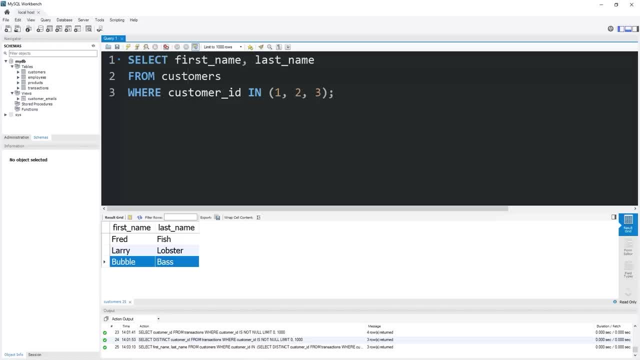 Select the first name and last name from customers where the customer ID is one of these values: 1,, 2, or 3.. You could do the inverse, too: Find the first name and last name of every customer where the customer ID is not in the subquery. 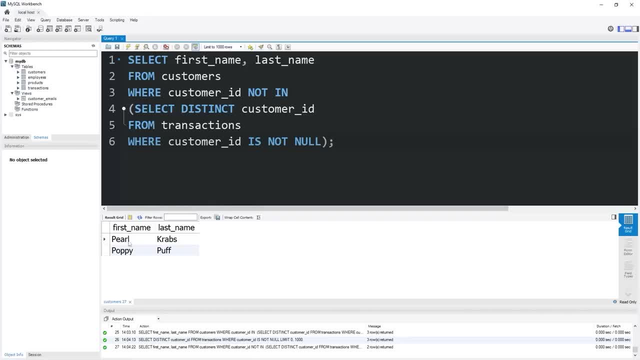 This query would return every customer that has never placed an order. Let's send them a coupon in the mail to convince them to place an order. We were left with values 1,, 2, 3.. Select the first name and last name from any customers where the customer ID is not in one of these values 1,, 2, or 3.. 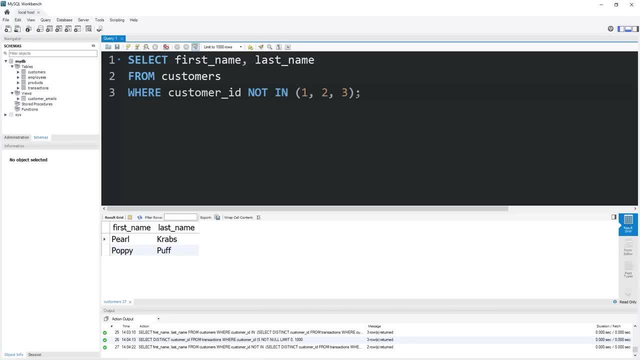 Pearl Crabs had an ID of 5.. Poppy Puffs was 4.. So yeah, that's a subquery, everybody. It's just a query within a larger query. It helps to visualize this step-by-step. Imagine that we're completing the subquery first. 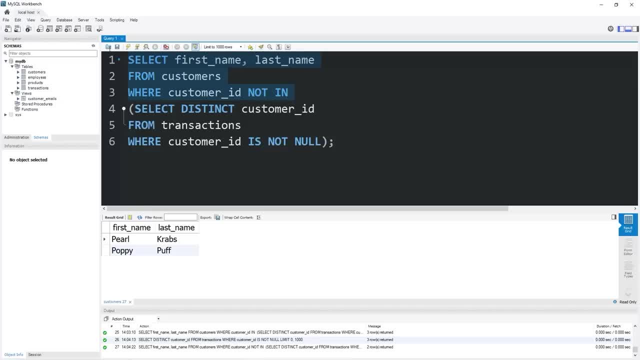 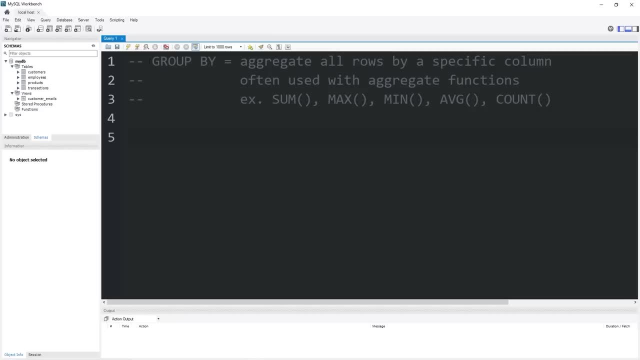 Whatever value or values are returned, we can use within a larger query. And well, yeah, those are subqueries in MySQL. Hello everybody, Today I will be explaining the group by clause. The group by clause will aggregate all rows by a specific column. 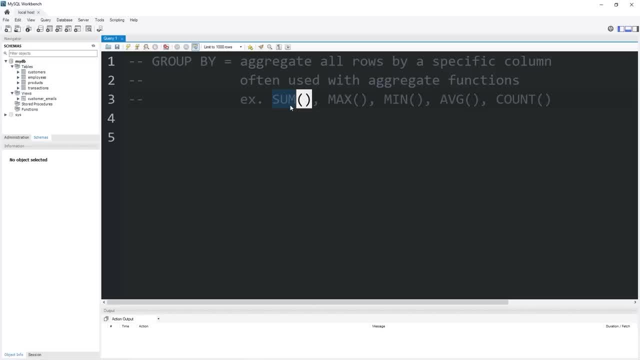 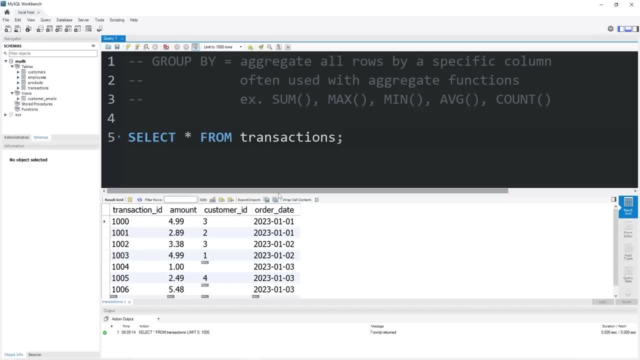 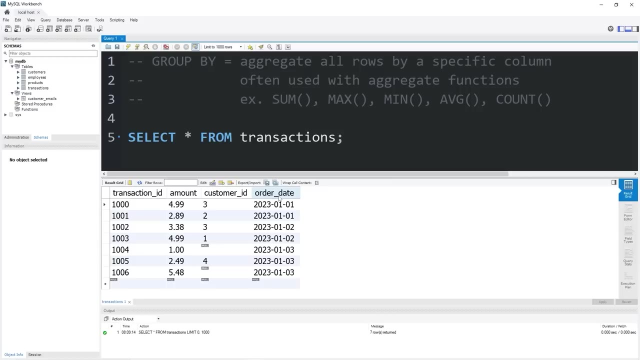 It's often used with aggregate functions such as the sum function, max, min, average count, just to name a few. For my example, I have a table of transactions. Now, if you've been following along in my video series, I did add an additional column named order date and filled in a few dates as well as two additional rows. 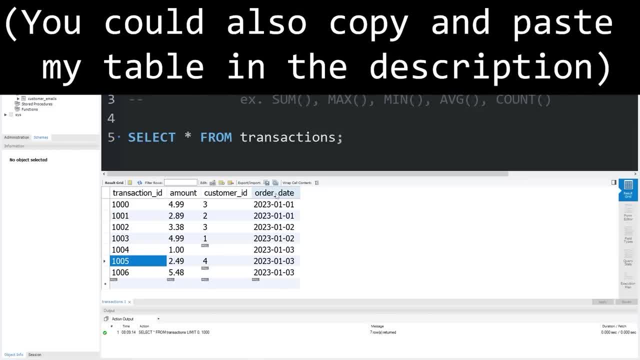 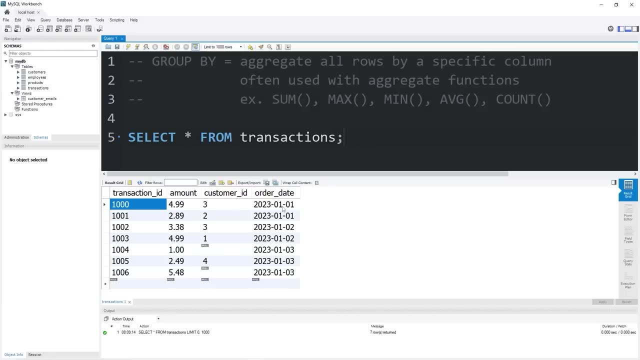 If you would like to follow along, I would recommend pausing the video, Adding a new column for order date. add these order dates, then add two additional rows. That's all the data that we'll need in this topic. Now our boss, Mr Krabs. he needs us to tell him how much money he made per day. 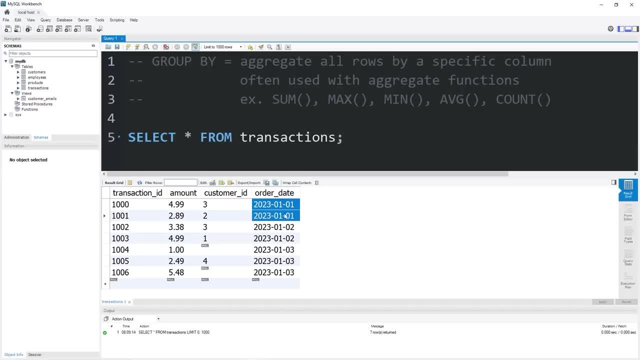 What is the sum of all of the amounts per day? We have three different dates: January 1st, January 2nd, January 3rd. What is the sum of every amount on these days, So we can use the group by clause? 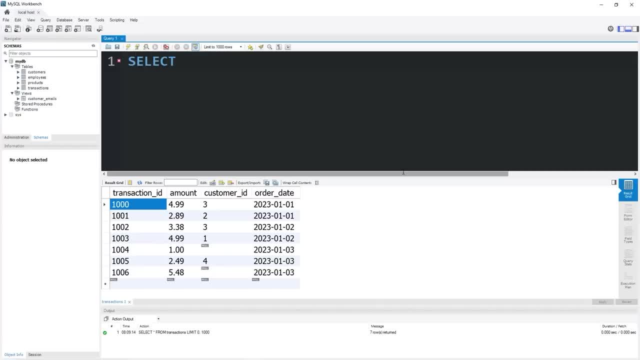 That would help us. We will add a new column for order date. We will select the sum of every amount as a column. We will also display the order date from transactions. Then we will group by. we are grouping by our order date. 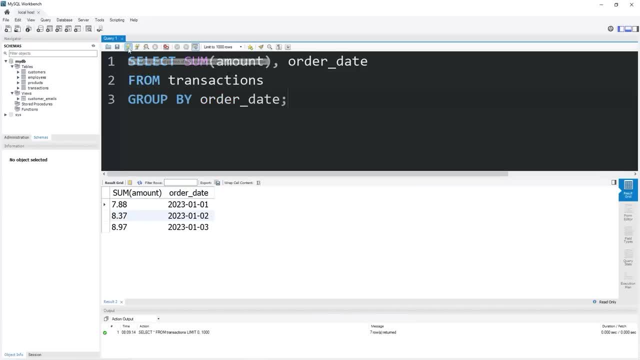 Group by order date column. Yeah, look at that, There we are. Here is the sum of every amount that is grouped by these dates. Here is the total amount we made January 1st. the total amount January 2nd. the total amount January 3rd. 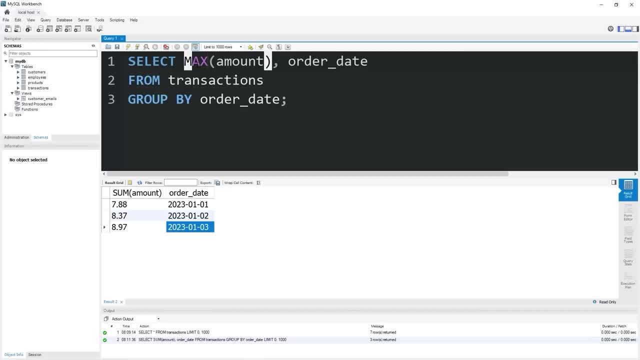 Let's try a different function. How about the max function? What was the maximum amount on each day? These are the maximum transactions that have occurred on these dates. What about min? These are the minimum amounts grouped by order date. What's the average order every day? 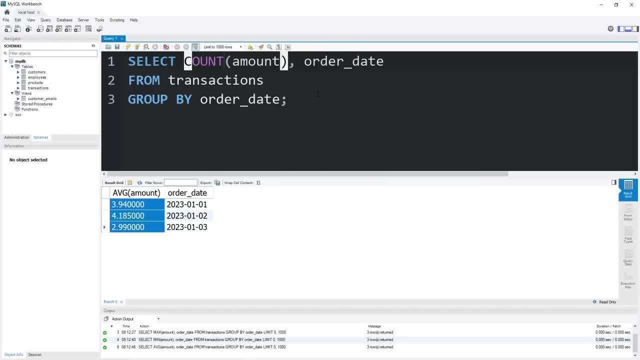 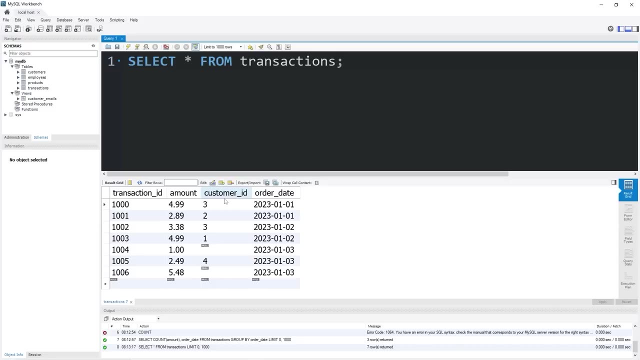 Here are the averages. Maybe count How many transactions have taken place each day. We have two orders on the first, two orders on the second, three orders on the third. Let's try a different column. Let's group by customer ID this time. 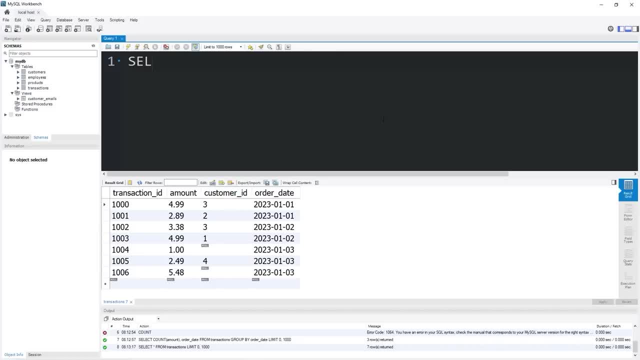 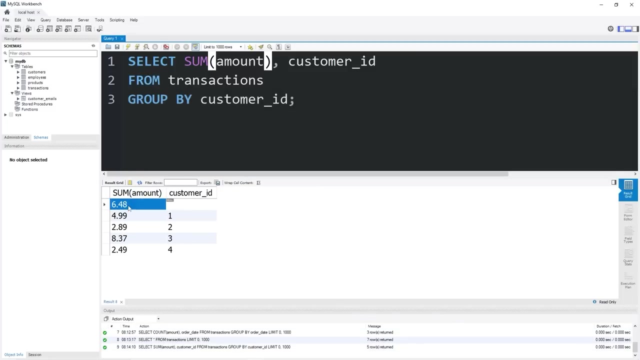 How much has each customer spent? total: We will select the sum of every amount. We will also need a column for customer ID From our table transactions. then we will group by the customer ID column. this time Here is the sum of every amount that each customer has ever spent. 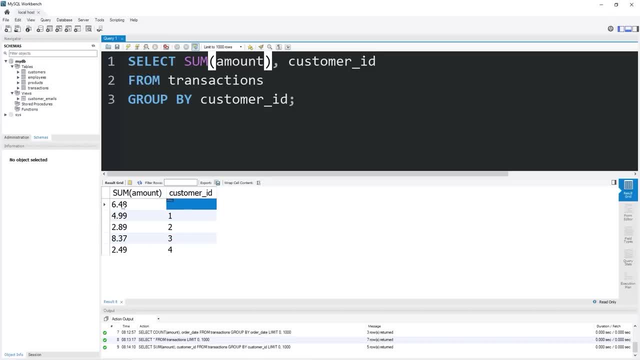 We do have some rows that don't have a customer ID, so we would sum those amounts as well. So far, the customer with an ID of three. they have spent the most amount of money at our establishment. What about the max? Here is the maximum order. 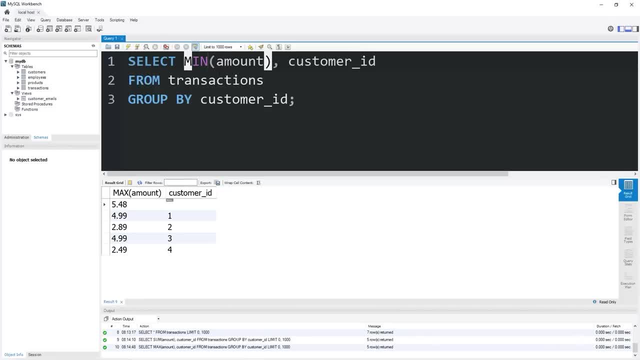 Here is the minimum order that each customer has placed: The min, The average, Then count. Here is the amount of times that each customer has ever visited our establishment. What if we would like to use a WHERE clause? Well, using a WHERE clause along with the GROUP BY clause normally doesn't work. 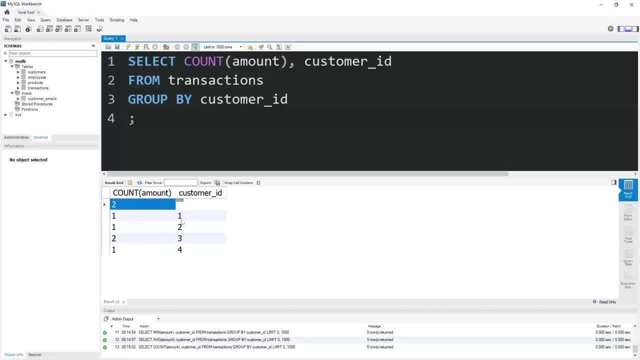 For example, I would like to display all customers that have visited more than once, Who are the repeat customers. There are one hundred thousand customers who could find customers who have made over $100 in the past year. So if I attempt to use this WHERE clause, 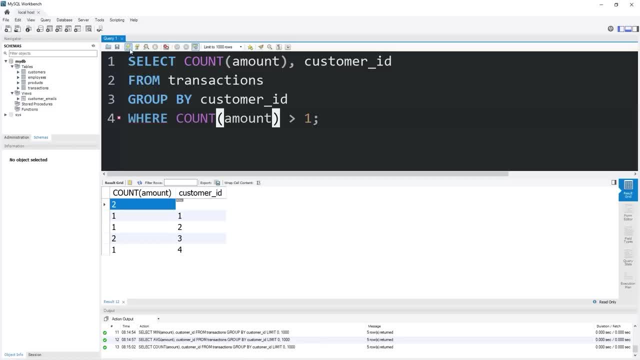 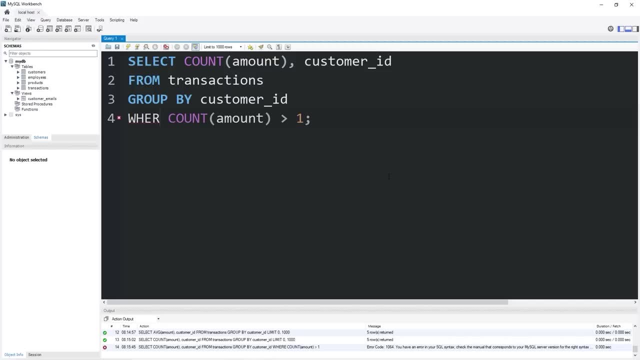 Where COUNT, our AMOUNT column is greater than 1.. Well, we would run into an error. So to run a WHERE where clause and we use the GROUP BY clause, we will use the jeden��고 NANDERING word: having. That would do the same thing. 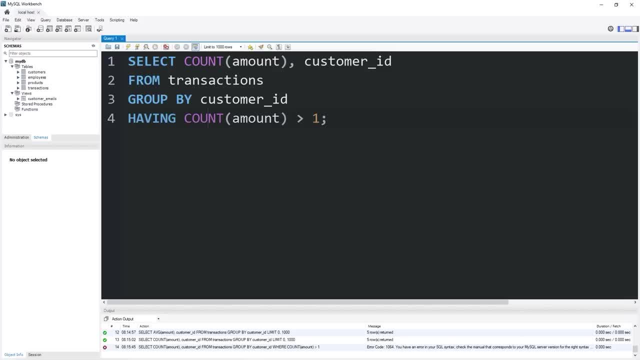 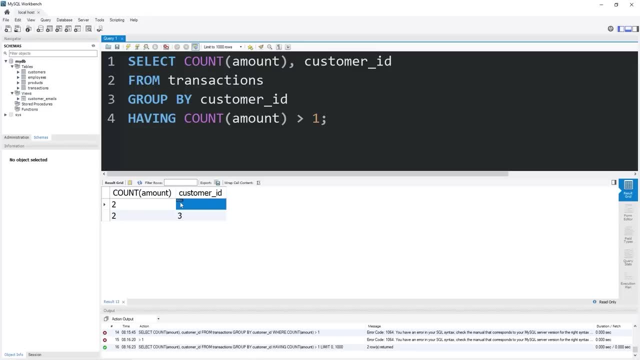 GROUP BY customer ID, where the customer ID had made more than 1 purchase. We are also agregating the customer to the group CORNER Club. GROUP BY customer id. ideas that are null. let's use the and logical operator to remove that. And customer ID is not. 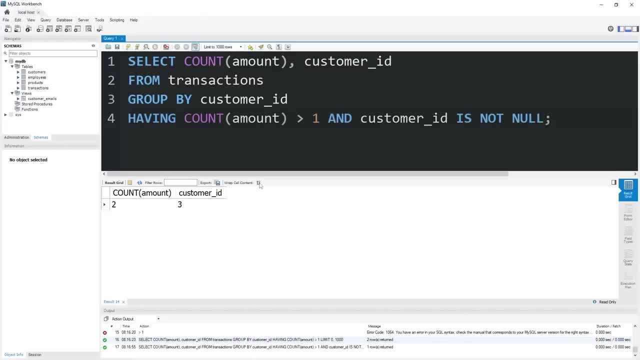 null. There we are The customer that has an ID of three. they have visited our establishment two times, they meet the requirements of this having clause. they have visited our establishment more than once and their customer ID is not null. So, if you ever need to use a where clause, if you're 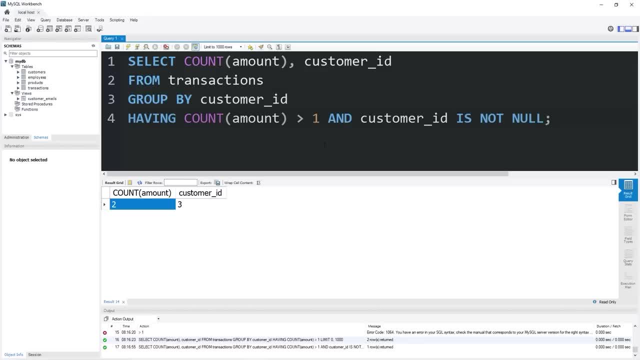 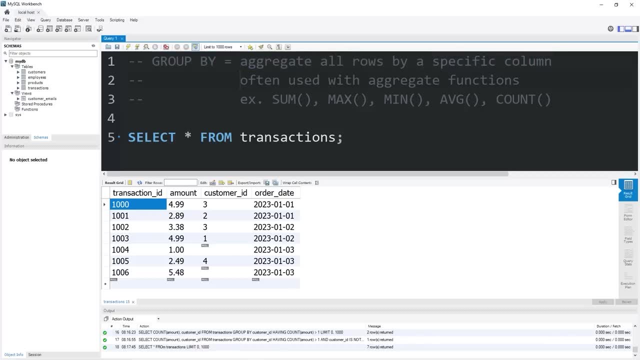 already using the group by clause, you would instead use having. So, in conclusion, the group by clause will aggregate all rows by a specific column. It's often used with aggregate functions, such as some max, min, average count, For example. you could group by an order date. what are the 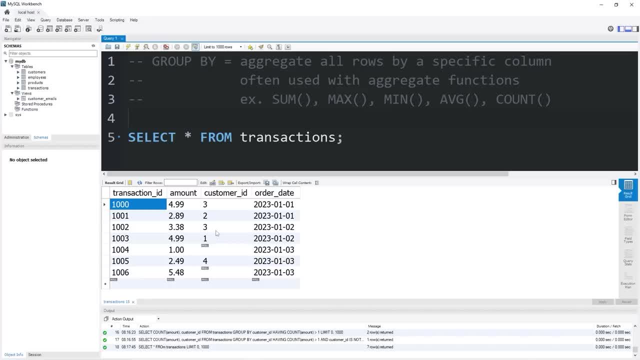 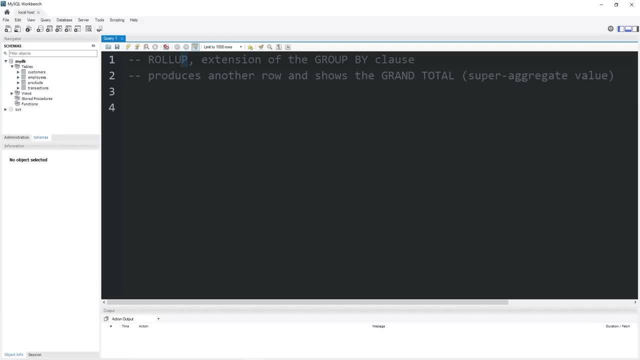 total sales per date or by a customer ID. How many times has each customer visited our establishment? Those are just a few examples. And well, yeah, that is the group by clause in MySQL. Hey again, it's me. Today I'm going to be explaining the rollup clause like a fruit rollup. 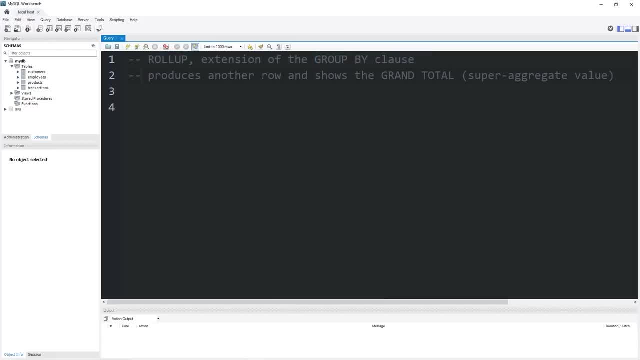 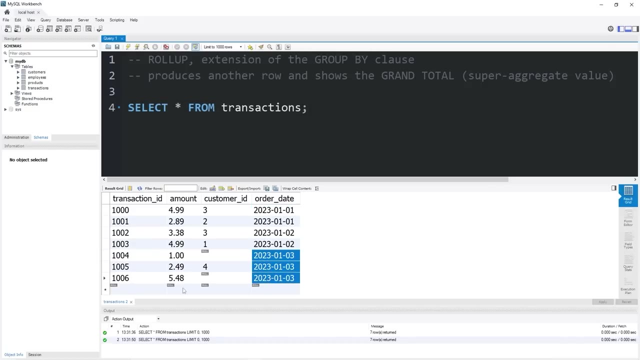 It's an extension of the group by clause. It produces another row and shows the grand total. It's also known as a super aggregate value. Here's an example: I have a table of transactions. What I would like to do is to group each transaction by the order date, then produce a grand total. 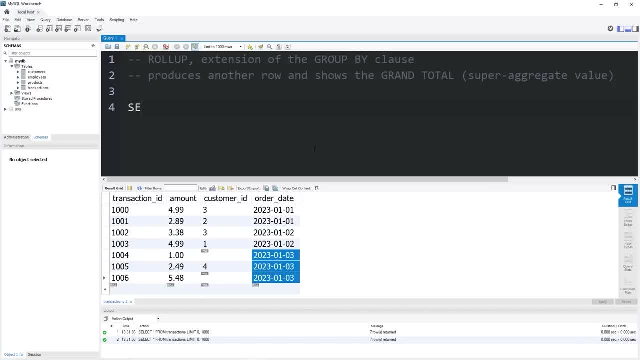 Here's what we'll do. I'll give you a few different examples. Let's begin by selecting the sum of the amounts and the order date from our table transactions. Then we will group by the order date And there we are: We have the sum of every amount. 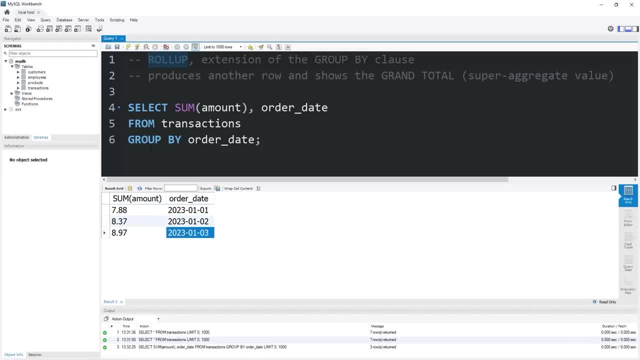 per order date. Using this rollup clause, I can add an additional row that shows a grand total, so to say. All I have to do after the group by clause is add with rollup And there you go. Here's the grand total: 7.88 plus 8.37 plus 8.97 is $25.22.. 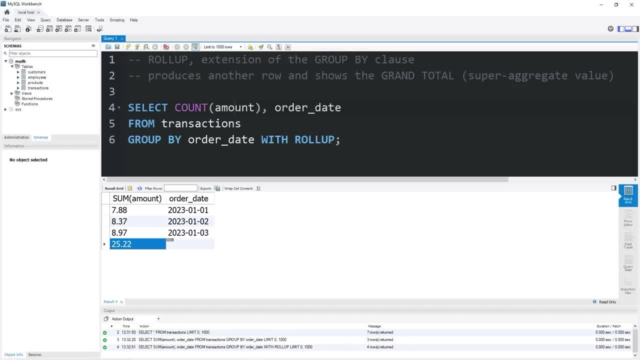 Here's another example. Let's count the transaction IDs By order date. We have two transactions on the first, two on the second, three on the third, for a total of seven transactions. I'll give you two more examples. Let's select. 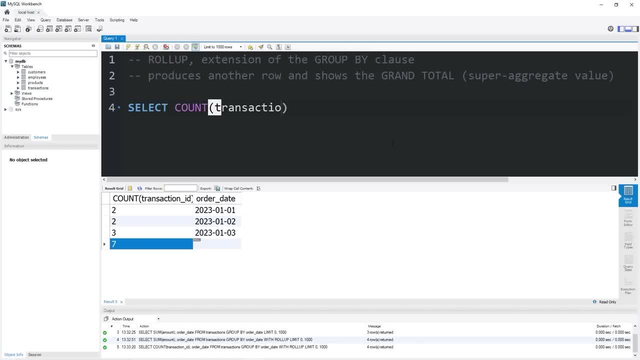 the count of our transaction IDs per customer. I'm going to give this count an alias as number of orders As well as the customer ID column from our table transactions. we will group by customer ID. Let's see what we have so far. 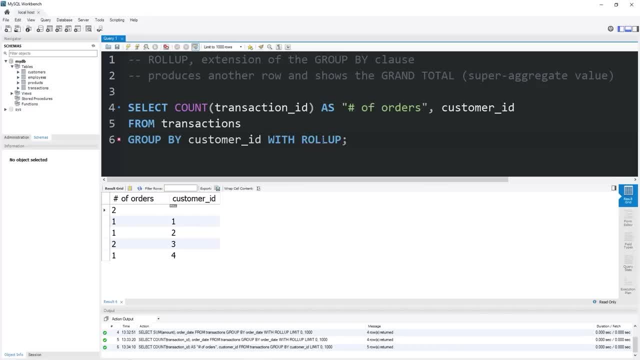 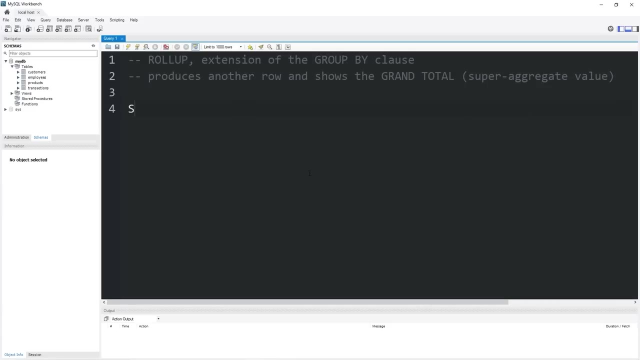 Then I will add with rollup. Here are the amount of orders per customer ID. The customer with an ID of three has visited here more than once. The grand total of the number of orders is seven. That's the rollup. One last example: Let's select our employees table. 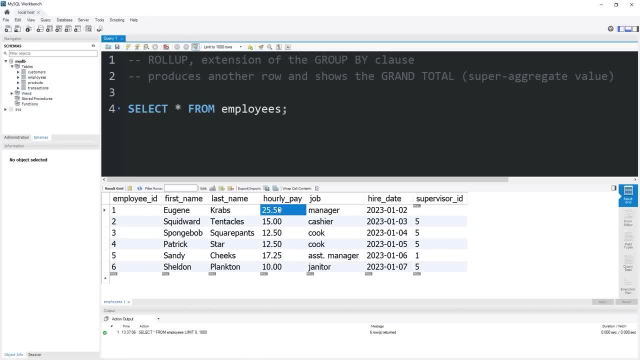 Select all from employees. We will group all of these employees by their employee ID, then display a rollup of all of the hourly pay. as a business, How much are we spending on all of our employees per hour? So let's select the sum of our hourly pay. 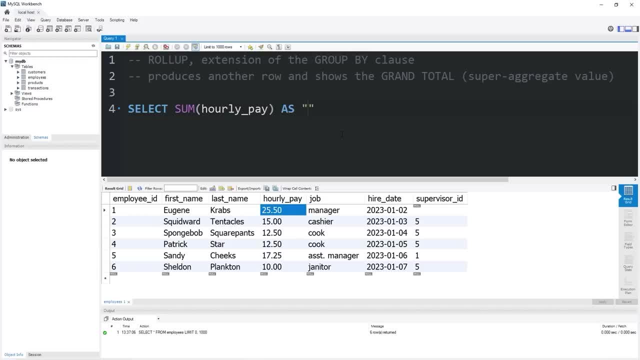 I'll give this an alias as hourly pay. I guess it really isn't different from the column name. We will display the employee ID as a column from our table Employees group by the employee ID with rollup. Here's the hourly pay of each employee as well as a group of employees. 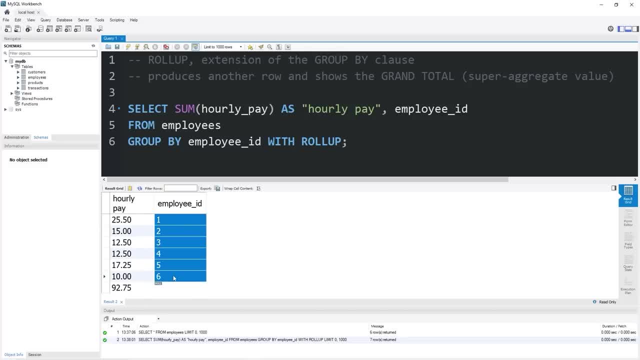 If all of our employees are working. currently, we are spending, as a business, $92.75 per hour. Well, yeah, that's the rollup clause, everybody. It's an extension of the group by clause. It produces another row and shows essentially the grand total. 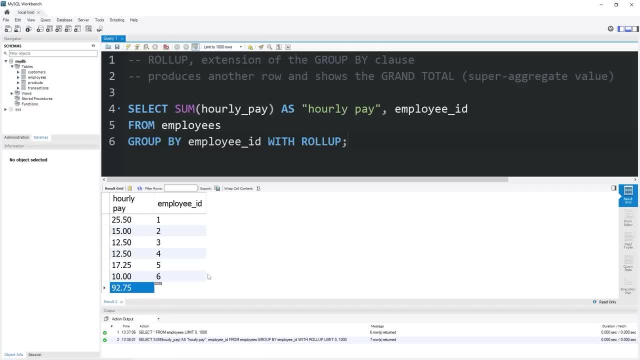 It's also known as a super aggregate value, To include a rollup after the group by clause. just add with rollup. It's probably good for accounting And well, yeah, that's the rollup, The rollup clause in MySQL. 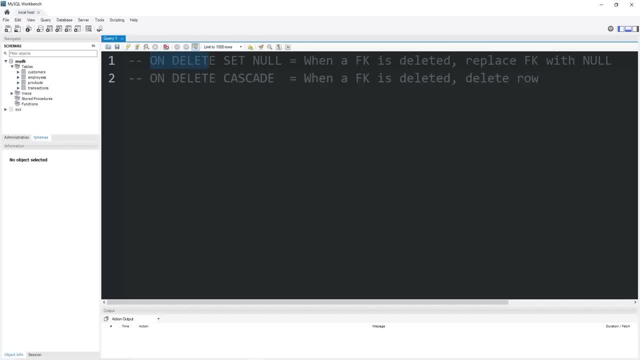 Why? hello there everybody. Today I will be explaining the onDelete clause. There's two versions: onDeleteSetNull and onDeleteCascade. With onDeleteSetNull, when a foreign key is deleted, we can replace the foreign key with the value null. 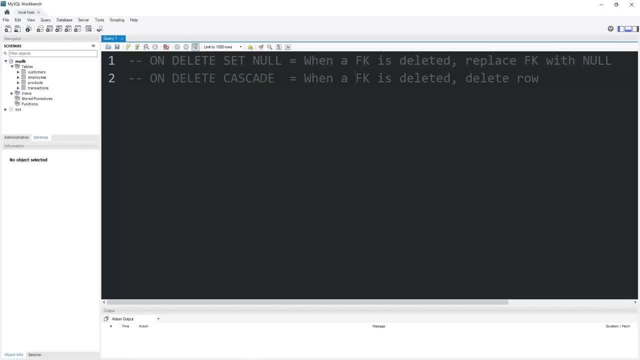 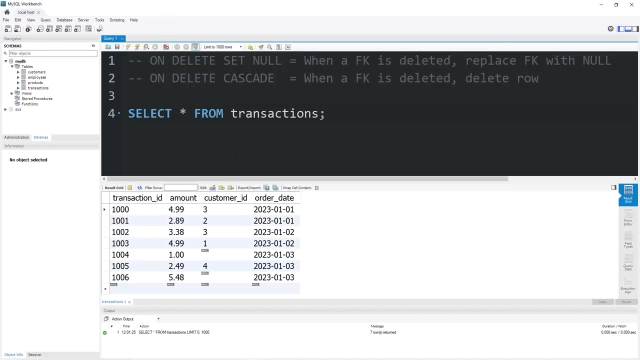 Otherwise there's onDeleteCascade. When a foreign key is deleted, delete the entire row. Here's an example. Let's take a look at our table transactions: Select all from transactions. In my transactions table the customer ID column is the foreign key. 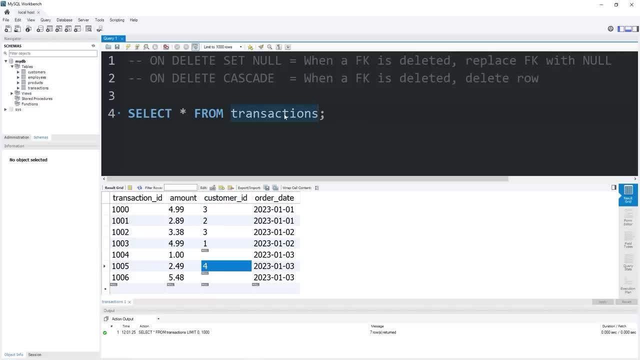 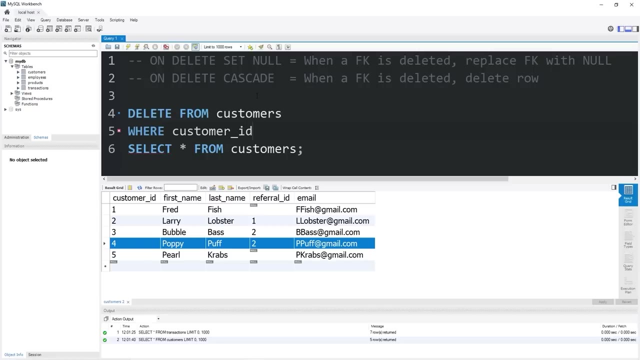 What would happen if I were to delete one of these customers? Let's select all from our customers table. I'm going to delete Poppy Puff. She has a customer ID of four. Delete from customers where customer ID equals four. If you run into this error cannot delete or update a parent row. 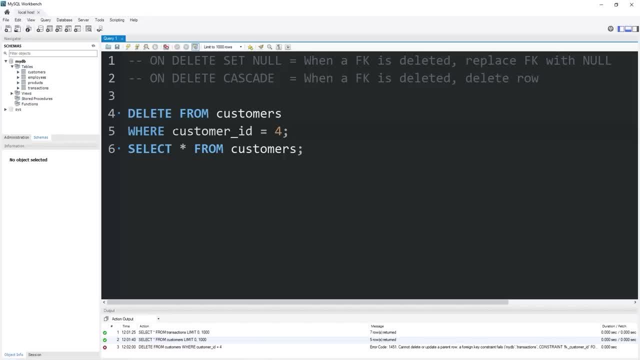 a foreign key constraint fails, There's a foreign key that's preventing us from deleting this customer, because this customer is used elsewhere, in a different table, like that transactions table. So just temporarily, for this demonstration, I'm going to set foreign key checks to be zero. 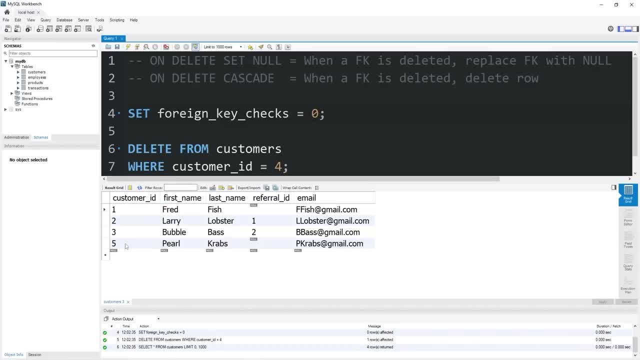 And that should work. Our customer with an ID of four is gone. One, two, three, five. Poppy Puff is no longer within our customers table. Before I forget, I'm going to set foreign key checks back to one. 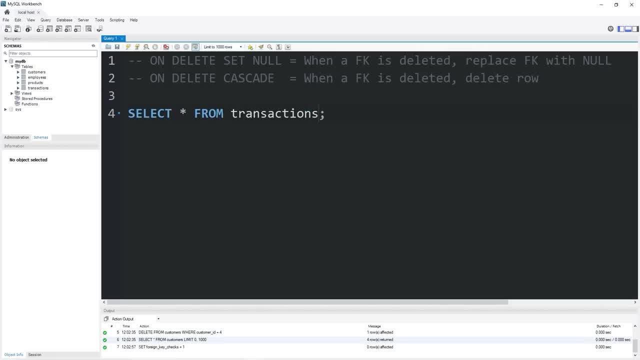 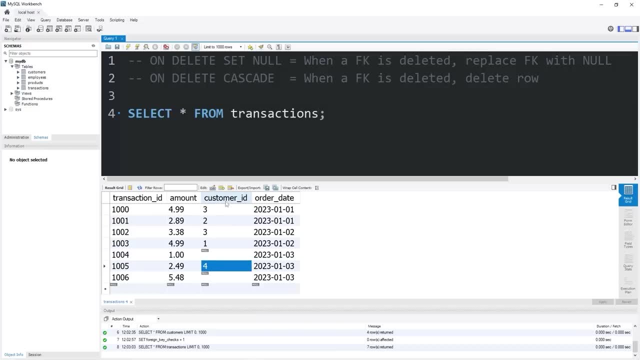 Let's take a look at our transactions table. Underneath this transaction of one thousand five, we're referencing a customer that doesn't exist. The customer with an ID of four is no longer within our customers table. We have a couple options whenever we delete a primary key from another table. 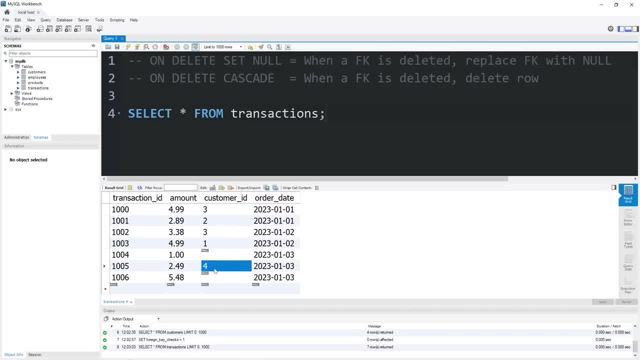 that's being used as a foreign key somewhere else. We can either Replace that value with null or delete the entire row with cascade with undelete set null. We can replace this value with null, much like these two rows or undelete cascade. 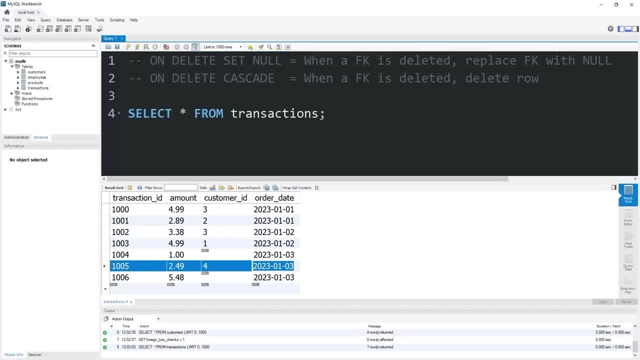 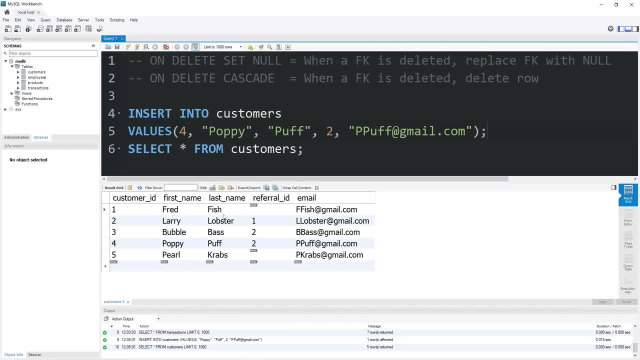 We can delete the entire row. Let's begin with undelete, set null. I'm going to reinsert Poppy Puff back into our table of customers. And there we are: Poppy Puff is back in the customers table Now, with. 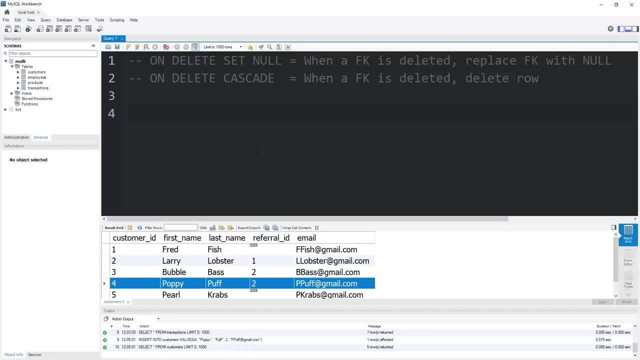 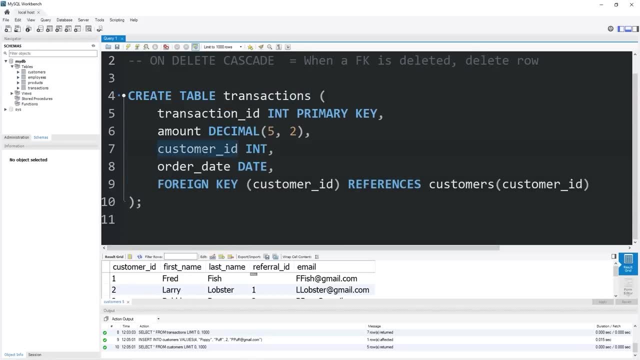 Undelete set null. If we're creating a new table- Let's say I'm recreating my table of transactions- after adding the foreign key constraint- Foreign key. our customer ID column references the customer ID column of the customers table. I can add this clause: undelete set null. 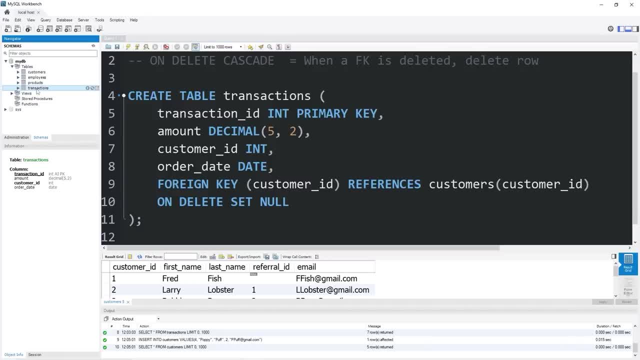 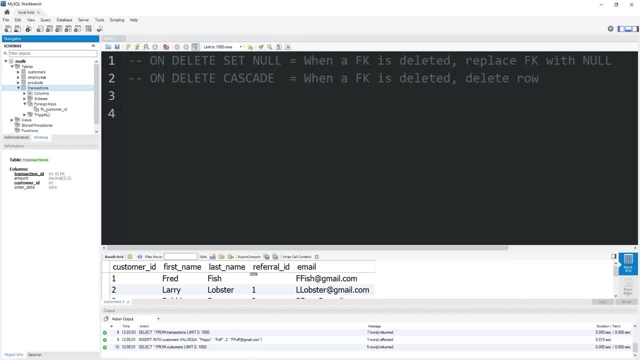 That's if I'm creating a new table but I already do have a transactions table. I don't want to update it. However, I can update an existing table with this clause. I already do have a foreign key constraint. I'm just going to drop it real quick. 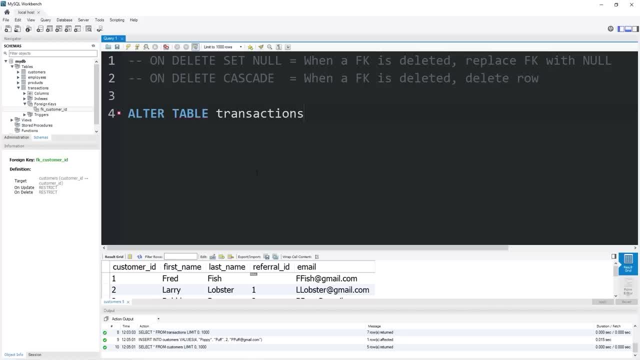 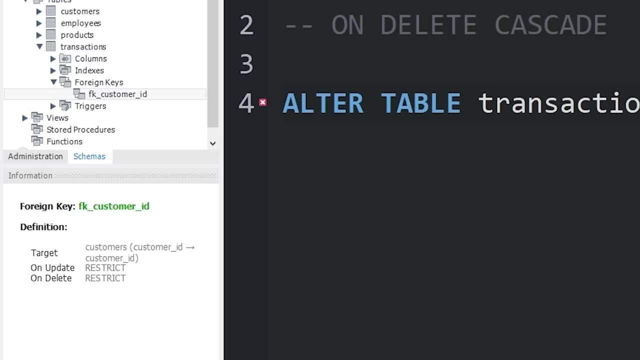 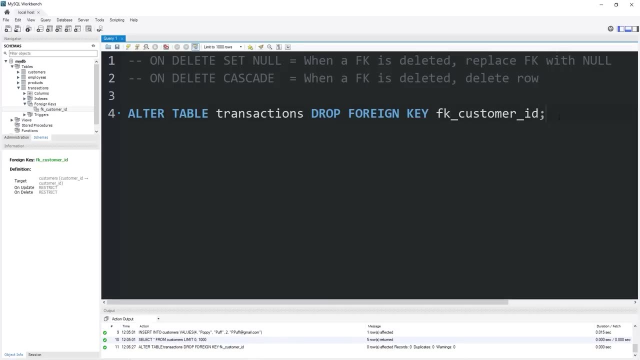 Alter table transactions- Drop foreign key. then the name of the foreign key- Mine is FK, underscore customer ID And that key is now dropped. We are going to add a foreign key constraint to our transactions table With this clause: undelete, set null. alter table the name of the table: add constraint. 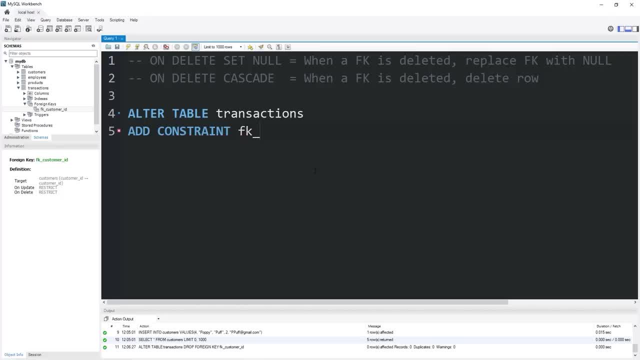 You can give your constraint the name. I'll give it the same name as before: FK. customer ID List- the foreign key, Foreign key. My foreign key is customer ID References Another table which was Customers, And what is the primary key of that table? 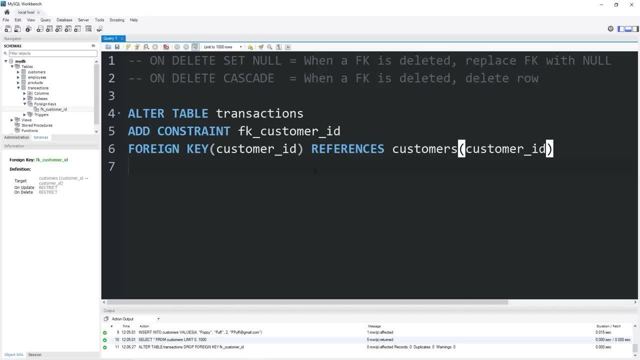 Customer ID, Then we will add the clause undelete set null. If I delete a customer ID from customers, the foreign key of that row will be set to null automatically. Let's execute this. Let's take a look at our transactions table. 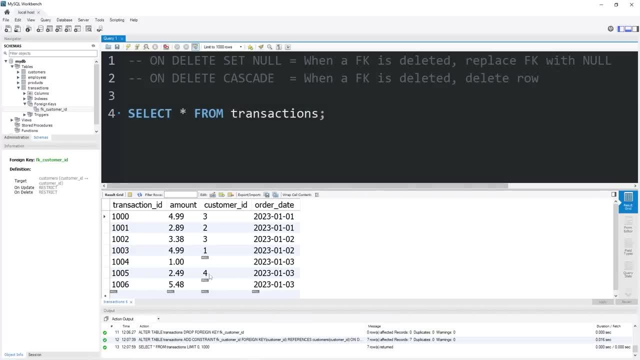 Select all from transactions. I am now going to delete customer number four from the customers table. Delete from customers where customer ID equals four. Yeah, check that out. With our transaction ID of one thousand five, the customer ID is now null. Now there's undelete cascade. 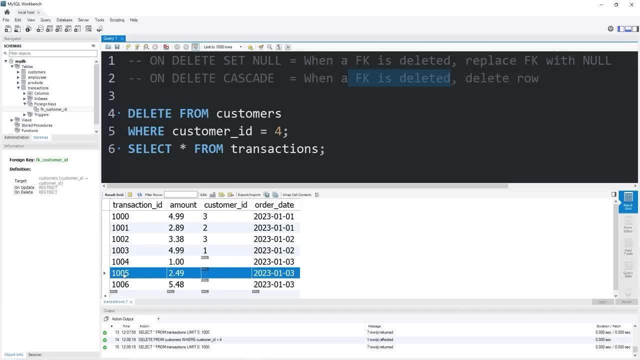 When a foreign key is deleted, we can instead delete the entire row. Let's go ahead and add Poppy Puff back to our customers table. All right, she's back in. Let's drop the current foreign key constraint of our transactions table. 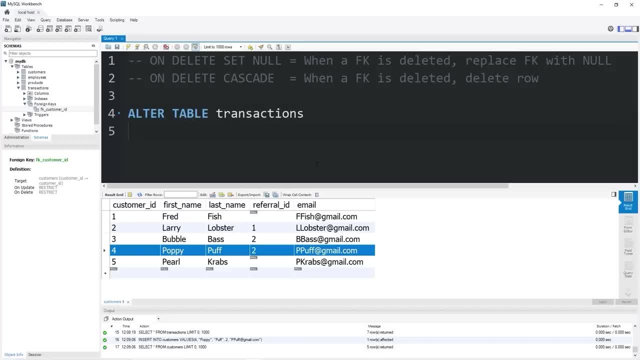 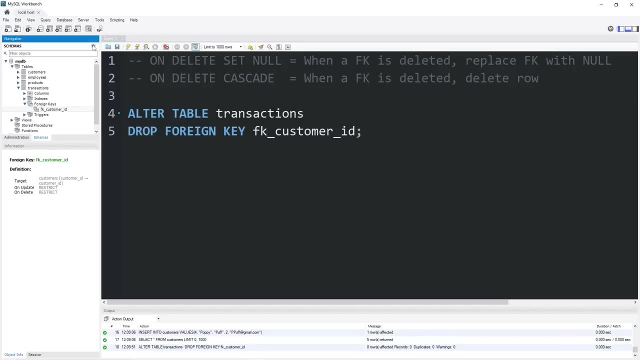 Alter table transactions. Drop foreign key: FK customer ID or whatever else it's named, And that key is now gone. We will add the undelete cascade clause to a table That already exists. Alter table transactions. Add constraint: You can come up with the name FK: underscore transactions. underscore ID. 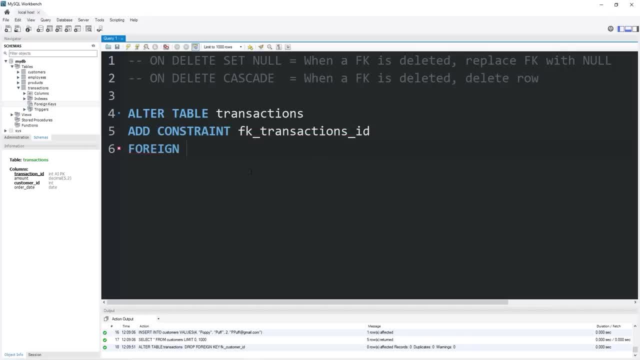 List the foreign key. Foreign key customer ID References The customers table And the primary key of that table is the customer ID. Then add undelete cascade. Let's take a look at our transactions table. Select all from transactions. Oh, let's update this customer ID real quick. 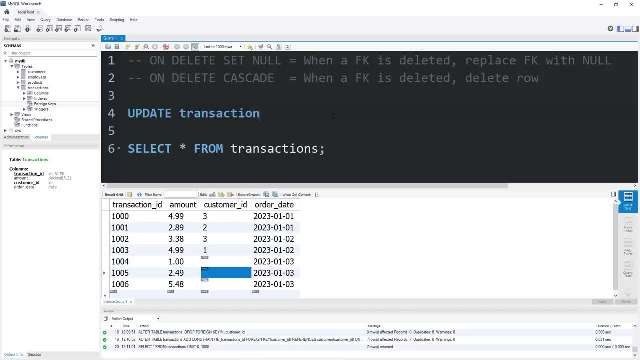 I forgot to do that. Update transactions. Set customer ID equal to four Where transaction ID equals 1,005.. Yeah, I forgot to add that back. Now let's do it. Delete from customers where customer ID equals four. Yeah, take a look at that. 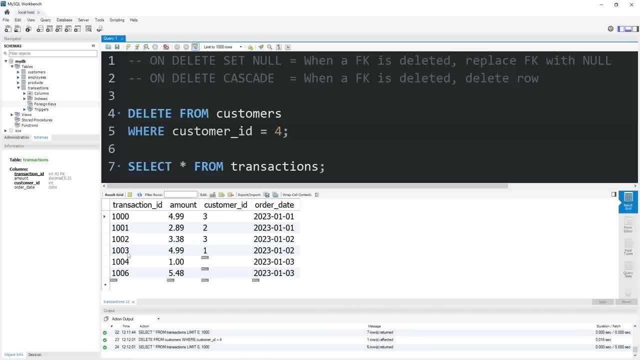 The entire row is now gone. We have transactions 1,003, 1,004, 1,006.. 1,005 is missing because it was referencing the customer with an ID of four. We set the foreign key to delete the entire row when that foreign key is deleted. 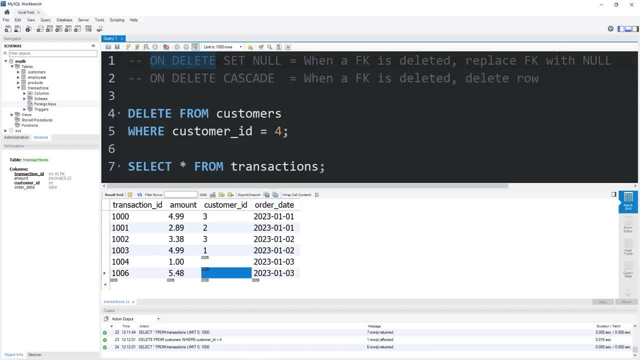 That is undelete cascade. Well, in conclusion, everybody, undelete is a clause where, if you delete a foreign key, you can set that value to be null or cascade, which will delete the entire row which has its uses. And well, yeah, that's the undelete clause in MySQL. 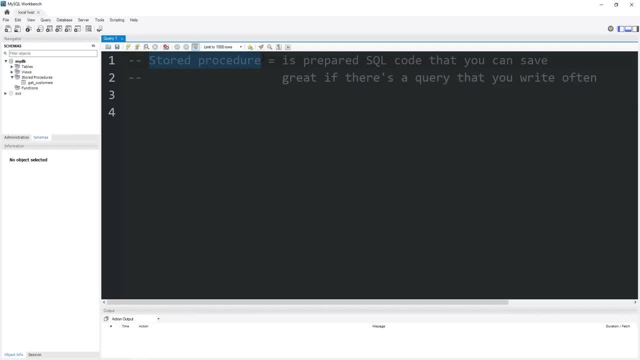 Why? hello again, it's me. So today I got to explain stored procedures. A stored procedure is prepared SQL code that you can save. It's great if there's a query that you write often. For example, I have this statement. 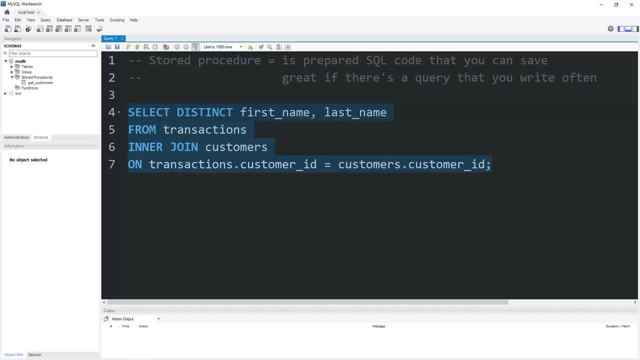 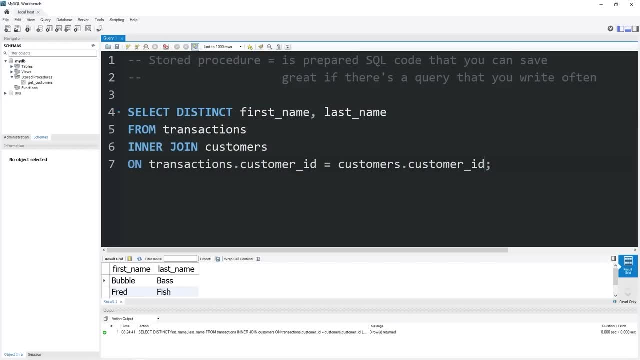 It's very verbose. There's a lot we have to write. If this statement is something I have to write often, I could save it and reuse it later. This statement will interjoin the transactions table and my customers table, then display all customers that made a transaction. 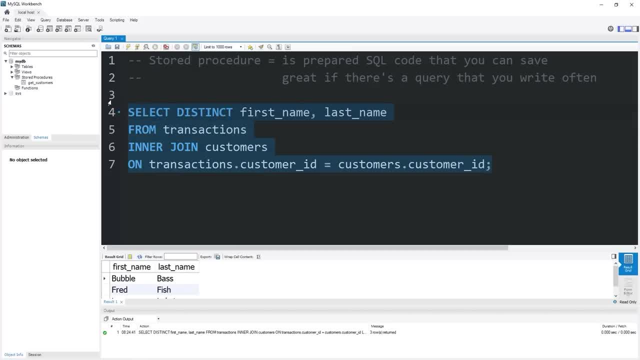 This statement is very verbose. If I have to write the statement often, I could save it as a stored procedure. I can refer to the nickname that I gave that snippet of code. The name I gave this procedure was get customers. Then I need to call this stored procedure. 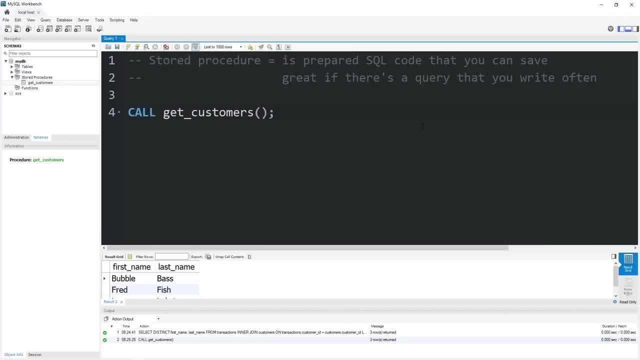 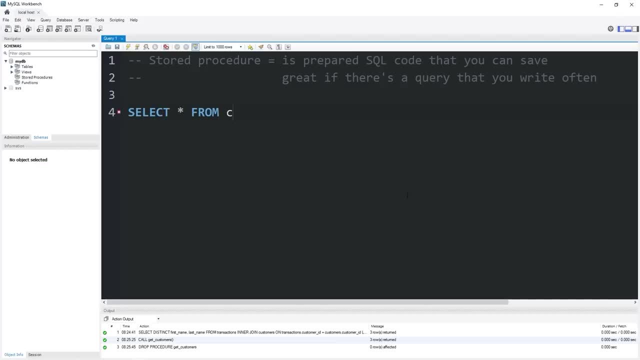 And that does the same thing, and it's a lot less to write. There's also a few other benefits which we'll discuss at the end of the video. Let's begin with something simple. I would like to select all from my customers table to turn the statement. 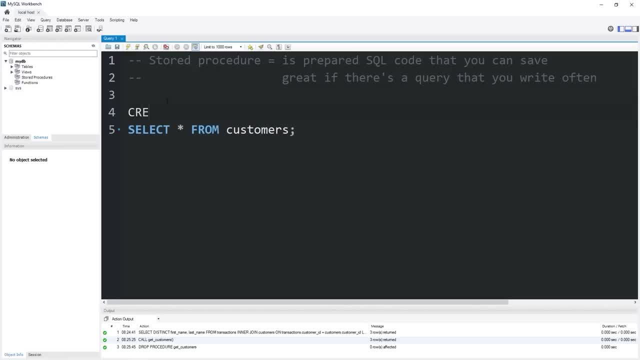 or statements into a stored procedure. I will type create procedure. then a name for the statement or statements. I will name this statement: get customers. Add a set of parentheses. Type the keyword begin Wherever your statement or statements end. Type end. 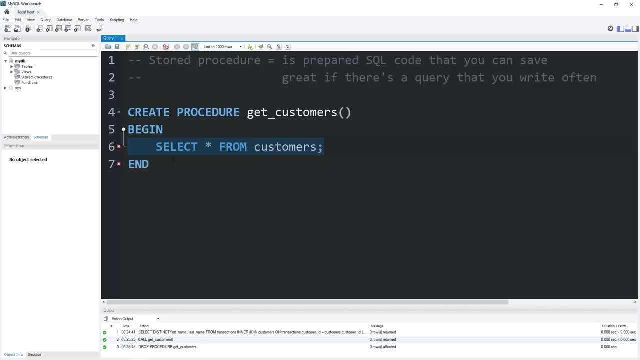 Then, for clarity, I'm going to tab all of my statements between begin and end. So we have a problem. We're trying to create this procedure. However, MySQL is stopping at the semicolon here. We end all statements with a semicolon rather than at the end. 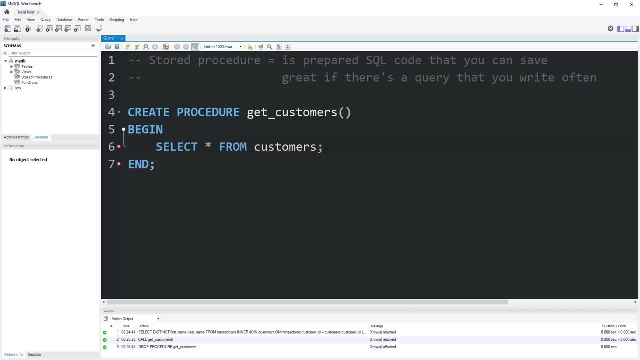 Our semicolon is known as a delimiter. It's kind of like the period at the end of the sentence. We're telling MySQL that our statement ends here, but we need our statement to end here. After the end keyword, we can actually change the delimiter temporarily. 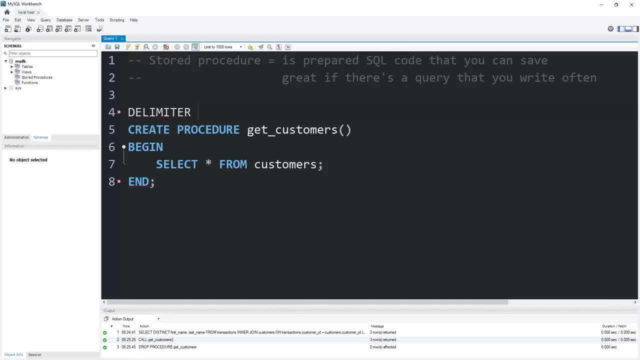 Type delimiter before we create the procedure. Typically, when people change their delimiter temporarily, they'll either use two forward slashes or two dollar signs. I'll stick with the dollar signs because I think that's cooler. After we create our procedure, let's change our delimiter back to the semicolon. 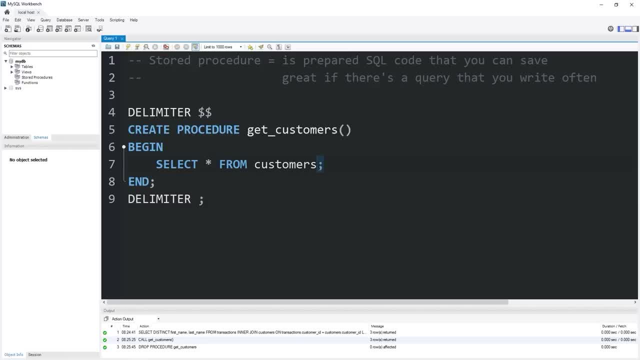 MySQL no longer recognizes our semicolon as the delimiter after the end keyword. I will use our new Delimiter to end this statement. That should work now. Let's execute this statement. We have created our procedure. I'm going to refresh my navigator window underneath stored procedures. 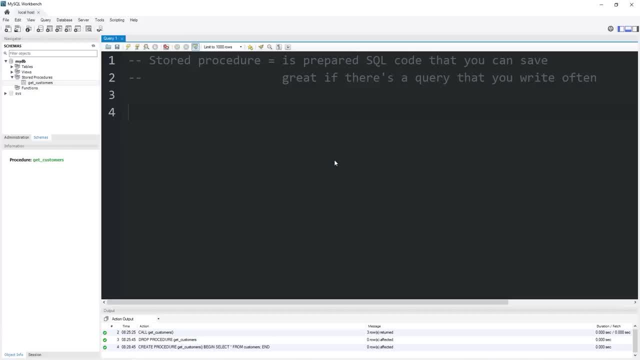 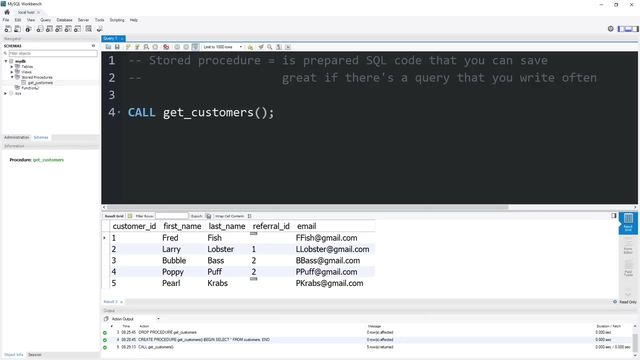 We have our stored procedure of get customers to invoke the stored procedure, Type call the name of the procedure. Get customers Add a set of parentheses, then a semicolon that will execute whatever code you stored within your stored procedure. To drop a stored procedure, you would type drop procedure- the name of the procedure. 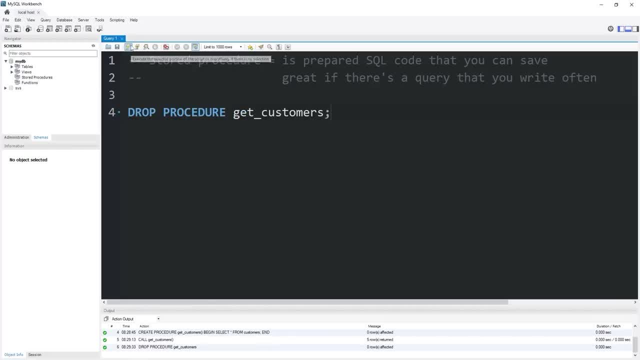 Get customers. Let's try another example. This time we will send our procedure a piece of data, within the set of parentheses, A customer ID number, such as one, two, three, four, so on and so forth. We will get a customer by their customer ID. 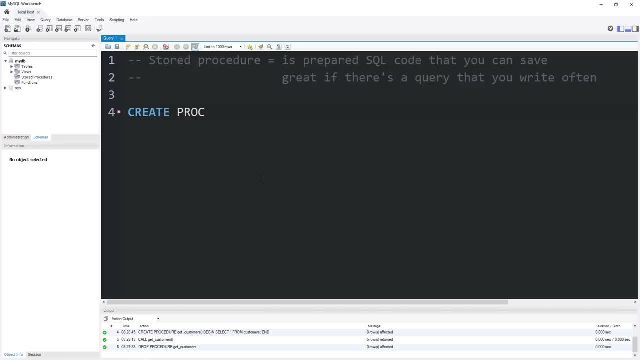 We will create A procedure. I will name this procedure: find customer. Add a set of parentheses to find a customer by their customer ID. When we invoke the stored procedure, within the set of parentheses we will need to place a customer ID. But when we create the stored procedure, we have to set up what is called a parameter. 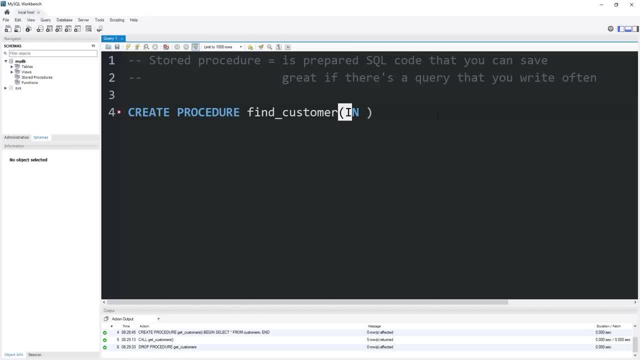 We will type in then a nickname for that piece of data We're passing in a transaction ID. I'll give this parameter a nickname of ID. Then we need the data type of what we're passing in. We're passing in an integer. 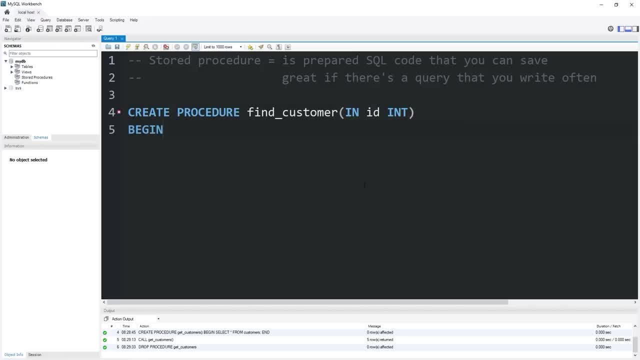 So we have one parameter set up. Let's use that begin keyword, that end keyword, List our statement or statements between these two keywords. I will select all from my customers table where my customer ID equals the ID that we passed in. I will select all from my customers table where my customer ID equals the ID that we passed in. 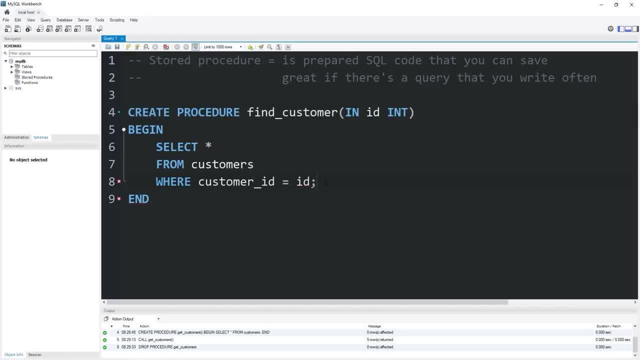 I will select all from my customer ID equals the ID that we passed in. I will select all from my customers table where my customer ID equals the ID that we passed in That nickname. We need to change the delimiter Because MySQL thinks we're trying to end our statement here. 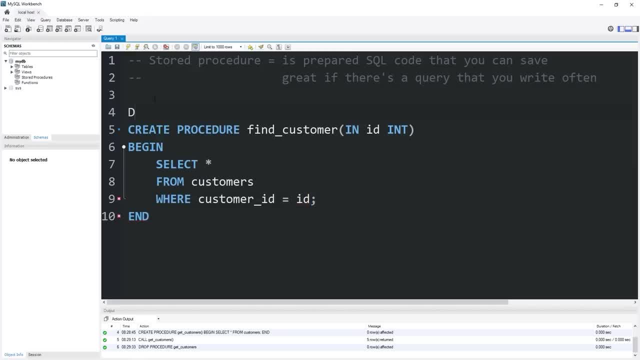 But we need it to end after the end keyword. So let's change the delimiter to double dollar signs, Then change it back. All right, we have created that stored procedure. Let's invoke it. Call: find customer. Within the set of parentheses, we need to pass in a customer ID number. 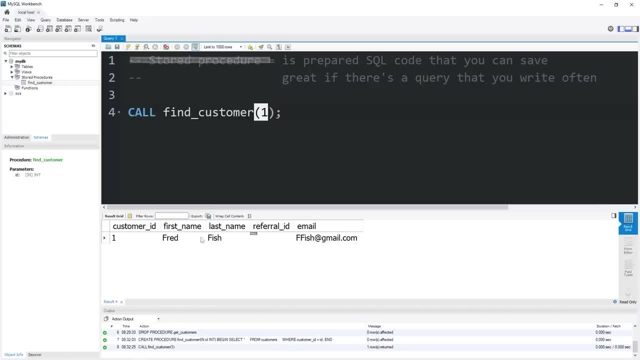 Let's pass in one. That would give us Fred Fish. Two is Larry Lobster. Three is Bubble Bass. Five is Pearl Crabs. When you invoke a stored procedure, you can pass in some data, Depending on what you need exactly for your stored procedure. 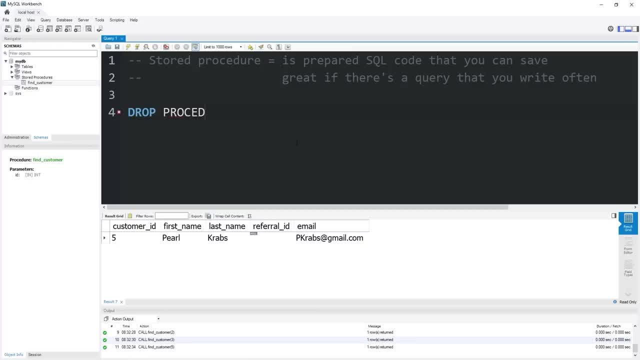 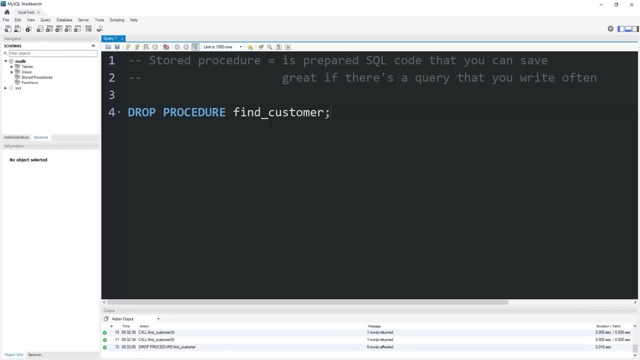 Let's drop this procedure. then do one last example. Drop procedure: Find customer. This time we will send two arguments, Two pieces of data: A first name and a last name. Create procedure: Find customer. Within our set of parentheses, the first piece of data we'll pass in will be a first name. 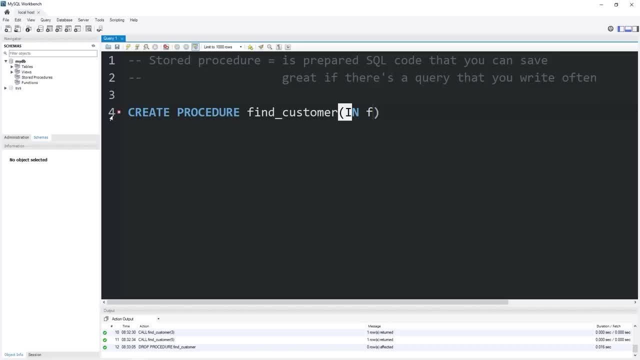 But first is already a keyword, Maybe F name Meaning first name, Then the data type. Let's see: For customers the data type of first and last names is Varchar50.. Varchar50.. For your next piece of data, you would separate that with a comma. 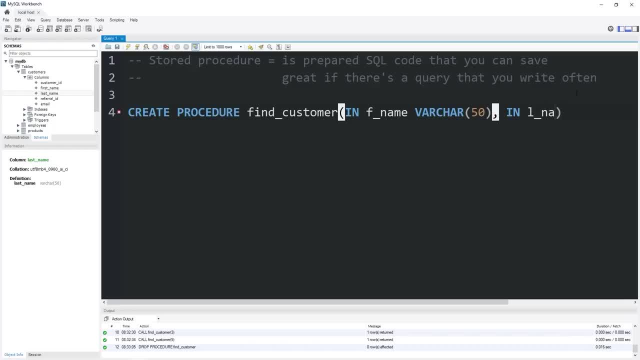 In Our nickname will be L name. for last name, Data type is Varchar50.. Then I'm just going to put that on a new list. New line for clarity: Type the begin keyword And write your statements between begin and end. 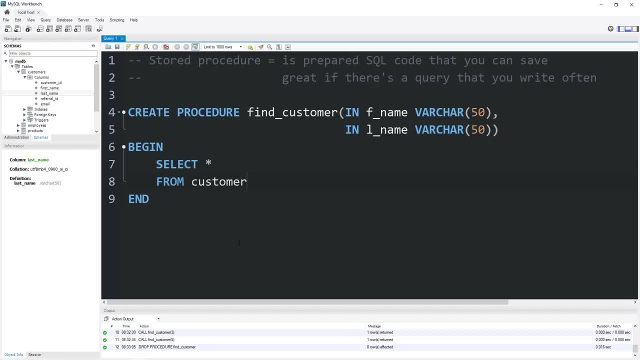 We will select all from our customers table Where first name equals the name of the data that we pass in And last name equals the other piece of data, The second piece, The last name. Again, we need to change the delimiter to create this procedure. 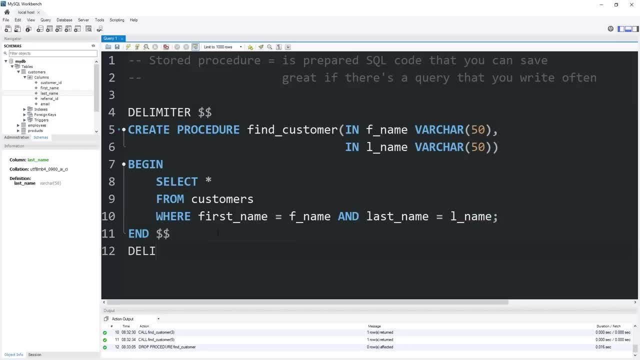 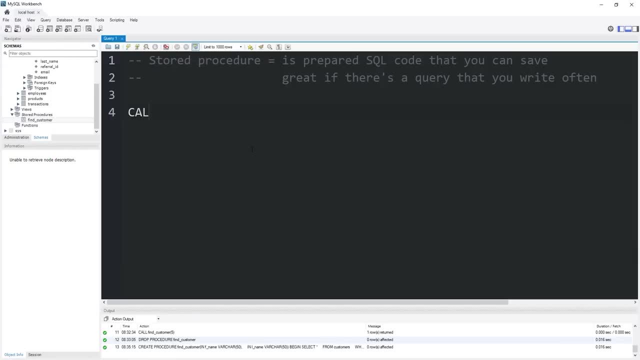 Double dollar signs, Then change it back. We have created our stored procedure. Let's invoke it. Call: find customer. Within the set of parentheses we will list a first name and a last name: Larry Comma Lobster. Get Larry Lobster's information. 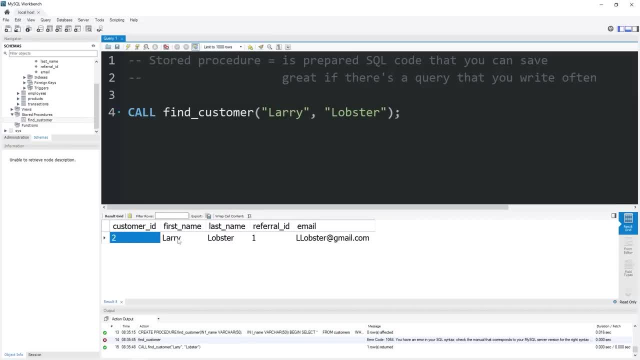 Let's find him, And there he is. Customer ID 2. First name: Larry. Last name: Lobster. Referral ID of 1. Email is llobster at gmailcom. All right, everybody, That is a stored procedure. 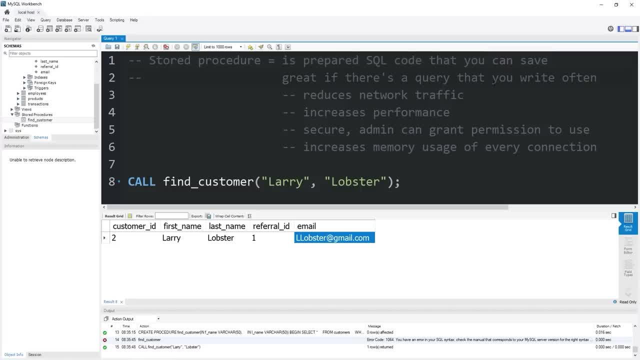 It's prepared SQL code that you can save. It's great if there's a query that you write often. A few of the benefits is that it reduces network traffic. It increases performance and is more secure. An administrator can grant permission to a user or an application to use a stored procedure. 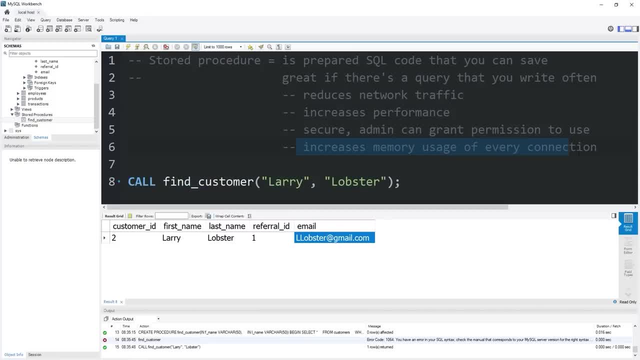 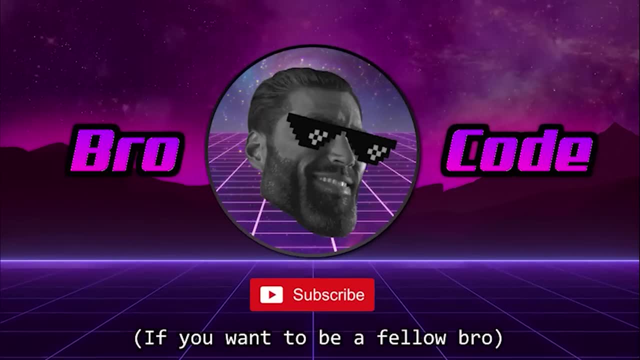 One of the downsides, though, is that it increases memory usage of every connection And, well, everybody. those are stored procedures in MySQL. Hey everybody, Today I need to explain triggers. When an event happens, a trigger does something. 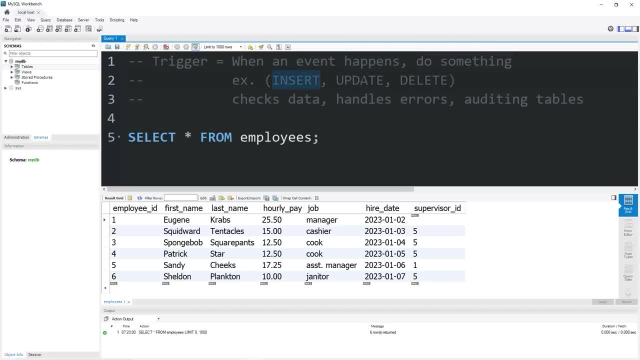 I know that sounds very generic. For example, when we insert, update, update or delete a record, we can use a trigger to check data, handle errors or audit tables. We can do a plethora of things. Here's an example: I have a table of employees. 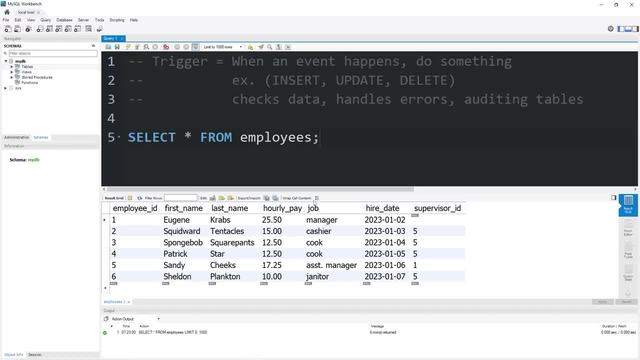 We have an hourly pay column. Maybe I would like a salary column. Whenever we add an employee or update our hourly pay, the employee's salary will be changed automatically with the trigger. Before creating a trigger, let's update our employees table. We'll add a salary column. 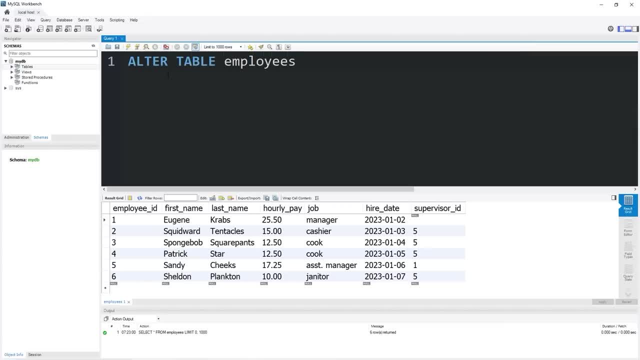 Filter table: employees- add column salary. The data type will be decimal ten digits, precision of two. We will place this column after the hourly pay column, Then select all from our employees table. Let's see what we have. 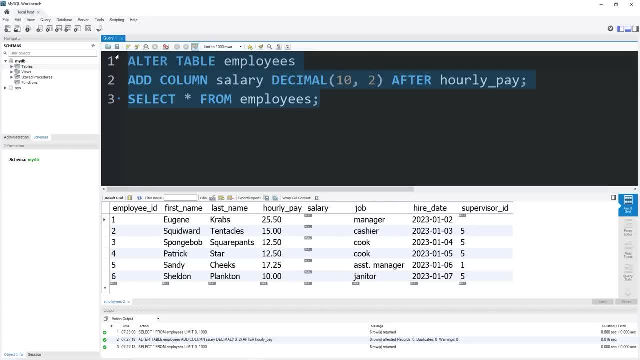 There we are. There's our salary column. Let's update our employees table. Set our salary column equal to the hourly pay times To calculate an employee's salary using an hourly pay- Sheldon Plankton, for example. take the hourly pay ten dollars per hour. 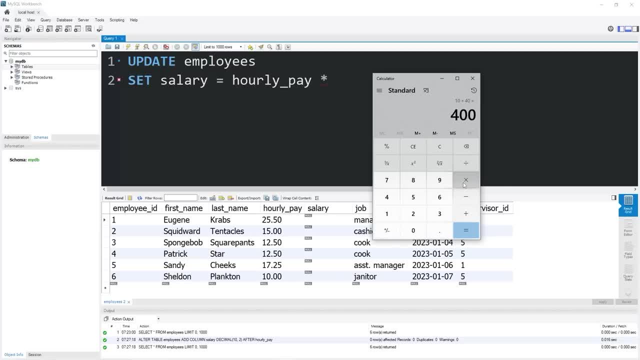 There's typically 40 hours in a work week, then 52 weeks in a year. Plankton would have a salary of $20,800.. So a shortcut: You could just take the hourly pay times 2080.. There are 2080 work hours in a typical year. 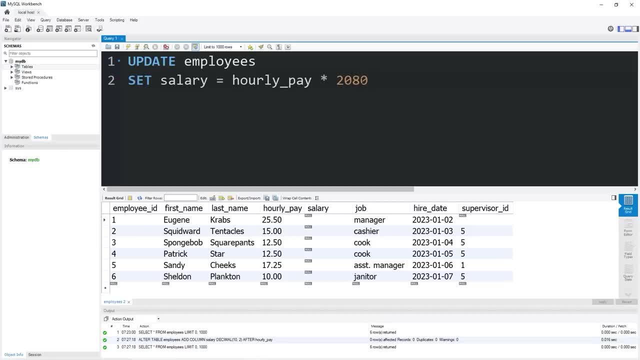 So take the hourly pay times 2080.. Then we will select all from employees. There is everybody's salary currently. Whenever we update an employee's hourly pay, I would like to also update the salary automatically with the trigger. I don't want to have to calculate every employee's salary manually. 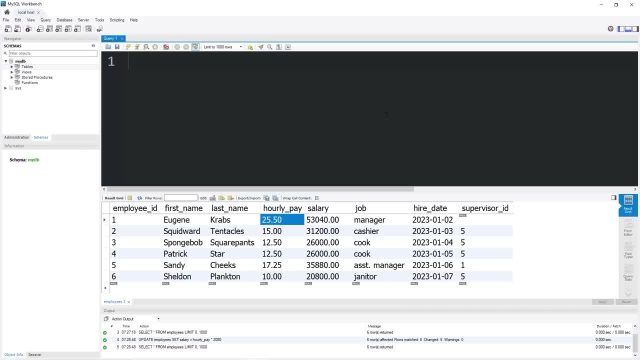 You know, using a calculator like I just did, We're going to create a trigger. Create trigger. Then we need a name for this trigger. Before we update the hourly pay, we're going to do something. I will name this trigger before hourly pay update. 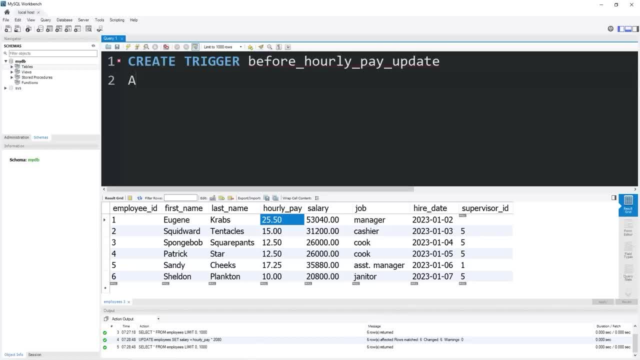 We'll use either the keyword before or after. Do you want to do something before or after? I would like to do something before. Before what? Before an insert? before delete. before an update. before an update, In this case on our table. employees, then add this line for each row. 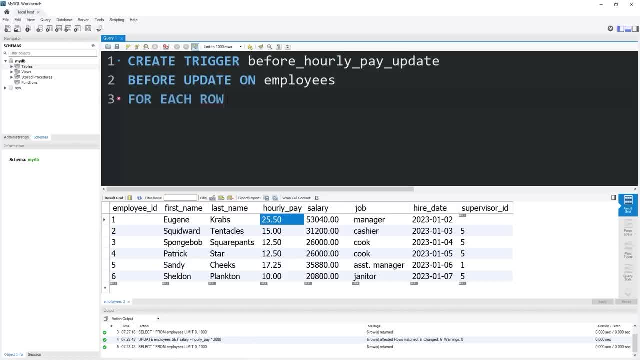 We may be working with more than one row using a trigger, So that's why we're including this line. This trigger can involve one or more rows. Now, what are we going to do before we update, We're going to add an employee's hourly pay. 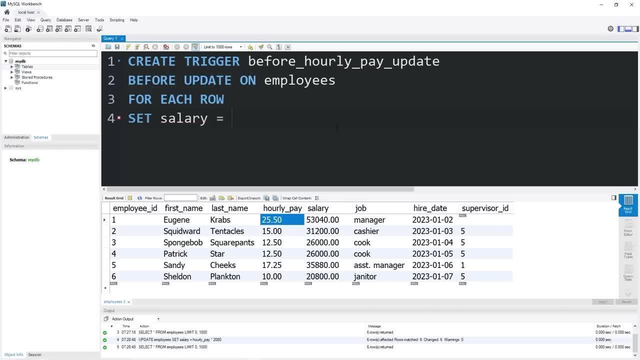 Let's set the salary equal to the hourly pay times 2080.. Because there's 2080 work hours in a typical year. Okay, there's one more thing I'm going to add. Let's prefix salary and hourly pay with this new keyword. 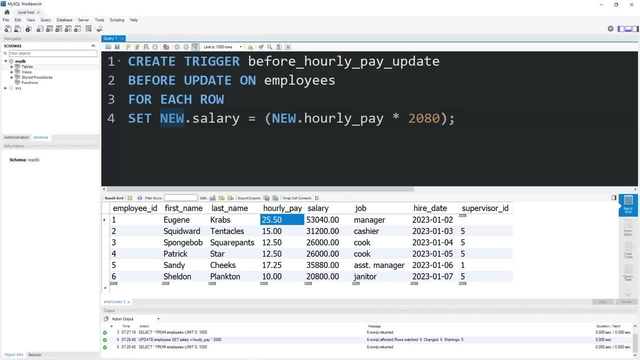 New dot salary. new dot hourly pay. Does it know if we're referring to the old salary and the old hourly pay? We're telling MySQL: we're calculating a new salary, Use the new hourly pay when that's changed in place of the old one. 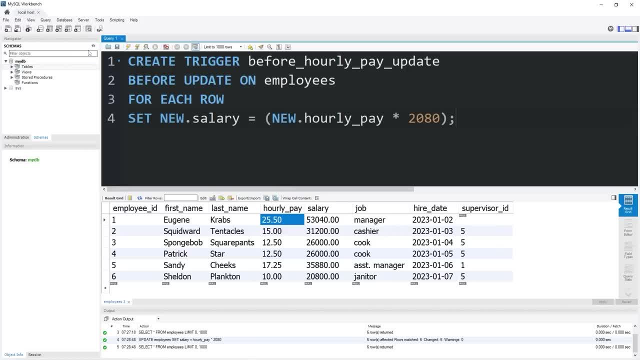 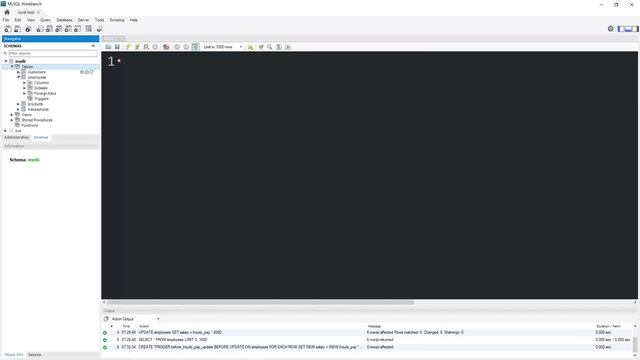 Okay, let's take a look. Let's execute this statement. Our trigger has been created in your schemas window to find any triggers, Go to tables, then find that table where we applied the trigger: Employees, then triggers. I probably need to refresh this. 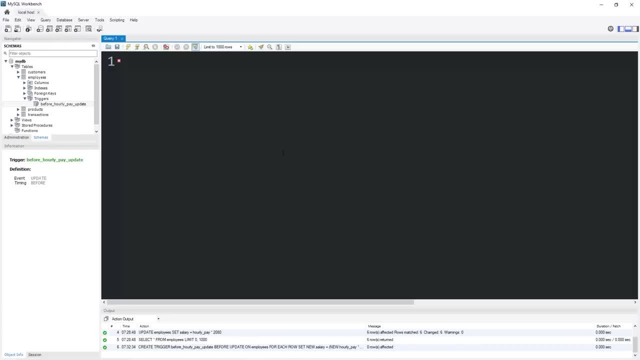 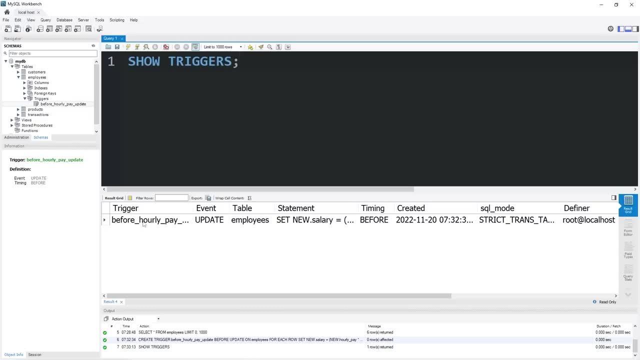 There it is Before hourly pay update. Otherwise you can type: show triggers And here is our trigger. Here's the trigger name: event: update the table, the statement and the timing. Let's select all from employees, Mr. 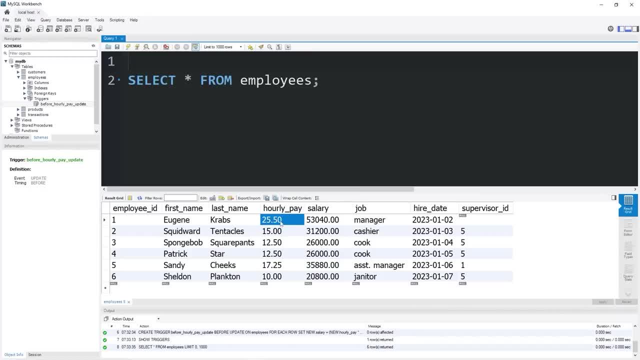 Krabs is going to give himself an hourly pay raise because he's greedy. Let's update our employees table. Set the hourly pay equal to $50 per hour where our employee ID equals one. So Mr Krabs salary is about $53,000 per year. 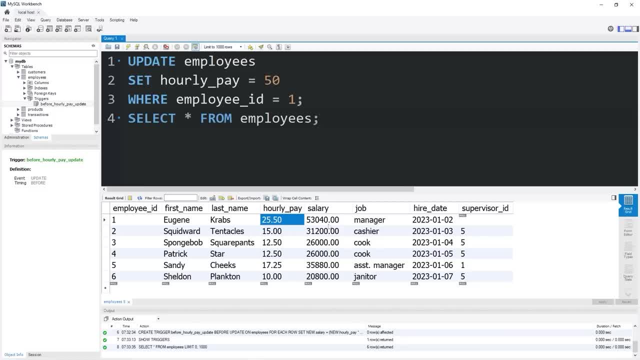 Before we update it, we will change the salary of this employee from $53,000 to over six figures, $104,000.. That change happened automatically with the trigger. Before updating the employee's hourly pay, we calculated a new salary automatically. 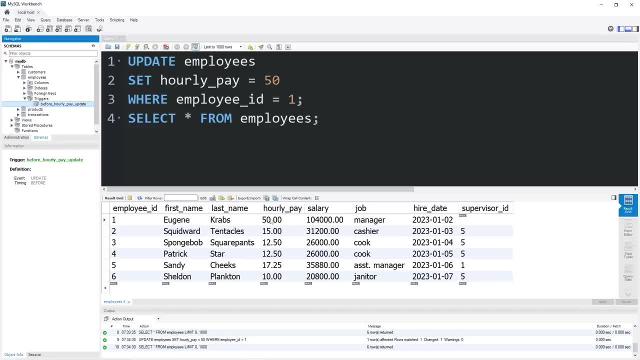 Let's make another change. Let's increase every employee's hourly pay by $1 per hour. Mr Krabs is now feeling generous. Update employees: We will set the hourly pay equal to whatever the hourly pay currently is plus one. We will apply this for every employee. 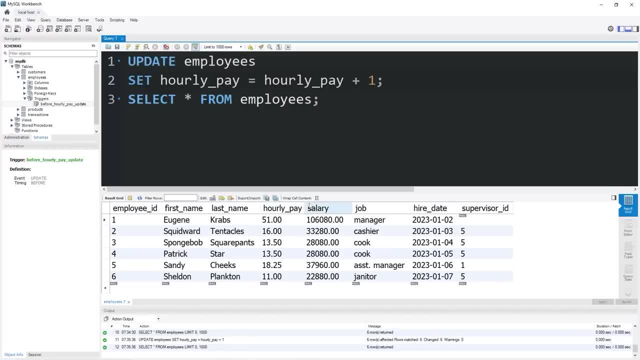 We don't need a where clause there. Everybody is now making one more dollar per hour and the salaries reflect that. Let's create a new trigger. We will calculate a salary whenever we insert a new employee. More specifically, whenever we insert a new hourly pay right now. 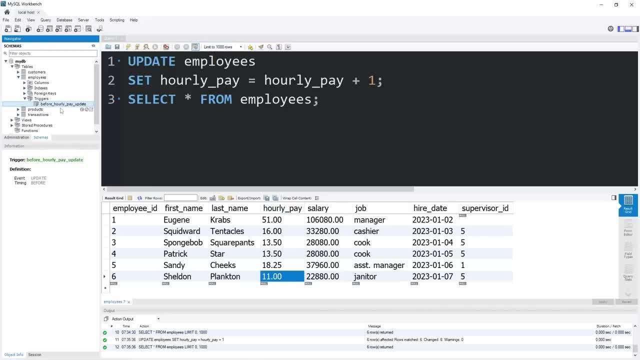 we have a trigger that only kicks in when we update an hourly pay. Okay, let's delete plankton. Plankton got fired. Delete from employees Where employee ID equals six. Select all from employees. Plankton is now gone. 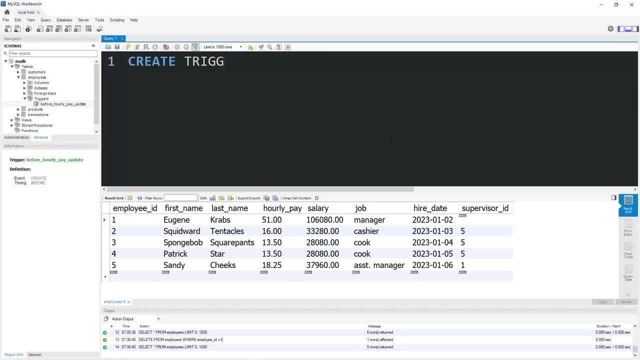 Let's create a trigger. Create trigger before hourly pay insert. Are we doing something after or before Before We're doing something before an event Before? are we updating, inserting or deleting? We are inserting Before we insert a new record on our table: employees. 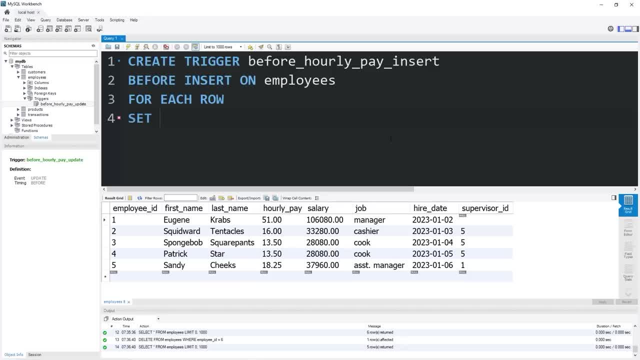 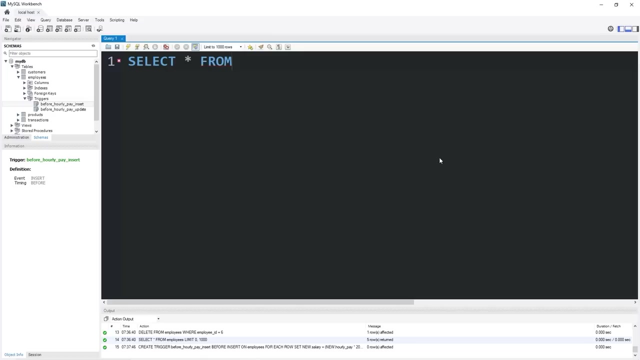 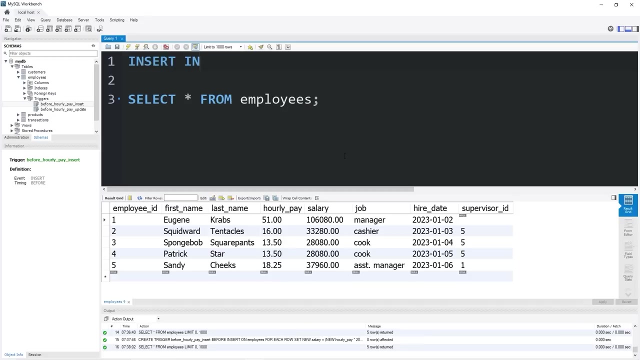 for each row. let's set the new salary equal to the new hourly pay times 2080.. Here is our new trigger. Let's take a look at our employees table Select all from employees. Let's insert a new employee. Insert into employees. 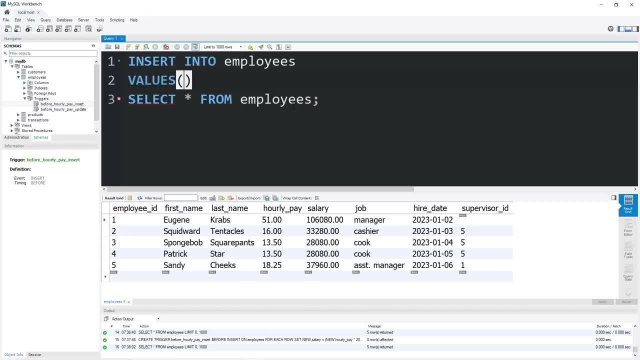 Values. I'm just going to follow these columns. Employee ID six: First name is Sheldon. Last name, plankton. Hourly pay is $10 per hour For the salary. I'm going to set this to null. Our trigger will kick in and set that. 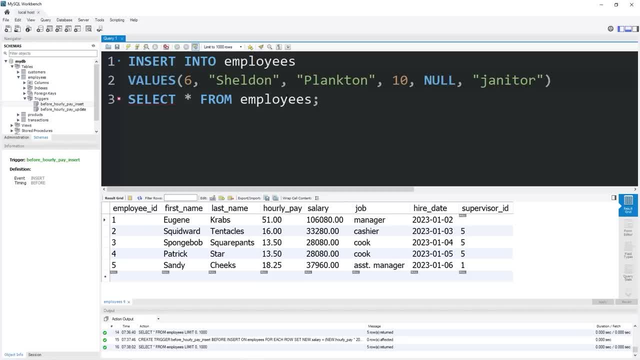 Position: janitor. Hire date: 2023, January 7th. Supervisor ID of five. Let's see if our salary is calculated. It was Plankton's hourly pay is $10 per hour, meaning he has a salary of $20,800 per year. 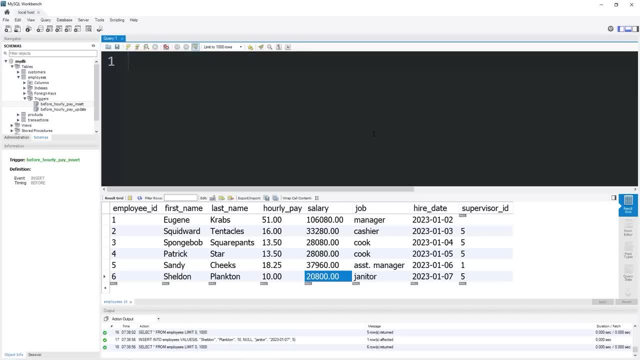 I do have a few more examples. Triggers are something you'll want to master. They're really helpful. We're going to create a new table. this time Create table expenses. Our expenses table will have three columns: An expense ID. 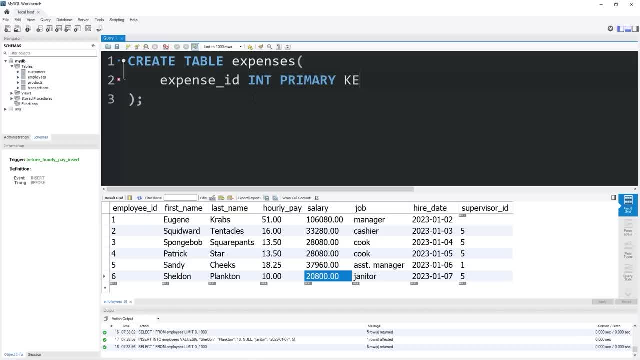 The data type will be int. This will be the primary key. You could set this column to auto increment if you want, but that's overkill for this topic. I would say I'm going to try and keep it simple: Expense name. 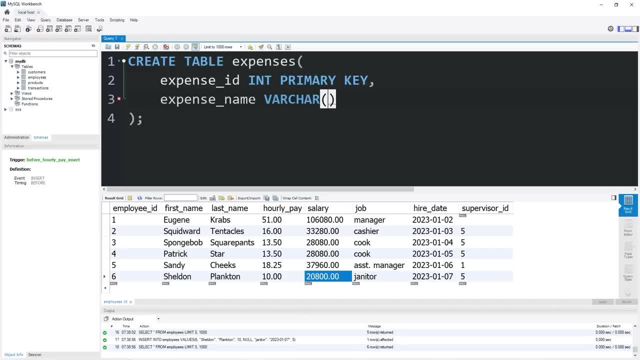 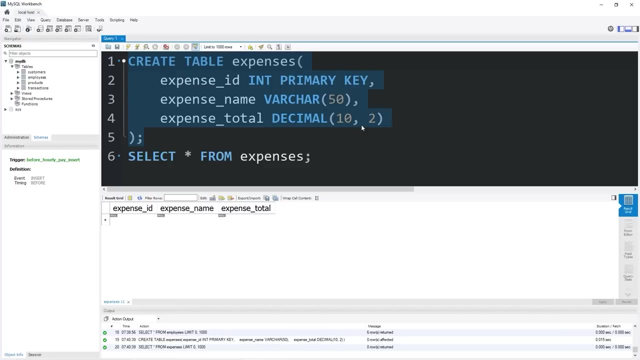 The data type is varchar. 50 is good, I suppose. Then expense total: I will set that to be decimal 10.. 10 digits, Precision of two is fine. Then let's select everything from our table expenses. Let's insert some values. 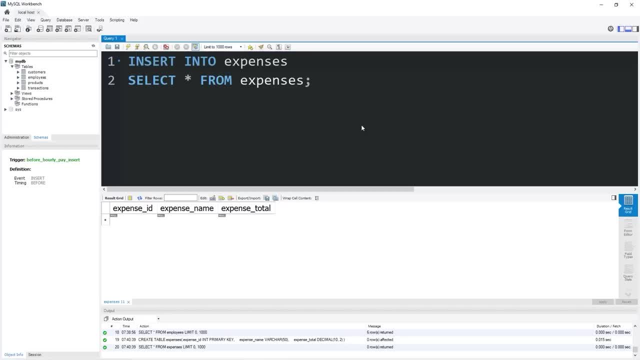 Insert into expenses. We have three rows: One, two, three. ID of one. The expense name is salaries For the value. for now I'm going to set that to be zero. The second row will be two Supplies Zero. 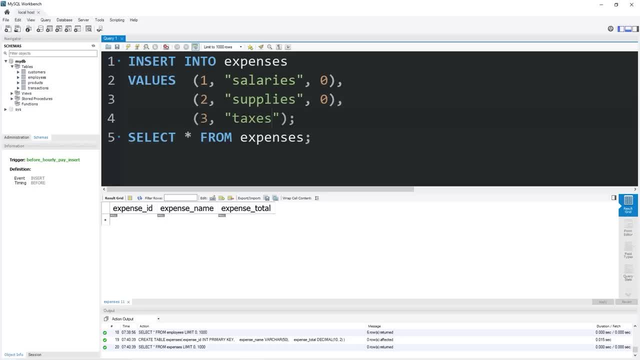 ID of three, Maybe taxes And zero. I will calculate the expense total of my salaries row. Update expenses. I will set the expense total equal to. I'll use a nested query: Select the sum of salary from employees where our expense name column right here is equal to salaries. 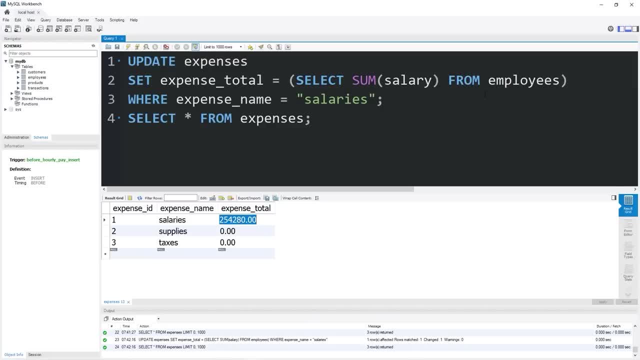 This is all of the salaries combined. from the employees table, The total is $254,280.. Whenever we delete an employee, we will update this value found within another table, our expenses table. So let's create a trigger. Create trigger after salary delete. 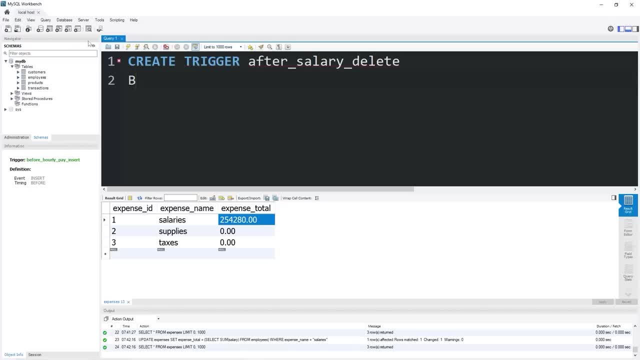 Are we doing something wrong? Are we doing something before or after? We're doing something after deleting a salary? After delete on employees For each row, we will update our expenses table and set the expense total equal to whatever the expense Total currently is minus that employee salary. 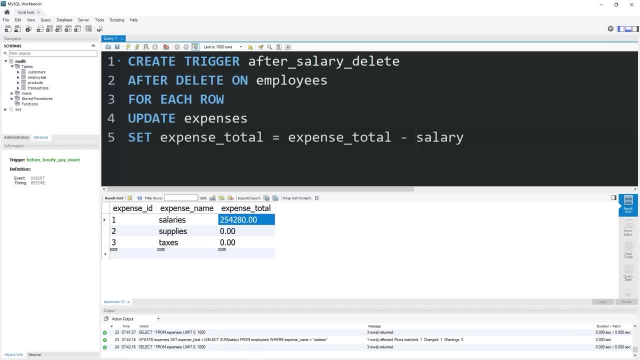 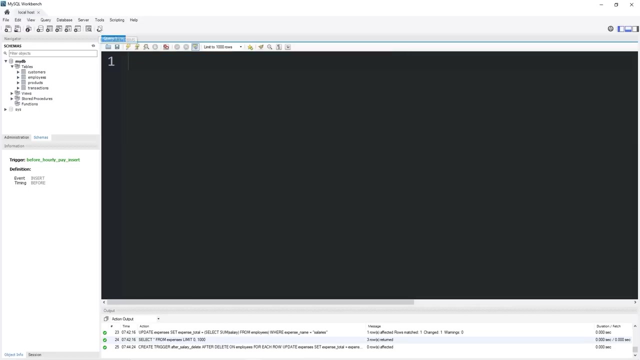 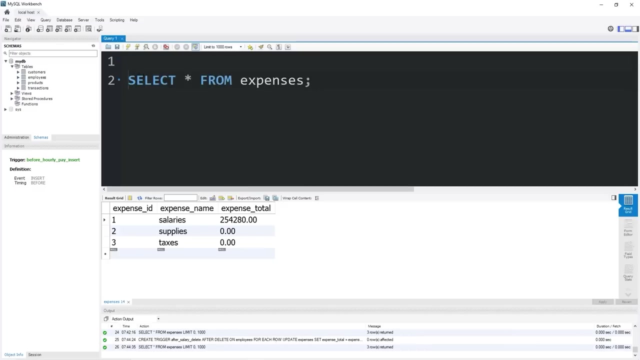 If we're deleting a salary, we will refer to that salary as the old salary. Then add a where clause where expense name equals salaries. Okay, We have created our trigger. Let's take a look at our expenses table. I'm going to delete plankton again. 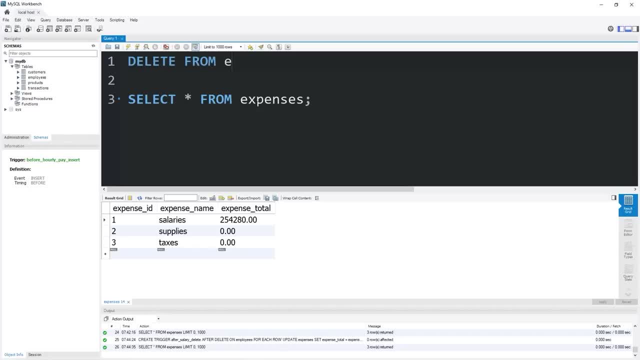 He's fired. Delete from employees where employee ID equals six. That's plankton. Then select All from expenses. Look at that. Our expense total changed. It's now $233,000.. Let's create a trigger that will update our salaries. 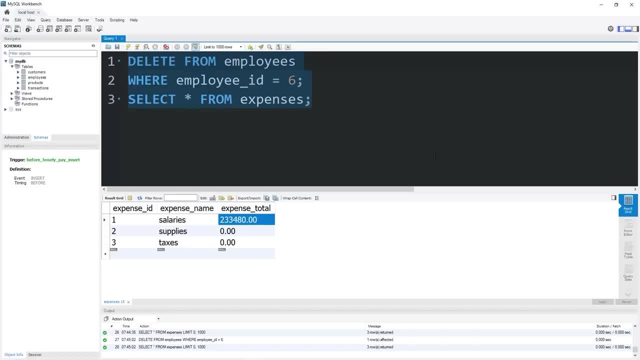 Whenever we insert a new employee, Create trigger after salary insert. We're doing something after this time, after an insert on our table Employees, for each row We will update our expenses table. We will set the expense total equal to the expense total plus the employees. 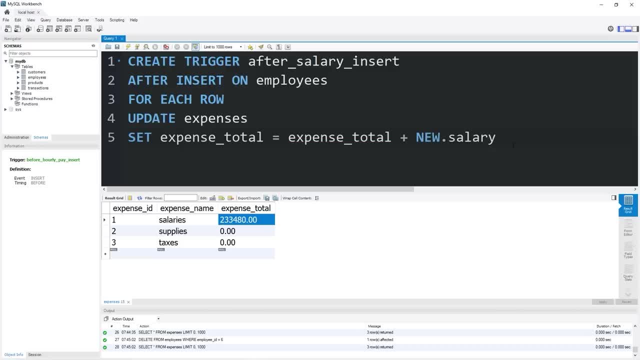 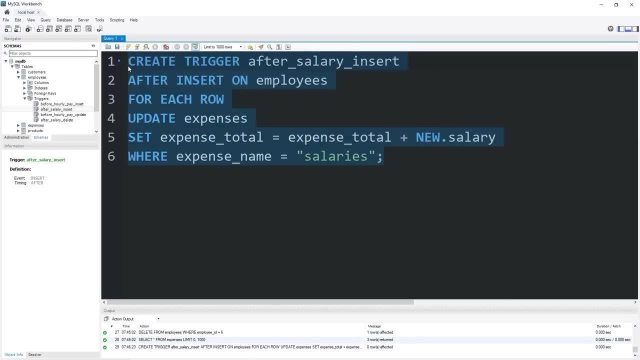 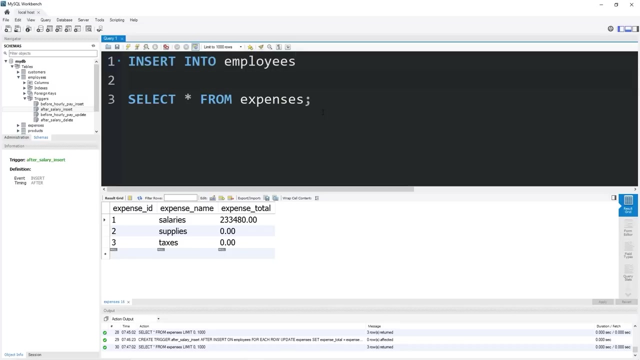 New salary, New dot salary Where expense Name equals Salaries. Let's insert a new employee. Let's take a look at our expenses table. Select all from expenses. We will insert a new employee, Insert into employees Our values. 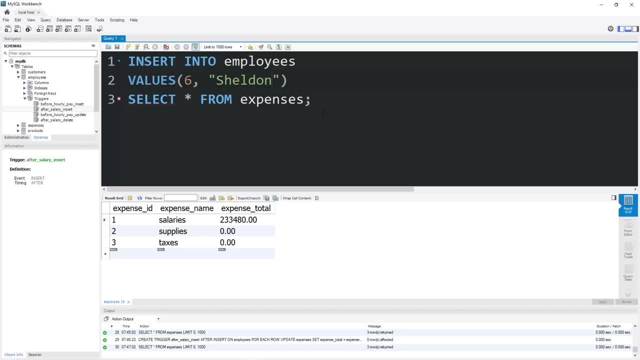 Employee ID six. First name is Sheldon. Last name: plankton. Hourly pay of $10 per hour. The salary will be null. That will be calculated automatically with the trigger Position is janitor, Hire date 2023-01-07 and a supervisor ID of five. 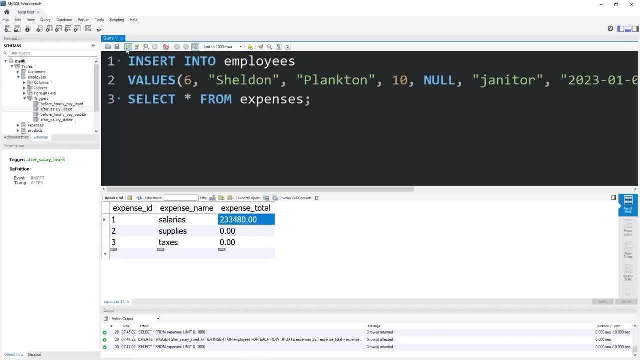 Let's see if this expense total will change, which it does When we insert a new employee or, specifically, a salary. our expense total of salaries will be updated. One last example, then. I promise we're done. Let's create a trigger that will update this value when we change an employee's salary. 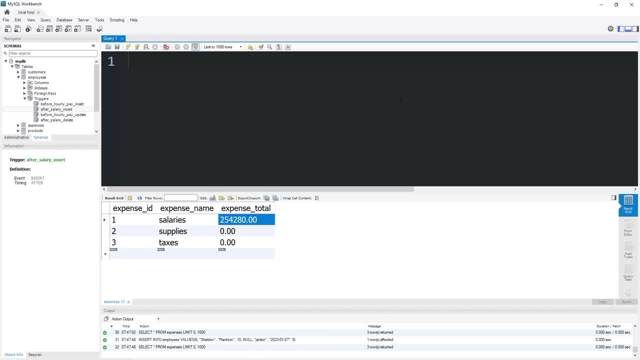 And that will probably be the most complicated one. Let's create a trigger. after salary update. We're doing something after we update on our table employees for each row. Let's update expenses: Set the expense total equal to the expense total plus the employees. 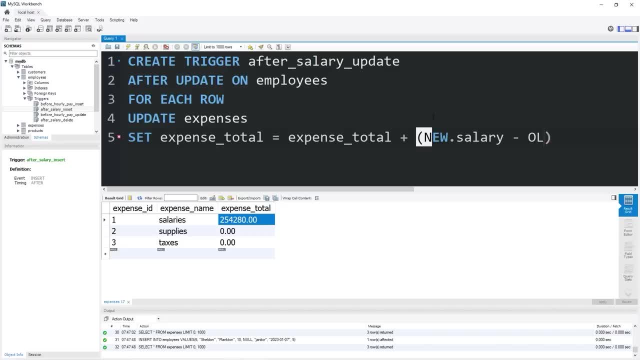 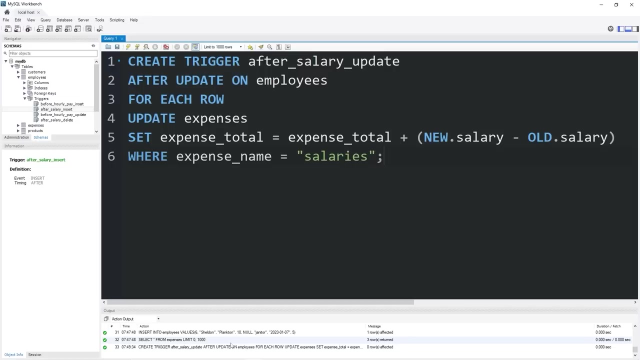 New salary minus the employees old salary. What's the difference? We'll find the difference between the employees new salary and their old salary. Add that to the expense total Where expense name equals salaries. We have created our trigger. Let's select all from expenses.